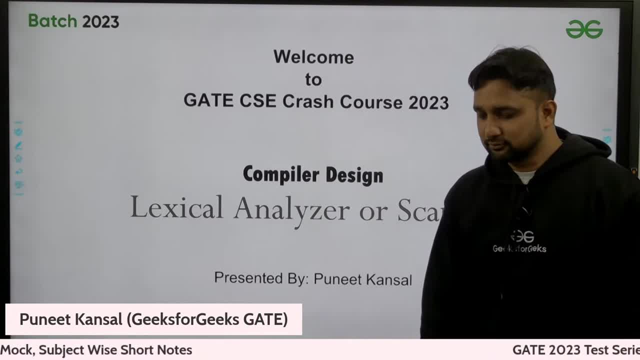 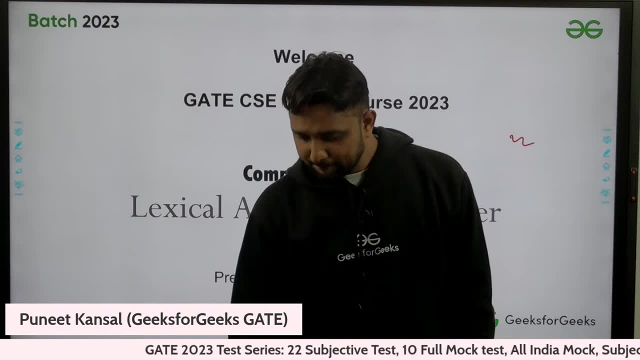 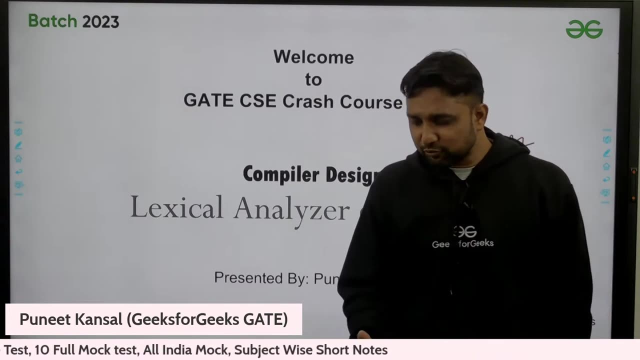 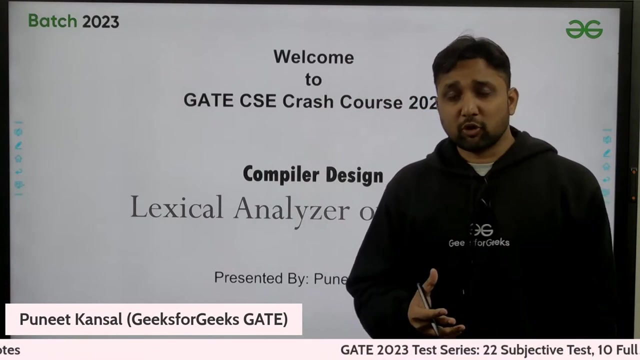 please write in chat Confirm me so that I can continue Anyone. So meanwhile, I get the response from you people. So let me tell you how this GATE crash course launched by the GEEKS4GEEKS is helpful for you people, How this can help you in your 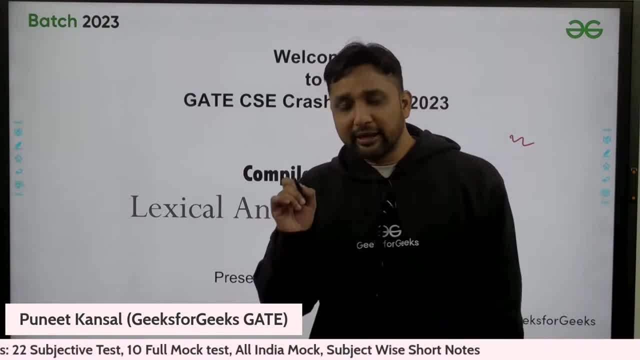 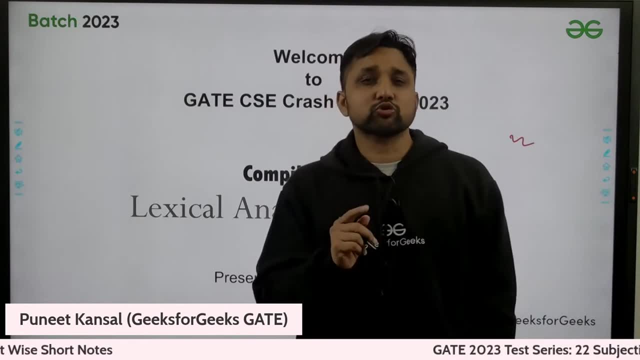 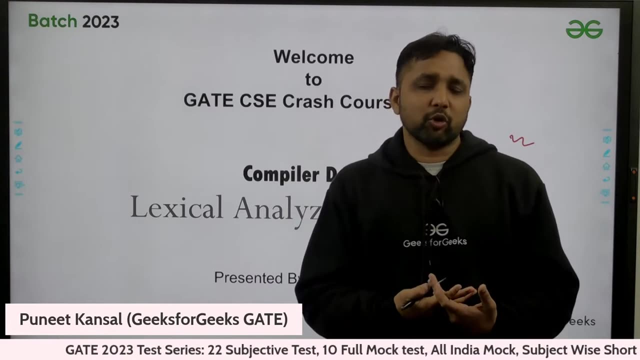 GATE preparation. So actually this GATE crash course is designed for, specifically for two types of students, Two types of students. One is those students actually who are not prepared yet, who are not serious about the exam or maybe they don't get time They want. 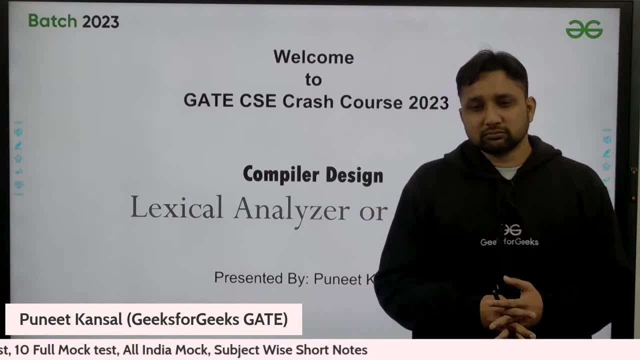 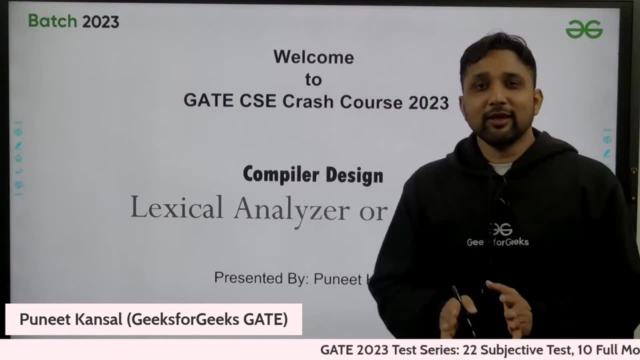 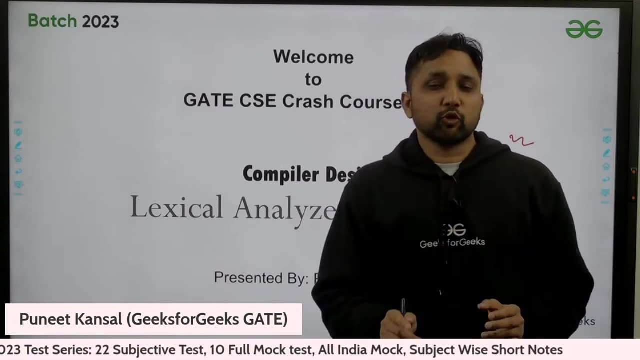 to crack the GATE exam, but they don't get time and they are not sure that they will clear the exam or not. They will clear the exam or not- I am using this word. Okay, So this GATE crash course actually will make sure to the students that those are not sure. 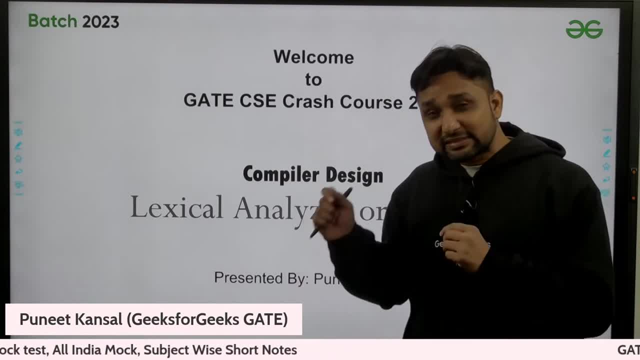 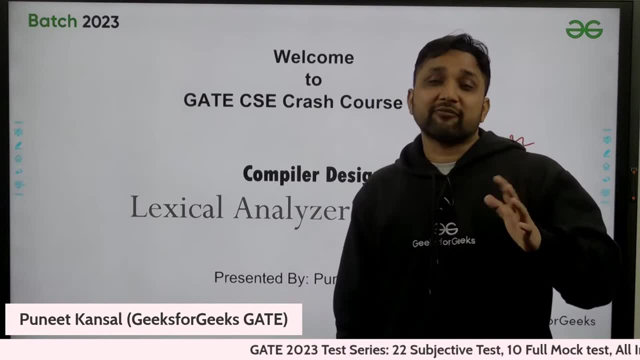 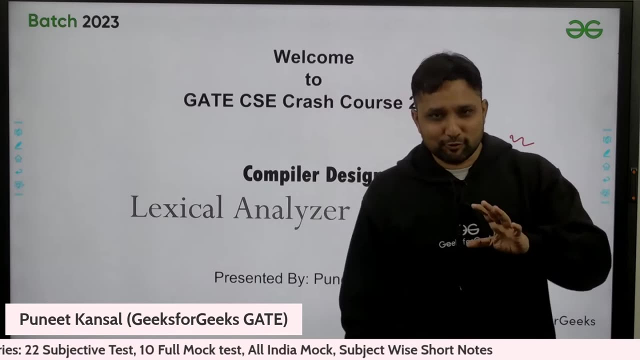 that they will be able to clear the GATE exam or not. This complete GATE crash course will ensure you that at least your GATE exam will be cleared. After taking this course, your GATE exam at least will be cleared. I am not talking about 60 marks, 50 marks, I am not talking about that, But at least your GATE exam will be cleared. 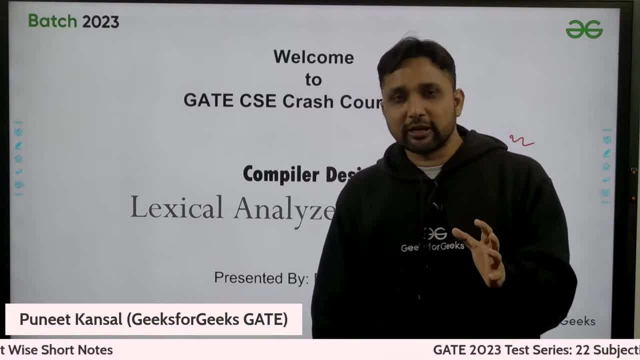 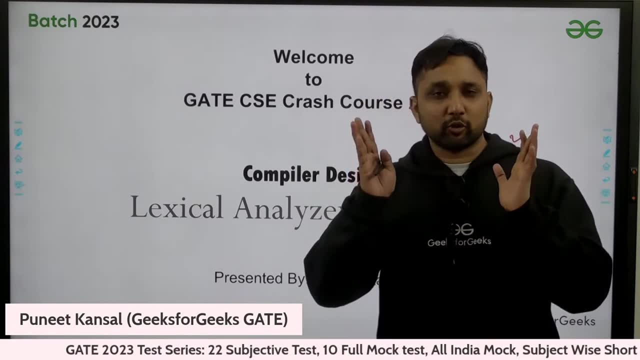 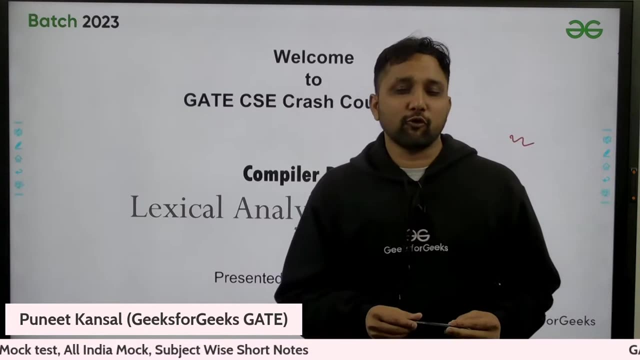 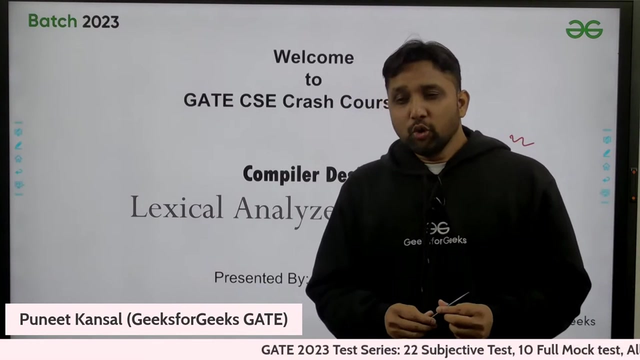 If you are not sure that you will be able to clear the GATE exam or not. Just you are interested to appear for the GATE exam and you want to clear it, So this GATE crash course is for you Okay. And the second type of student for whom also this GATE crash course can be helpful is those students actually who have prepared a lot. who have prepared a lot. They want to revise. 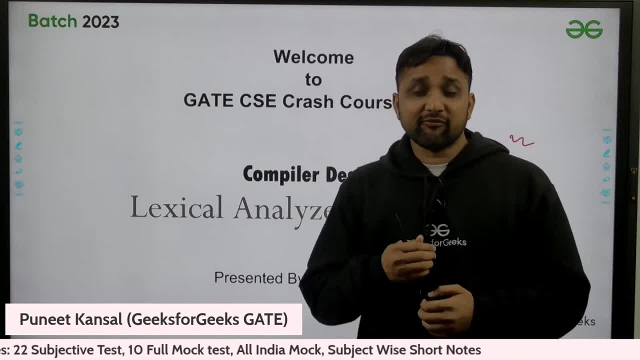 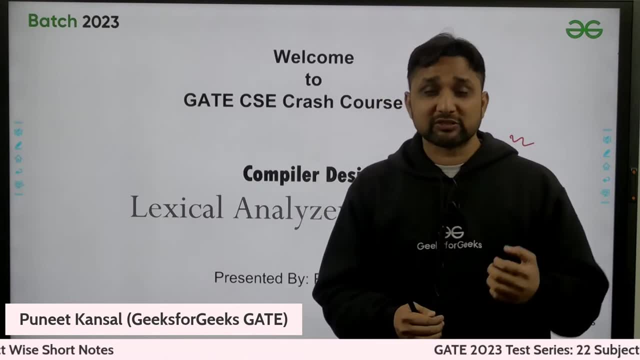 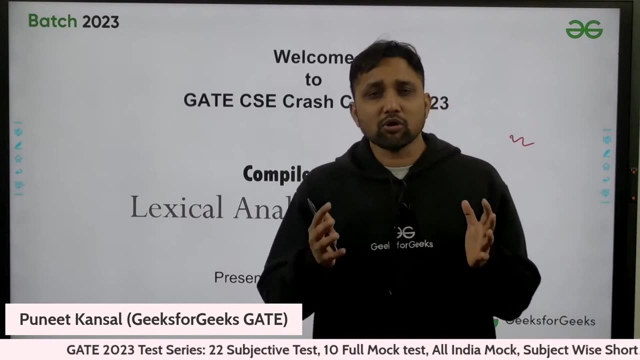 They want to revise now And I have to say that they want to revise the most important topics, or, another word I can use, most expected topics for GATE 2023.. Okay, So in this course, actually, we are covering most expected topics, most expected topics which are going to become in GATE 2023. 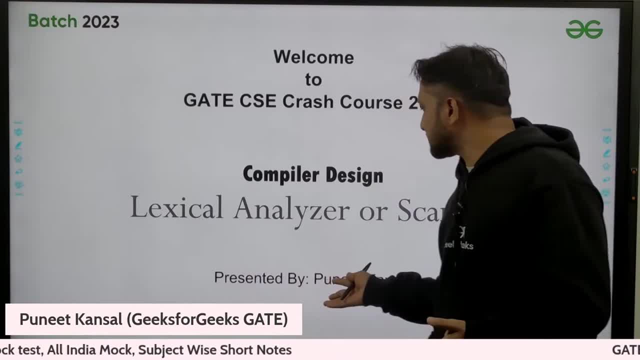 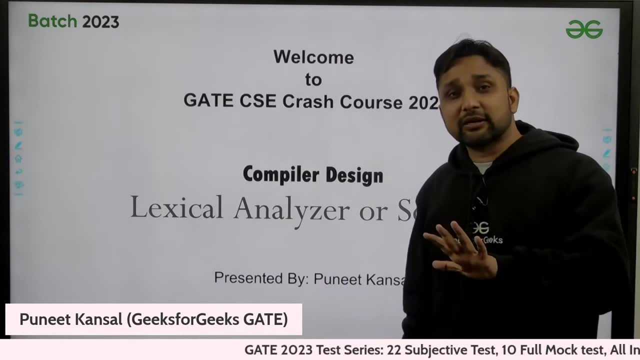 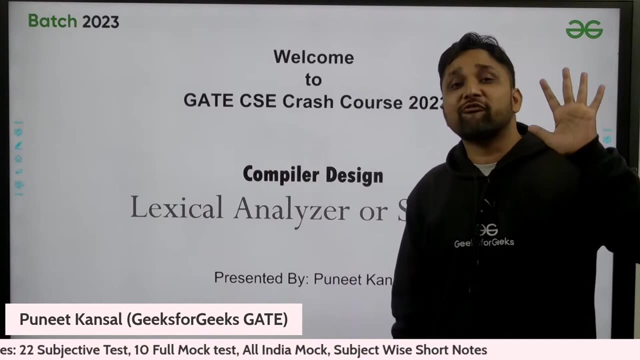 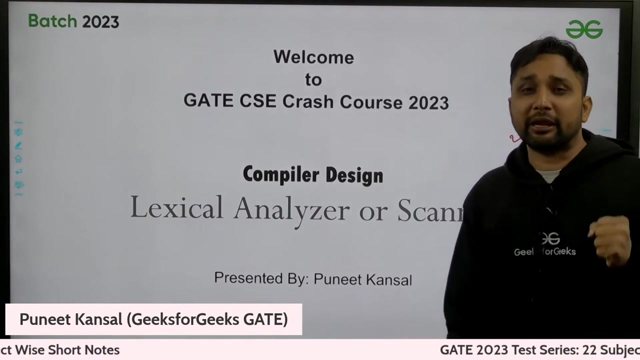 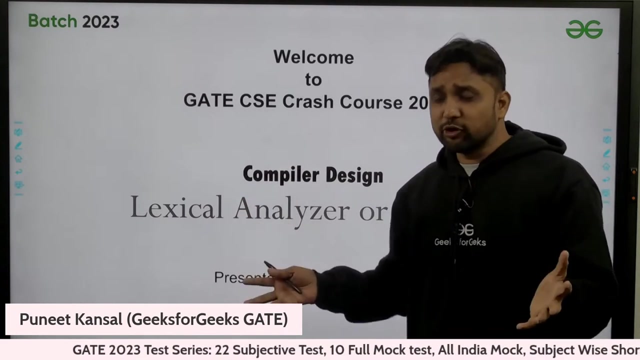 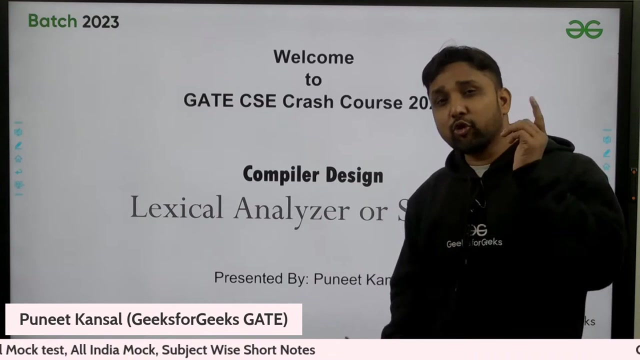 From every subject you can see that this is my first lecture from compiler design. After this first lecture, four more lectures will go in, and in every lecture There will be one important topic from compiler design. Similarly, from every subject this is going on- We are taking only five topics, five most important topics, five most expected topics which can come in GATE 2023. Okay, So only we are covering- we are not covering the complete syllabus here because we don't have time also And that will not be useful at this time for you people. What will be useful if you are serious about GATE 2023?? 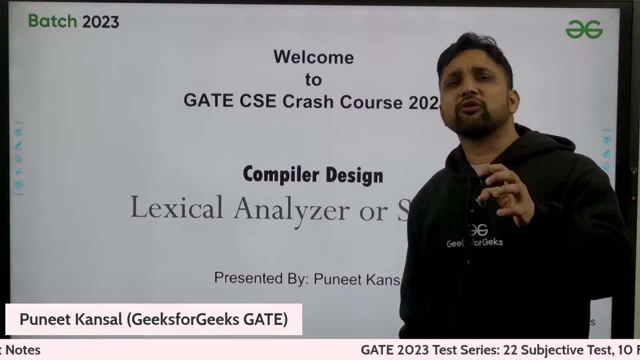 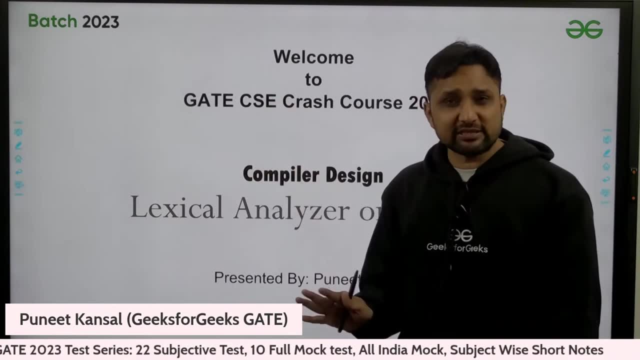 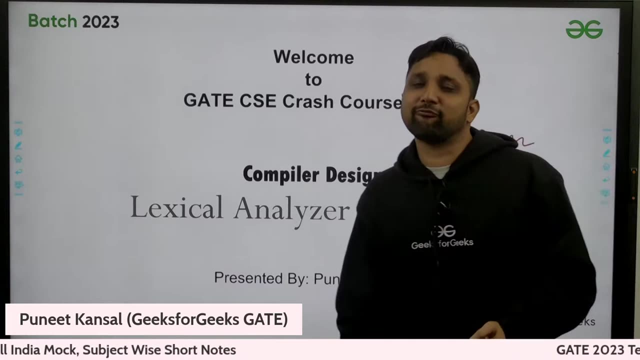 a great exam and you want to revise. it's better, you revise the most important, important topics. so here we will cover these most important topics from every subject, five most important topics from every subject we will cover. in every lecture there will be one topic and that will be helpful for you. 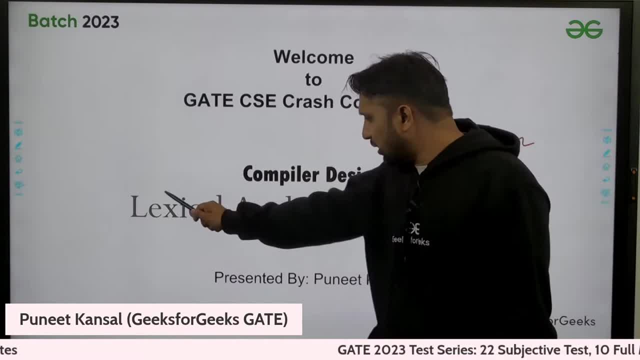 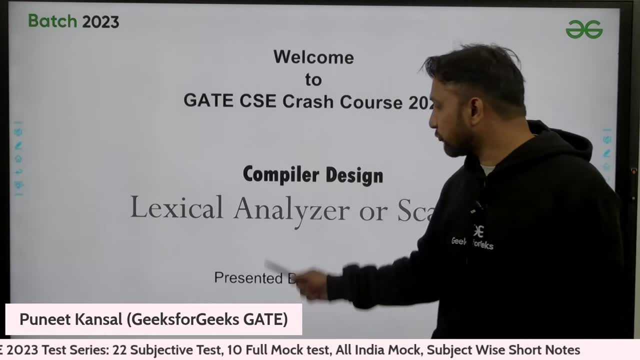 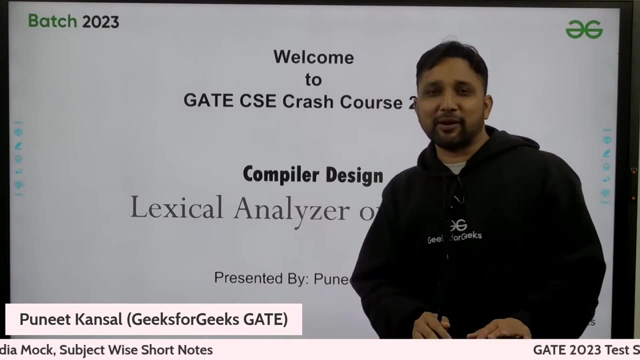 because this topic- let's suppose i'm covering- lexical analyzer. after this lecture. i can ensure you that you can attempt each and every question from this topic. after attempting the gate exam, you can again come back to this video, and you can. you can write in the comment that sir. 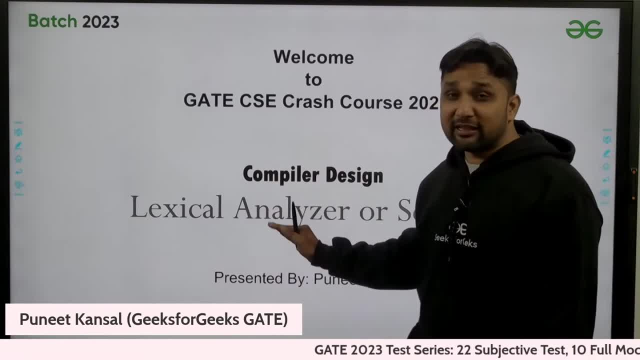 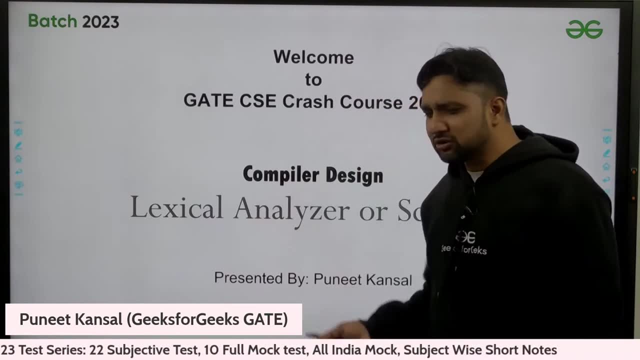 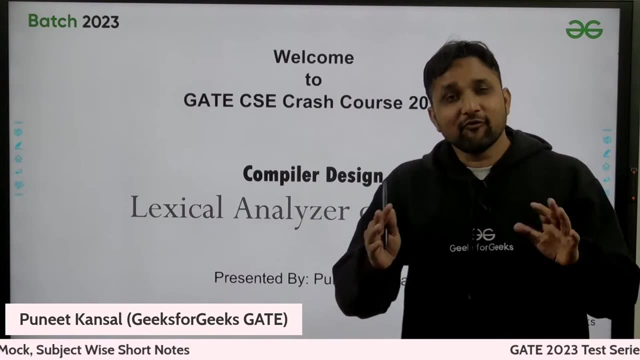 i was not able to attempt the question. if you have taken this lecture seriously, believe me, you will be able to attempt all the questions related to this topic, because we are not going to leave anything. see we, what we are doing here is in this lecture. we are not doing any magic. 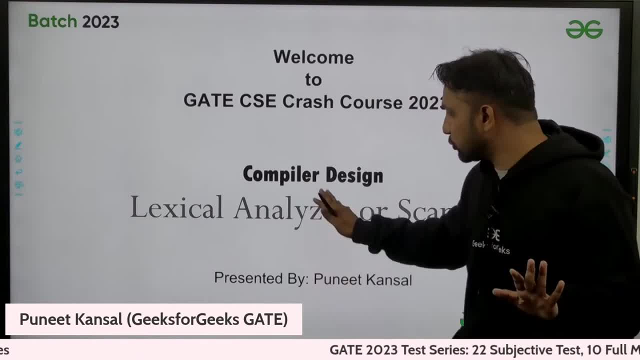 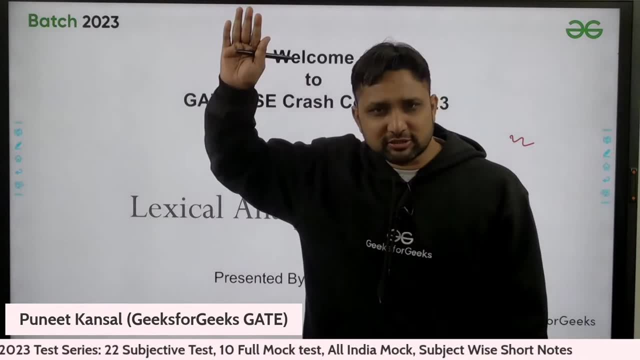 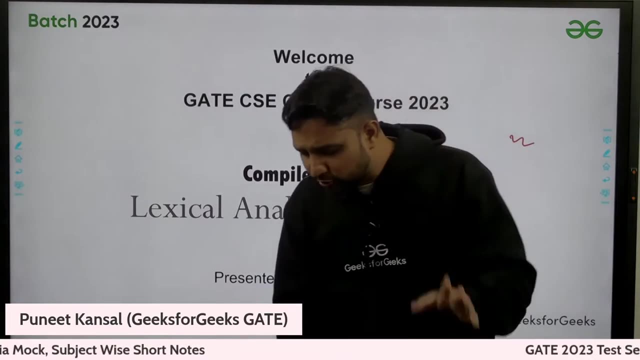 we are simply covering each and every concept related to lexical analyzer. after that, after covering the concepts, we will cover all the last 30 year gate questions. we will attempt all the last gate 30 year questions. and me alone will not attempt all these questions. you people will also attempt. 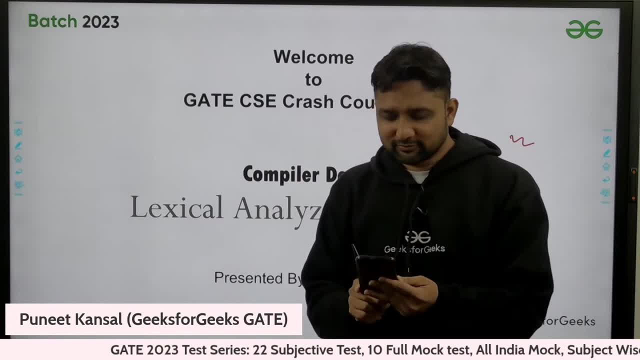 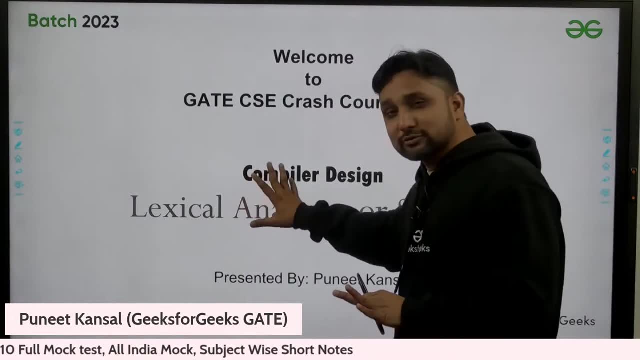 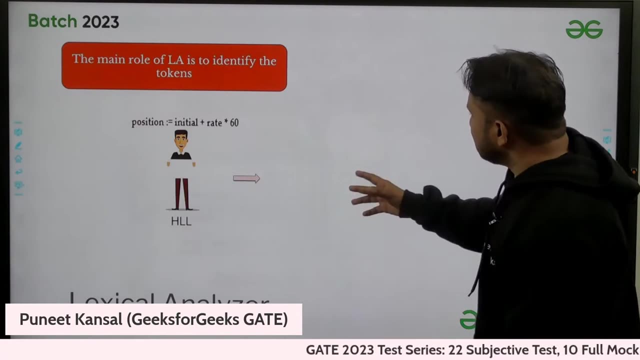 you people will also attempt with me, okay. so believe me, i will just tell you the concepts. i will tell you the concept of lexical analyzer, and then we have, i can show you right now also i can show you. so there are some uh easy way to explain the things. also i'm using that thing. 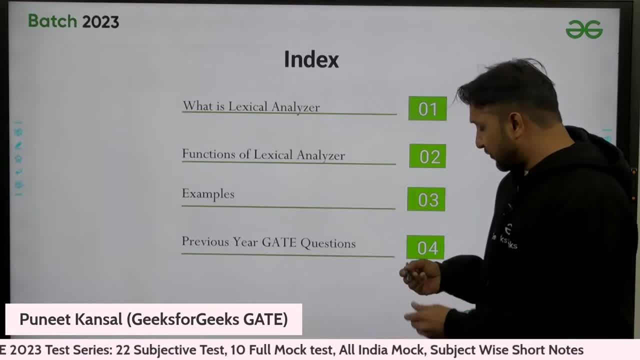 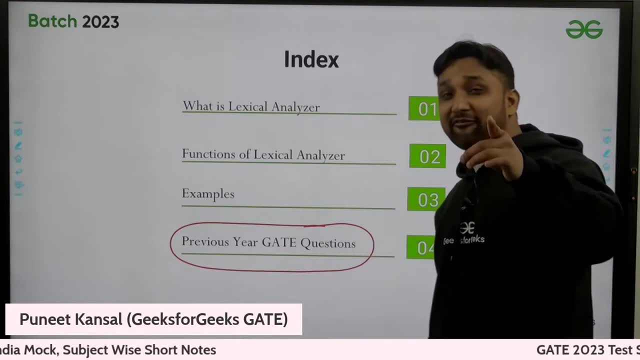 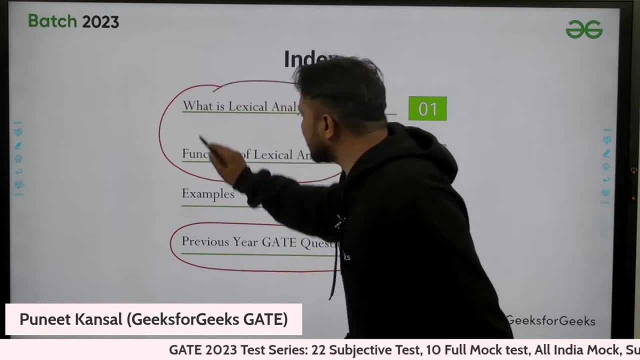 so, okay, i will show you. i will show you the. i will. we will cover various previous year gate questions and first i will ask you people, you people try with yourself and you people will be able to solve these questions. after i will cover the fundamentals, fundamentals and some examples. 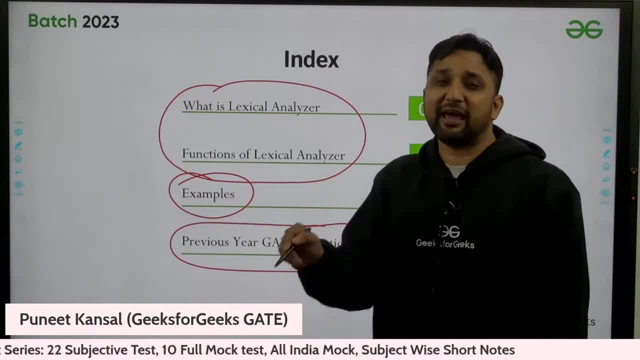 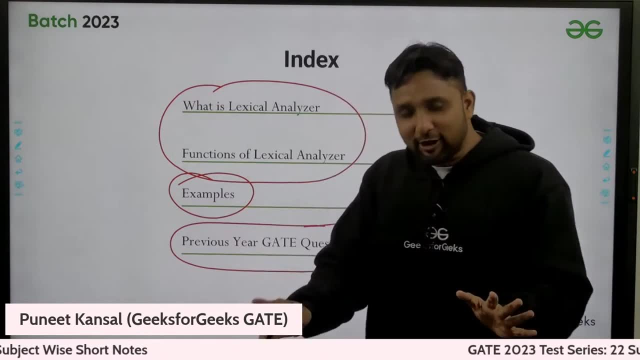 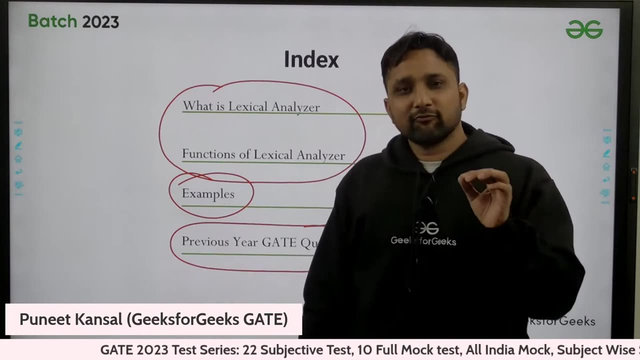 related to this topic. okay, this is what we are doing with every topic, every five most important topic in every subject. okay, so let me wind up this thing now and let me come back to my this today's topic. so the benefit for this complete gate, crash course. 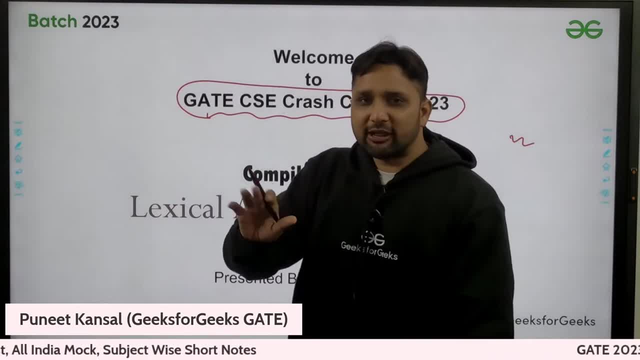 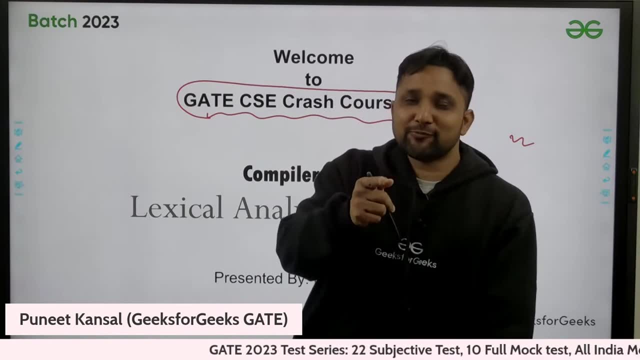 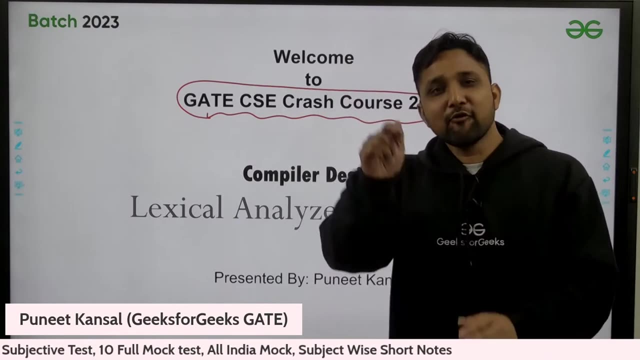 this will go for one and a half month maximum. we are covering five most important topic from every subject and if you are beginner, that is going to help you, because this course, i'm telling you, will ensure you to clear the gate exam. why? why? i'm saying this again: there is no magic. 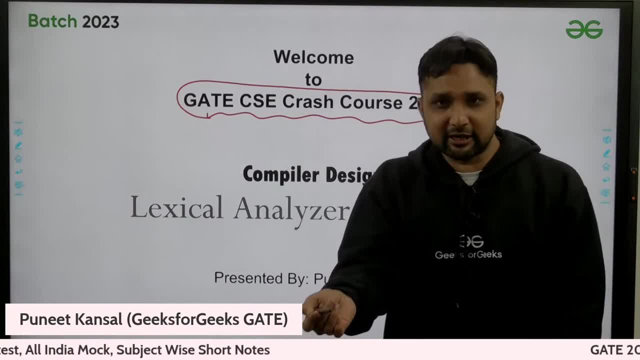 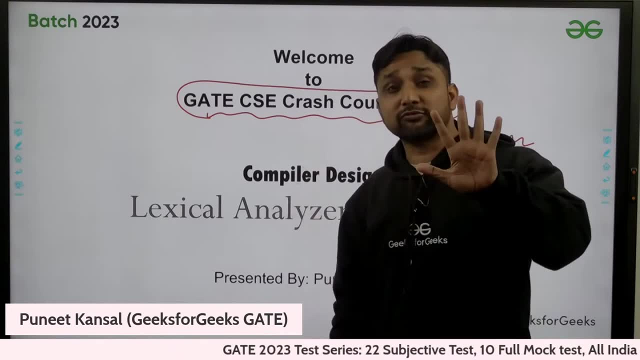 we are covering my five most important topic from every subject every year. the question is coming from there every year. maybe this year don't come. so another topic from: we have five chances with us. we have five chance with us. okay, even one chance will be get hit. five most important topic: 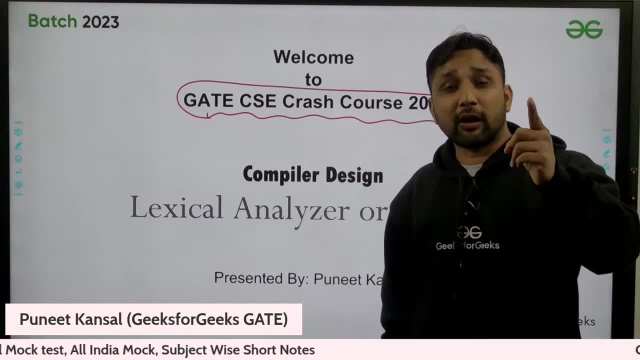 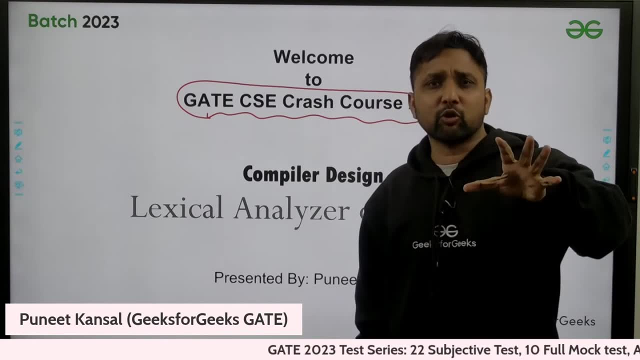 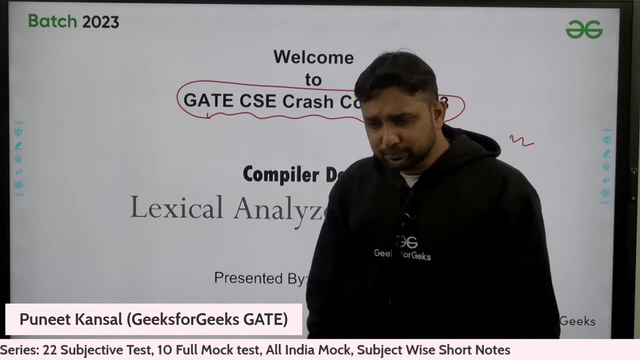 we are taking and even one chance get we hit, one topic will come you, you people will be able to attempt to 11 to 12 questions. 11 to 12 question means you will be able to attempt near about 30 marks paper. okay, near about 30 marks paper you will be able to attempt, okay, so so this will 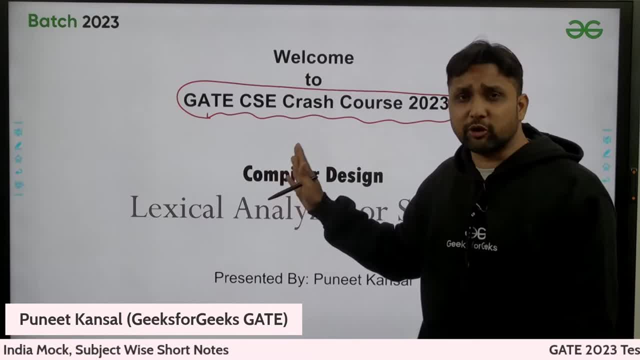 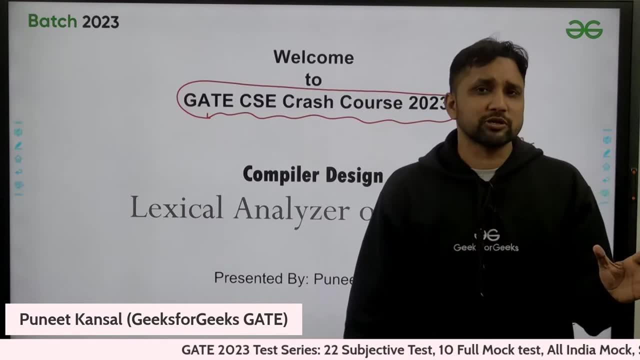 ensure you definitely. this is going to ensure you that this crash course is going to ensure you that you will clear the gate exam okay, and you are. if you are serious- already serious about the gate exam, you have already done so much- then this is a revision for you people, for the most. 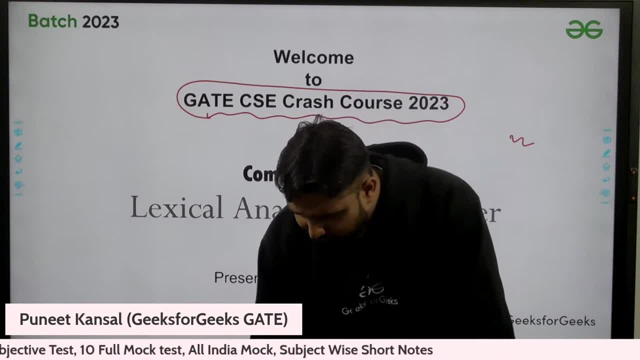 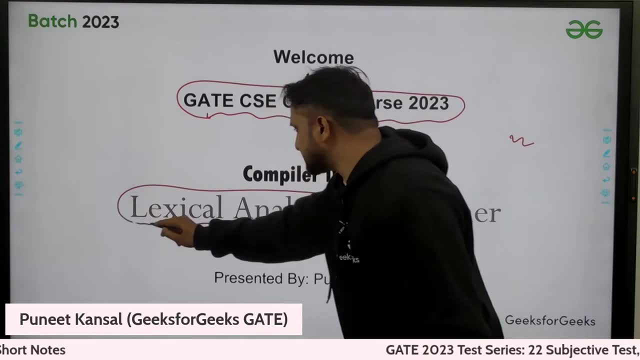 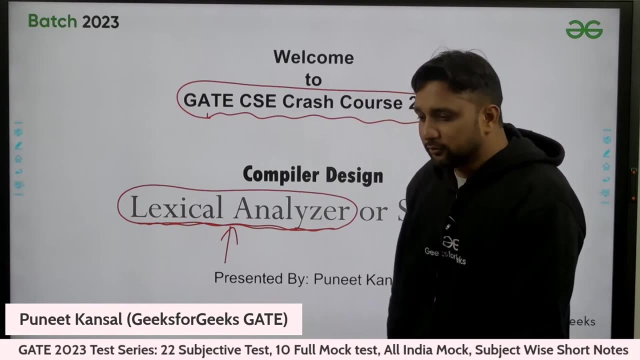 important topics. okay, so that's it from my side. so keep with me. and, uh, let's start with this, one of the most important topic in lexical, in compiler design, that is, lexical analyzer. before moving to this topic itself, let me tell you. okay, uh, one of the student asked me actually in in. 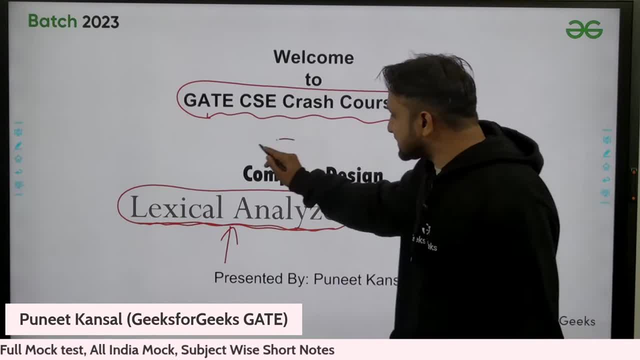 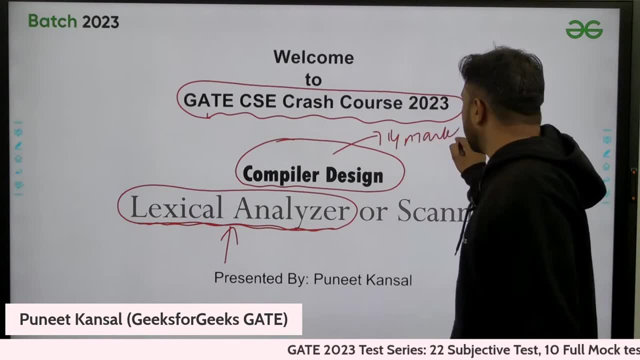 one of in one of the gate class. sir, can i leave this subject? compiler design bit is only of maximum of four marks. this is of more four marks paper. subject: actually four marks or sometimes six marks paper come from compiler design, sometimes only so. maximum time: four marks. 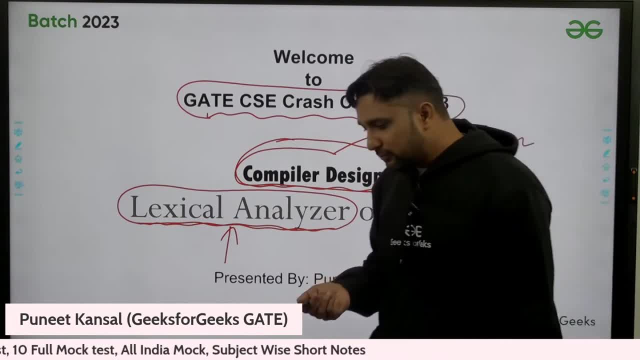 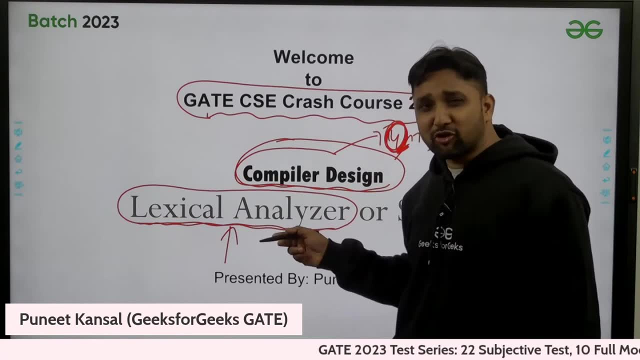 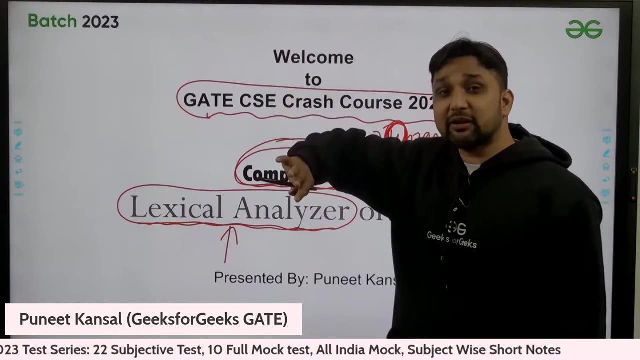 paper come from compiler design, so i. so what i can tell you people is that see, no doubt these, these are four marks okay, maybe you you can. first of all, you should not think that this is small number. okay, because this can make the difference of thousand ranks. this can one marks even can make. 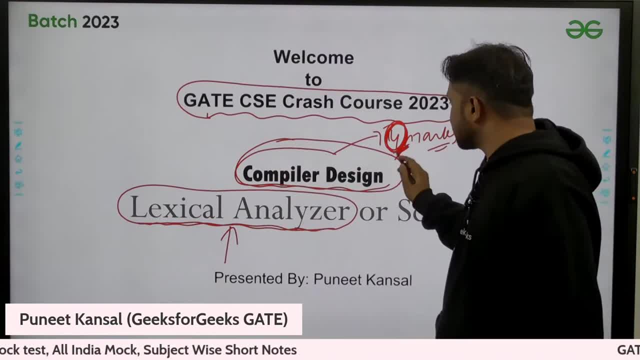 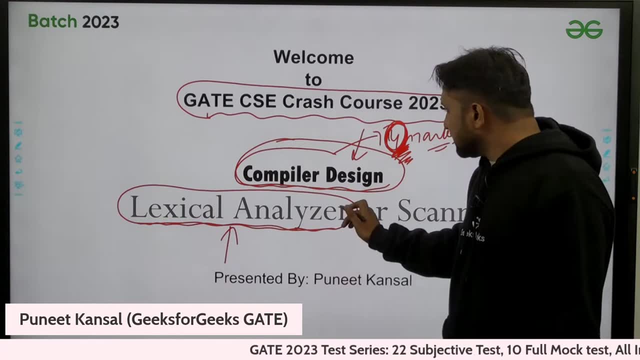 the difference of 100 of ranks. okay, so these are four marks first of all. maybe you get the easy question from here, only, okay. another thing, another thing i'm telling you see, i'm i'm covering only five topics. we are covering only five topics from compiler design. i'm not covering complete compiler. 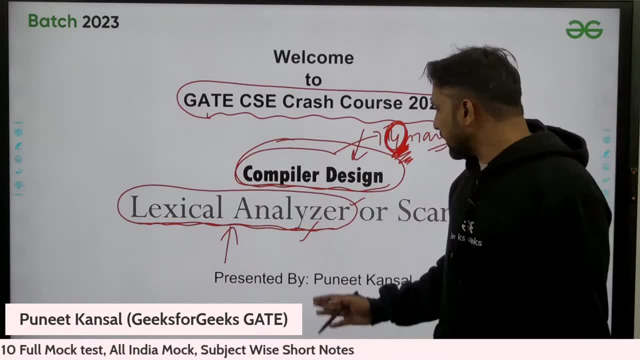 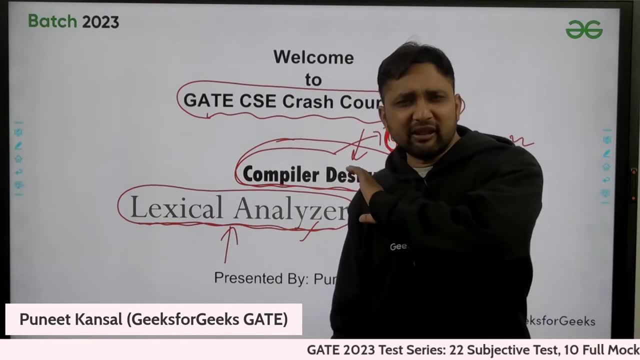 design. now i'm covering only five most important topics. so at least for four marks we can. we can study four marks paper and then we can study the other four marks paper and then we can study the five lectures. we can cover five lectures in which we are completely finishing those topics. so i'm 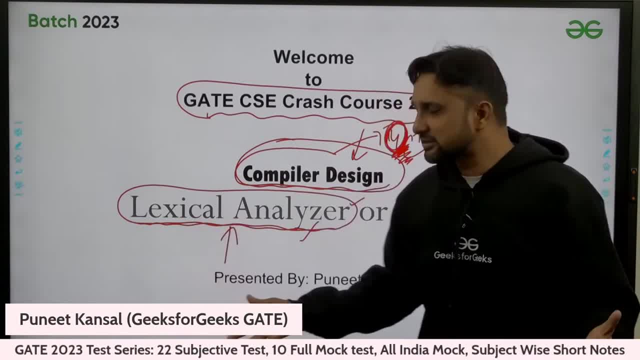 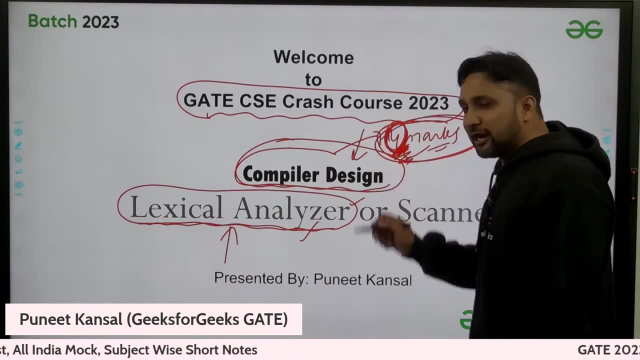 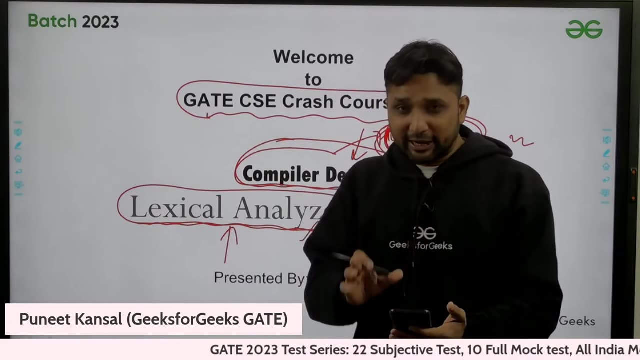 not asking you to come cover the complete compiler design. i'm just asking you to cover these five lectures of compiler design for these four marks. okay, so that is not a bad trade actually, and if you have any doubt- related to general doubts also, you can ask me right now and after. 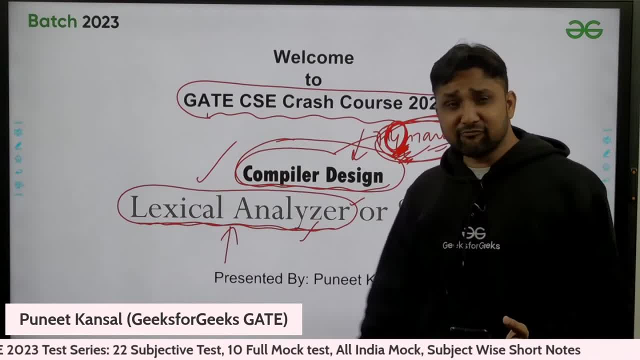 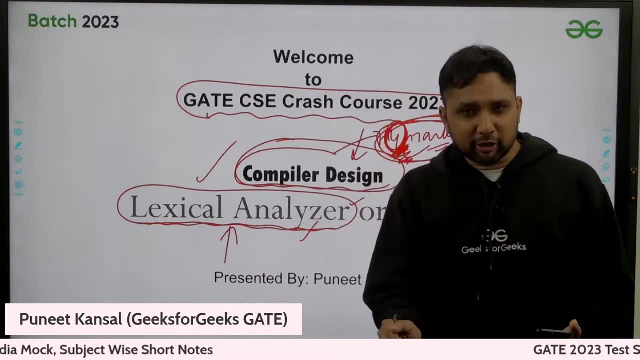 that i will start with my topic, today's topic: lexical analyzer. we will finish this topic. even you don't know anything, i'm not bothered about that- i will tell you right now, i will give you the information right now and you will. you will be people. you people will be able to solve the 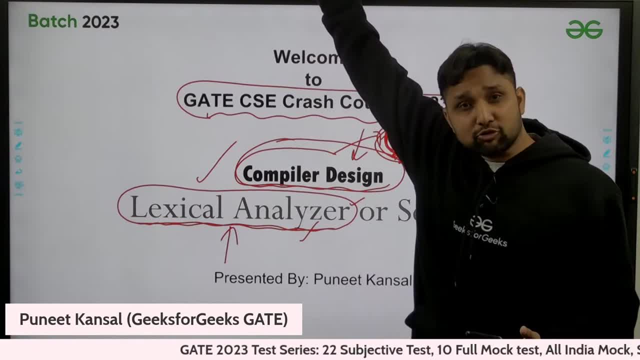 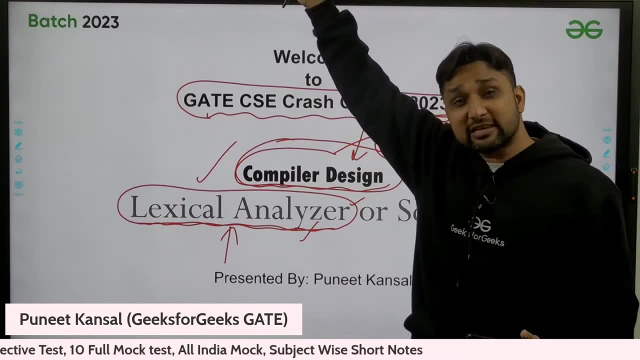 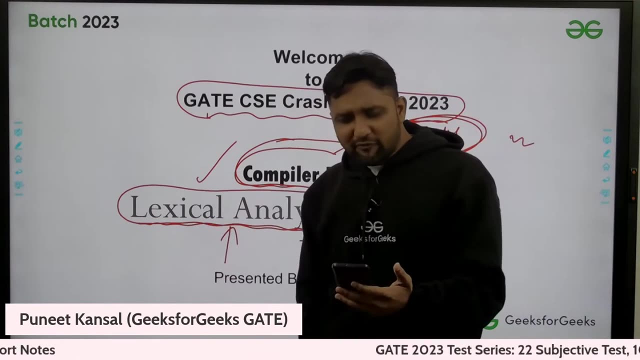 question right now, which question the gate previous year questions. these questions are not mine, my question. okay, these are great standard level questions which are which already come in previous exams and you people will be able to solve those questions, okay. so meanwhile, moving to this topic, if you have any general doubt related to this crash course or how you are going to be, 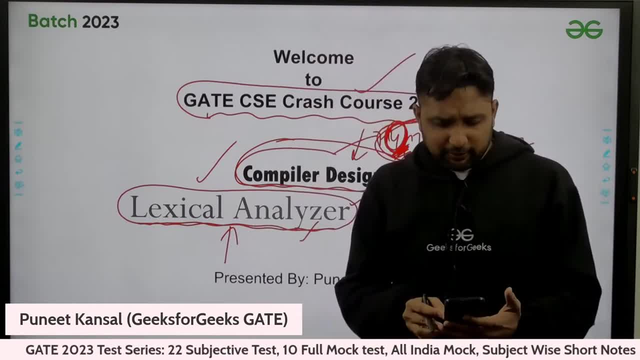 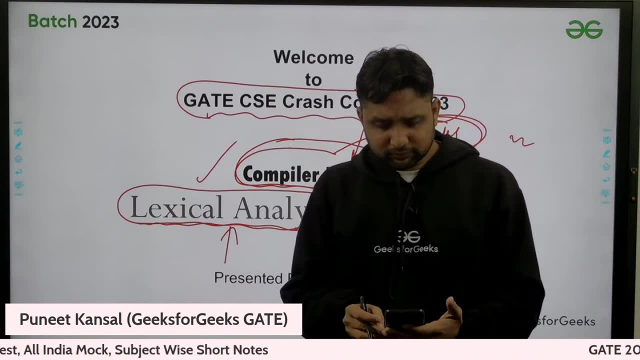 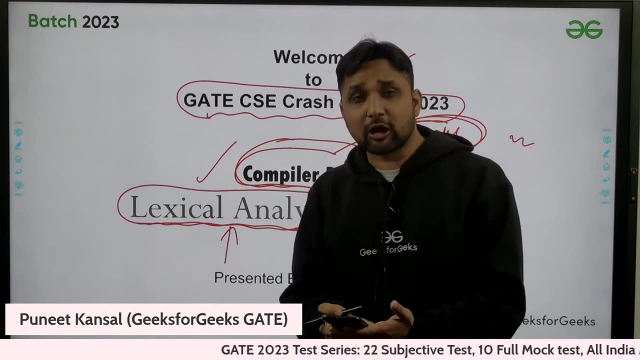 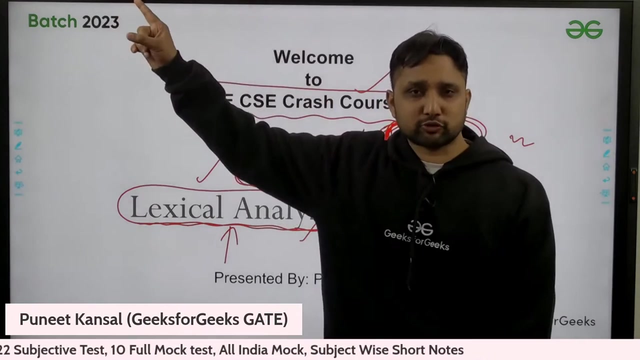 able to solve this course or how that can benefit you or anything. you can ask me. okay, then after 10 seconds i will move on. that sign up is asking: okay, can i watch if i'm starting this course now? see this course is designed. this is very beautiful question actually. this will help lots of students also. 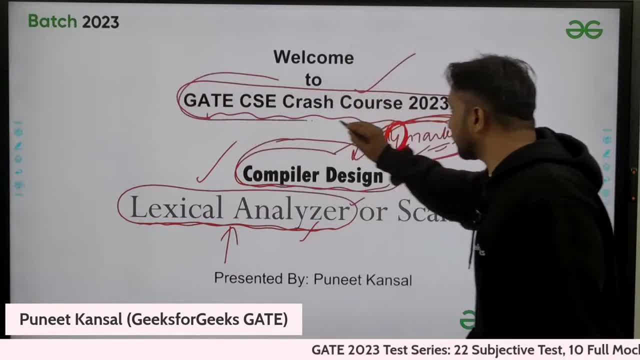 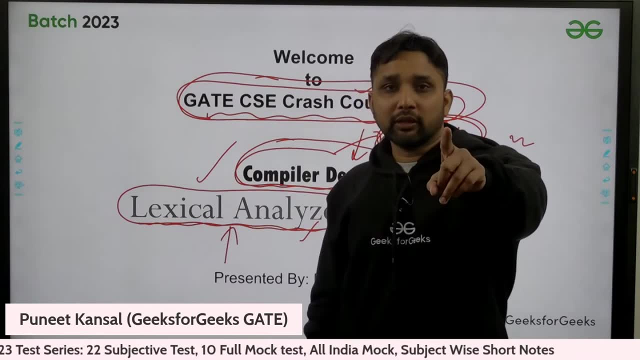 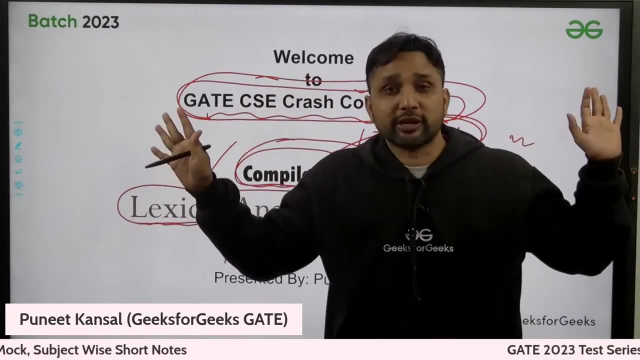 try to find out something that you will be able to do for yourself in this course. but so far it has been presented that every lecture of this complete course- i'm telling you every lecture of this complete course- is designed in such a way that even you are attending one lecture only, you can attend that lecture without knowing anything back. 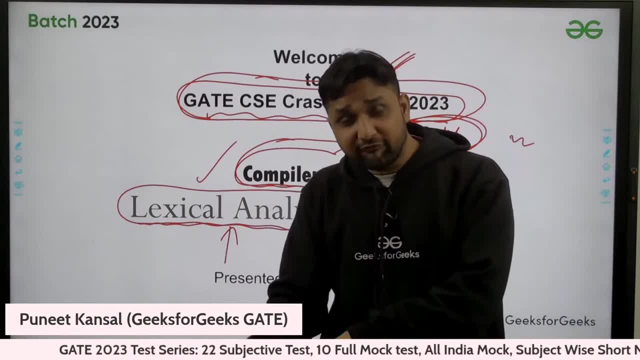 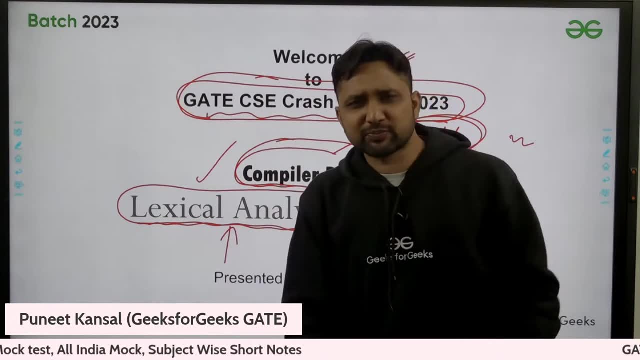 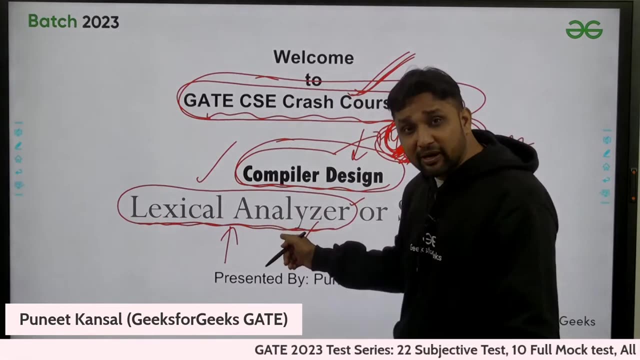 you can attend that lecture without knowing anything about that subject. okay, every lecture is designed in such a way in this, in this series, actually, complete complete means you do not, we don't expect you. you, you need any prerequisite for that every lecture. i'm talking about second. when second lecture will come of compiler design, i will not. 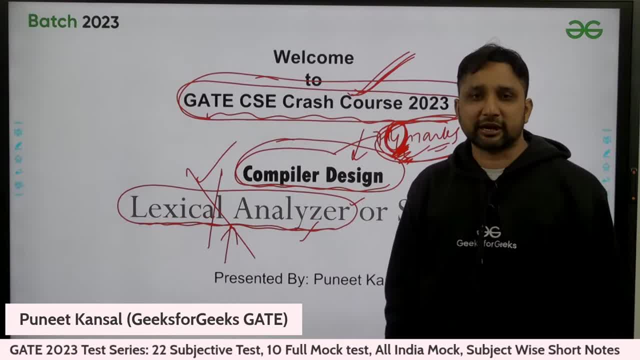 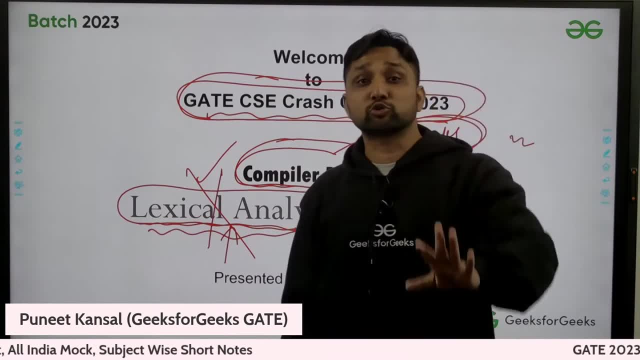 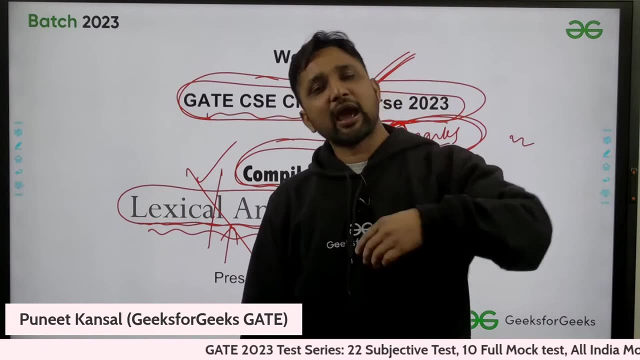 ask you about the lexical analyzer. i will not ask you about the lexical analyzer, okay. so even though i'm starting today, lexical analyzer, i'm not asking about the basic automata. also i'm. some people say that automata is the prerequisite of the compiler. okay, i'm saying, whatever will be required, i will. 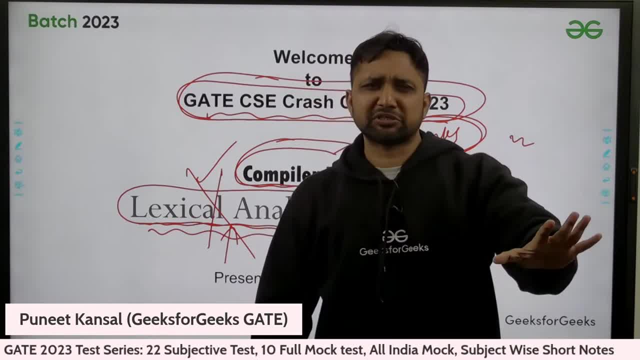 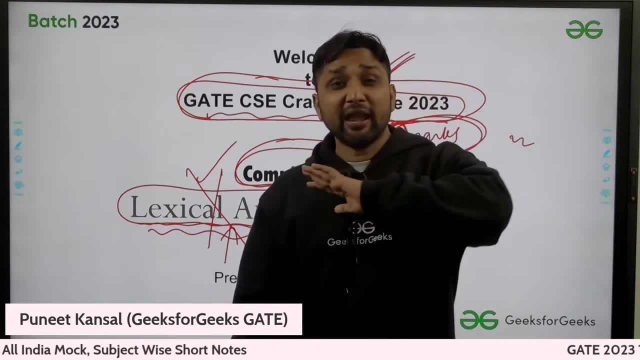 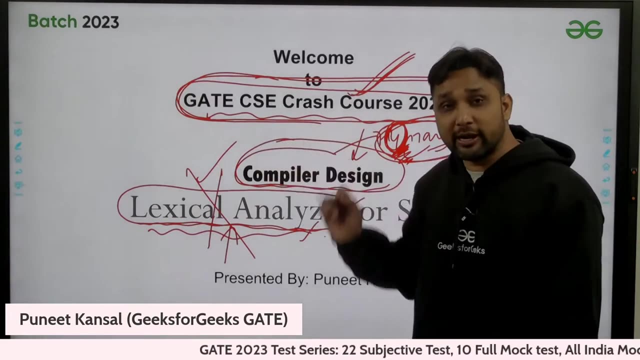 tell you right now, not too much information is required, little bit is required. i will tell you right now, i will finish it and you do not need any prerequisite for any lecture. i'm telling. i'm telling for any lecture in this course, not only about mine- for any lecture. okay, you can attempt. 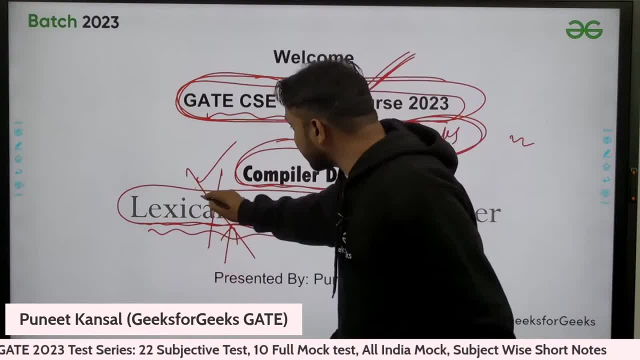 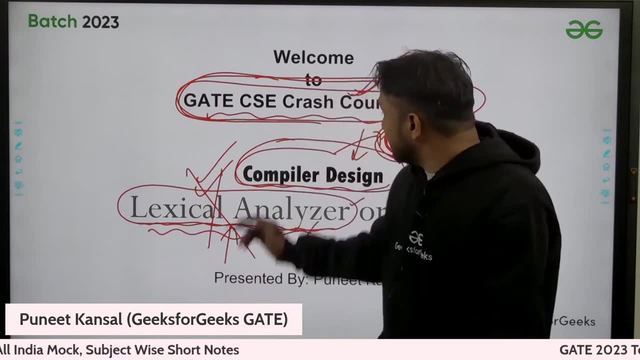 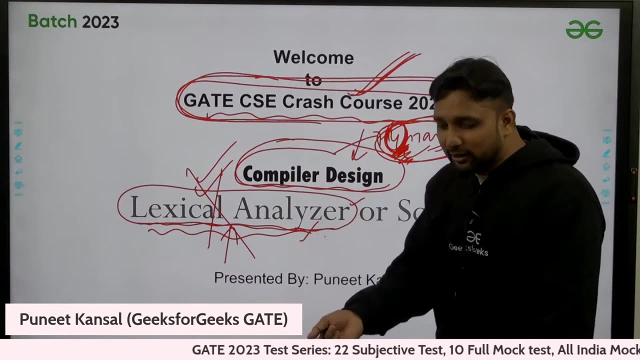 you can attend any lecture, you can finish, you can take that topic and you can finish that topic, okay, okay, and you can enroll in this course. this is free course, uh, free course. so if we are getting the free knowledge, and so you can register in the course, 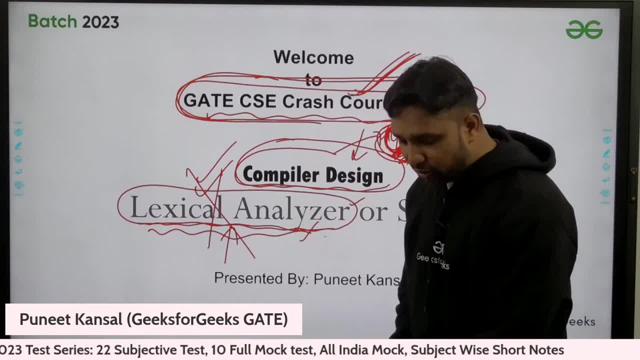 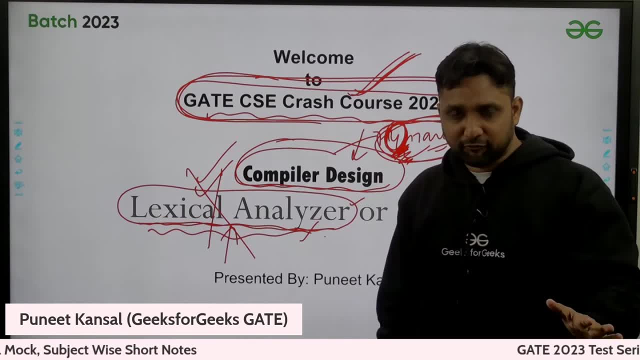 the link is already available so you can register over there if you have not registered every lecture. every lecture is just like individual lecture and that topic will be finished. forget point of view. okay, so let's start with today's class. so we are going to cover the lexical. 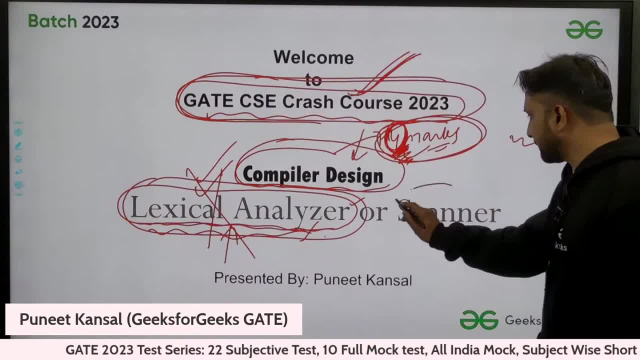 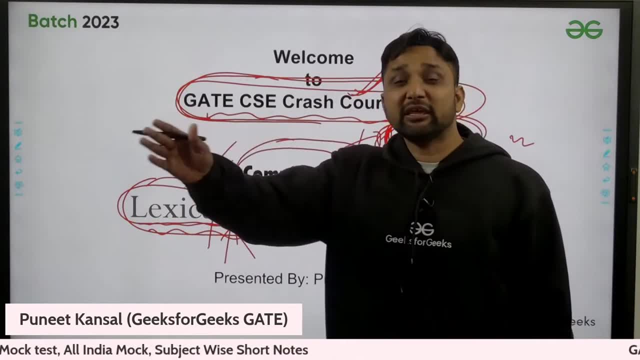 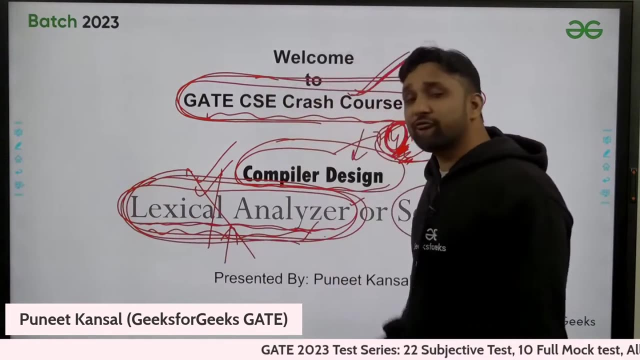 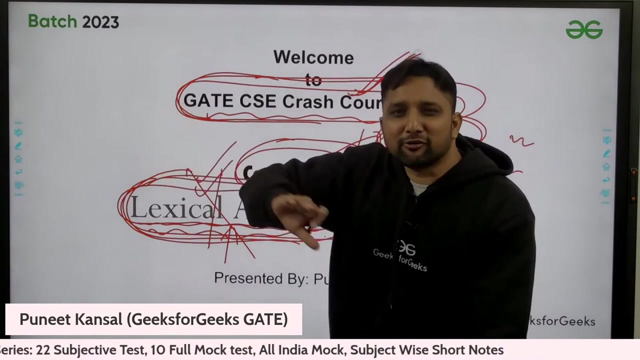 analyzer, which is also known as the scanner, scanner, scanner strings, that is going to scan, the scan your program, actually. okay, so lexical analyzer is the actually first phase of the compiler. that is the first phase of compiler. we have six phases in the compiler and this is the first phase of compiler. in five lectures we are going to cover 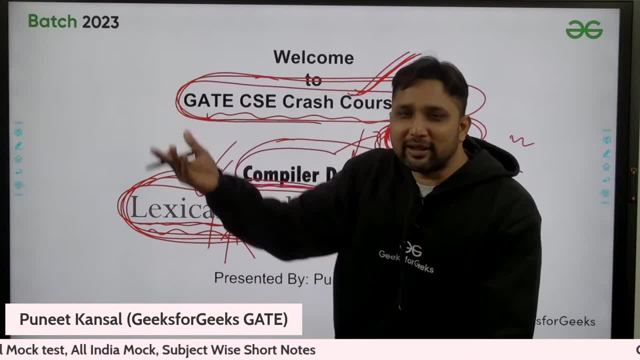 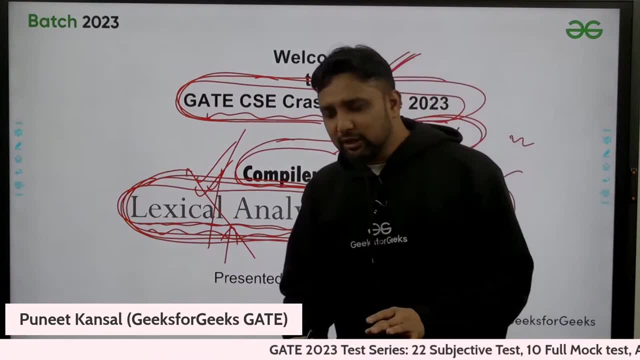 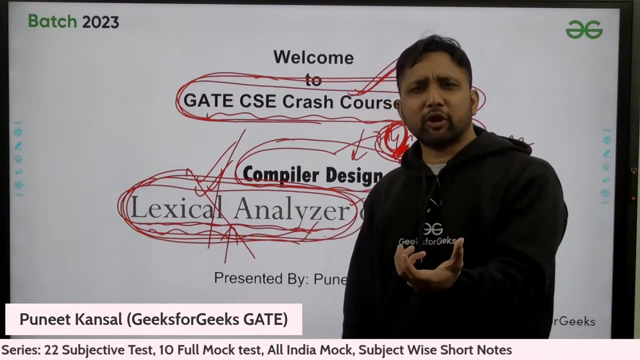 the most important phases of the compiler. actually, okay, so this is the first phase of the compiler and we will finish it today only okay. lexical analyzer: actually, in lexical analyzer we take the high level language as an input. we know that what compiler do take the high level language as. 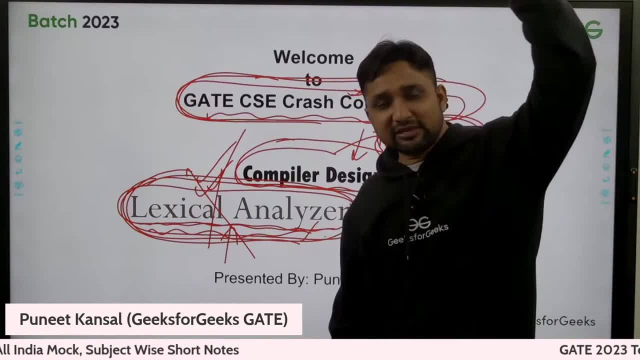 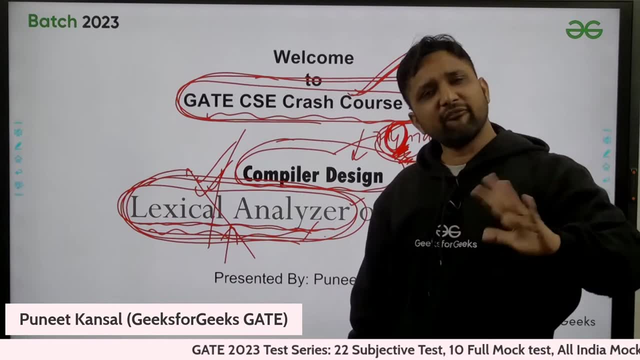 an input, convert into low level language. for example, if we are giving c, if you are writing code in c language, that will be converted into the assembly language. if you are talking about the c compiler, okay, every compiler is doing like that, converting high level language into low level language. okay, so this is the first phase. 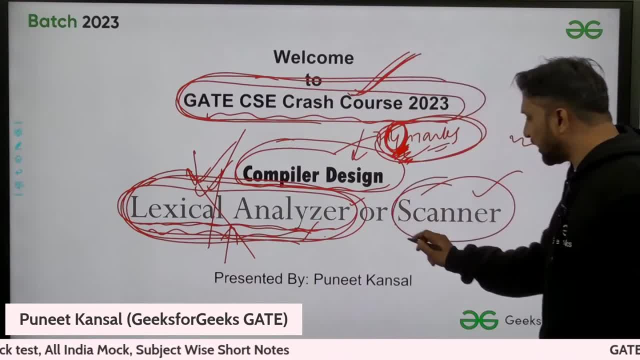 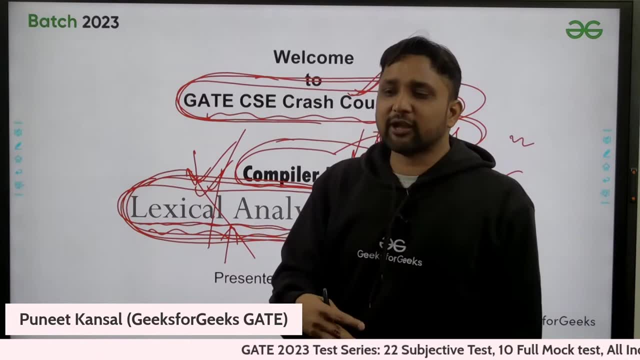 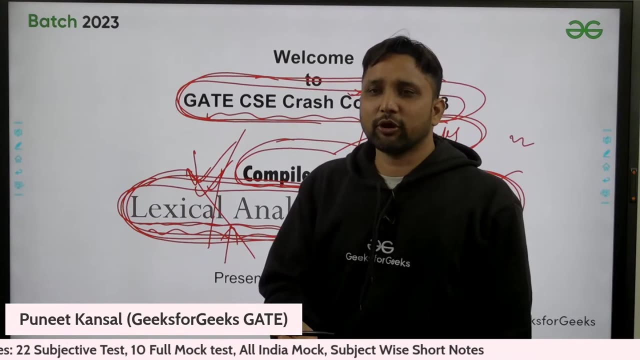 which is taking the high level language and which is scanning the high level language, scanning the high level language and actually finding some information, finding some information for the compiler. what information we will discuss that, like tokens, that is finding. like i will say okay in simple language, that is, that is finding okay. which are the variables? 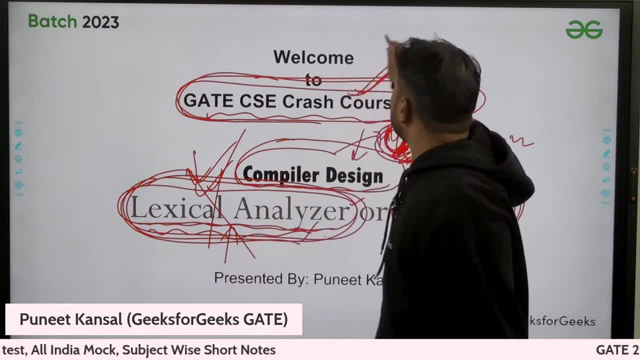 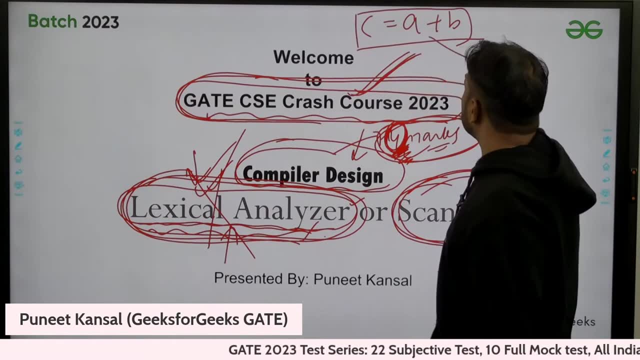 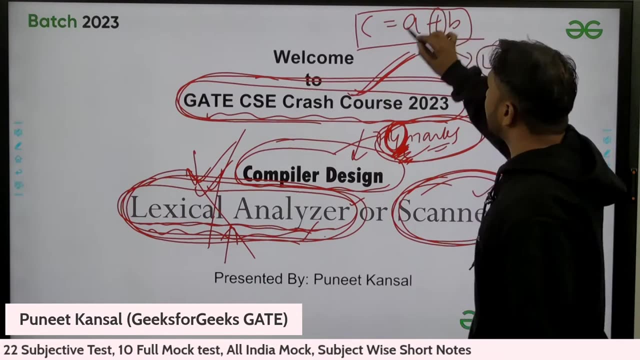 which are the operators. okay, if i write okay a plus b, i write okay c equal to a plus b. now, this is high level language. i give it to the lexical analyzer, i give it to the c, it to the lexical analyzer. so lexical analyzer will tell us: okay, i'm using plus operator, i'm. 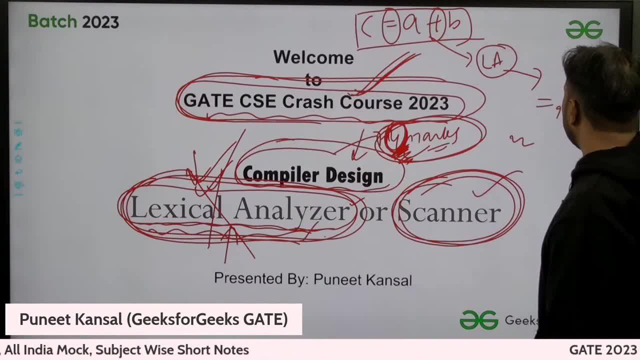 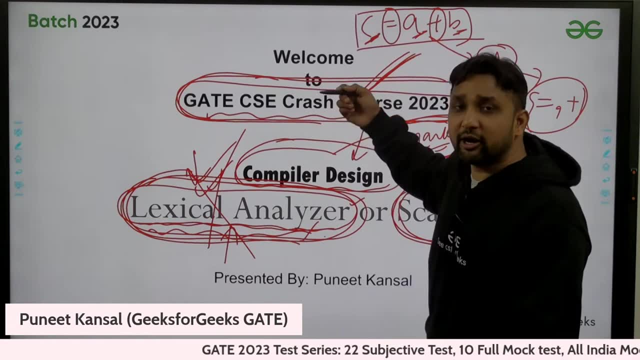 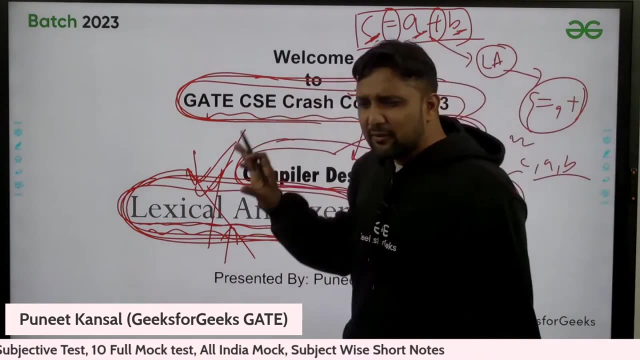 using equal to operator. these are the operators i'm using. this is telling me: okay, these are the operators you are using and these are the variables. or we can use another word: identifiers. these are the identifiers. c, a, b are the identifiers. so, simply, this is telling us: uh, this is dividing. 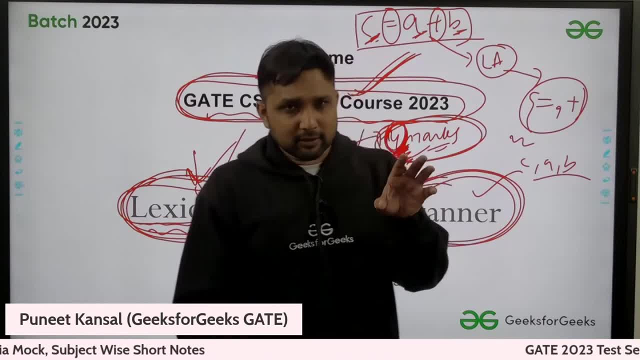 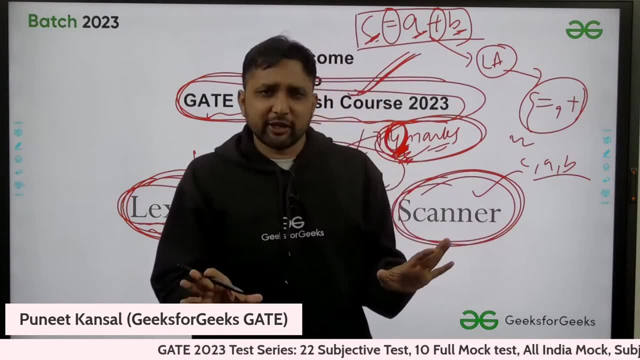 a big statement into small small parts actually. okay, a small small groups actually. so this is one group, this is another group. okay, so meanwhile, right now, i'm just telling you this is the first phase of the compiler. okay, we will cover from very basic, from the definition itself. so i have some 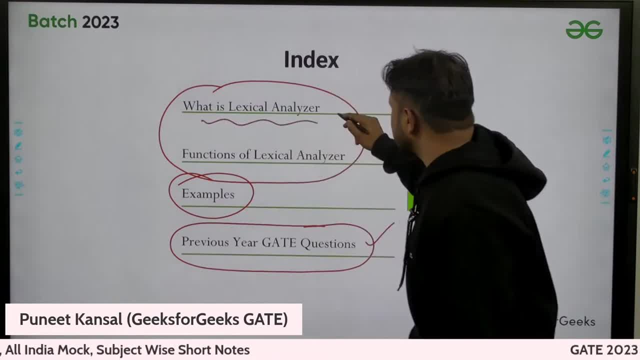 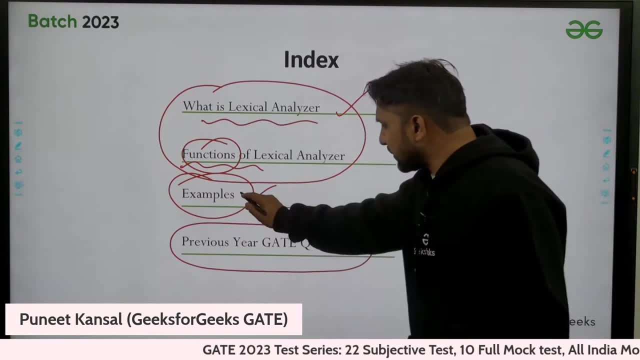 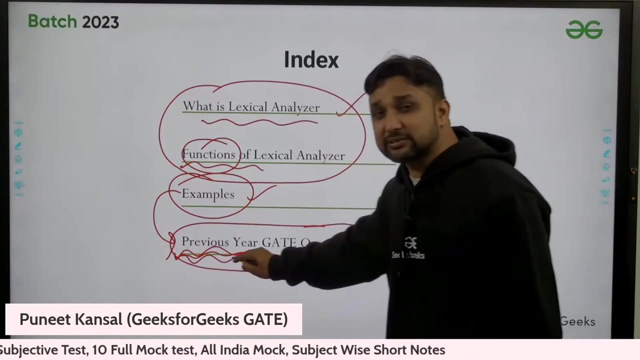 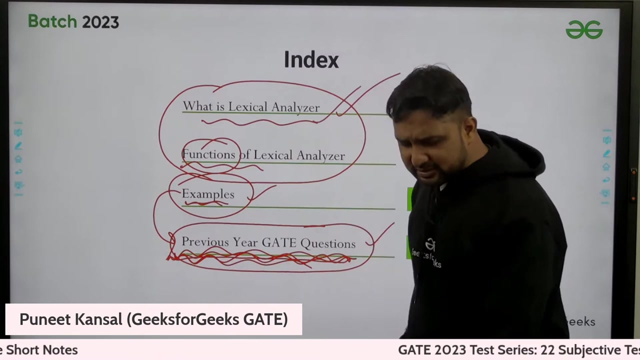 little uh. so we will cover what is lexical analyzer, functions of the lexical analyzer. we will cover various examples. these examples are designed in such a way that you can solve maximum gate questions, maximum pyqs you can solve that. these examples is covering all the concepts, actually, okay, okay. so let's start from very basic: what is, which is the 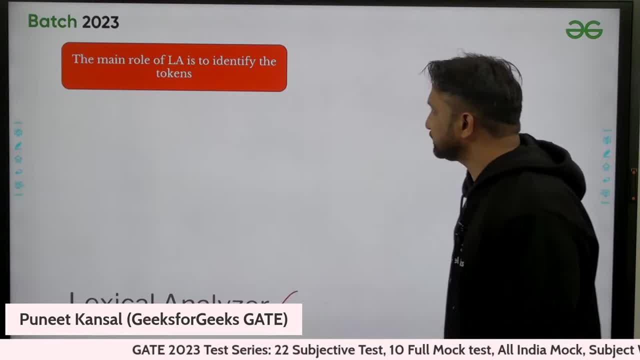 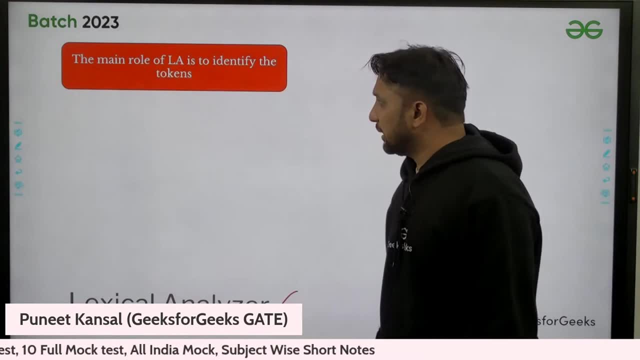 first questions comes in our mind: what is lexical analyzer? so lexical analyzer is one thing. is that is the first phase of the compiler, and what is the main role of that phase? the main role of lexical analyzer is to identify the tokens. and what is, what is these tokens? 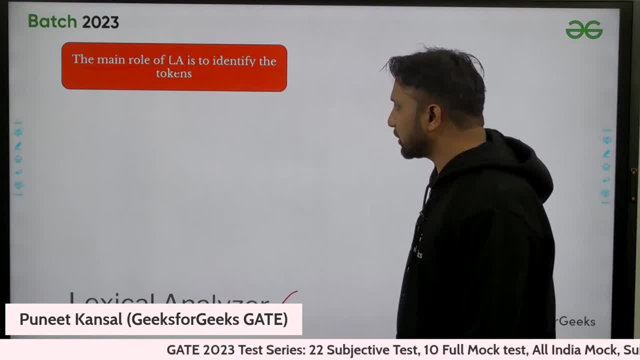 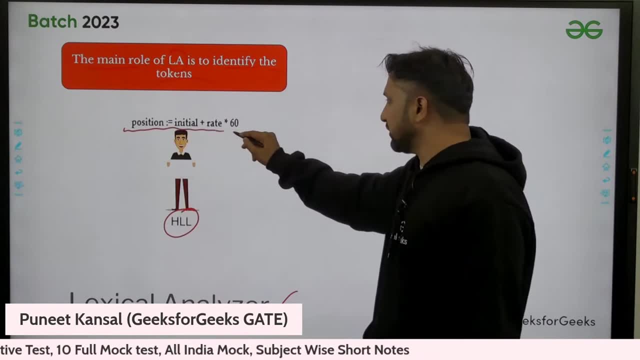 so that is identifying the tokens. what is this token? okay, let's try to understand it now. so let's suppose, uh, this is he is saying i'm. i'm high level language. this is our high level language. this is one statement written in high level language and uh. position equal to initial. 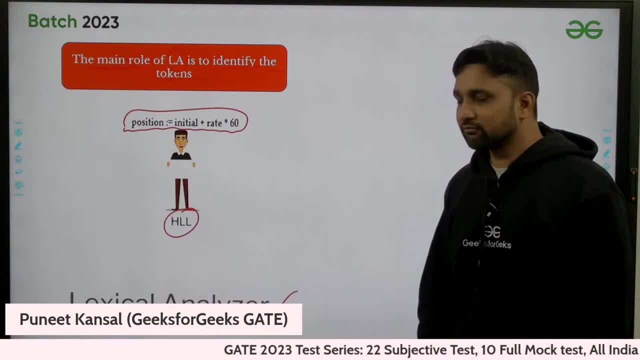 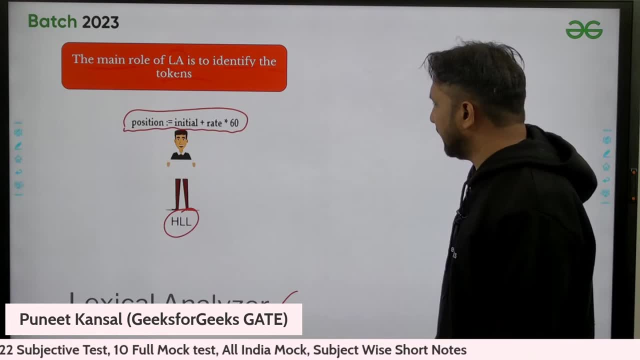 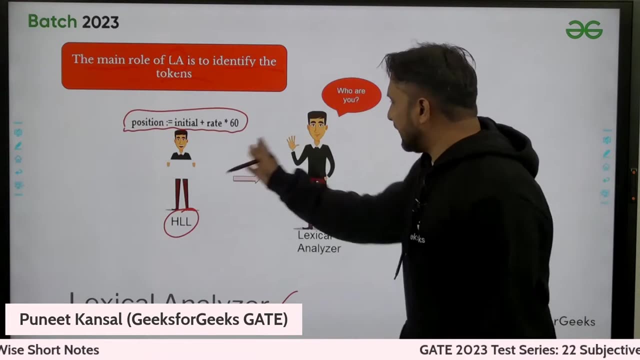 plus rate into 60.. okay, i have just taken the standard from the book actually, uh, so from woolman book actually i have taken this example, but just i try to animate it. so this is high level language and we provide the high level language to the lexical analyzer. 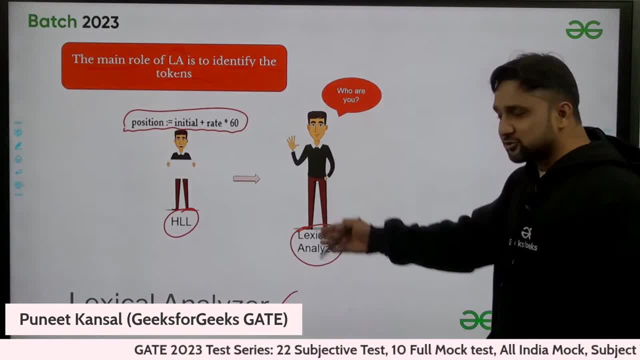 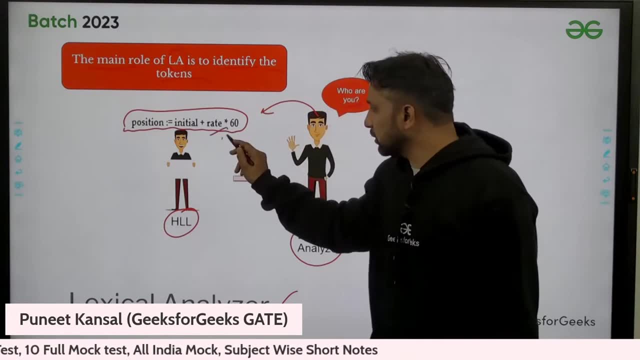 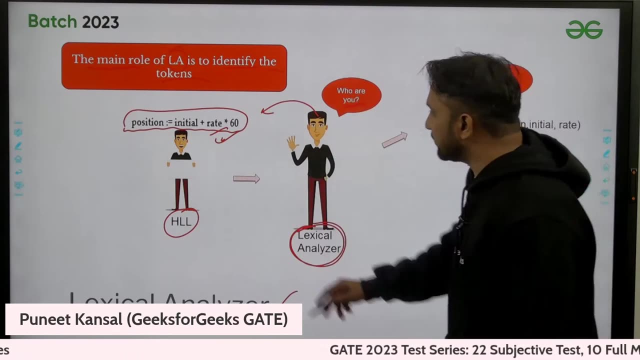 who is the first phase of the compiler. and this first phase of the compiler is asking to the high level language: who are you? he is asking him: who are you? who are you? so this lexical analyzer is asking to the high level language: who are you? okay, then he is telling that okay, out of these. 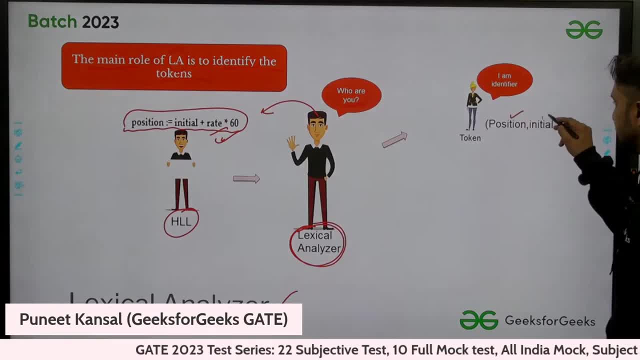 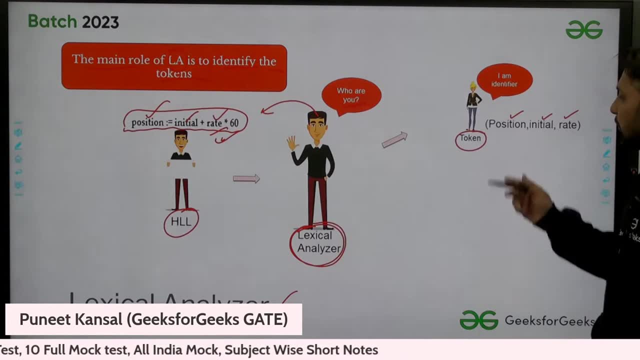 things. these are telling that, okay, uh, position initial and rate. this position initial and rate is telling that we are tokens. we are tokens. we are one type of token. which type of token identifier? we are identifier and we are tokens. tokens are one smallest unit. you can say, okay, one. 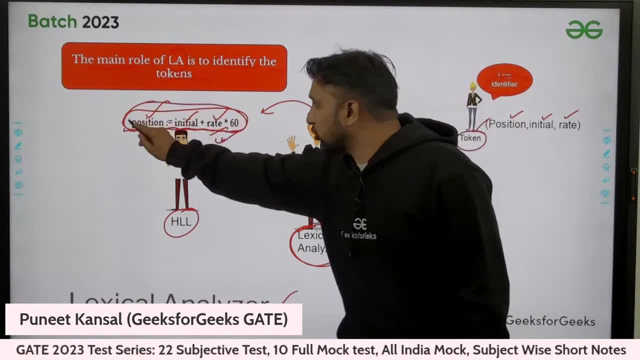 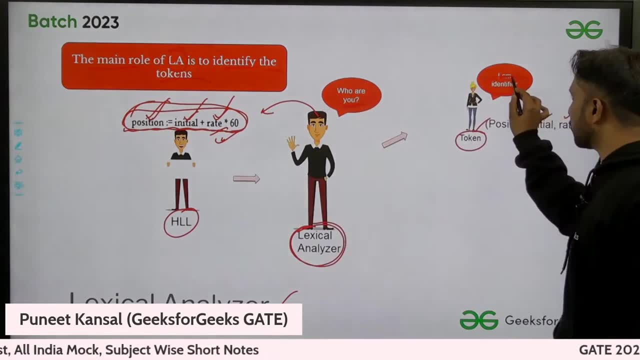 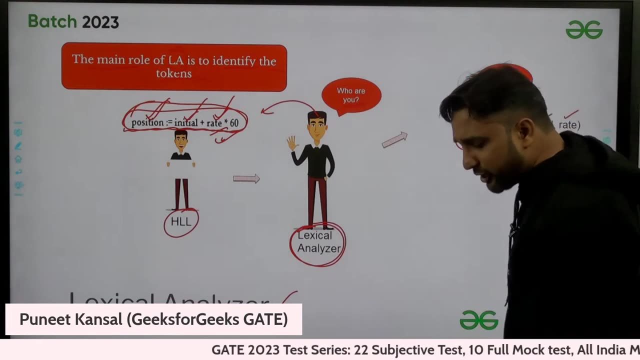 of the smallest unit inside the this statement. okay, so position, initial and rate are some similar type. these are, these are variables. actually, we also call them the identifiers, we call them identifier and uh, these are tokens. actually, these are tokens, tokens. so they are saying that we are tokens. similarly, other tokens also come. 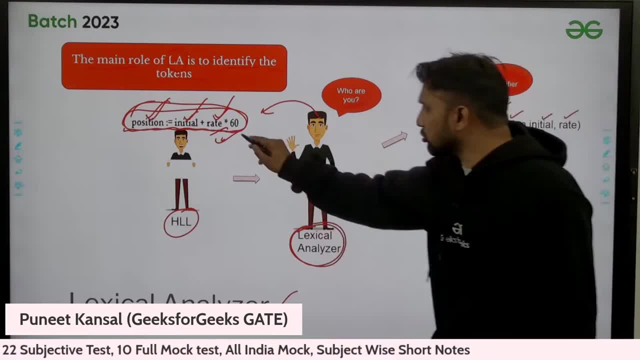 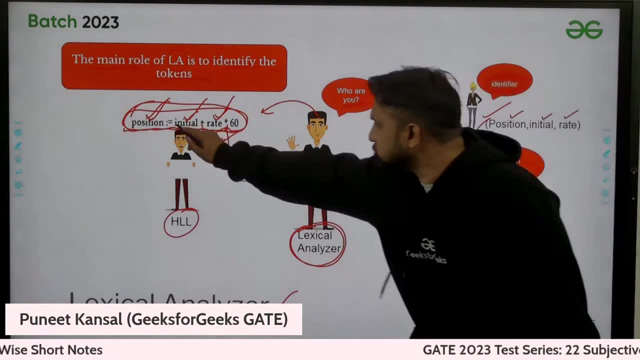 plus and multiply also come. they said. they said we are also token, we are also token, but we are. we are operator type of token, we are operator, these are operators. okay, equal to is also there. i do not mention here. let me mention here. so, equal to plus, multiply or equal to, these are. 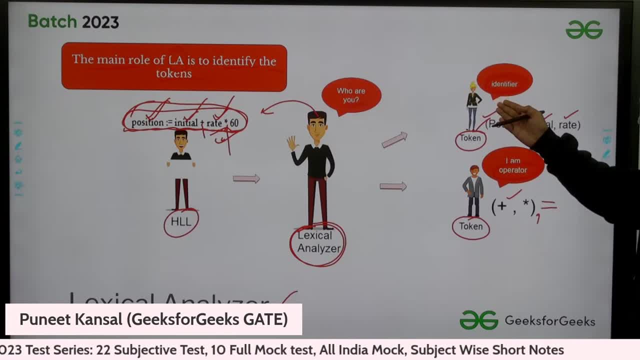 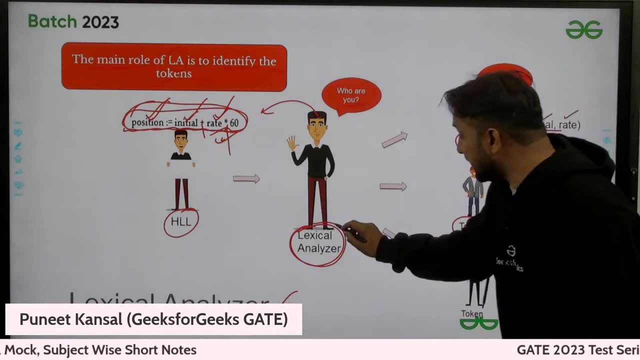 operators: type of token: okay, these are different type of token, these are different type of type of token, but these are also tokens. these are also tokens. okay, another, uh, another type of token which lexical analyzer find out is the constant 60 says: i am also a token, but i am a 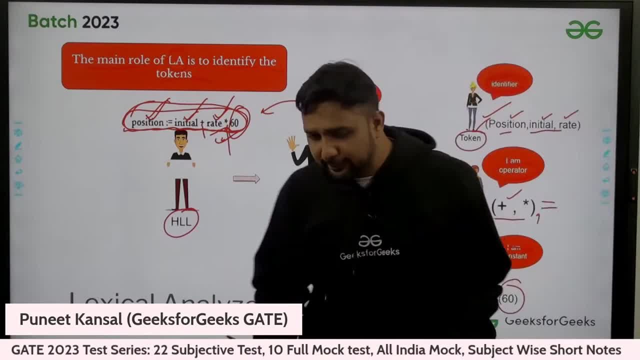 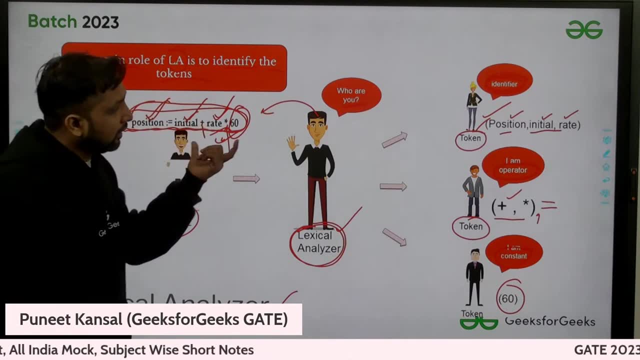 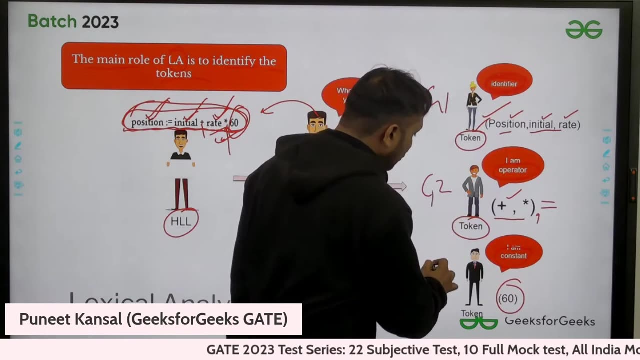 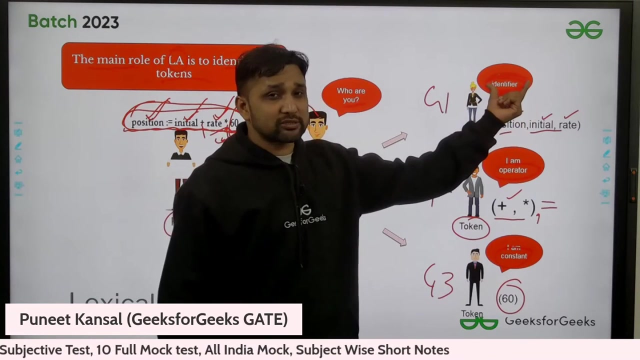 constant token. okay, so you can here see that what lexical analyzer is doing is that is, taking a high level language, high level statement, dividing it into some groups: group 1, group 2, group 3. this is one type of token in group one, which is, which are known as identifier. another type of tokens is the operator plus. 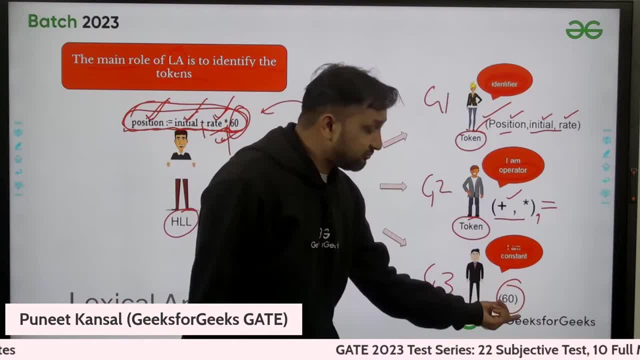 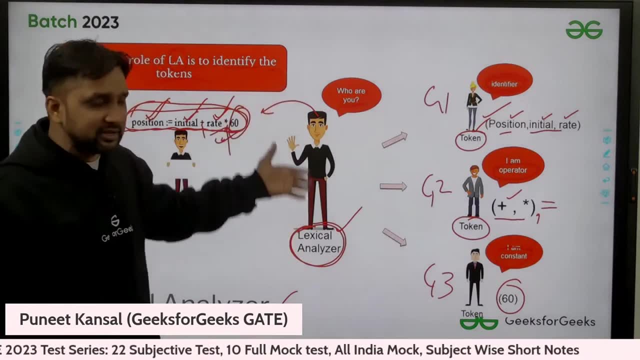 multiply equal to. another type of token is a 60, which is a constant type of token. so what this like? if somebody asks you what is lexical analyzer, it is the first phase of the compiler. he is the first phase of the compiler which is taking high level. 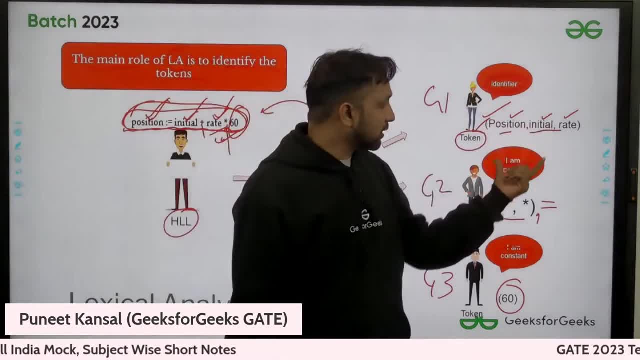 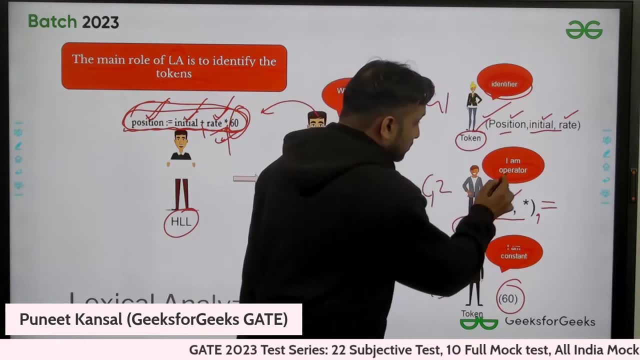 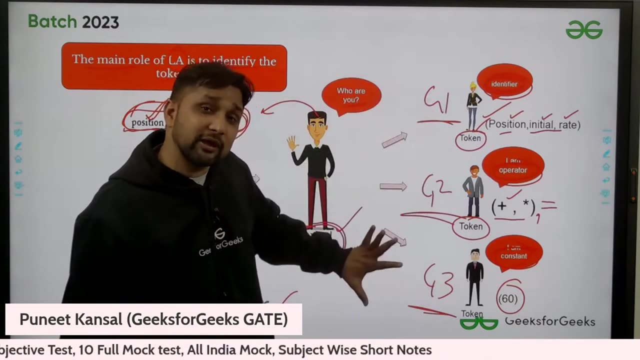 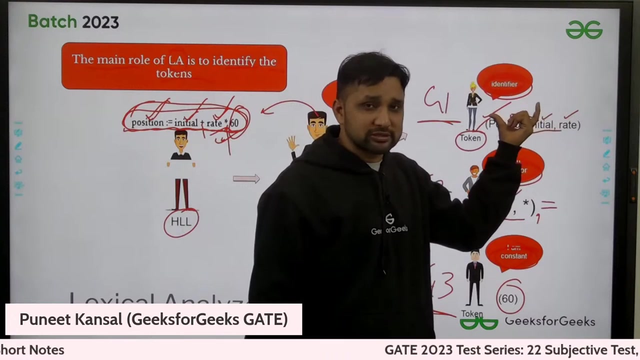 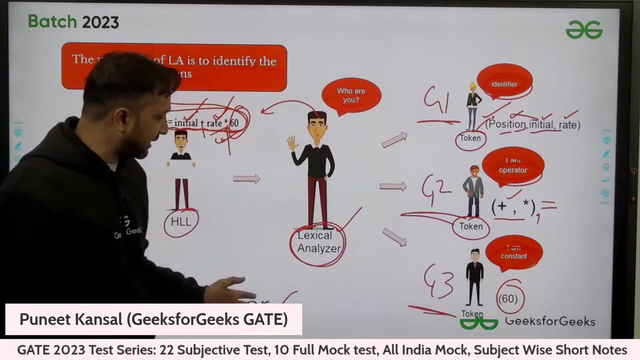 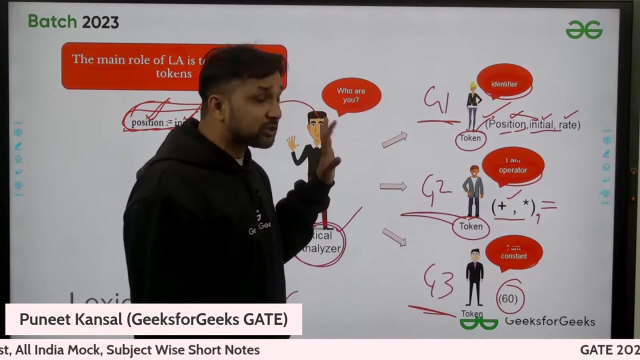 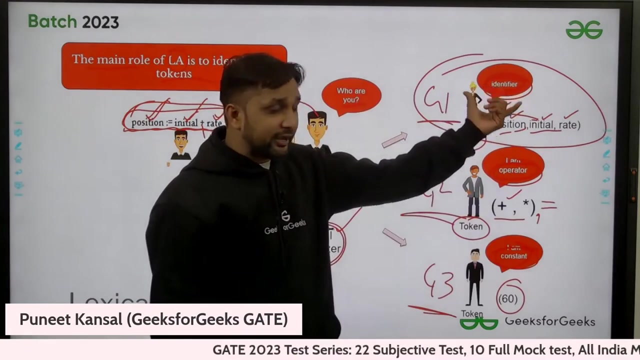 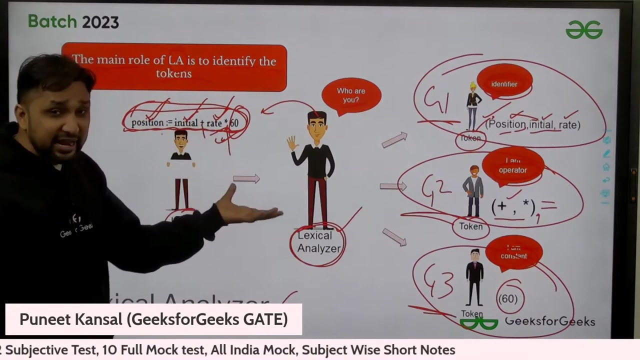 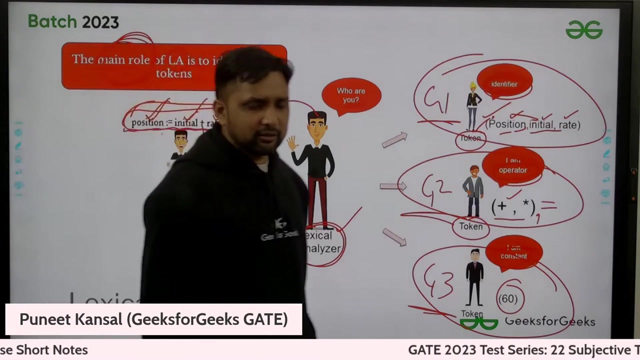 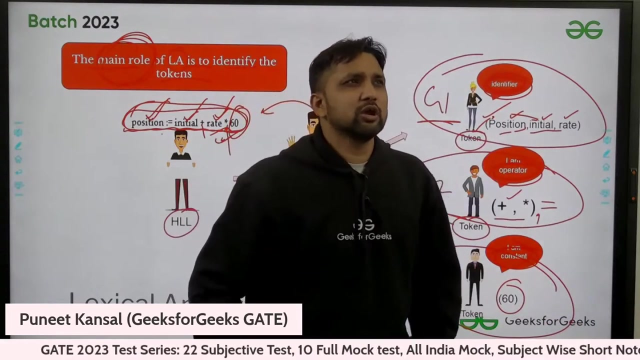 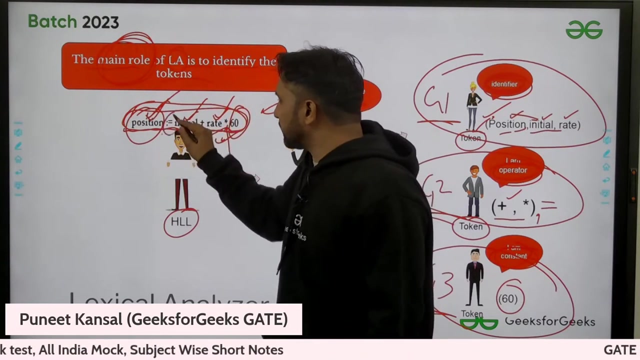 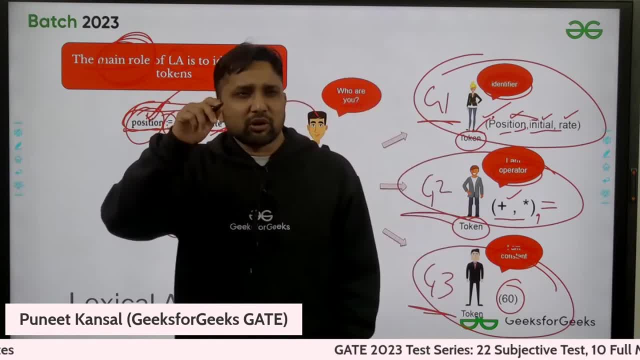 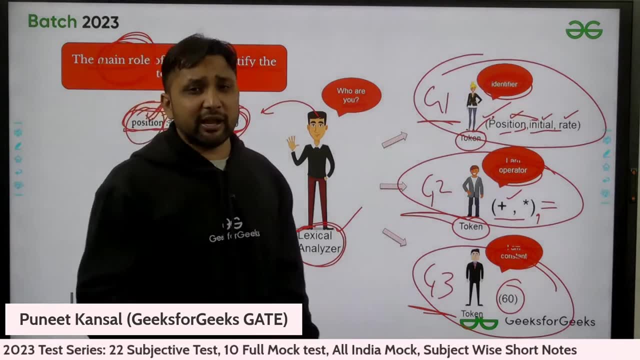 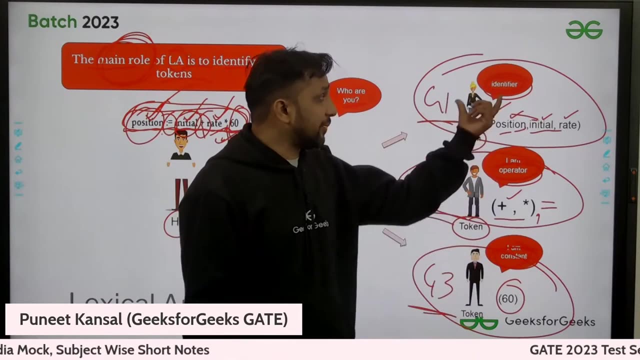 an another thing. plus is another thing. so these are the smallest unit we can say inside the high level languages which are identified by the lexical analyzer and we simply give them a name. and what is that name? that name is token. that name is token and that group also similar type of top. 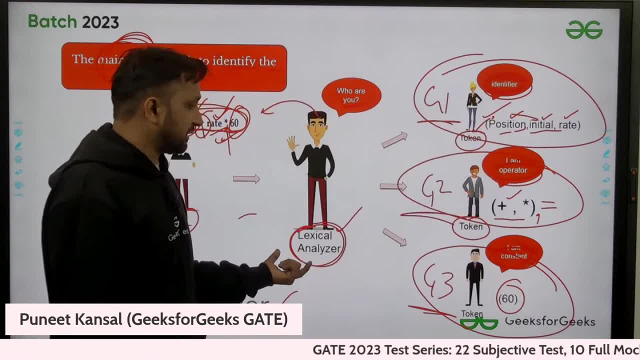 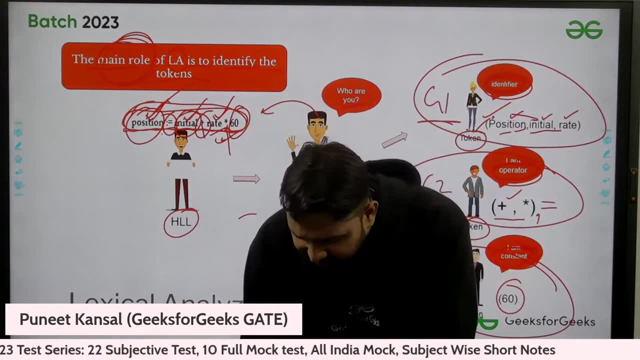 tokens, that is grouped also by the lexical analyzer. that's it. this is lexical analyzer. this is lexical analyzer. if any doubt, please ask me, please write in the chat if you have any doubt. we will finish this topic starting from very basics and we will cover all the previous. 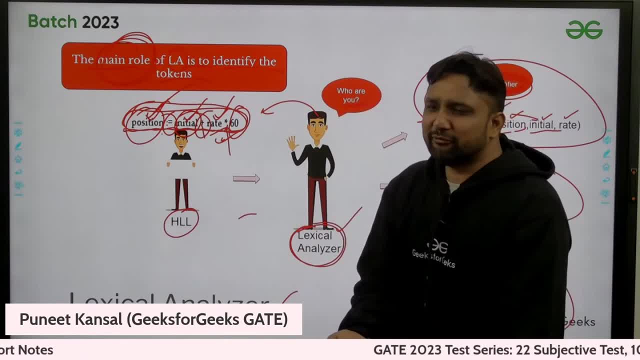 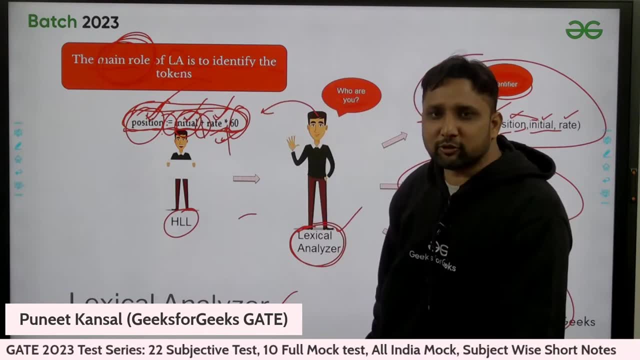 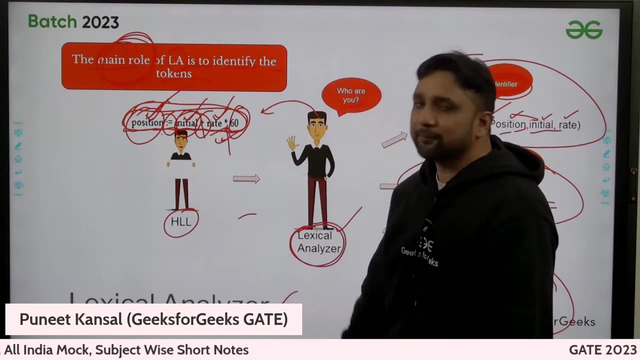 gate questions and you people will solve yourself, because nothing will be left. i will cover everything. then they cannot generate the question out of the concept. they cannot generate the question out of the concept. they need to generate from those concepts only. so i i don't think if the question will come from this topic. 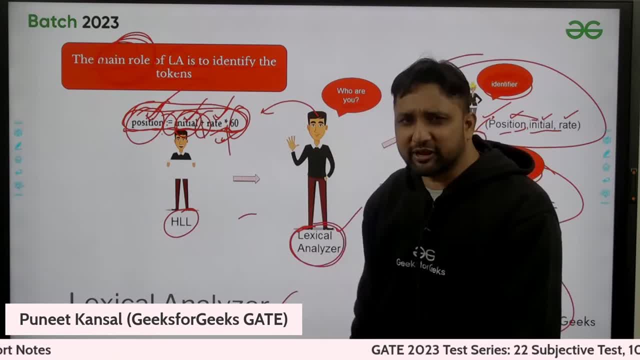 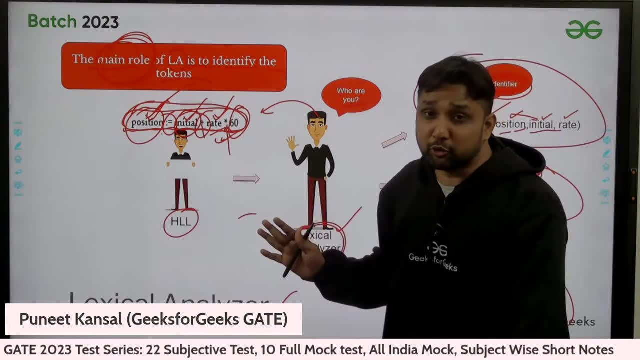 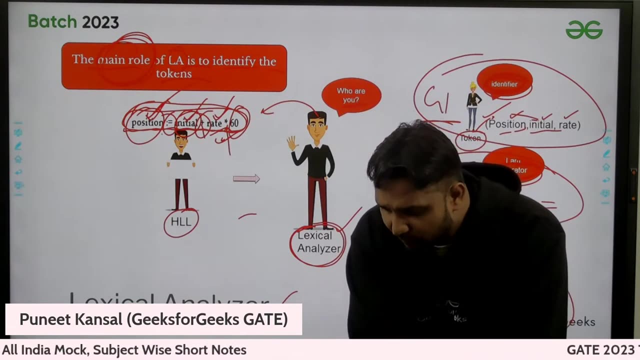 i'm making you sure that you will able to crack that. you will find that question very easy, believe me. but ask the question. if you have any doubt, please write in the chat that you need to do. please write in the chat if you have any doubt, please. okay, so i'm moving on. uh, if you have any doubt, you can. you can write in the chat. 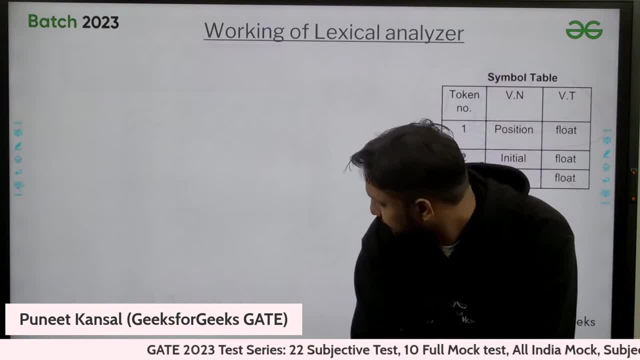 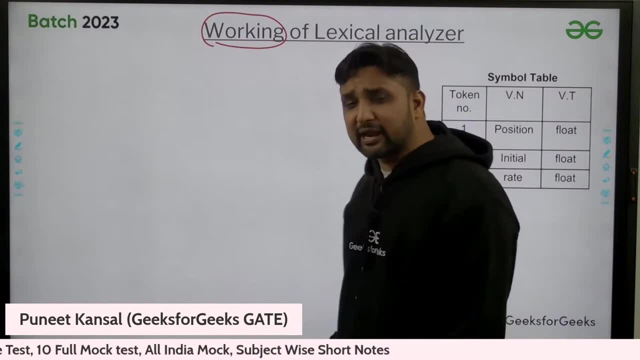 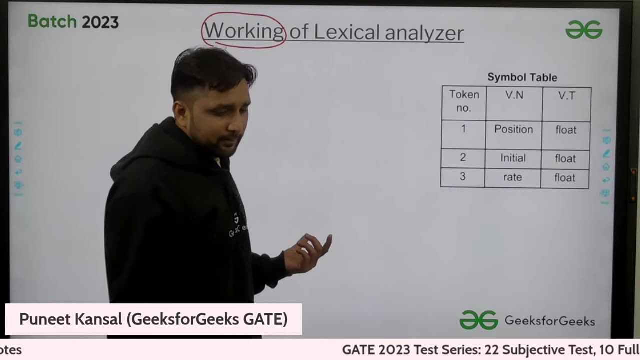 so still, i'm moving on. okay, so let's see the working, how that is finding the tokens. one thing is clear: lexicon analyzer is finding the tokens. that is the main role of lexical analyzer. but how that is finding the tokens, okay that, let's identify that thing. 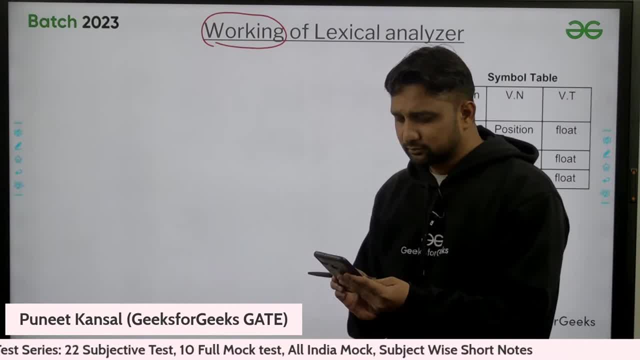 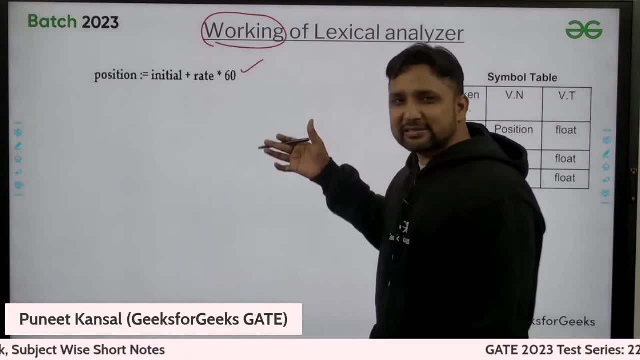 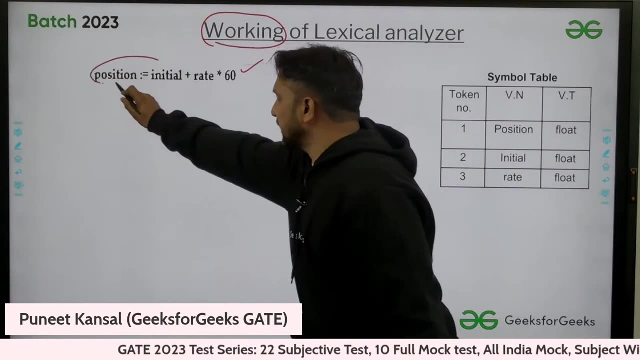 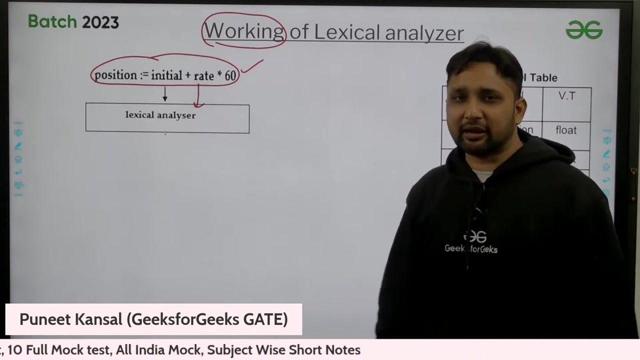 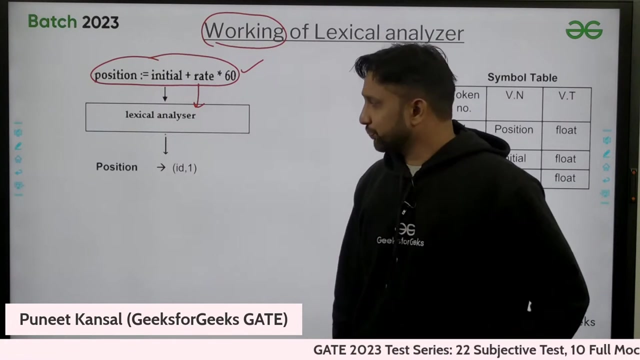 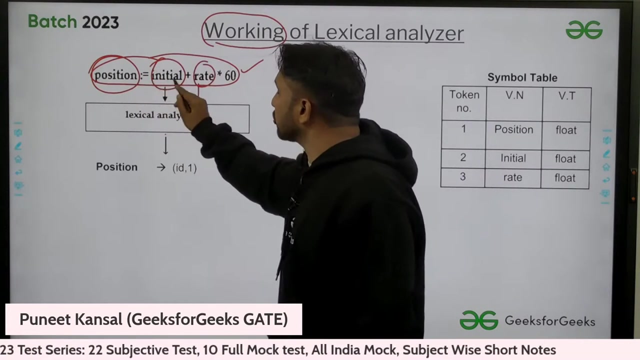 okay, thanks for replying. okay, clear here. okay, so this is a high level language. we fed it to the first phase of the compiler lexical analyzer. okay, this lexicon analyzer. what that will do is now that will identify these, all these different type of tokens here. maybe these are identifiable type of token, these are: 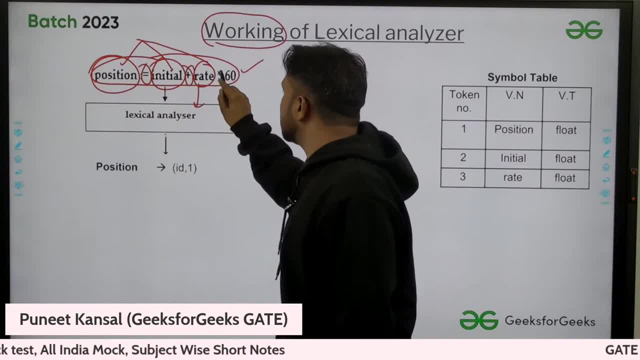 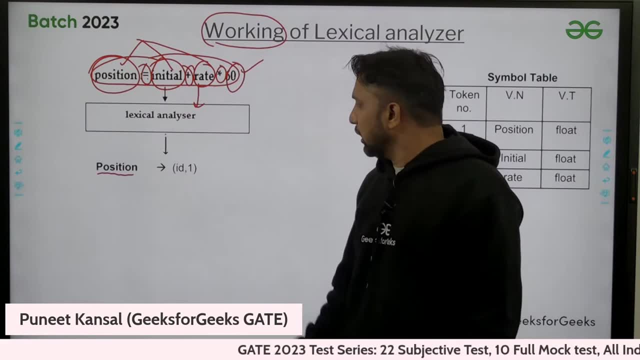 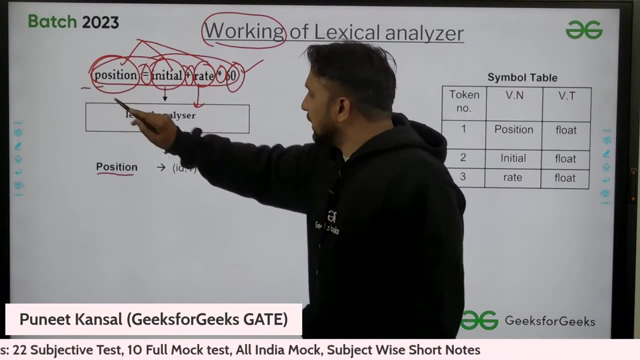 operators: type of token plus equal to one star: this is questionable. type of token: okay. R type of token. so one token he find out is the position: okay. so he is saying that this is an identifier. this is giving us two information. after looking at this, lexicon analyzer will start from: 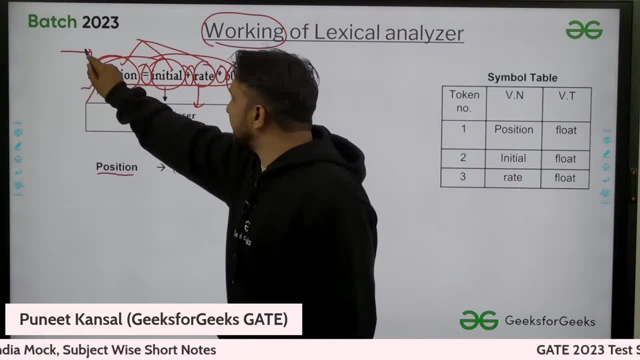 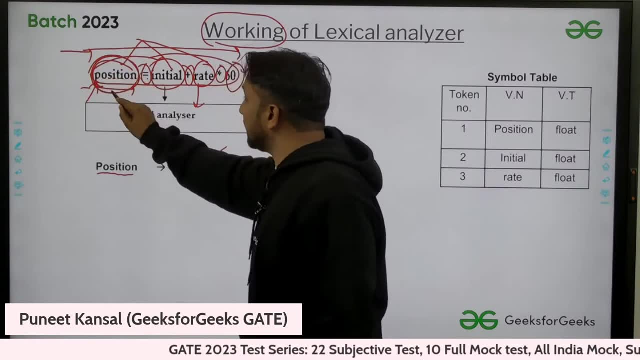 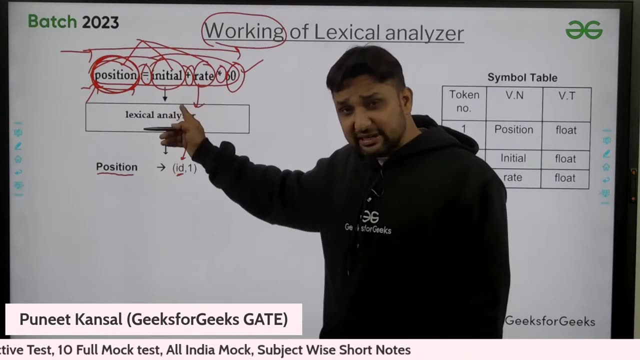 the very first character actually, and that will keep moving on. okay, so from very first vector that will start, and then we'll identify that. okay, this is a, this is a variable, this is an identifier. so he will mention that this is an identifier and, after mentioning that thing, lexicon analyzer. 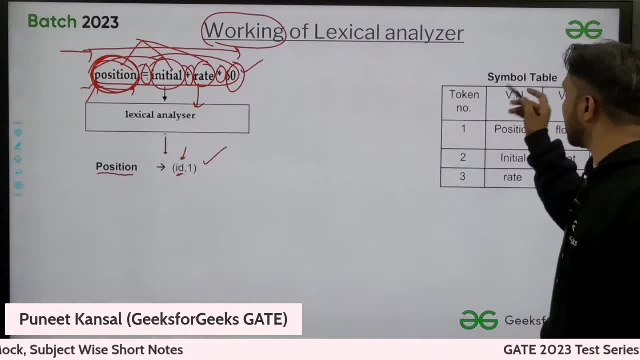 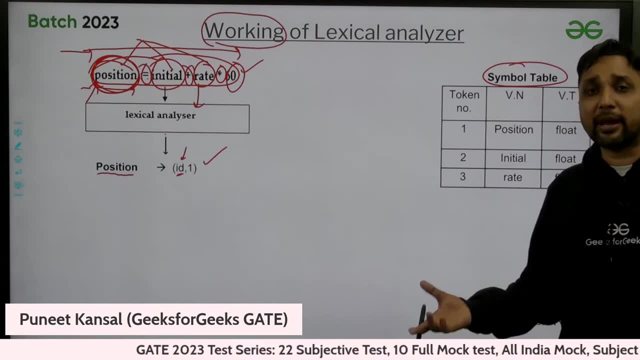 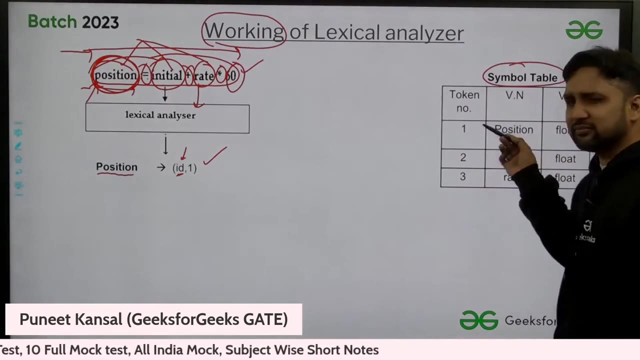 will store this identifier into the symbol table, into the symbol table. so what is symbol table? symbol table is a data structure used by the compiler. compiler use this data structure to store what? to store identifiers, to store the identifiers. so you have. you have, maybe you have using the variables. identifier nothing, variables you are, so you are using in your 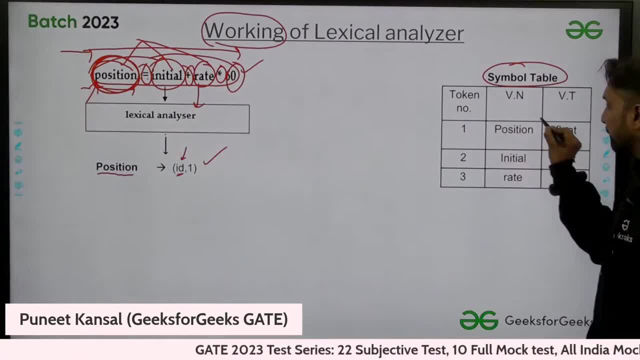 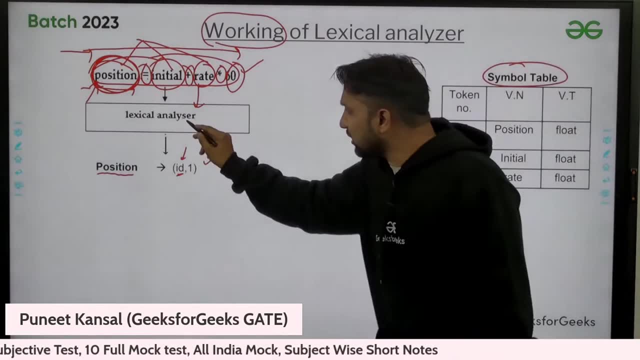 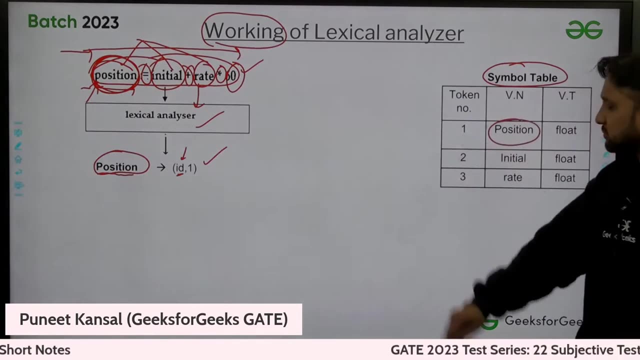 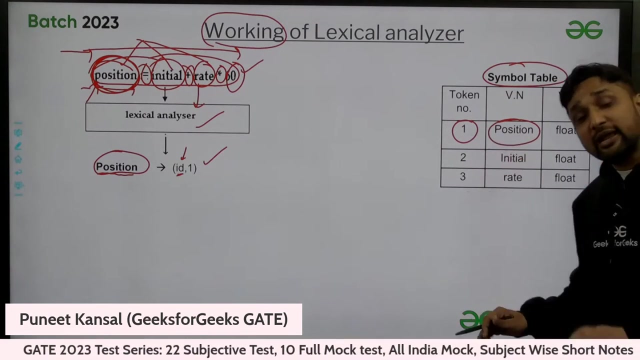 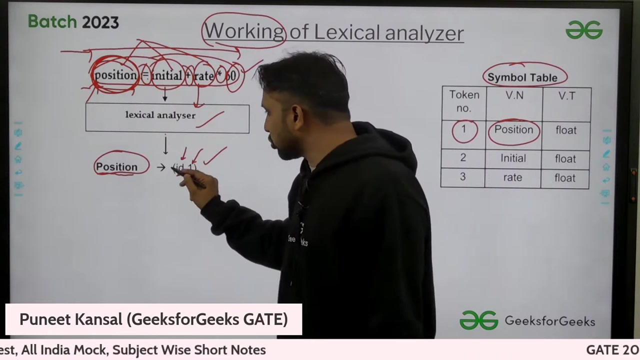 in your program. so these variables are stored where in the? in the symbol table in this data section. this data structure is used by the compiler. so, yeah, that can identify later on. okay, so it's not the first time is i find out this token and, uh, i store it in the table and its number is one now. 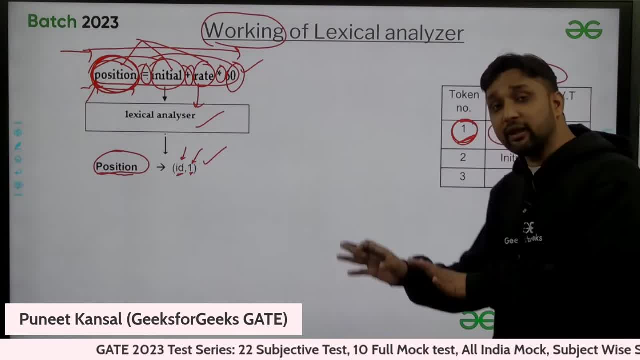 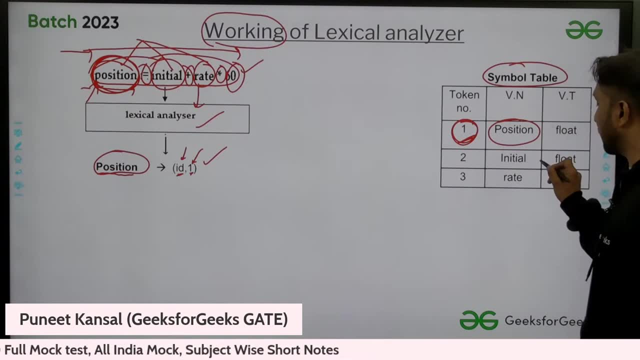 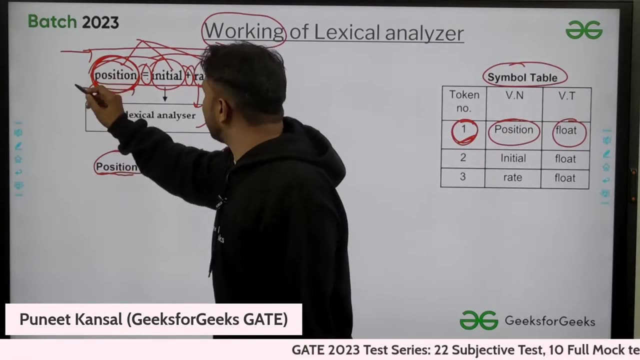 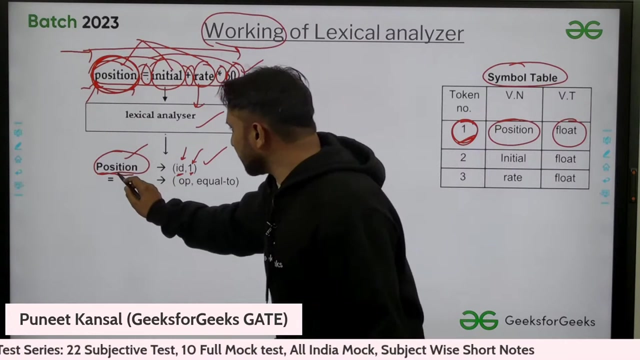 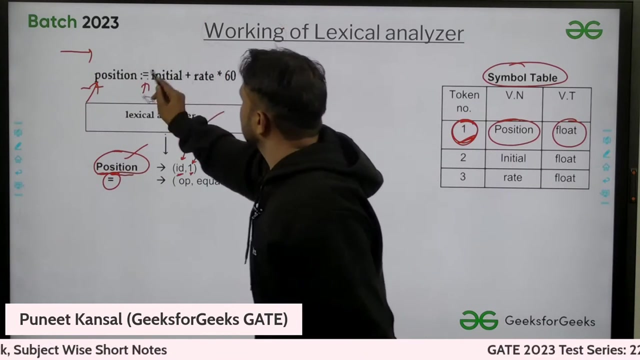 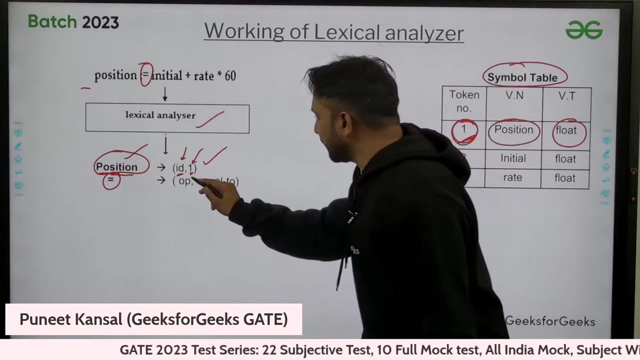 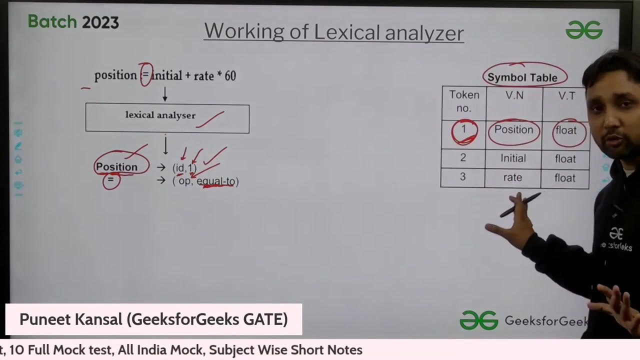 okay, so that later, if you will use this variable in the program, then the compiler can identify, can find out this variable here in this, uh, in this symbol table. okay, so, maybe we have assigned it earlier on, okay, so, okay, okay, okay, uh, is is, is it is. 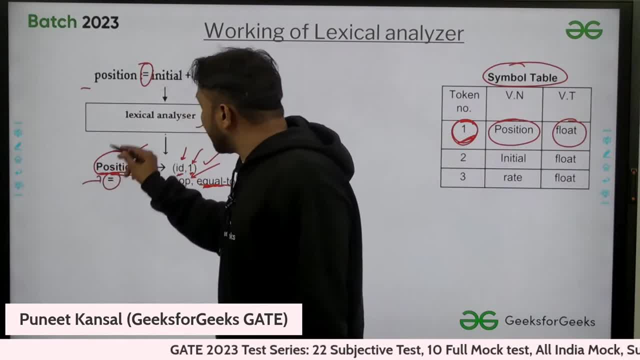 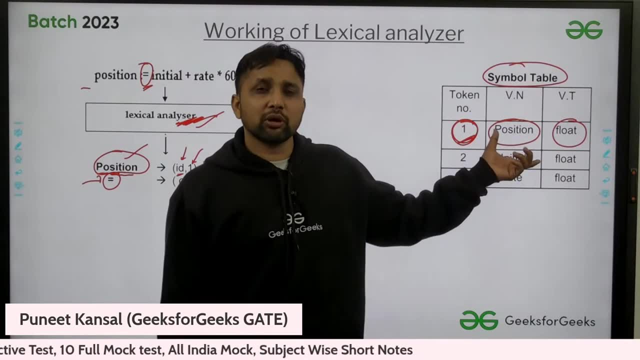 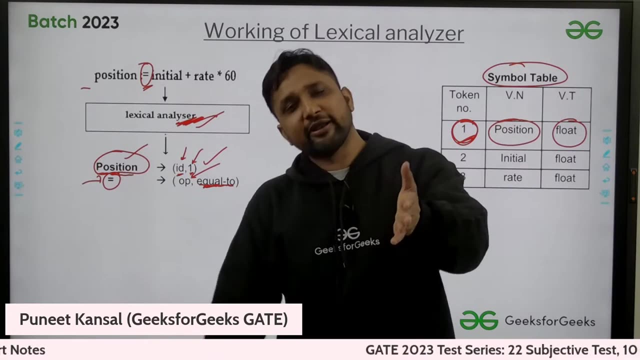 is, The operators that are stored in the symbol table are not stored in the lexical analyzer. Why are they not stored in the symbol table? Because the compiler already knows this. When you designed the compiler, the compiler has already defined all the operators. The compiler is also a program. 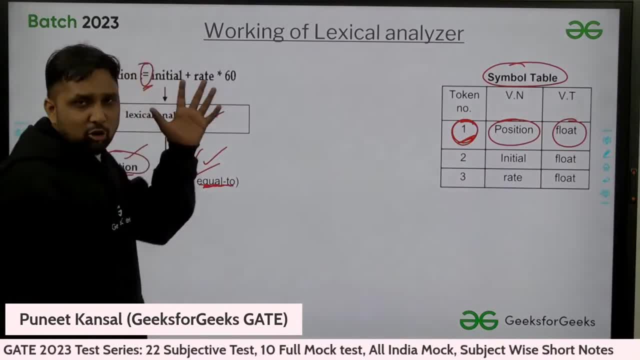 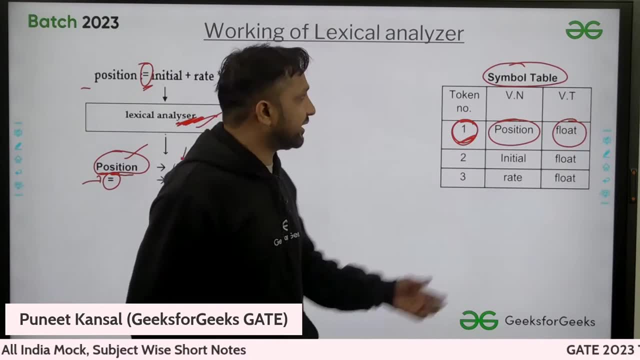 In that program. it has already defined all the operators. Have you identified the variables? No, we haven't identified them. For their information, we are using the data structure in the symbol table And we are storing it in it. Who is storing it? I am not doing it. 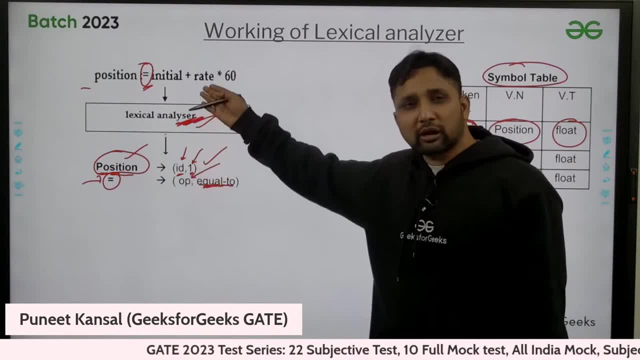 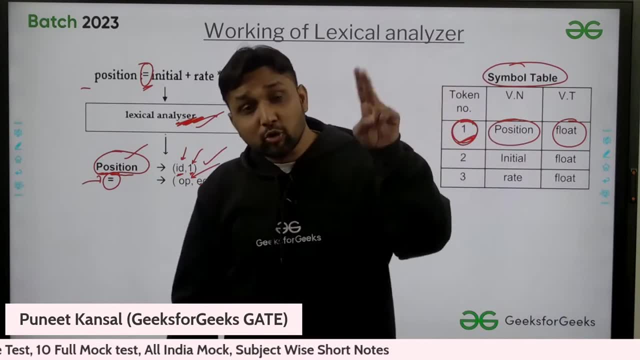 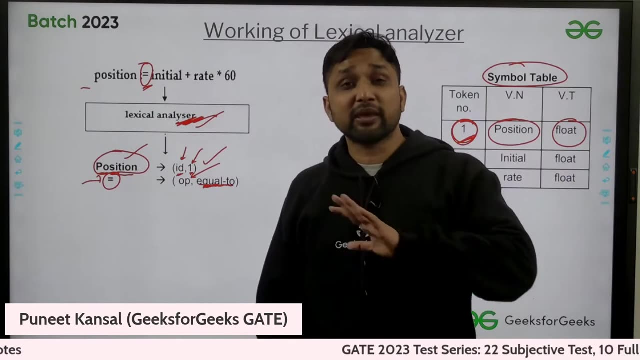 This lexical analyzer is doing it. If you ask who is storing this symbol in the symbol table, Who is storing it? The lexical analyzer is storing it. But there is one more question in the exam: Does the lexical analyzer only access the symbol table? No, all the faces can access this symbol table. 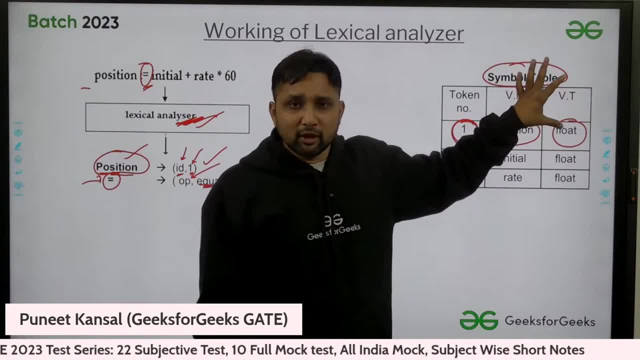 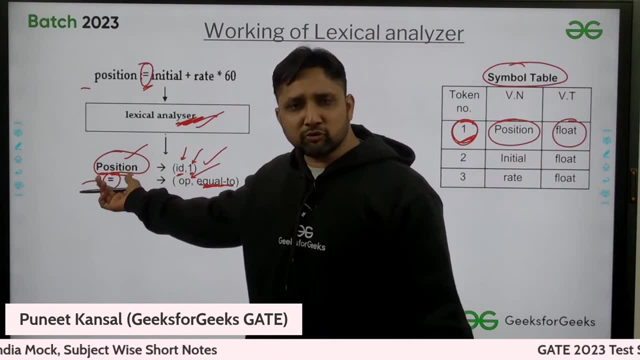 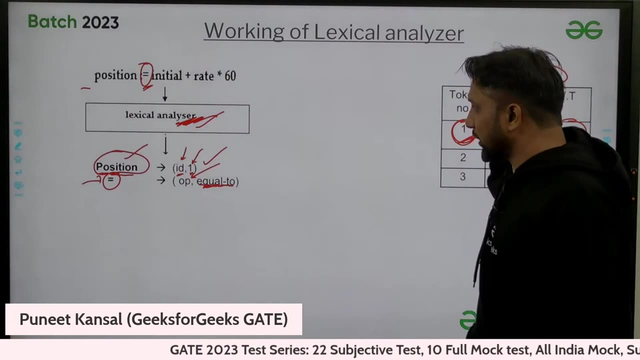 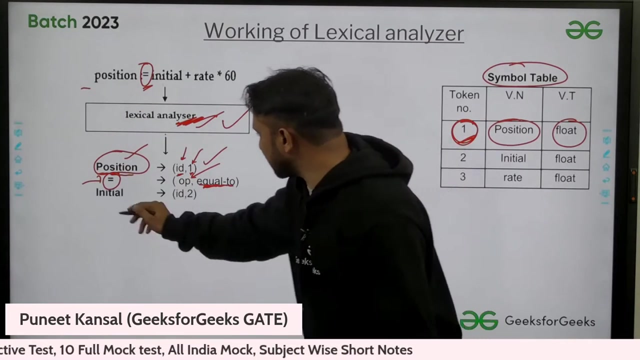 They can modify this Somehow. modify it So this symbol table can be accessed by all the faces, Because all these variables will have to be used. All the six faces will use this data structure. This is not the only phase This token is finding out, So let it do. 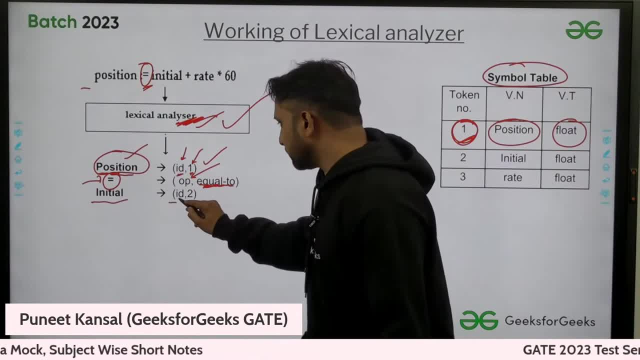 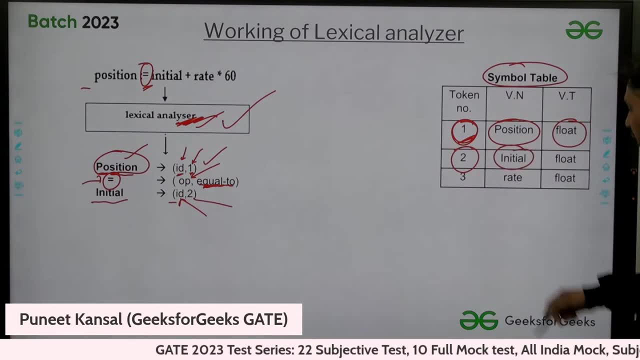 It has found out the next token initial. That is a variable. Again, it is saying that it is an identifier And I have given a number to it too. I store it into the symbol table. Now it has written. The lexical analyzer has put it. It was not there before. 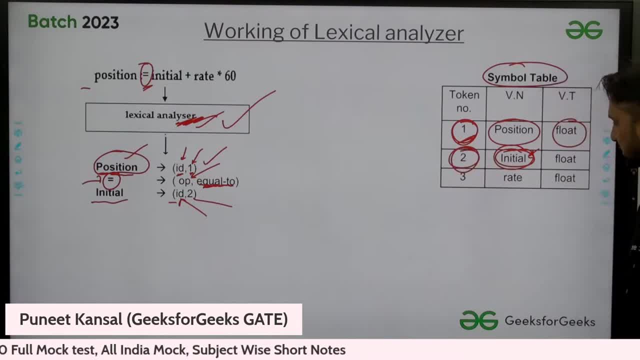 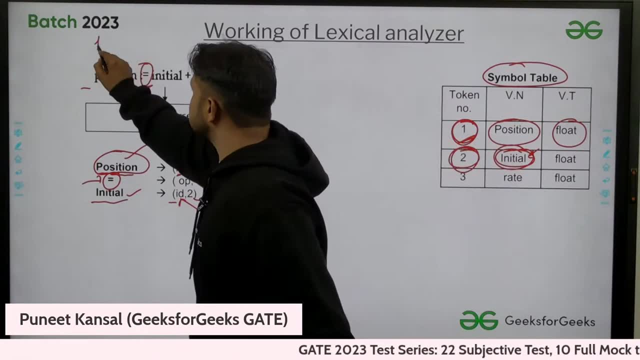 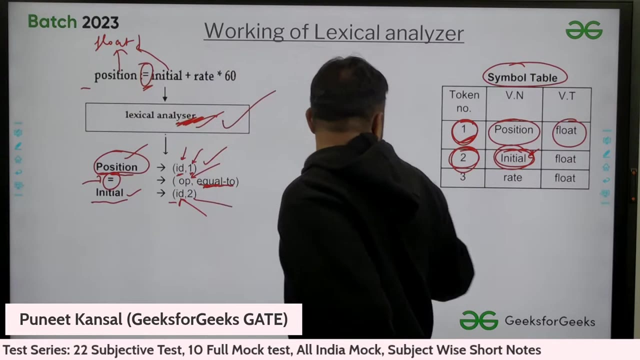 The lexical analyzer has stored it. It has assigned a token number And its type. What type of variable is this Float type? Okay, So that must be mentioned earlier. actually, This is float. Position is float. This is also float. This is also float. Actually, I think rate is also float. 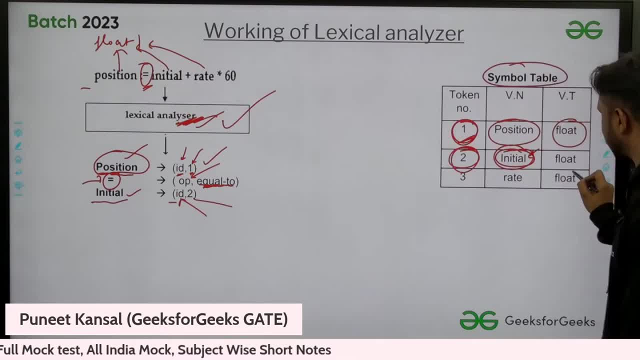 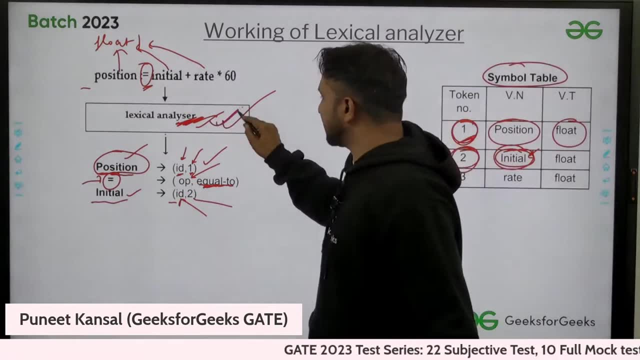 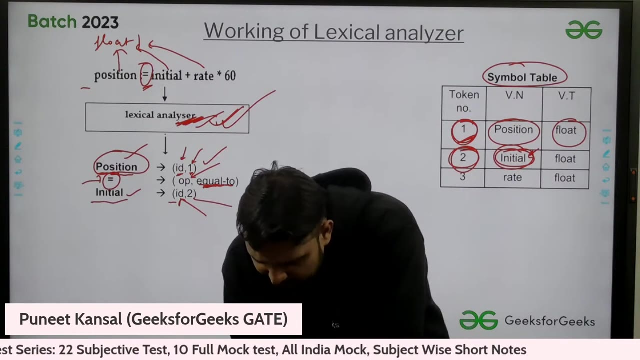 So this must be mentioned. Then only that will mention that. Okay, this is float type. If this is type int, Then that will type int here. Okay, All this is done by the lexical analyzer, Okay, Okay, Let me speak in English now, If you are asking me to deliver in English. 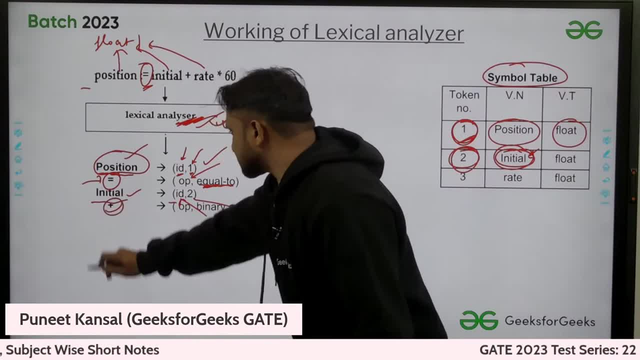 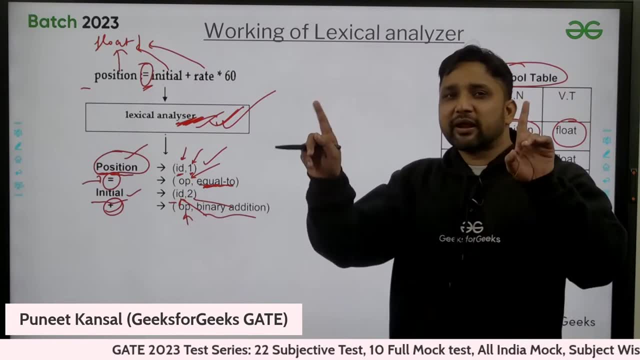 It's okay. So next one is the plus. Plus is another operator. That is a operator That is a binary operator, Binary addition. Two numbers: Two numbers are required for addition, Like 5 plus 6. Two operands are required. Okay, I cannot write 5 plus. This don't have any meaning. 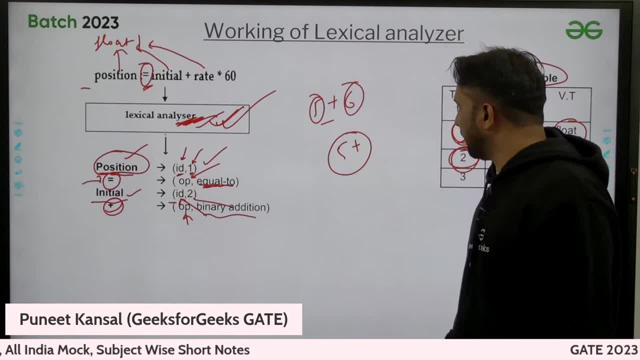 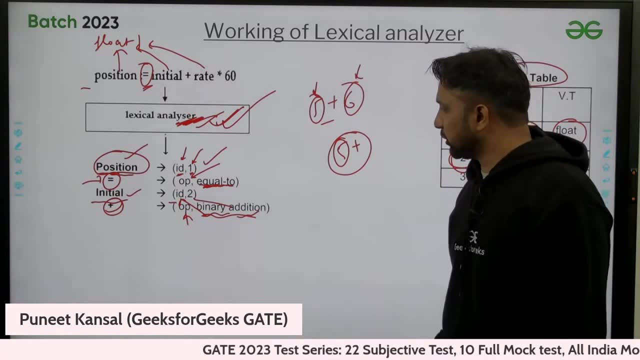 Okay, I need to write two operands, So that's why this is binary, Binary operator. actually. Okay, This is operator And binary operator. We do not need to store it into the symbol table. Very easy. Next one is the identifier. We store it into the symbol table. Give it a token number. 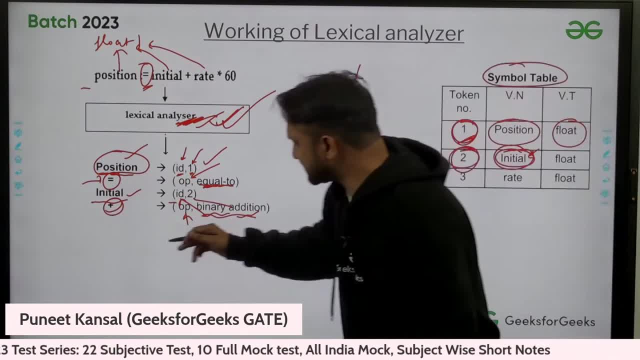 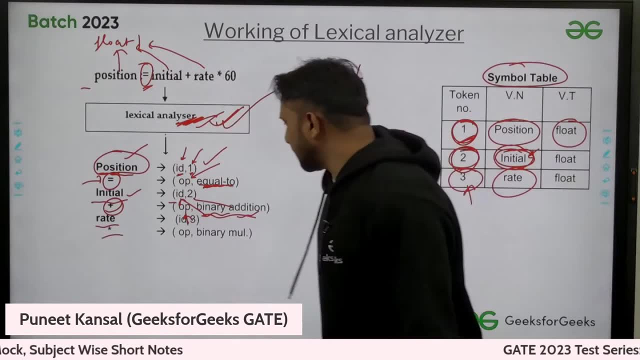 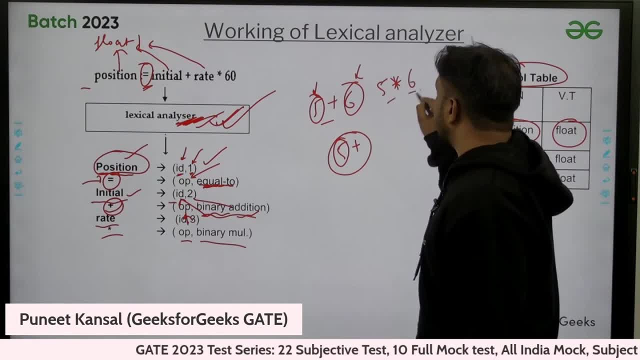 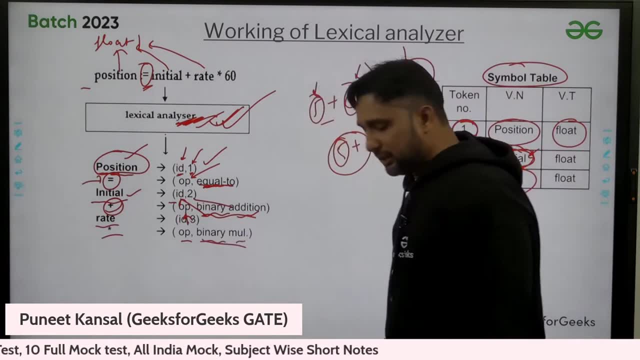 We need two, Two operands to multiply. I cannot say like this: This doesn't have any meaning, This need two operands, So that's why this is binary Operator, Binary multiplier. Another one is: 60 is a constant, Which is a integer constant They have mentioned. Because this is not like this. 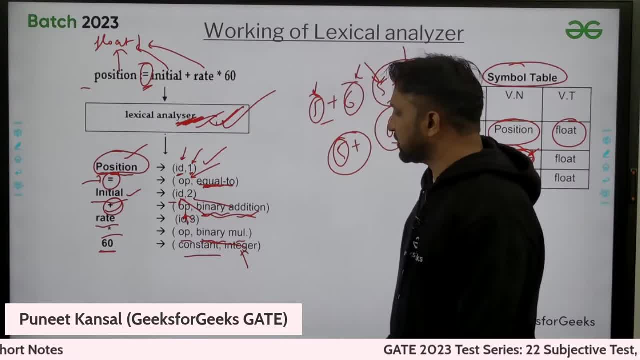 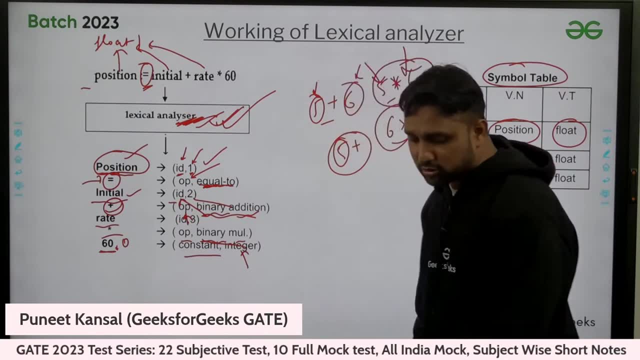 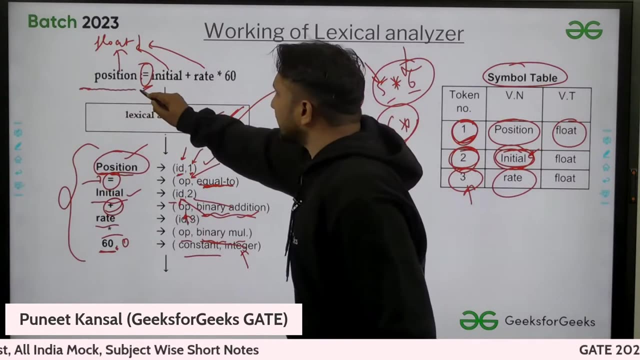 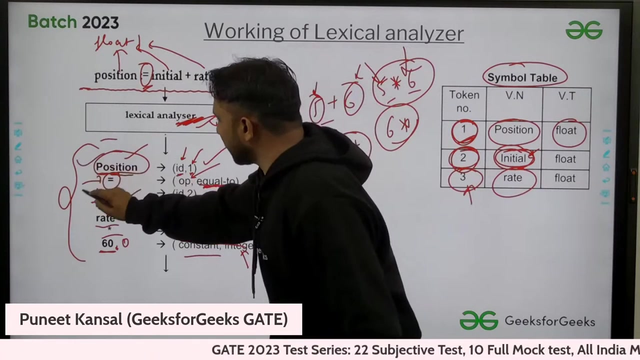 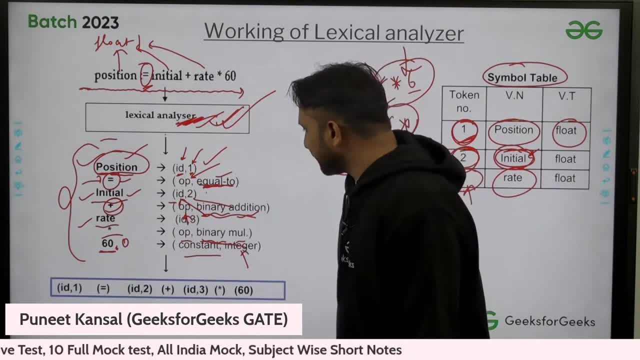 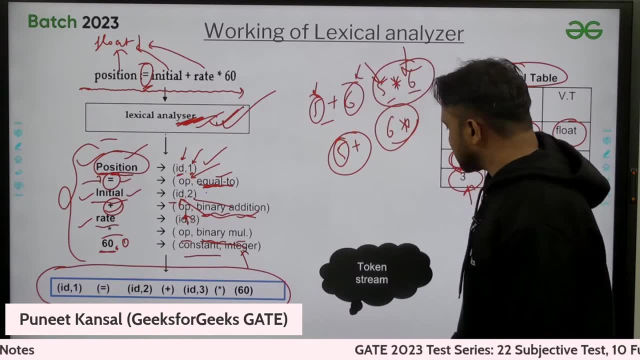 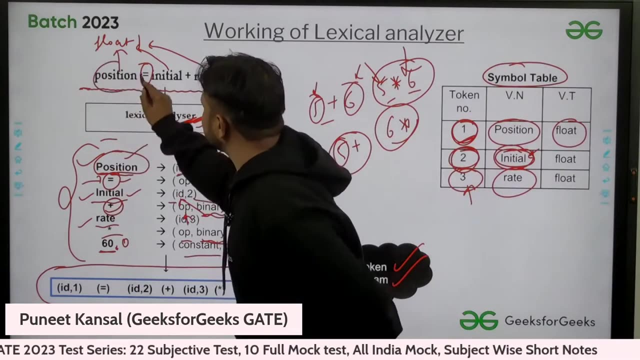 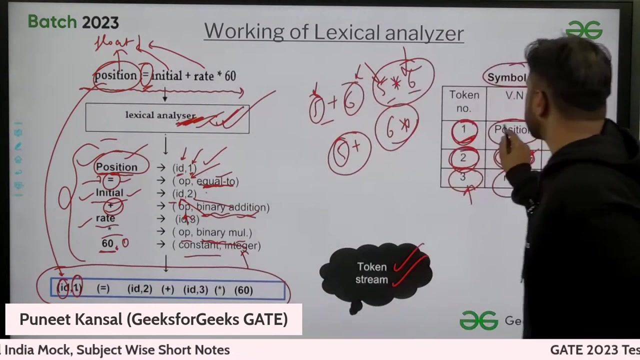 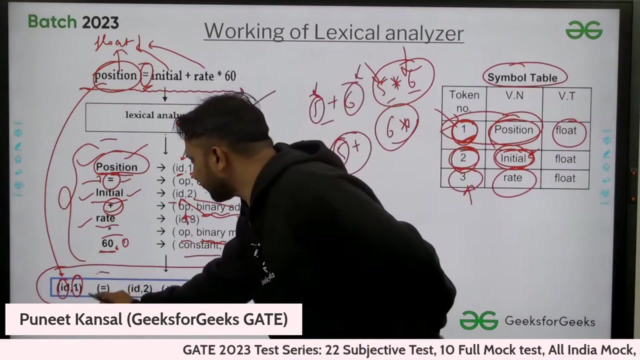 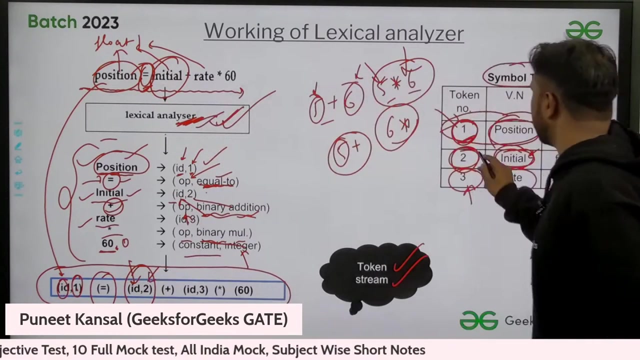 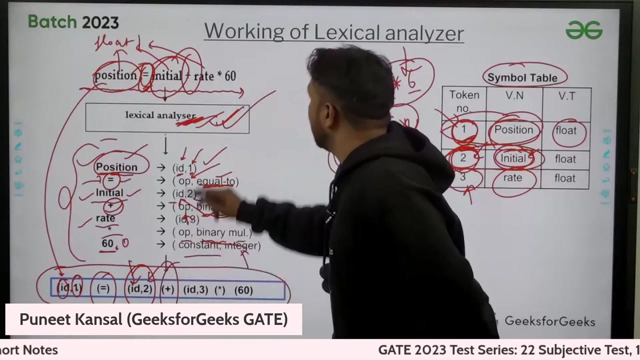 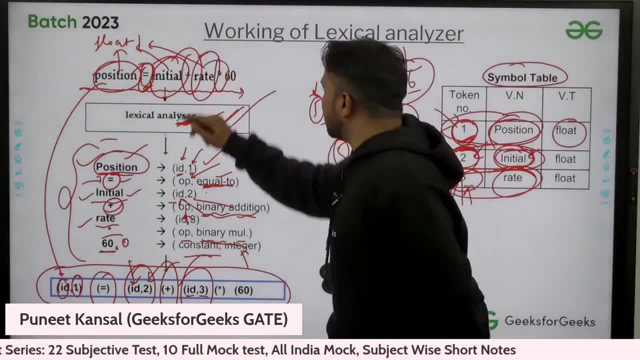 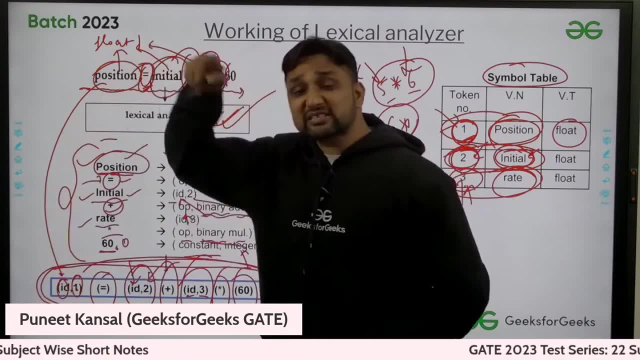 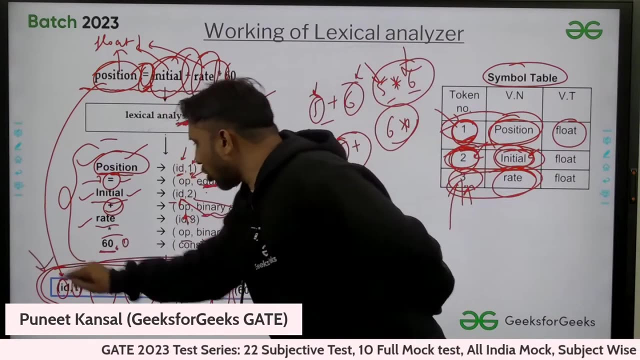 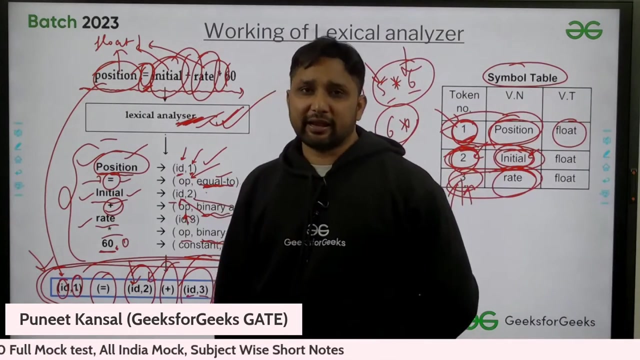 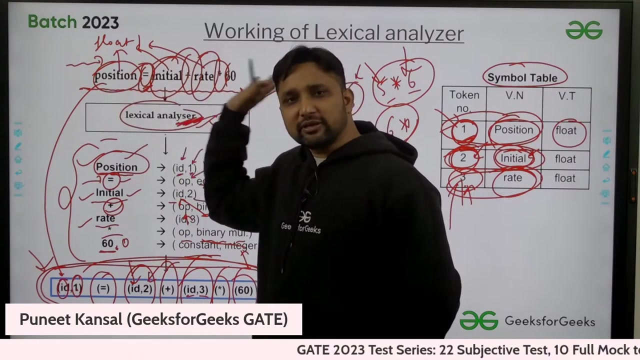 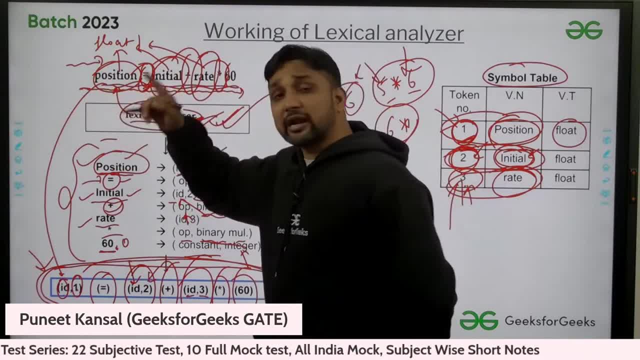 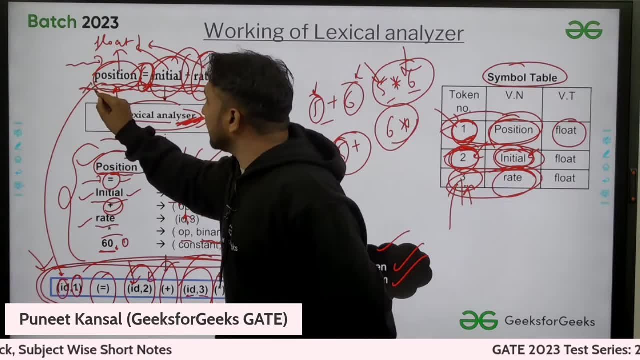 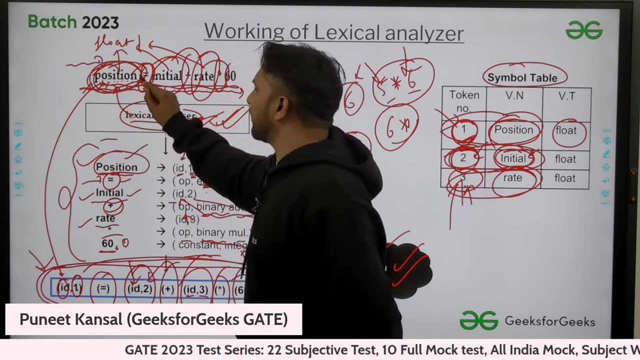 characters. scan the string. this string actually character by character, character by character. okay, just like character by character means actually that will start from p, then o, then s, in position also p o s i t i o n. after that that gets spaced so that can identify it okay. 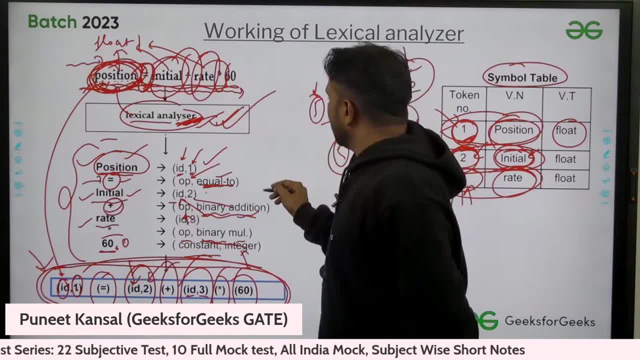 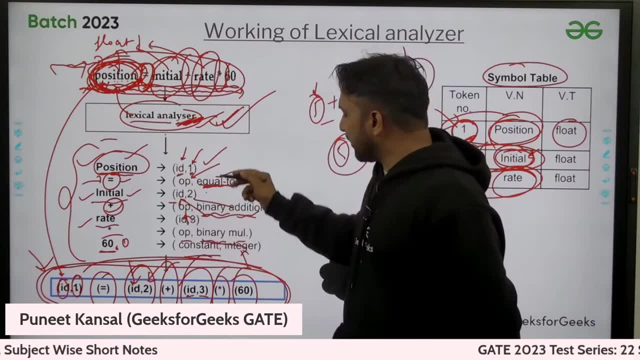 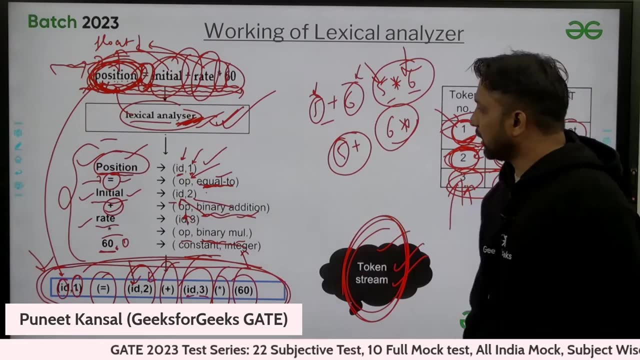 this is a variable. this is a variable. okay, so this is: scan from left to right this stream, this complete string, character by character, and what is the output? somebody ask you what is the output of lexical analyzer, token stream, token stream, and these identifiers are stored into the symbol table. 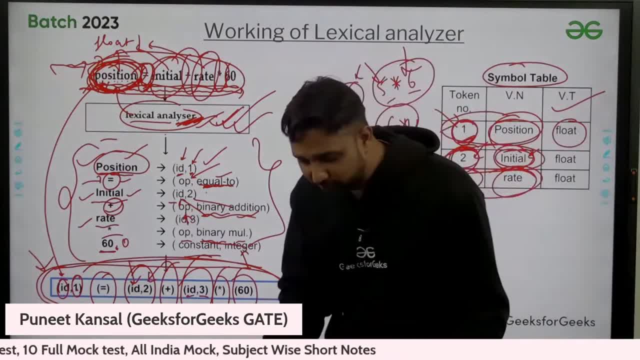 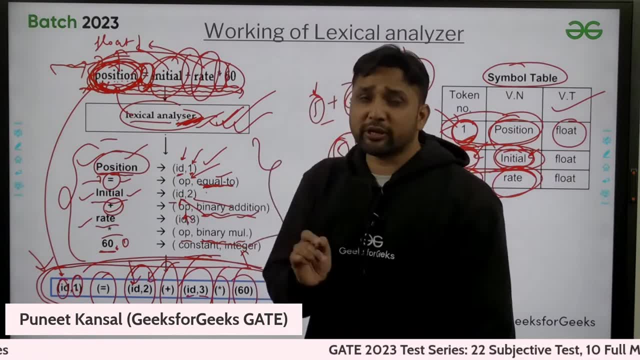 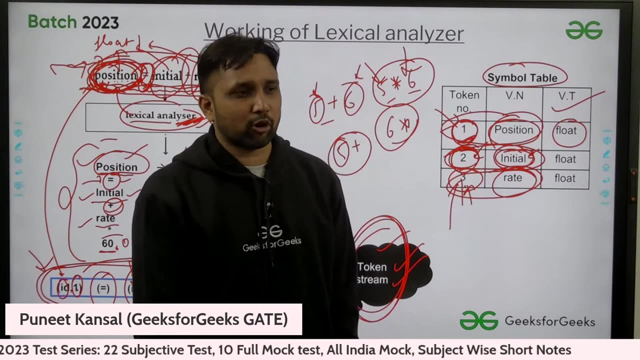 by the lexical analyzer so we get so many information from here. anything else please ask me. ask any question which is coming in your mind. the important thing is that there should not be any doubt in your mind. if any doubt is there in mind, then then there may be. there may be a problem, there may be a chance that you are not able to. 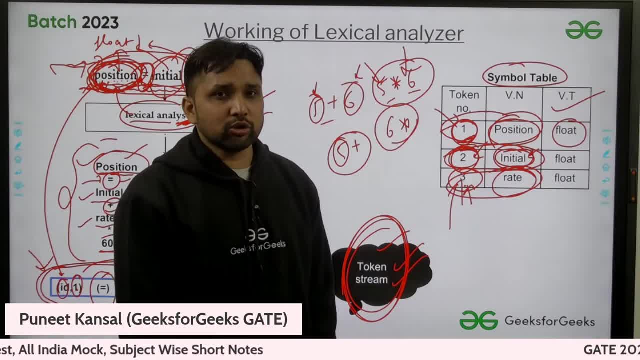 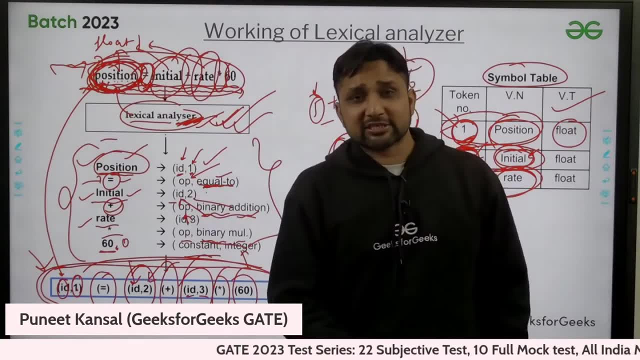 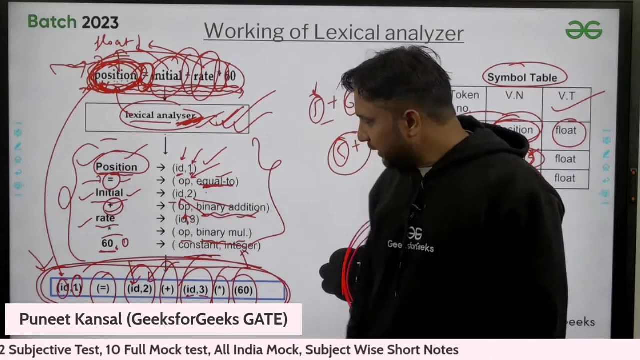 solve the question in exam. but if there is no doubt, i am giving you surety you will be able to attempt every question and you can check it right now in this lecture, when we will attempt previous year questions, you okay. so please write if you have any doubt. clear that doubt, then we will move on. simple that is. 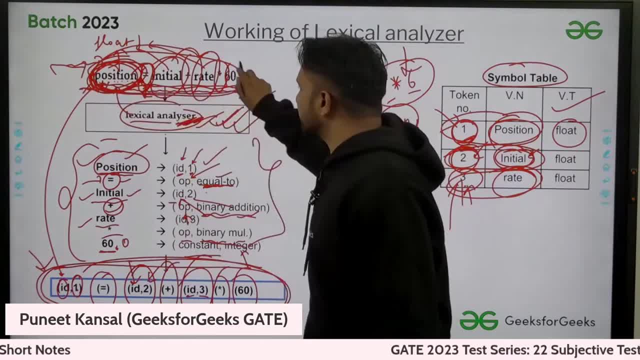 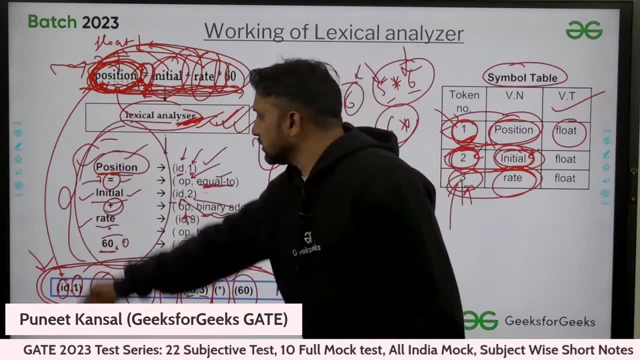 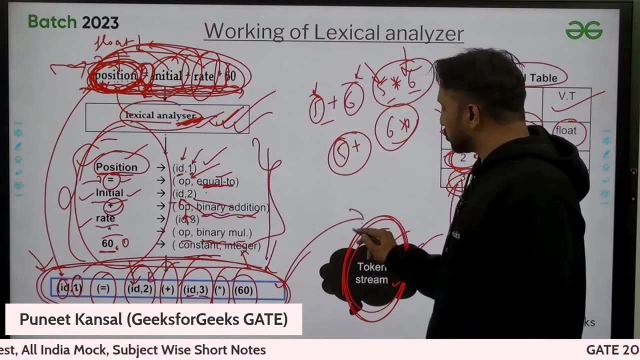 taking this stream of. this is a string, complete string, as a input, scanning it character by character, identifying the tokens and after that, that is, generating a token stream. this token stream is given pass on to the second phase of the compiler. this is the first phase. lexical analyzer. 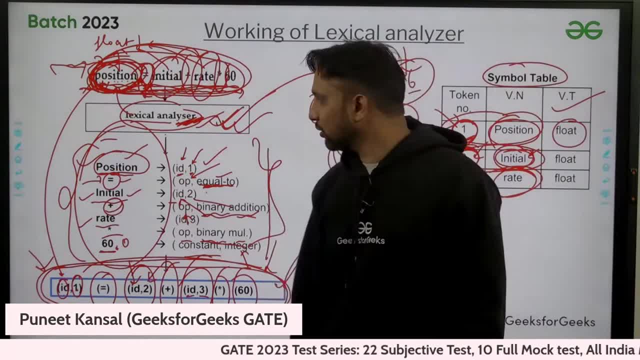 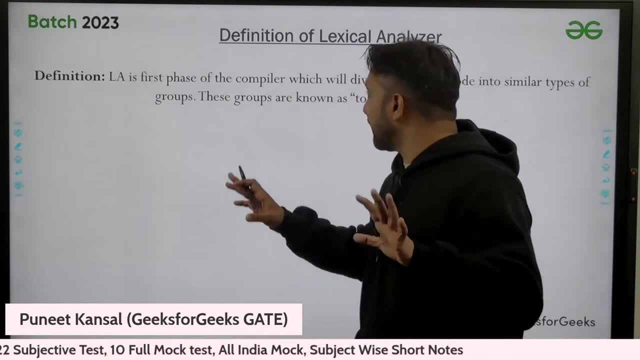 second phase of the compiler is the first phase of the compiler. this is the first phase of the compiler phase of the compiler is actually syntax analyzer. okay, okay. so that's it about it. now, again, from very basics. definition of lexical analyzer. now you can understand the definition. 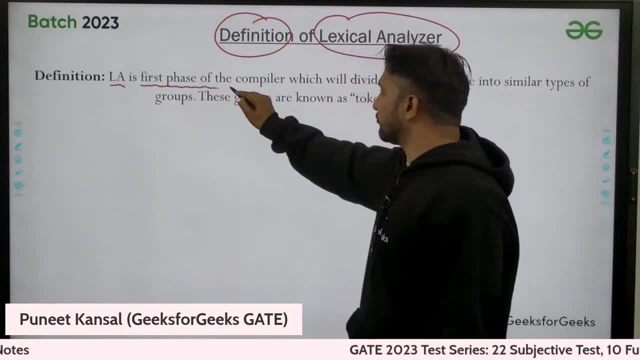 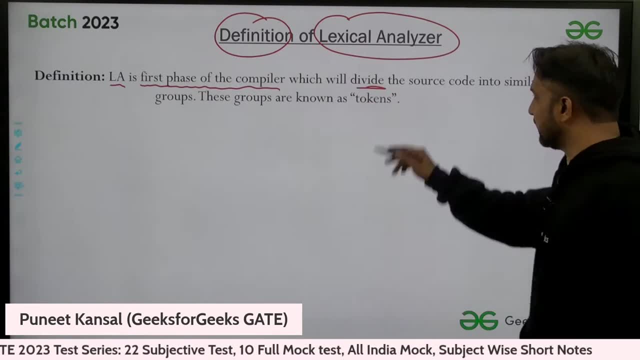 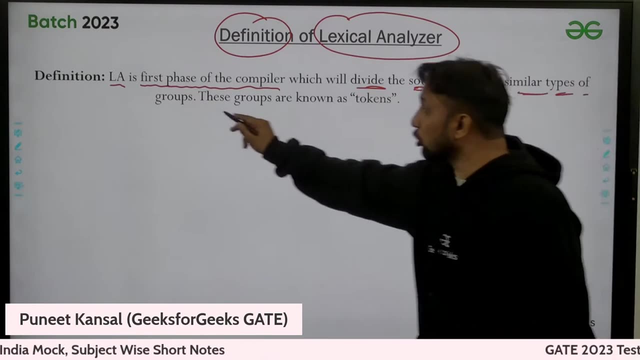 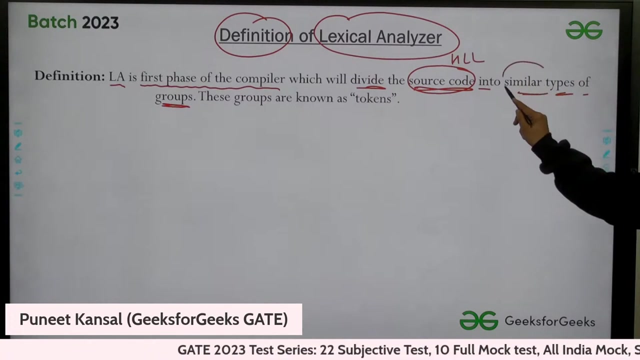 also so. lexical analyzer is the first phase of the compiler. yes, you people already know this thing which will divide the which will divide. you already know this thing which will divide the source code high level language into smaller, similar type of groups, which divide the source code high level language statements into similar type of groups. 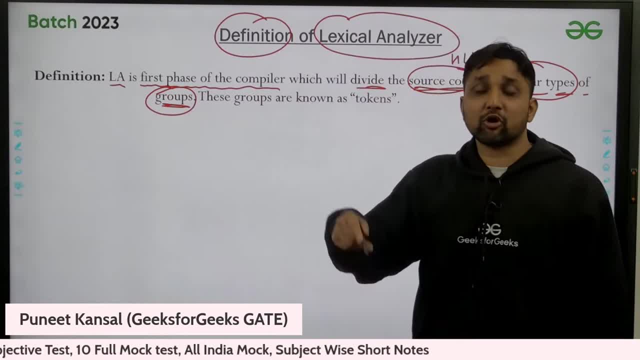 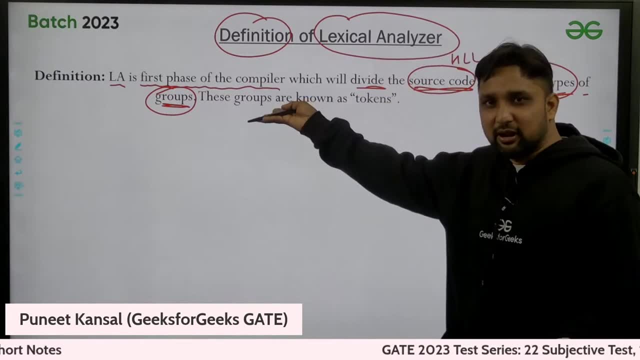 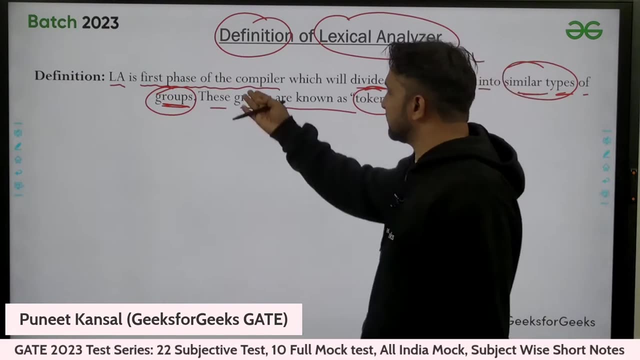 like operators, like identifiers, like constant. these are different groups, groups of tokens- okay, simple, that is given in the definition what the lexical analyzer is, and these groups are known as the tokens. so you know, you people know what is the definition, what this step in the definition is talking about. even we can understand with this diagram in more clearly same thing. i am repeating. 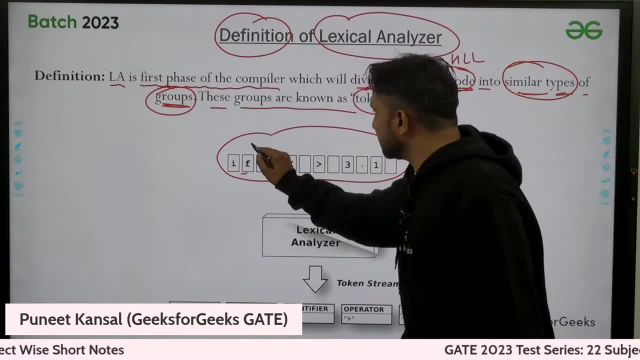 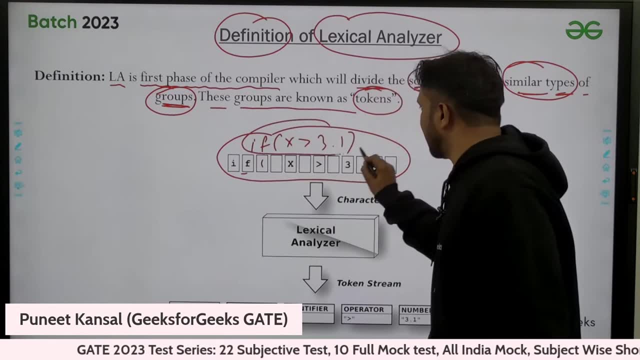 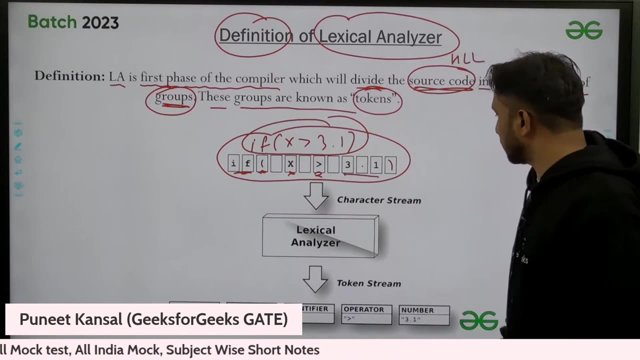 again and again we have a statement. if this statement, let me write it right here: if x is greater than 3.1, this is the statement- high level language. if this is the opening bracket, x is greater than 3.5, let me write the closing bracket also, okay. 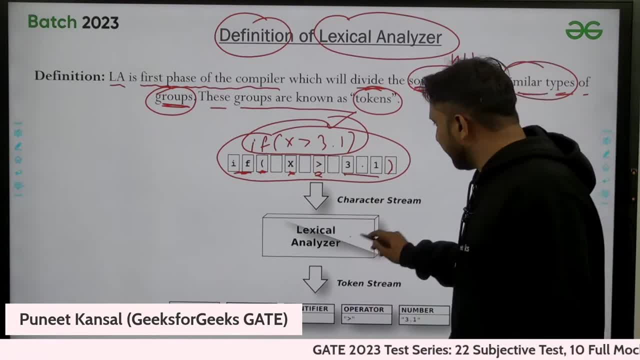 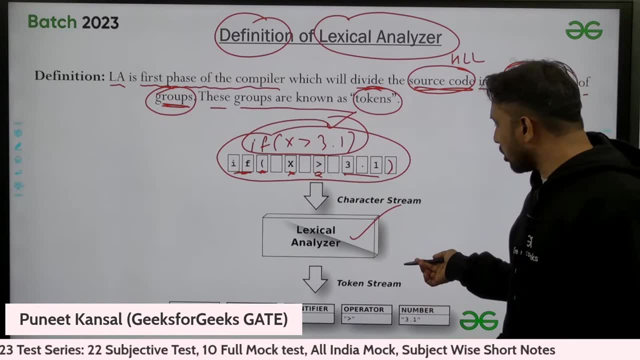 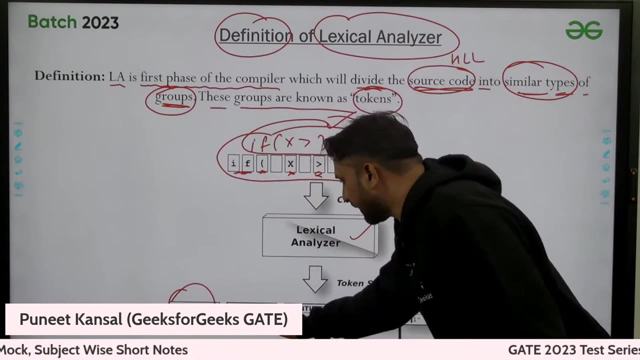 so this is the high level language we have. we give it to the lexical analyzer and that what that is doing? finding out the finding out the tokens, finding out the tokens like: if is a keyword. if is a keyword. these are the brackets x is an identifier. we use one identifier, x only here. 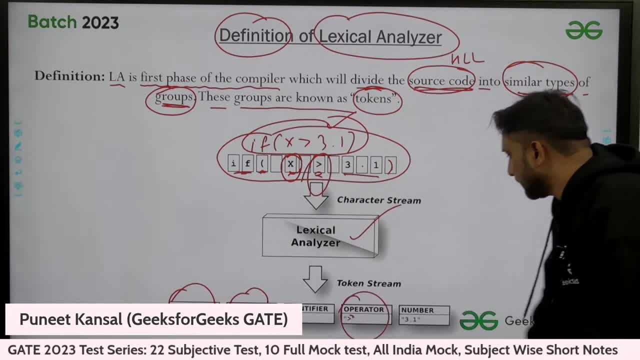 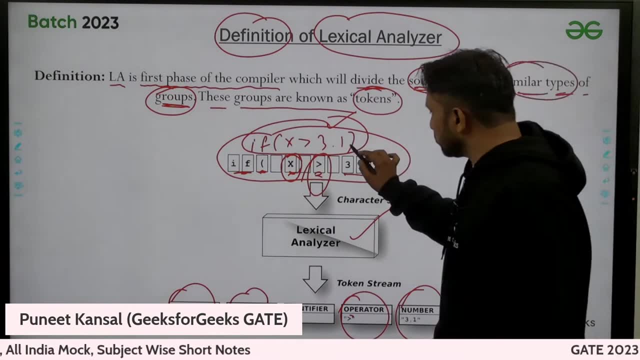 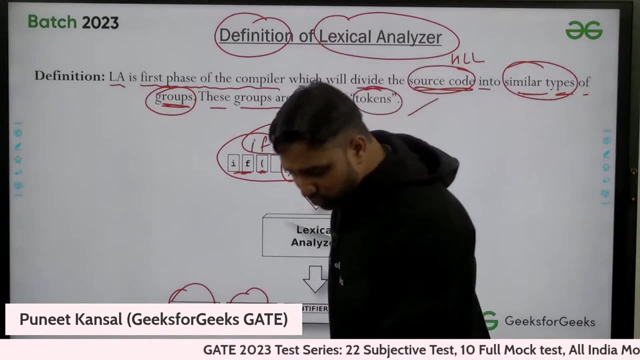 greater than is an operator. greater than is an operator. three point one is a number. three point 3.1 is a number, or you can say that, constant number. okay, so these are same thing, given in the definition also. okay, one more thing i'm adding here in this slide. actually, i have one more thing. 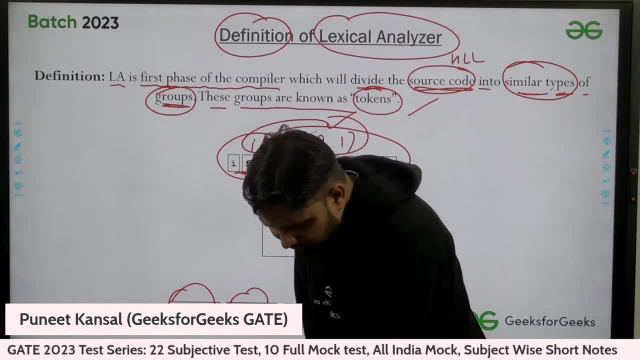 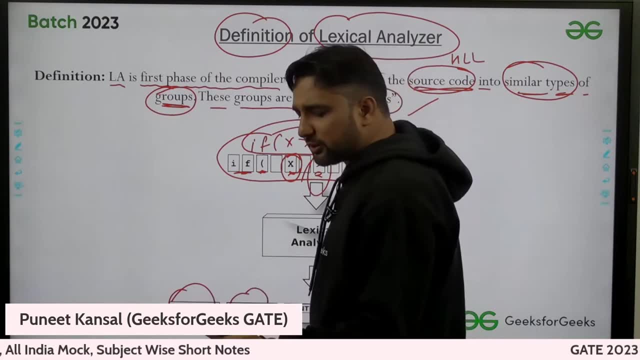 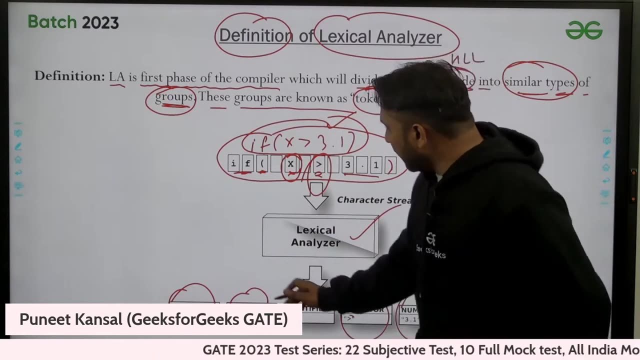 and uh, yes, uh, you're asking that, okay. uh, sir, only identifiers are stored in symbol table. yes, only identifiers are stored in symbol table. okay, only identifier. see you people tell me: okay, okay, compiler know about the compiler know about the operators or not? compiler already know about. 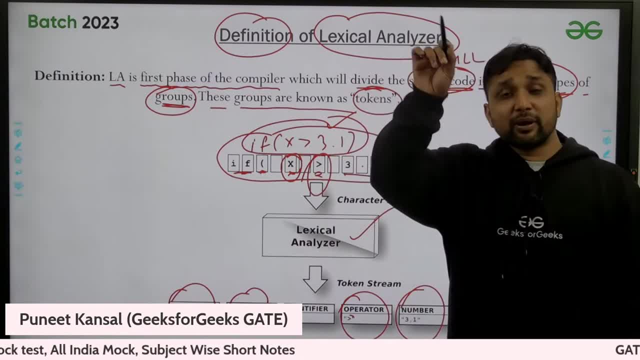 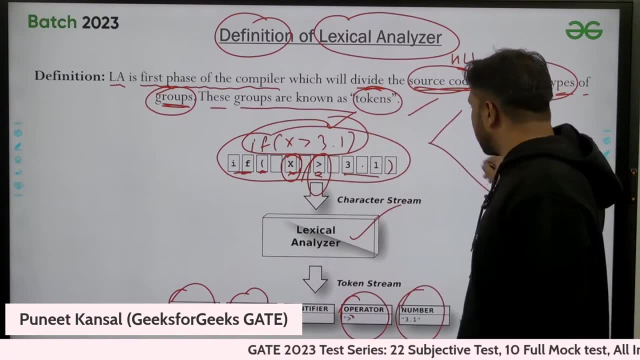 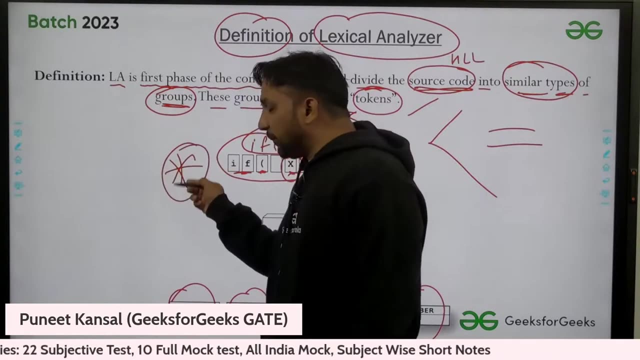 all the operators compiler are. when i, when somebody was designing the compiler, that will define: okay, this is, this means, is greater this one, this mean is smaller this man, what means means smaller? this one? this operator means is equal to this is multiplied. so if we will not define the meaning, 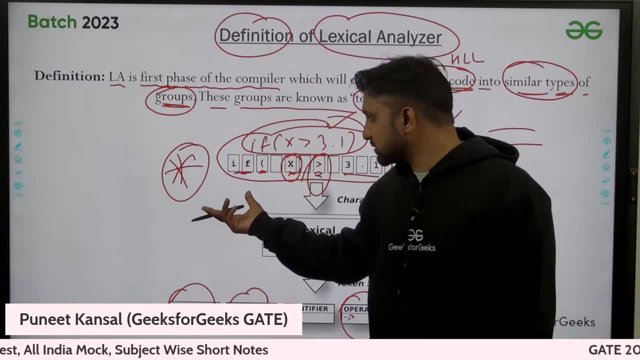 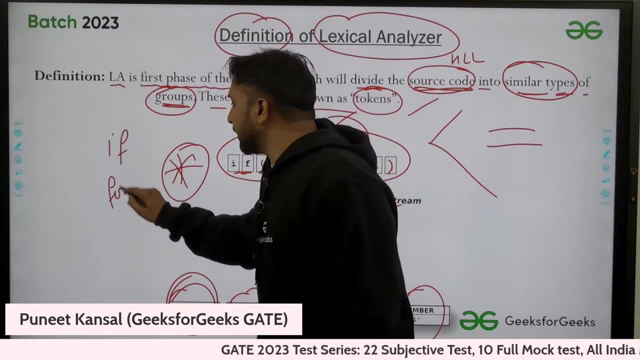 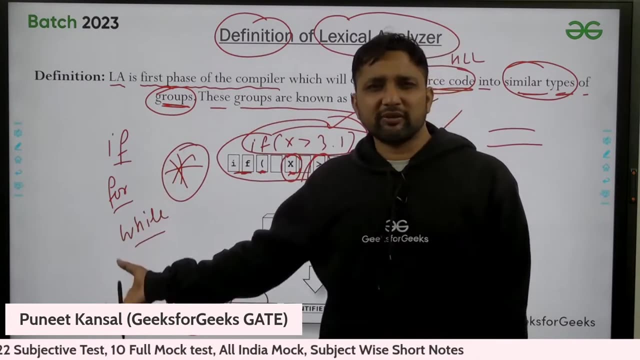 how we will use them if a compiler don't know these operators. okay. and another thing: keywords. also keywords compiler already know about. if statement for statement, while statement, these are keywords. these are keywords already defined in the compiler. if they are already defined, why we are unnecessarily storing them in symbol table in. 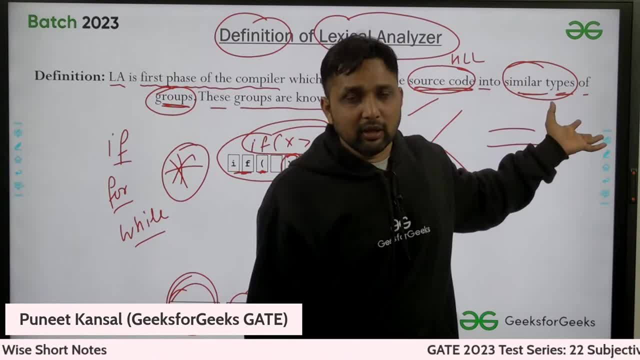 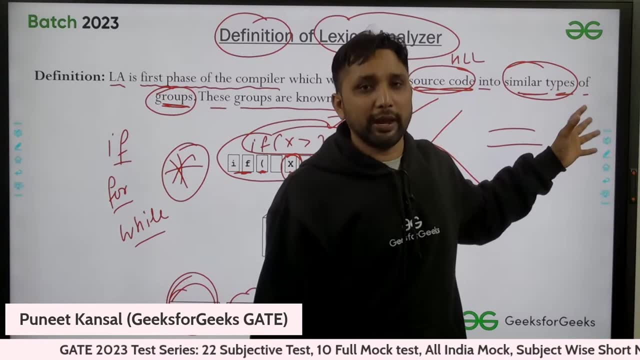 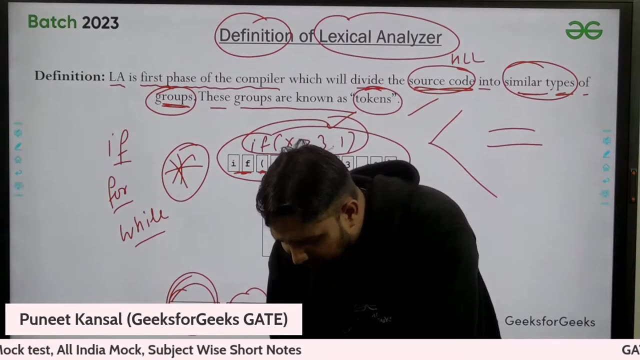 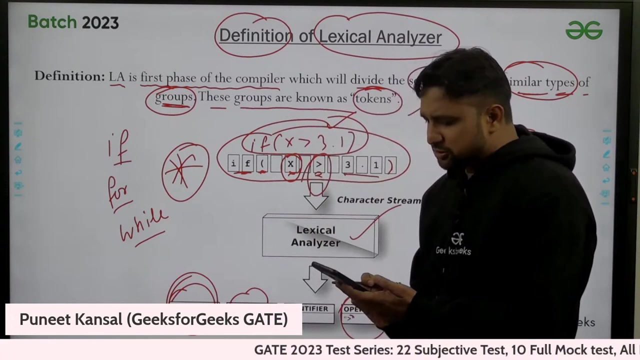 our in our data structure symbol table, we will store the only those things in the symbol table which are which are new, which are new and identifiers are the new one. identifiers are the things which which you are entering into the which are giving as a input. okay, okay, i will come to your question. next question is from: uh, sign up, is this course is? is this? 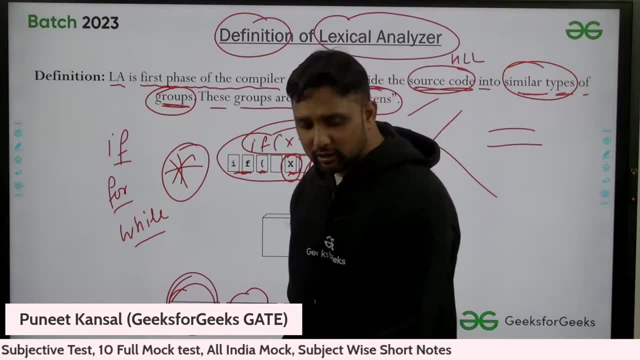 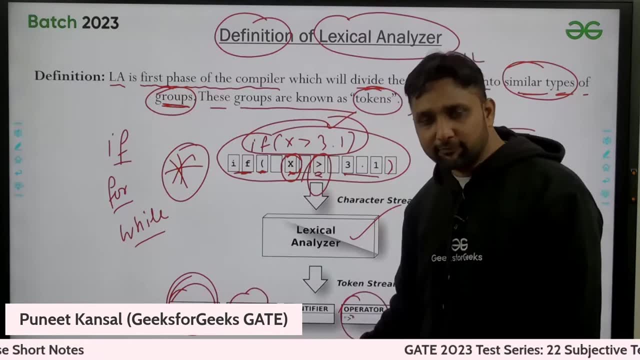 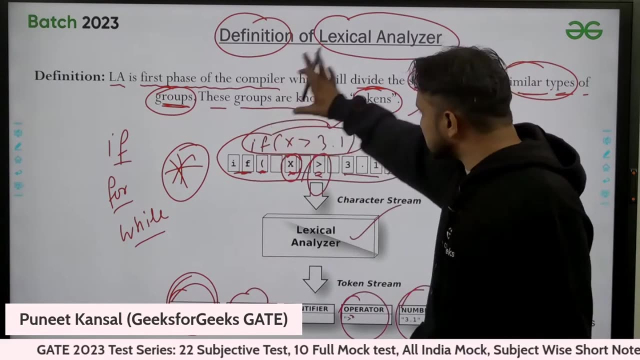 crash course is sufficient to to solve questions of gate. i will solve here 10 to 15 questions from gate, from lexical analyzer. i will solve here itself and you people will also be able to solve you. so you will solve yourself. i will not solve you, people will solve yourself. i will just giving you this information. 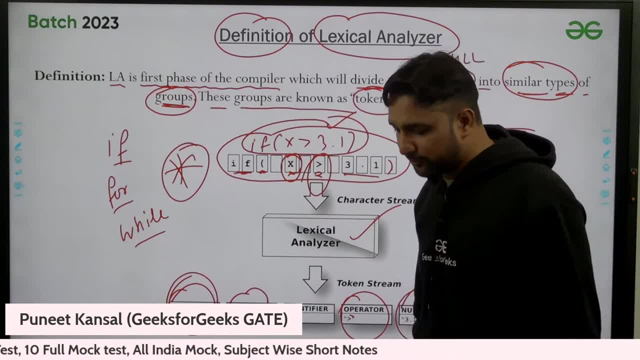 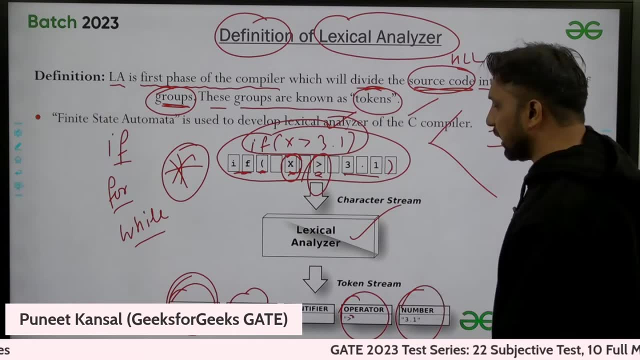 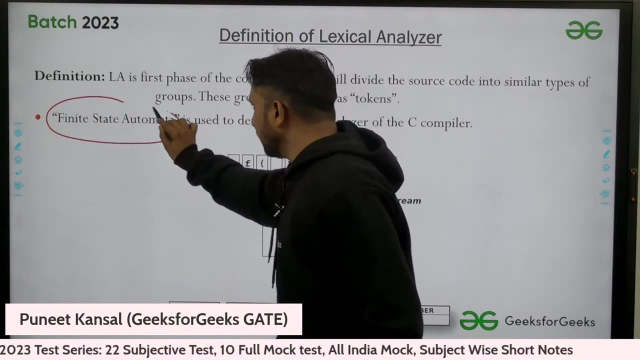 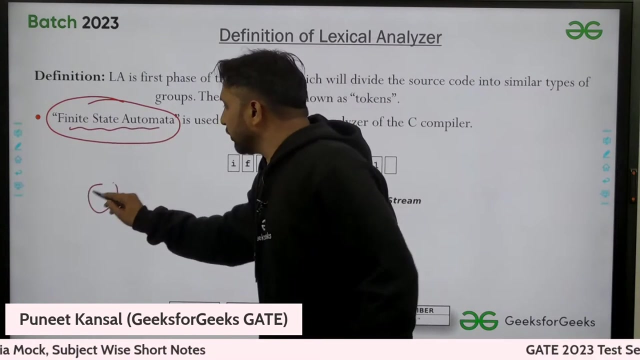 if you know this information, you can solve. that's it, okay. okay, so this is about the lexical analyzer. one more thing i want to add here is that let me erase this screen. first, and this is also important, lexical analyzer is developed actually using finite state automata. if we know about little bit, 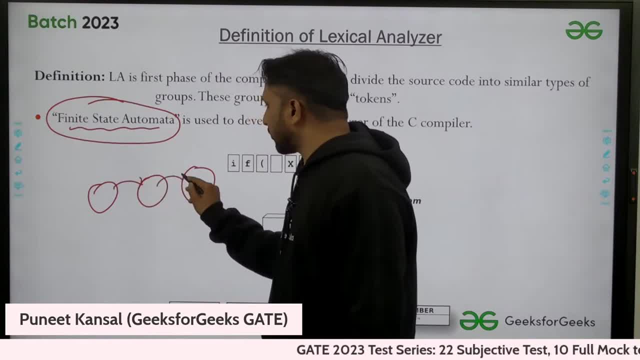 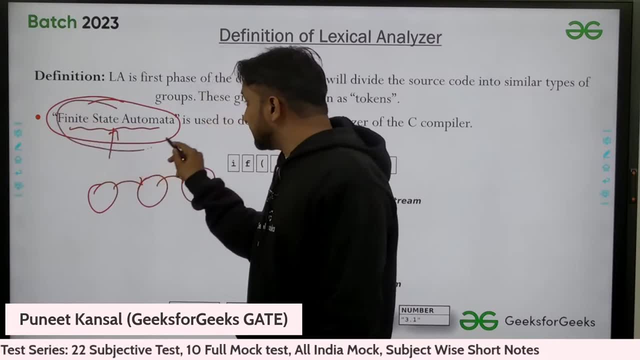 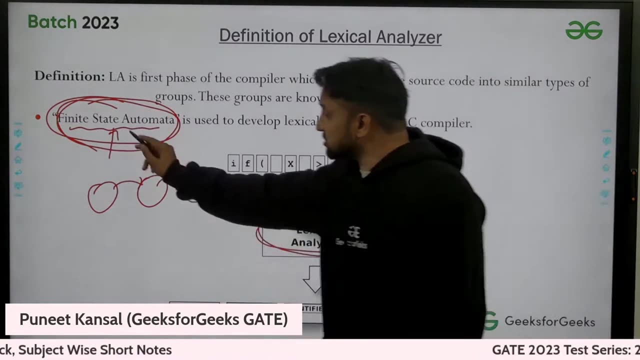 about automata. so we have states and we make the transition from one state to another state. okay, so we know a finite state, automata. so we are using this machine. this finite automata machine actually is working behind the same, behind the lexical analyzer. this machine is actually 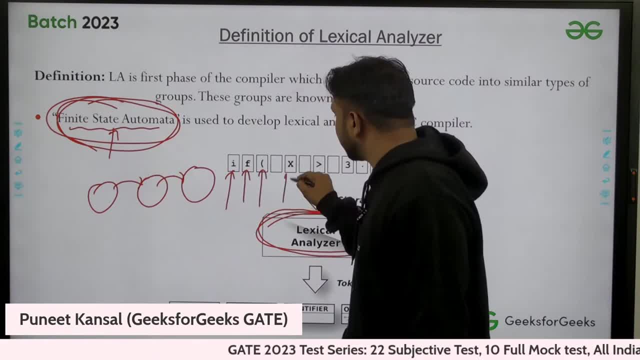 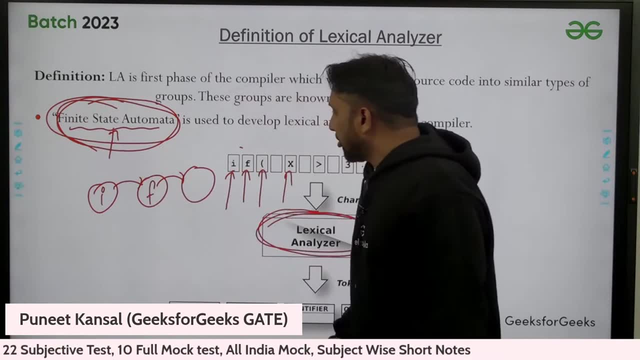 scanning the characters one by one. that is, scanning the characters one by one. so maybe it's like that. okay, first i will find i, then i find f, and i find f is just f. so let me change this thing, that i find space, then i can say that, okay, this is a keyword, this is a keyword, so this should be the. 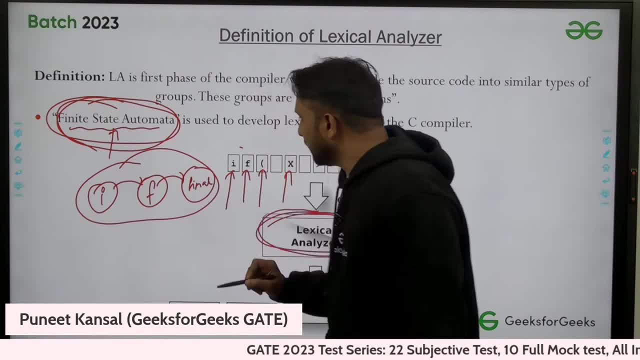 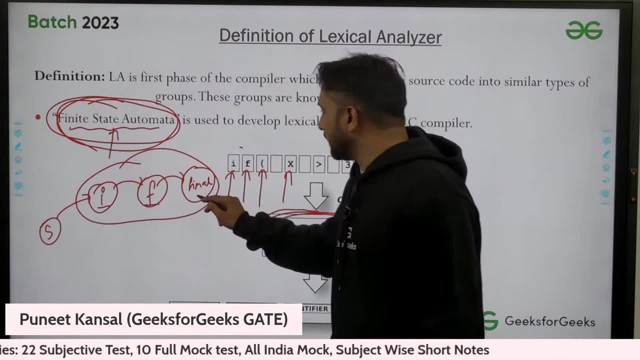 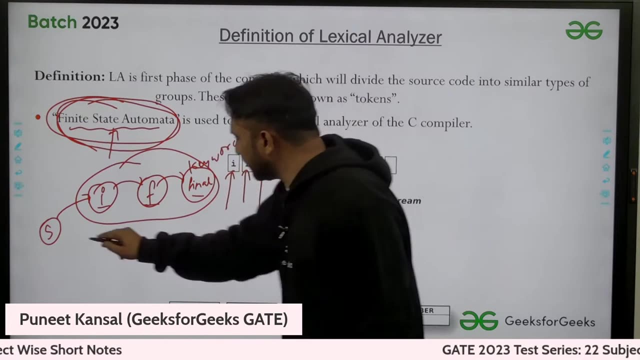 this should be the final state. final state, okay. similarly, let's suppose this is our start state. i start from here. first i find i, then i find f and then i find space and i say that, okay, this is my final state and i can say that this is a keyword, this is a keyword. similarly, i can go for: 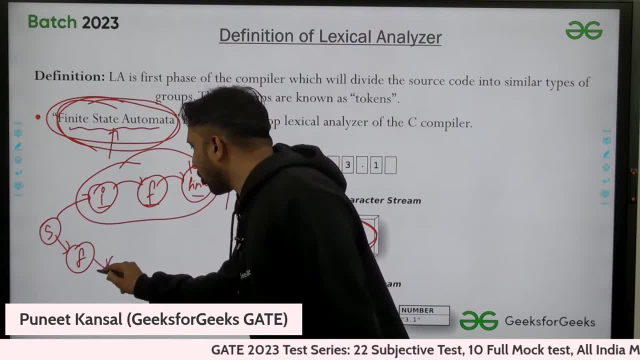 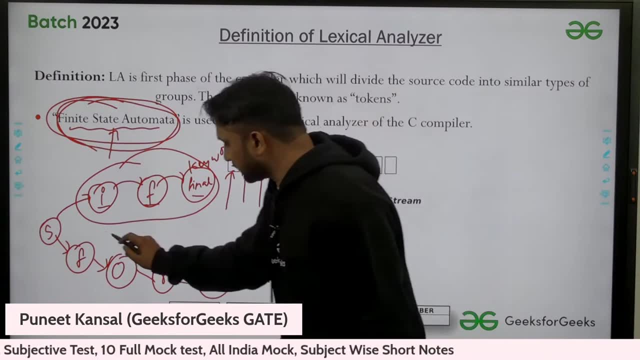 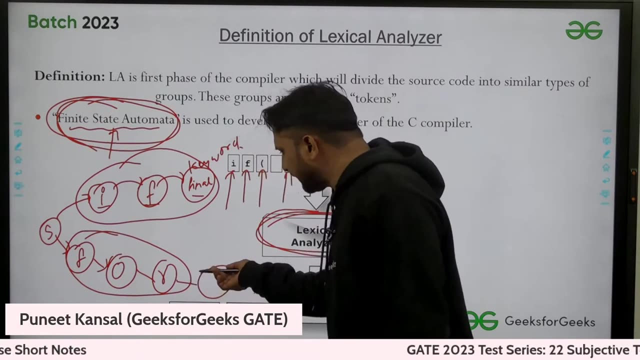 others also. i find f first, then i find o, then i find r, and after that i find space. after that i find out space. that's means this is a, this is again a keyword, for is again a keyword. but after this, if i find out something else like k fork, now this is not a keyword, this become a variable. 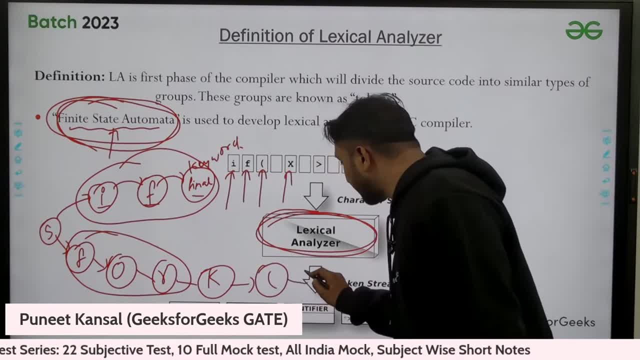 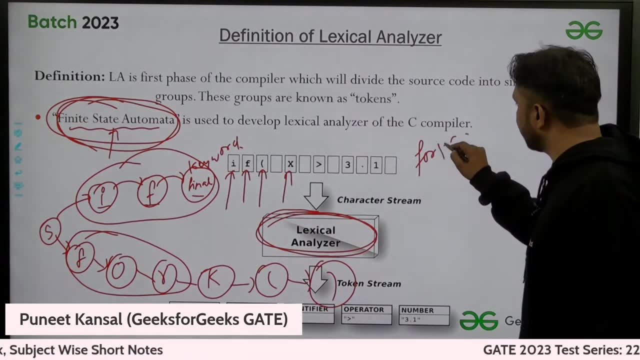 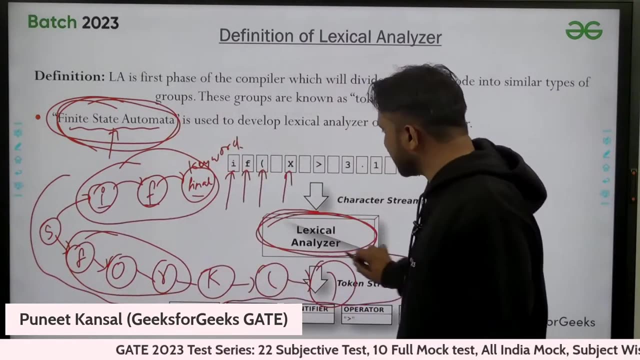 maybe after that, if i find out, opening bracket and closing bracket, opening bracket and closing bracket. now, this, this become a function. what is the name of function fork? okay, so this is: these all are developed with the help of the, this machine. actually, all the keywords, everything is developed. 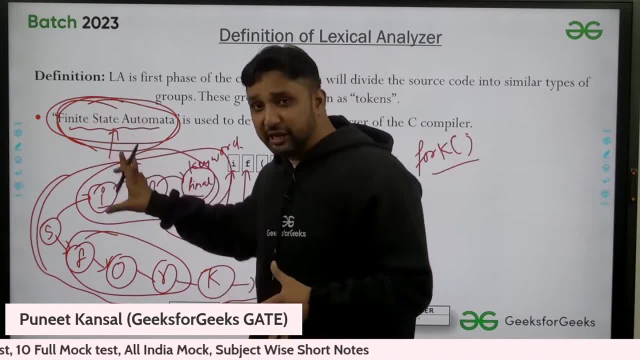 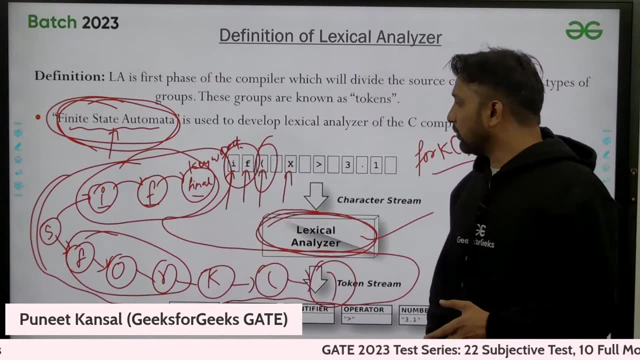 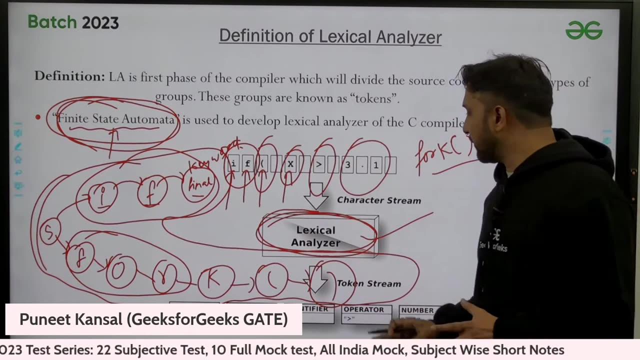 with the help of a big finite automata machine. this machine is working behind the scene, which is finding out. this is, this is keyword, this is a, this is the opening bracket, this is identifier, this is a operator, this is a constant. these all are identified with the help of finite automata. 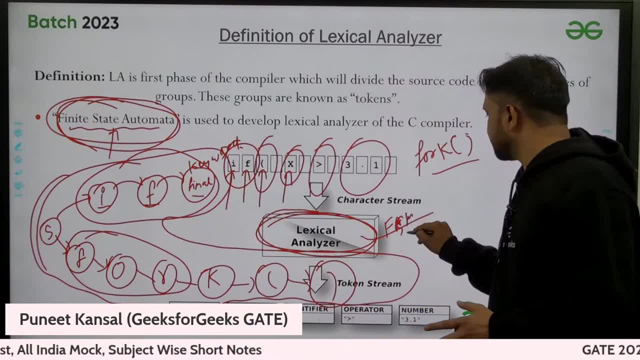 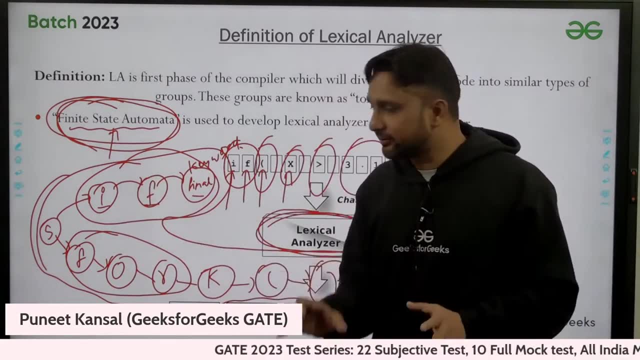 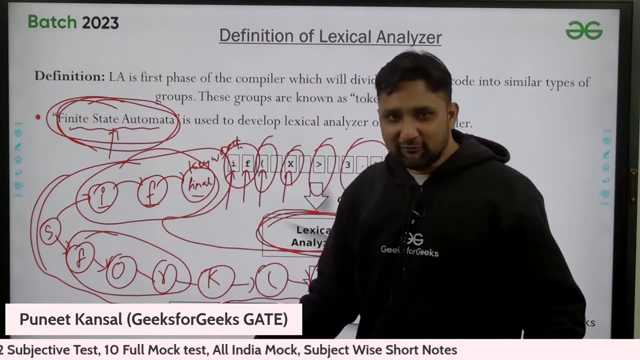 finite state automata. okay, this machine is working behind the scene. this is the only thing. you need to know how this machine is working. you do not need to go inside that. i just give you an idea how this machine is working on. otherwise, you do not need to develop this machine yourself. 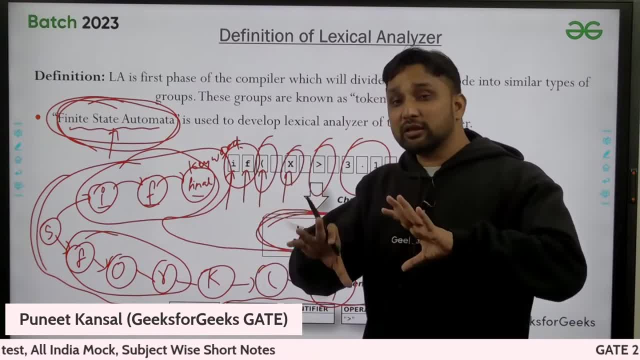 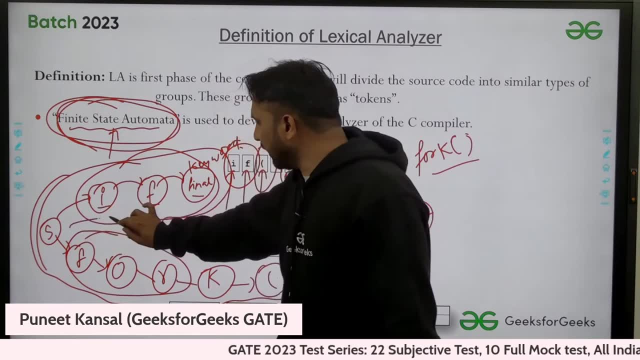 they are not going to ask you how this machine is developed actually. you do not need to ask you how this machine is developed actually. so you need, you need to just know that. okay, a little bit. you need to know the idea, okay. uh, if we are starting, let's suppose, if we are finding, if keyword, then there must be space after. 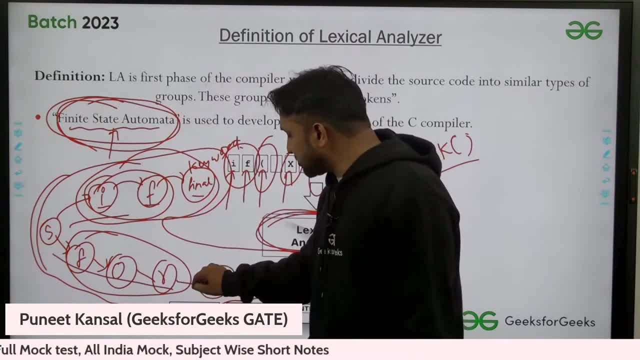 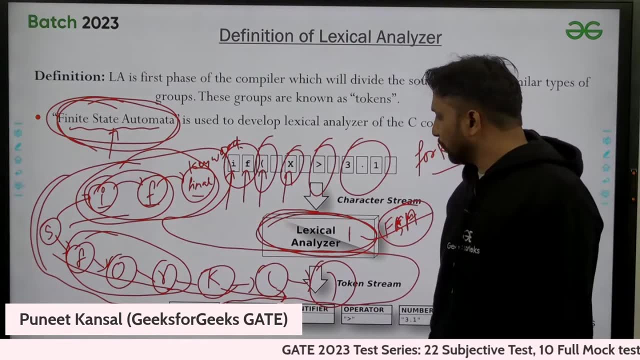 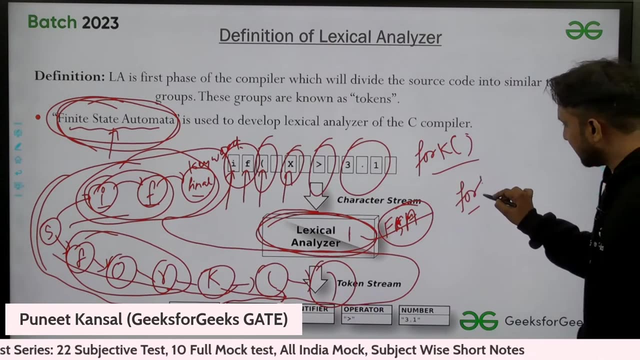 if there must be space after four. if there is no space, then that become a variable again. if you find out bracket, that become a function. okay. so for being a, for being a variable, for being a keyword, you need a space. if i add something else, then that become a variable, okay. so 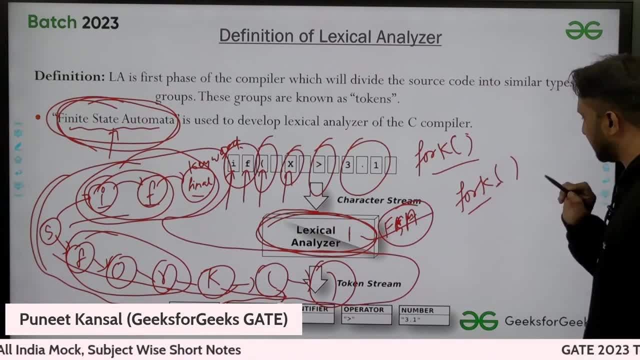 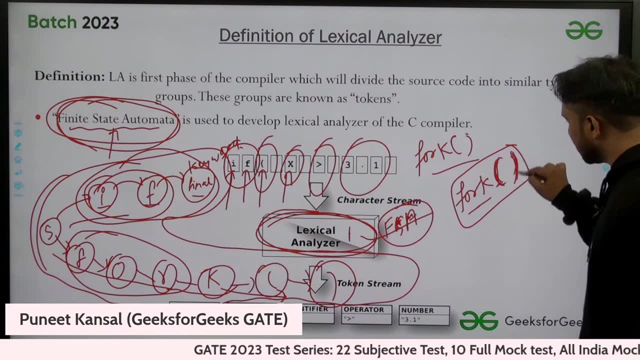 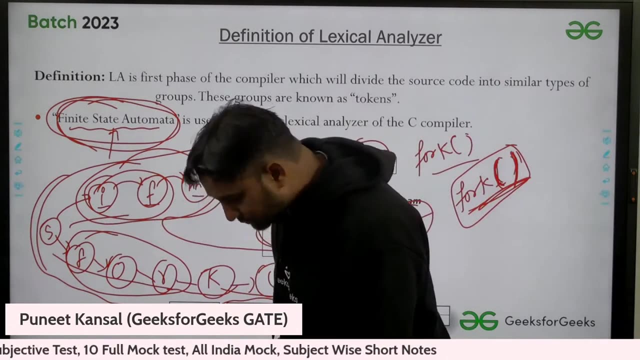 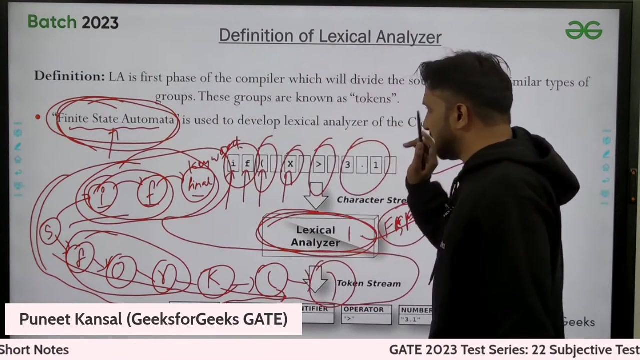 variable. but if i again i add something, i do not give any space here, i add brackets, this become a function. this become a function because we know that every functions have these brackets, okay, okay. so only one thing i tell you actually is that one thing i tell you only in this, in this is that finite auto machine, automata machine is actually. 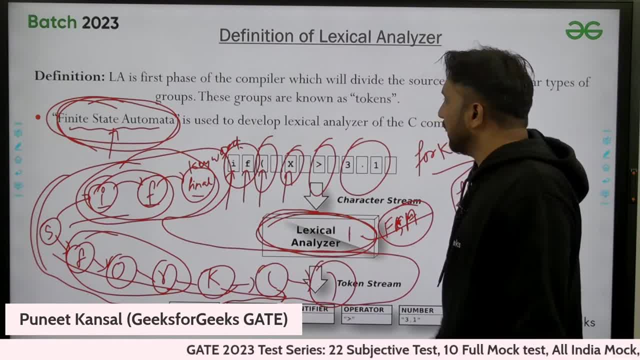 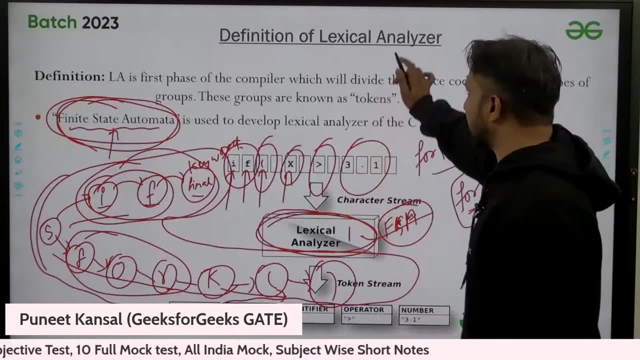 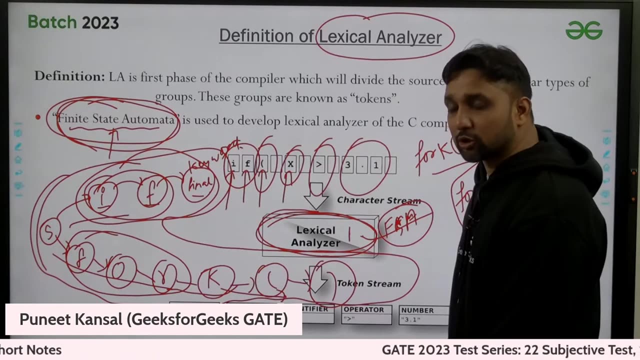 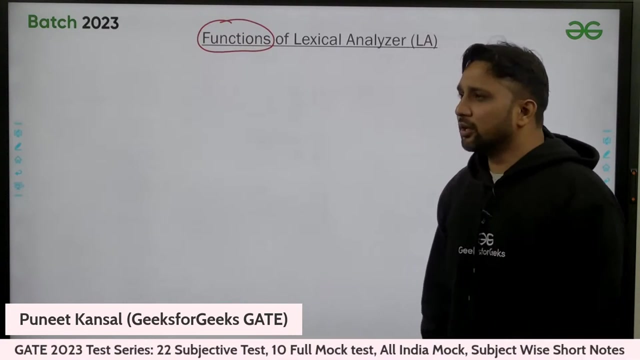 working behind the scene, behind the lexical analyzer, okay, which is finding out the token. okay, so these are thus. this was the introduction to lexiconalizer. now that is finished. okay, i will take two or more, maximum three slides. after that we will solve the questions only, okay. so i'm i'm using a word, i'm already saying you that, okay. 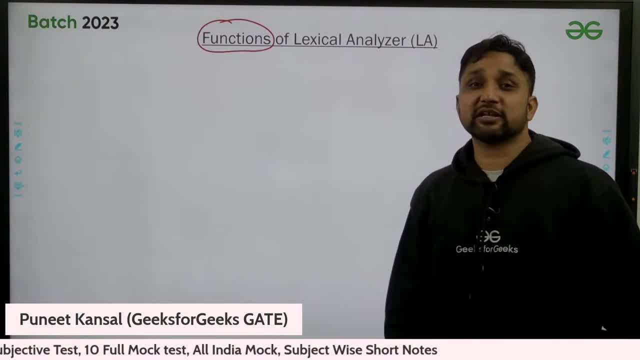 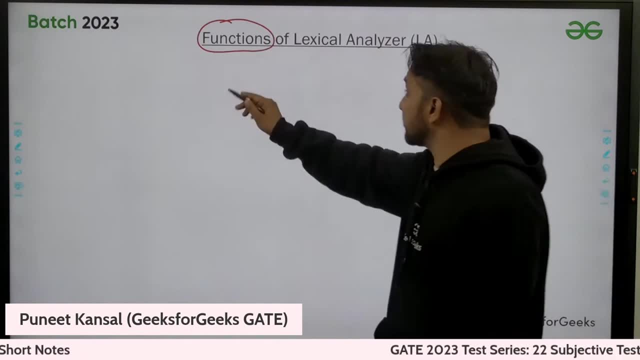 the main function of lexicon lexical analyzer is finding the tokens. main function- i'm saying main function. so there are many other functions also. there are many other functions too. so this is one functions of the lexical analyzer. Lexical analyzer phase, first phase of the compiler. 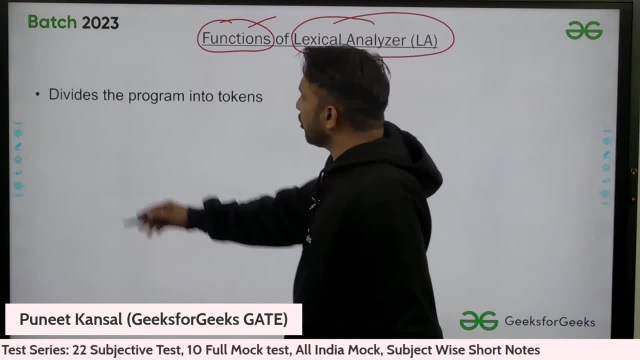 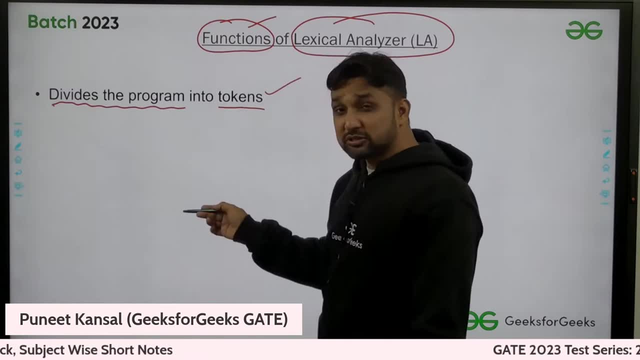 have many other functions. Which are those functions? Okay, this we already know. Divide the program into tokens. This is the one function of we already know. we have already discussed so much because this is the most important one. also, Another functions of this phase: 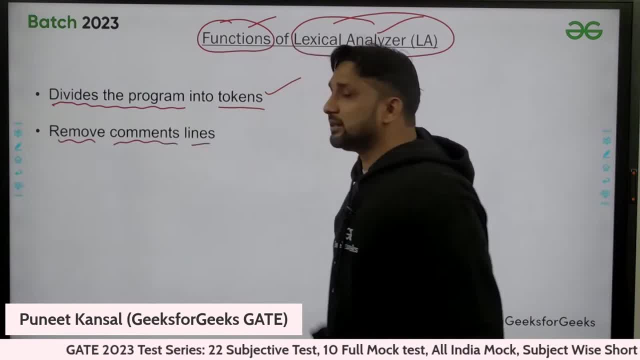 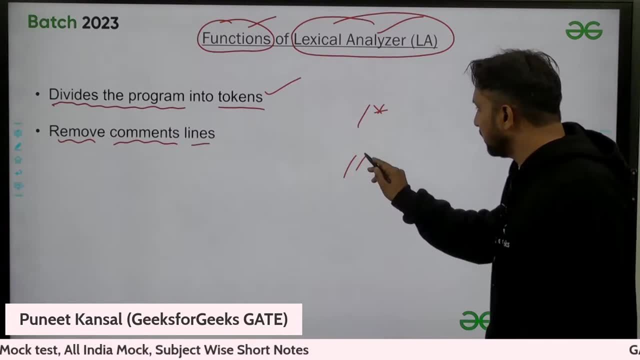 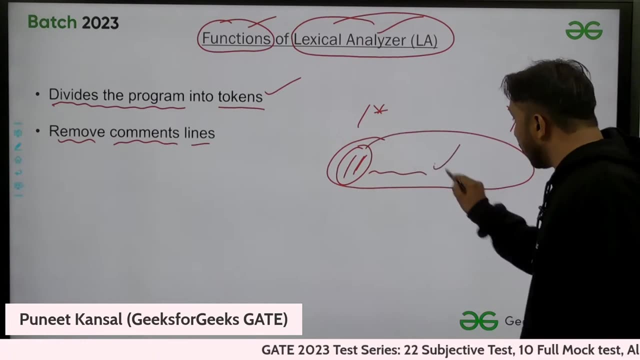 lexical analyzer phase is: remove the comment lines. You must be using the comment lines in your program, Maybe like this, maybe like this in C++. So if you are writing something after this comment, this comment line is removed at first phase of the compiler. They can ask. 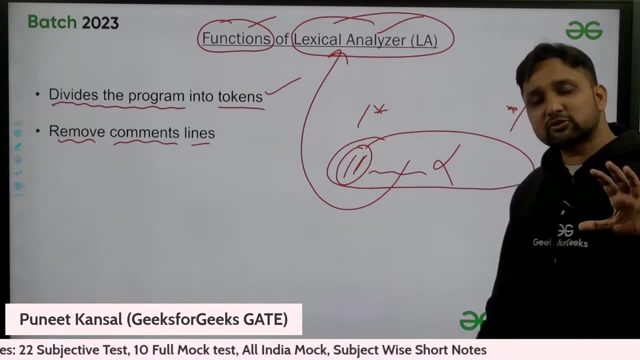 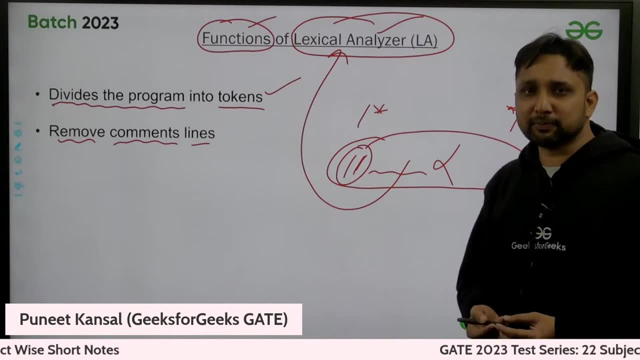 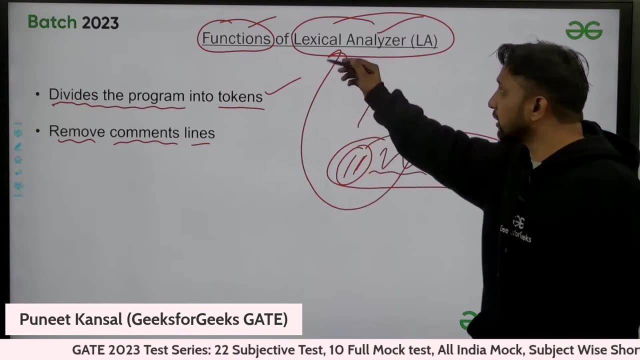 they can see. what they can do is they will ask question from here only. They cannot ask question from out of the concepts. But they can change their question. What they can ask is which phase of the compiler remove the comment? You mention the comments in your program. Who remove the comments? Which phase of the? 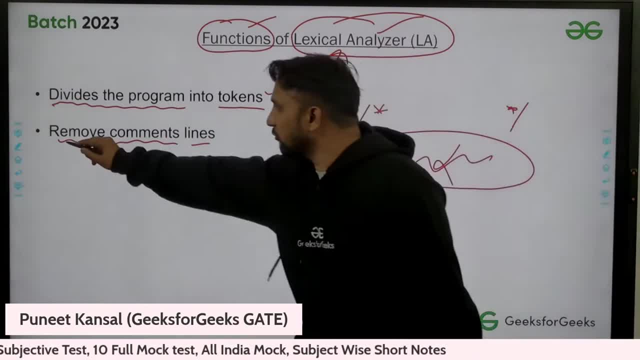 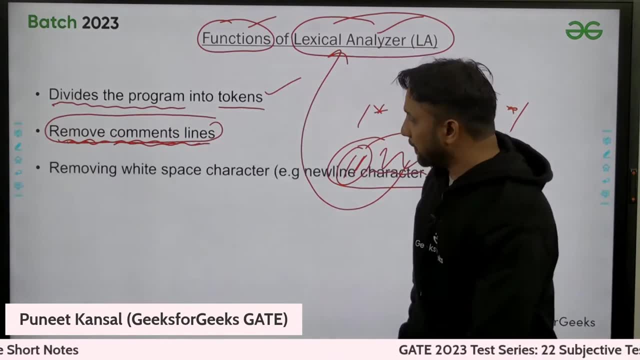 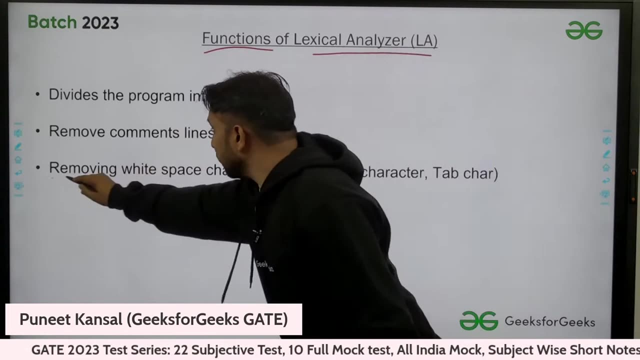 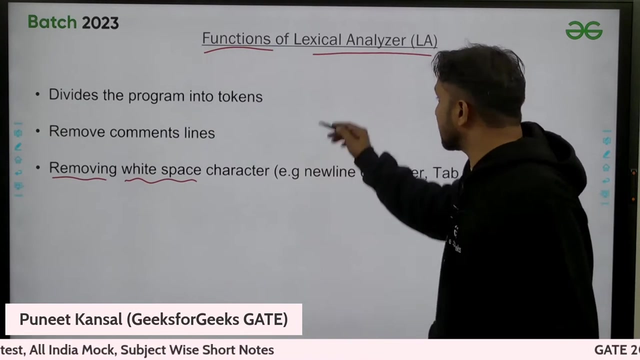 compiler: remove the comments. First phase of the compiler: remove the comments. Who remove the comments? First phase of the compiler: remove every type of comment from your program. Okay, another function of the, another function of lexical analyzer is removing white spaces. See, white spaces are allowed in C language, in C++ also, in Java also, White spaces are. 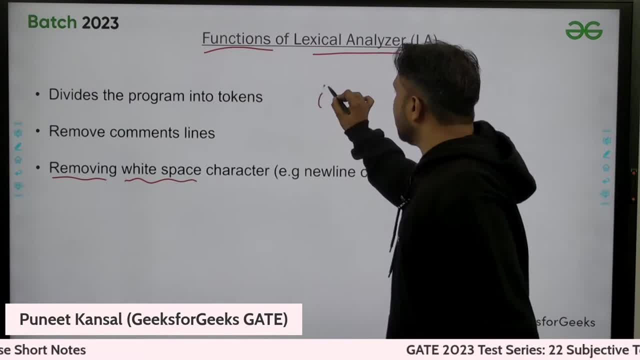 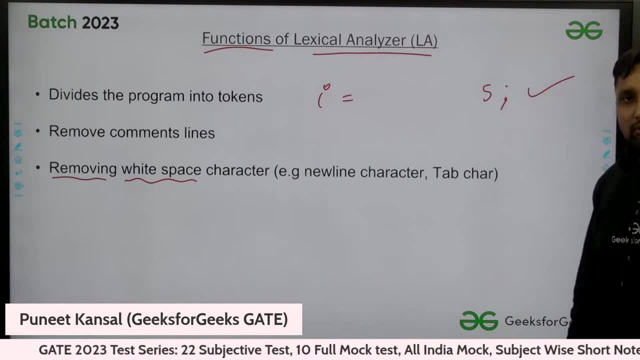 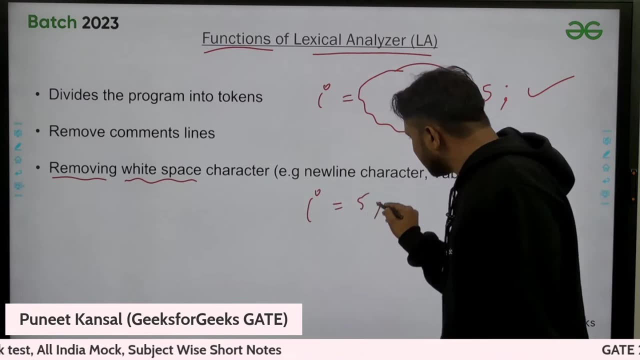 allowed, I will write that. okay, i equal to after tracking 10 space, I am writing 5.. This will work. So this is unnecessary space I am giving, Even though you are giving one space only, this will also work. And if I am not giving space, this statement will also work. This. 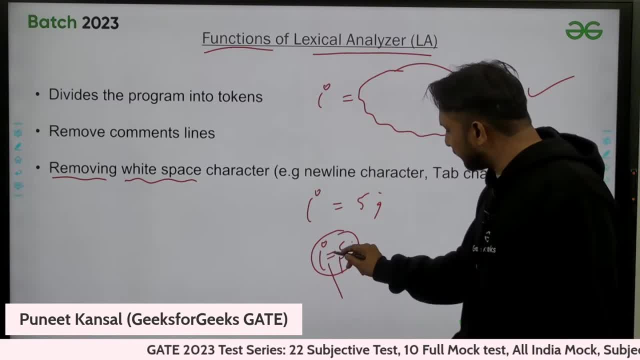 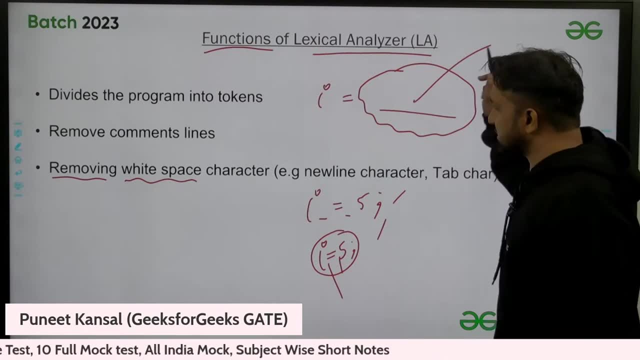 is also working. I am not giving any space between i equal to and 5.. Here I am giving 1, 1 space. Here I am giving lots of space. All will work. So this extra space is removed. This white space is removed. by which which phase Lexical? 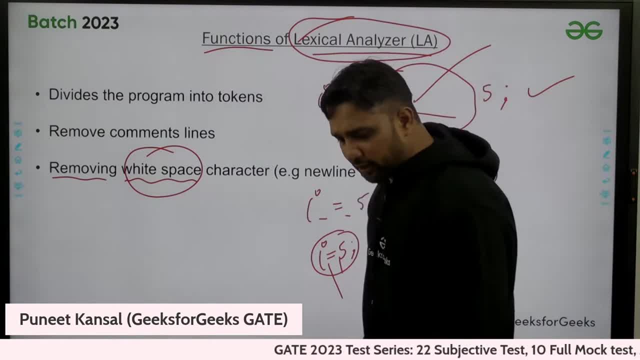 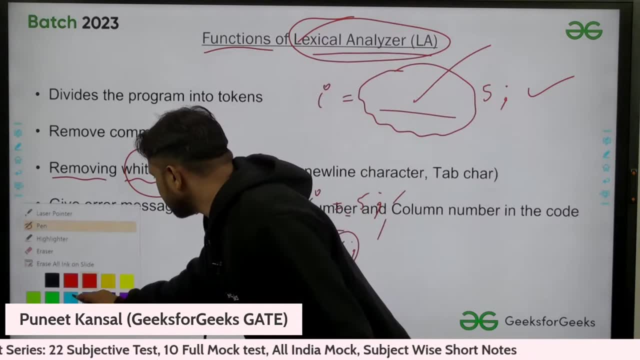 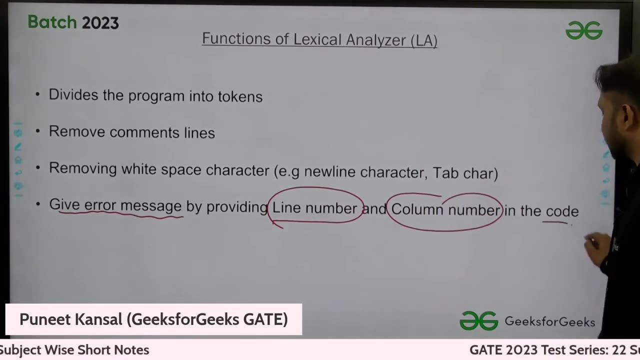 analyzer phase. Okay, okay, I am coming to the comment section. this your chat box, But let me finish this slide. Another one is give error message by providing line number and column number of the code. When you compile your code, you get the error And you also get, okay, in which line the error is. 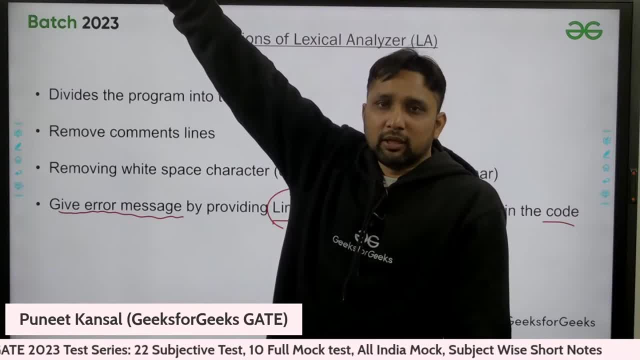 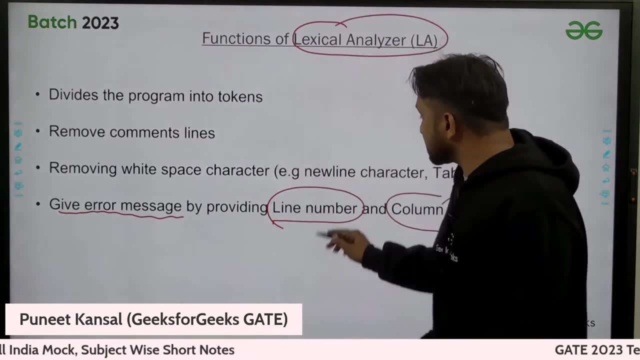 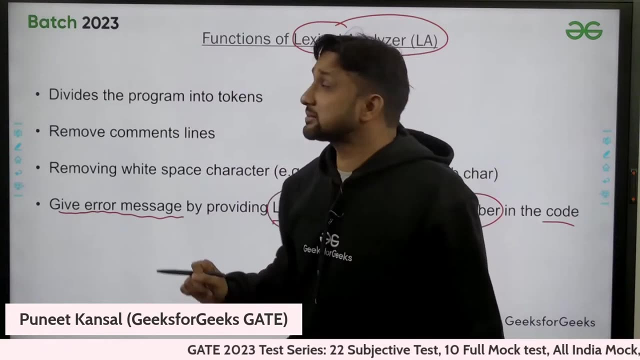 occurring In which line- Line number 50, the error is occurring. So who is telling line number in which line error is occurring? This phrase is helping, Telling us about the line number and column number in which particular line the error is occurring. This information is: 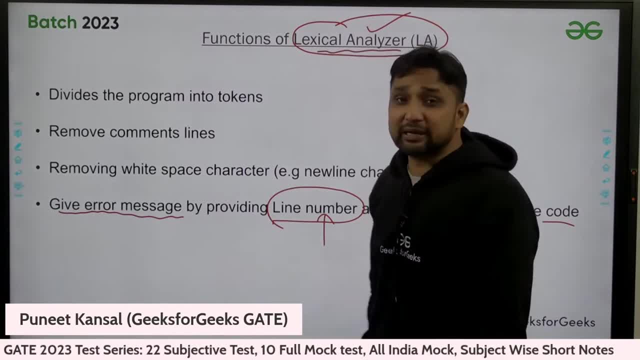 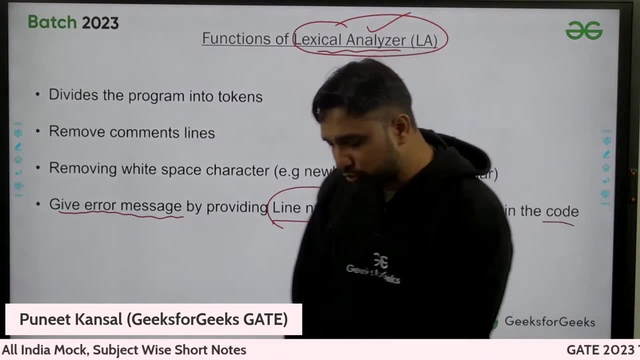 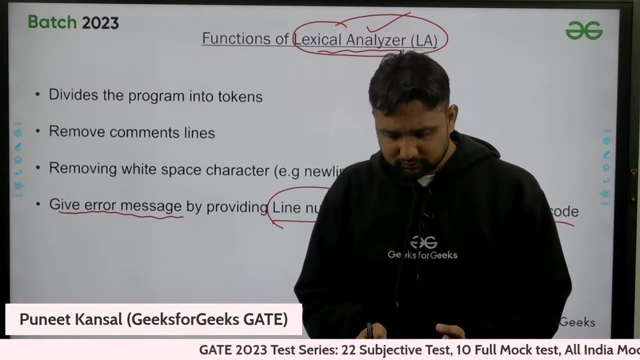 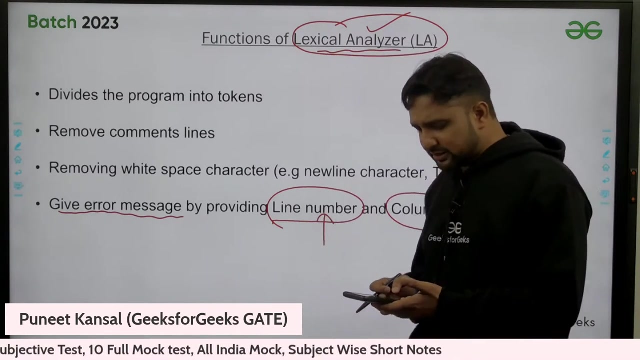 tell us about by the lexical analyzer. Okay, So these are the functions of the lexical analyzer. Yes, These are the functions of lexical analyzer, So let me go to the. you can ask any question till now. Any doubt? please clear your doubt. So you are asking that Jerry is asking. 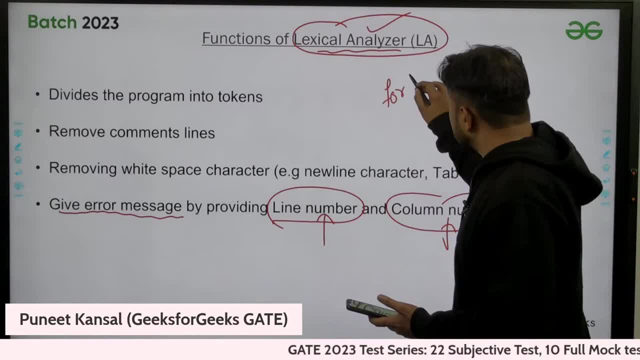 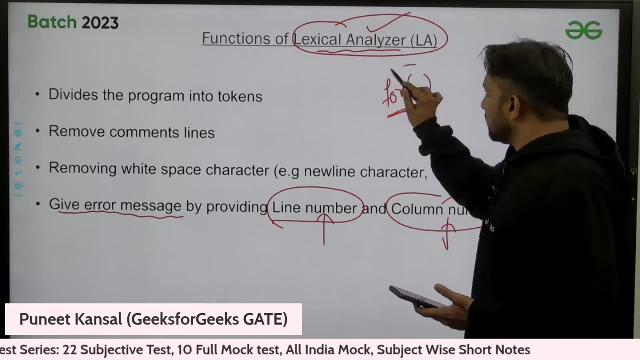 that okay, if there is there is no space. if somebody define it like this: okay, see, if somebody is defining this has no space. So you are asking that okay, if there is no space, if somebody 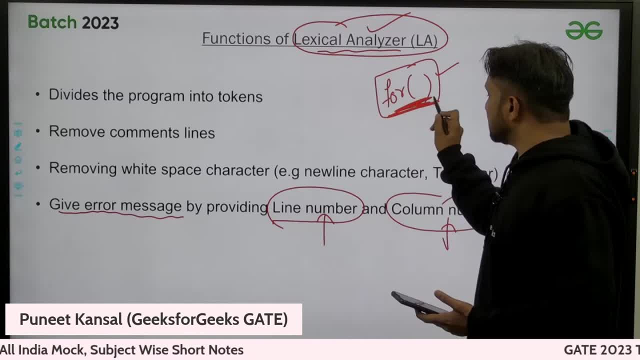 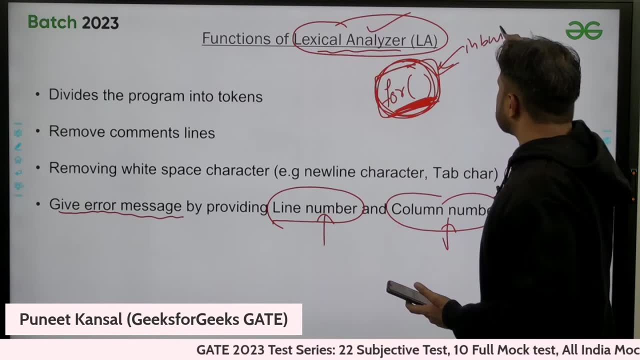 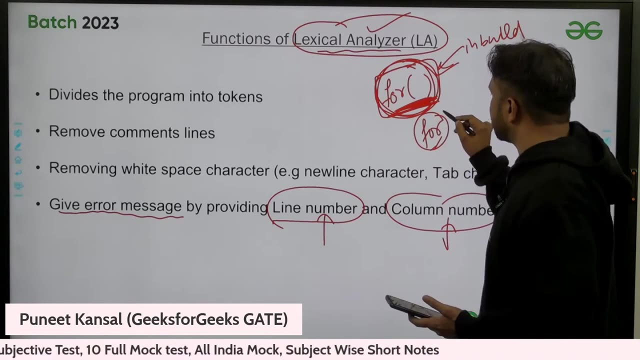 have some. this is again. have this again have different meaning. This is a function. This is a function. This is again a function, But this is a inbuilt function. This is a inbuilt function. Okay, This is a keyword. This function is built with the. with the help of a keyword, you can say: 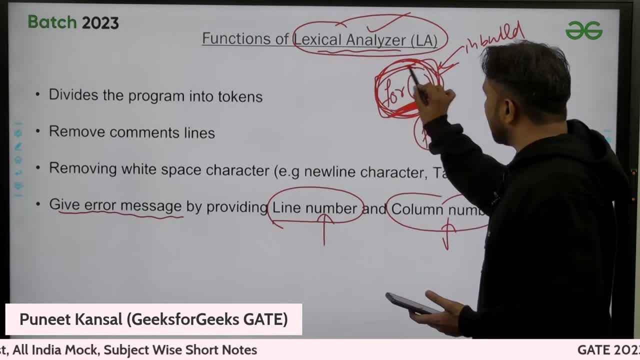 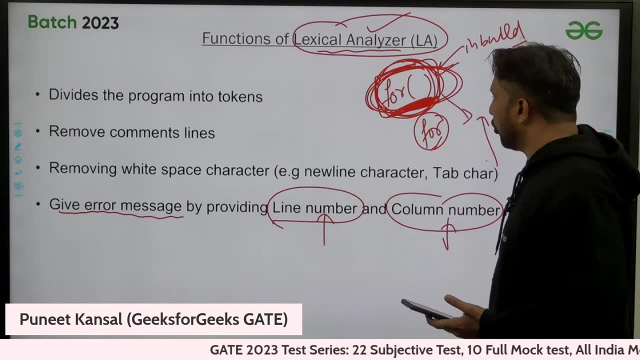 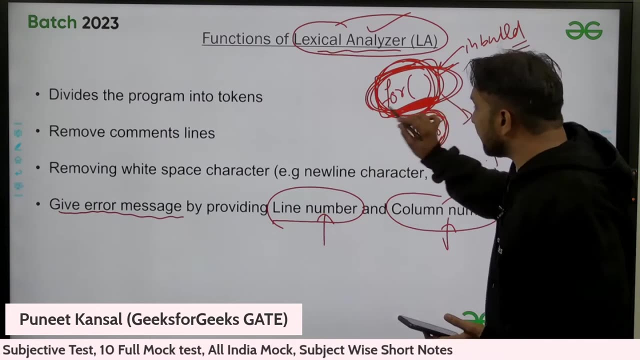 that. Okay. So actually we use this as a as a loop only, But this, this function is helping us to execute the loop. This same function is helping us to execute the loop. Okay, So you, that doesn't mean that. okay, this is a keyword. This is a keyword, What I was trying to. 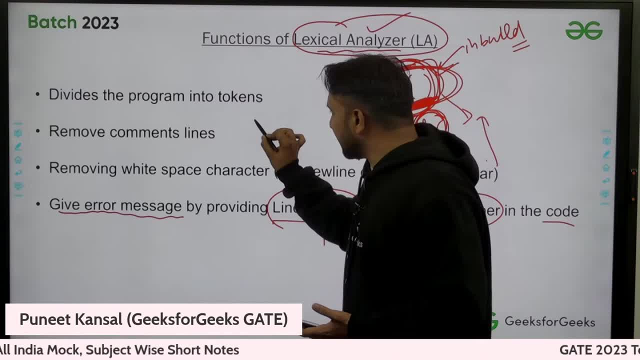 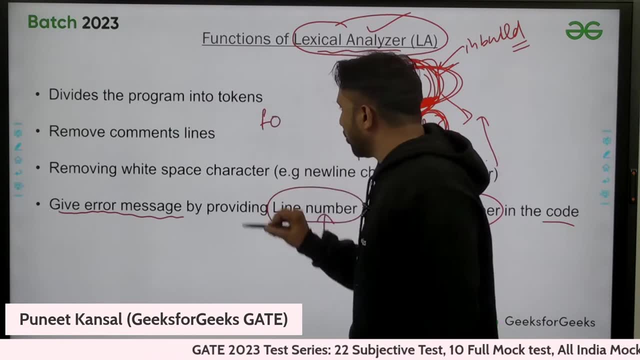 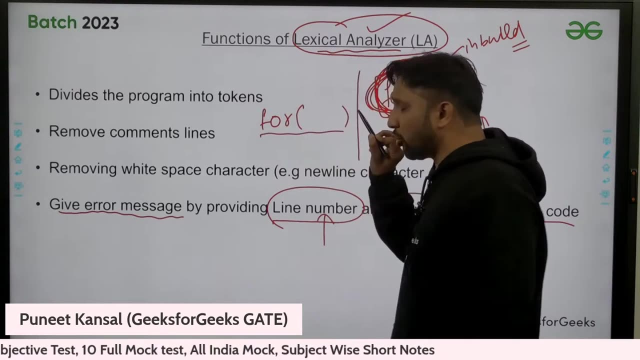 tell you that what I was trying to tell you, that lexical analyzer scan character by character, character by character. Let it F first, then he find out O, then he find out R. Okay, After that, okay, we know, we know this thing, This thing is already known by the compiler. Okay, He also know. 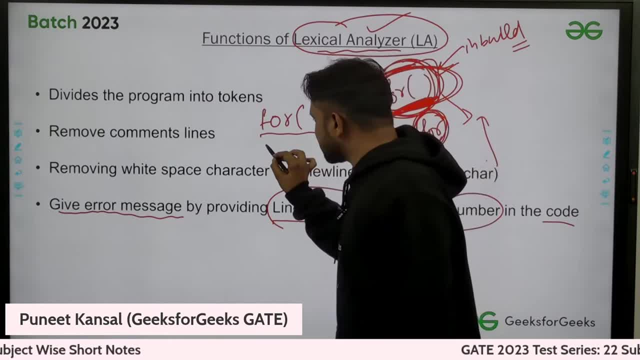 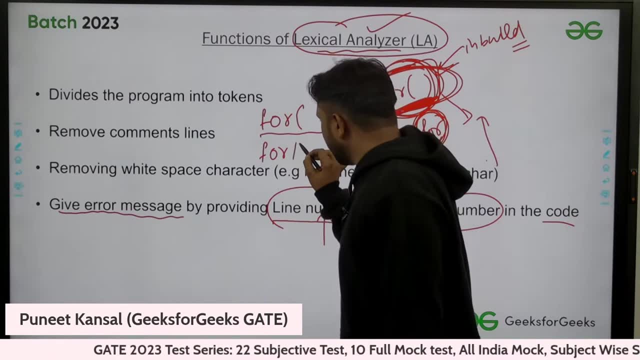 this thing. He, he also know this thing. But if I say that F O R, let's suppose I write, I don't know I can write any word. Let's K. If I write K here, and there's a space here, there's a space after this. 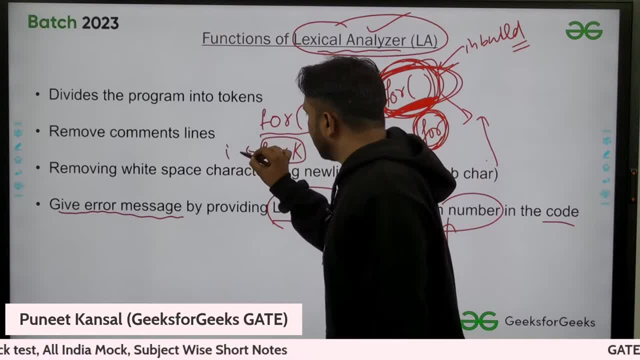 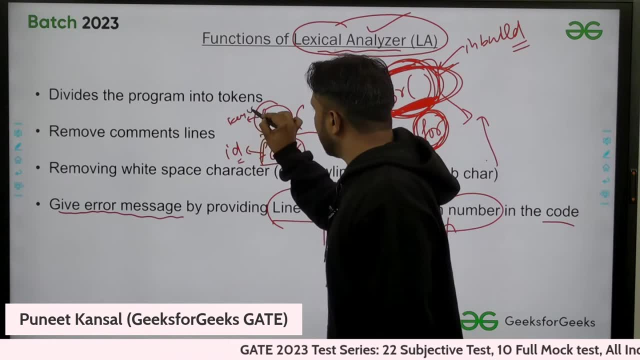 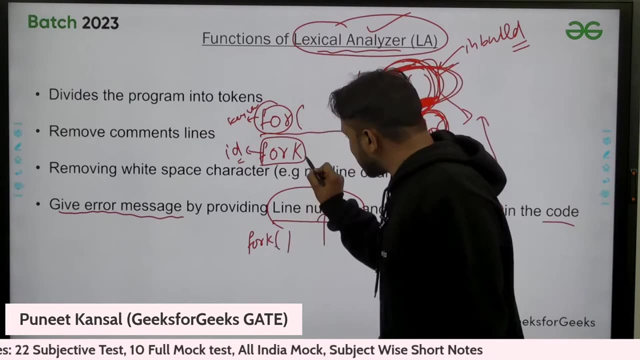 then this will be considered as an identifier. This will be considered as an identifier, And this will be considered as an keyword. And if I'm writing, if I'm writing F O R K brackets also, there is no space after this. there is no space. This is considered. 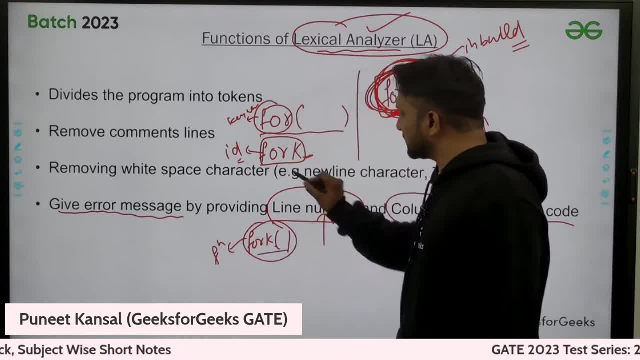 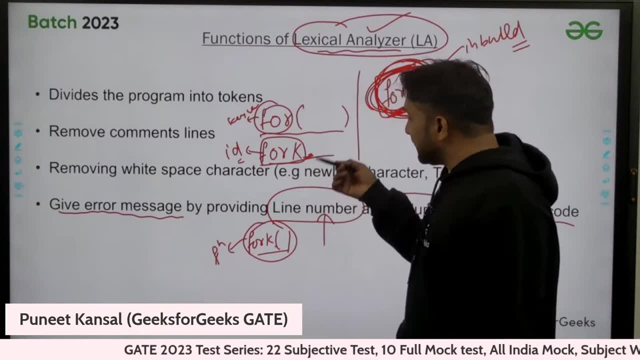 there's a function. We know this thing. This is a function, This is a variable, If there is a space out of this. So how the lexical analyzer is identifying his VFA, his finite automata, is finding out. okay, if there is a space, then this will be considered as identifier. Otherwise, 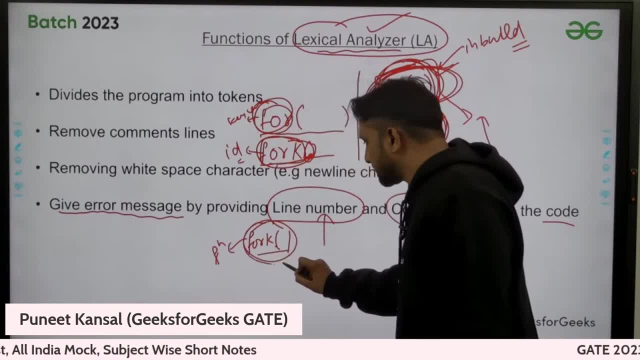 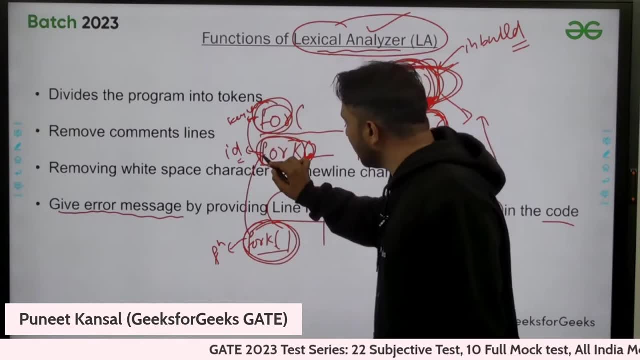 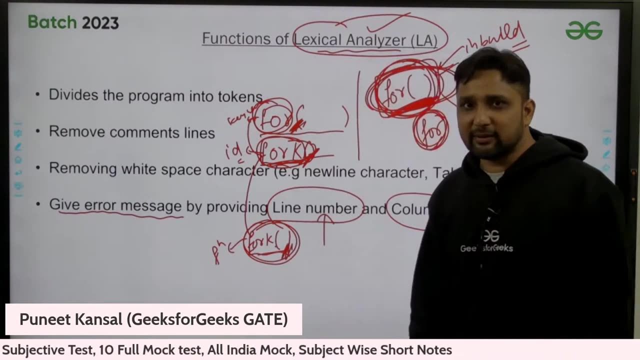 this is considered as a keyword. Otherwise, this will be considered as a function. Okay, So this is what I'm trying to tell you, that okay, How, how that is differentiating between keyword variable and the function. So this space is actually helping. There's a question also in in in GATE exam related to this itself. 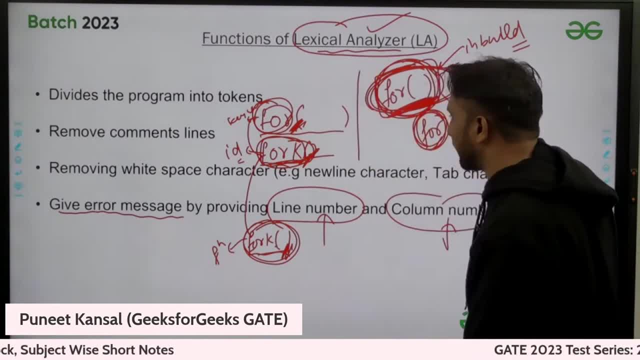 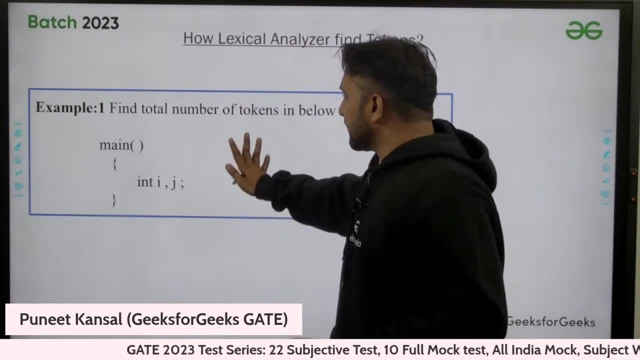 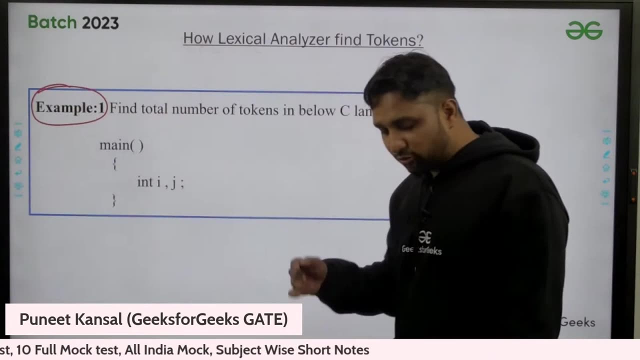 more clarity will come from there. Okay, If any doubt, still you can ask, please. Anyone any doubt? please ask. Otherwise, now we are taking some examples. We are third part of our session Here. we are going to take the examples. After these examples, we will cover the GATE. 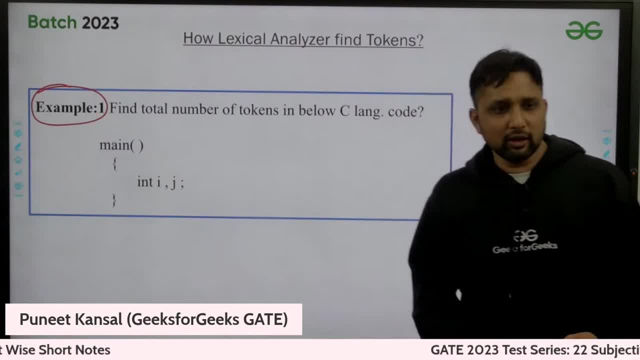 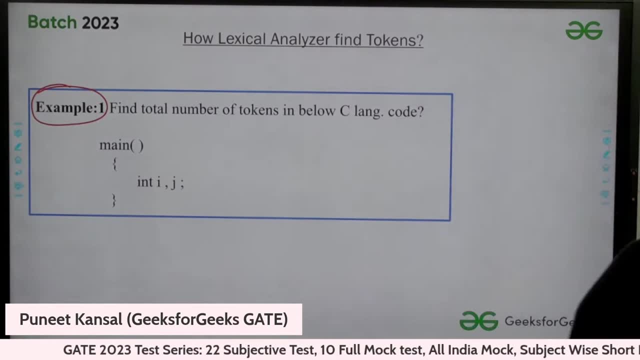 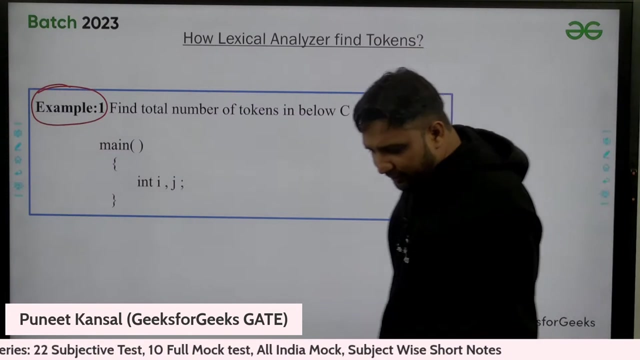 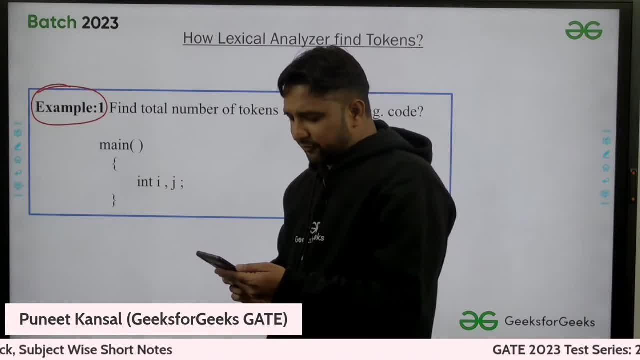 we get, we get the answer. Okay, We can't get the answer. Okay, We get the answer. We can't get the answer. Okay, Okay, get. Kavya says 10, Sriharsha says 10, you people are right actually, so don't worry. 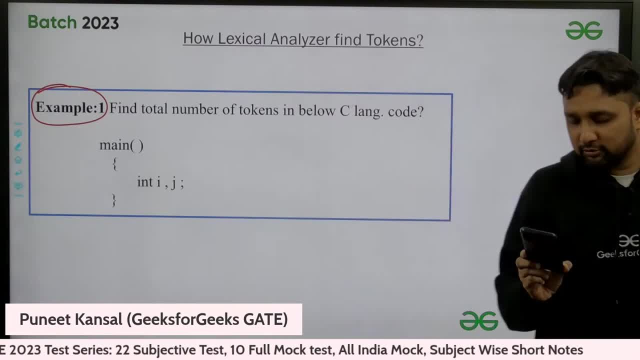 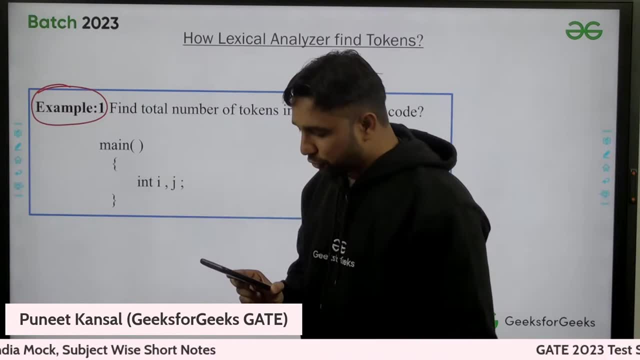 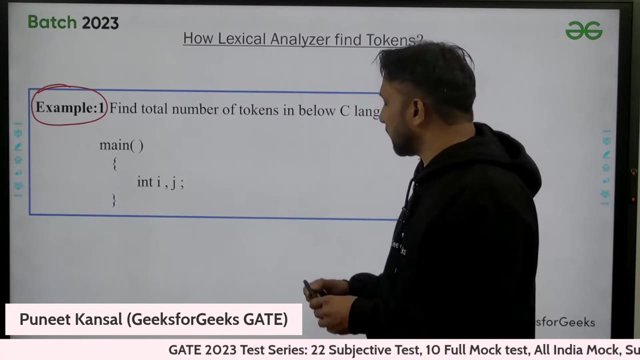 I am going to give you some more tough questions also. I will not leave you. if you are already prepared, then also. we have some other tough questions for you people also, okay, so meanwhile, you people, please keep helping, please keep replying, so that other people can also get. 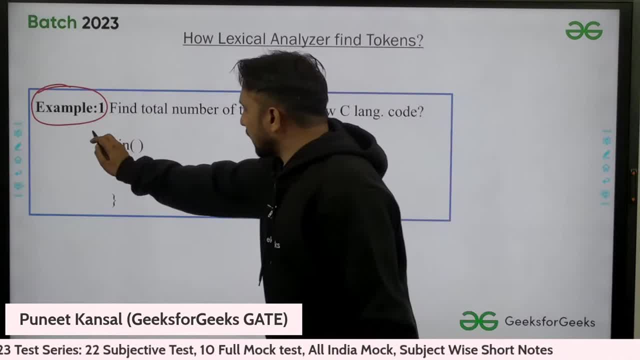 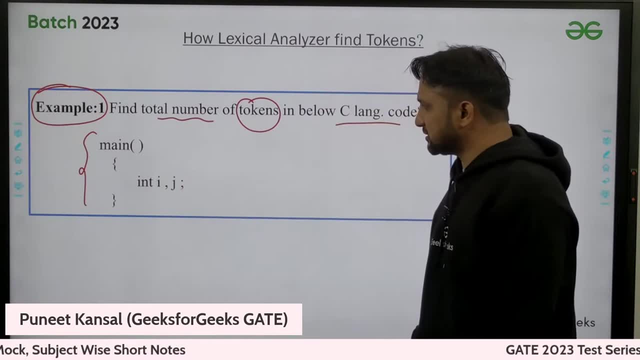 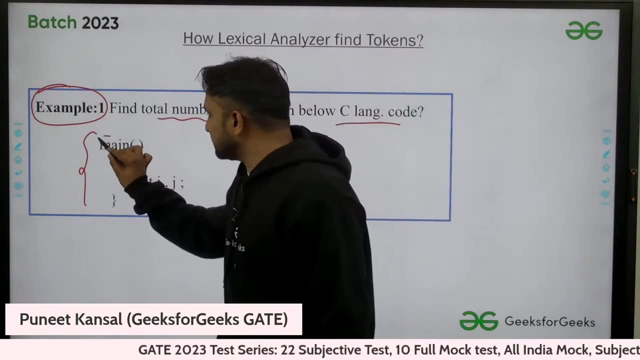 help. so here this is the program we need to find out number of tokens in this C language code, actually number of tokens. so we are already getting 10, 10 is the right answer. actually, how they are finding 10 is C how they are finding 10, this is one token. this 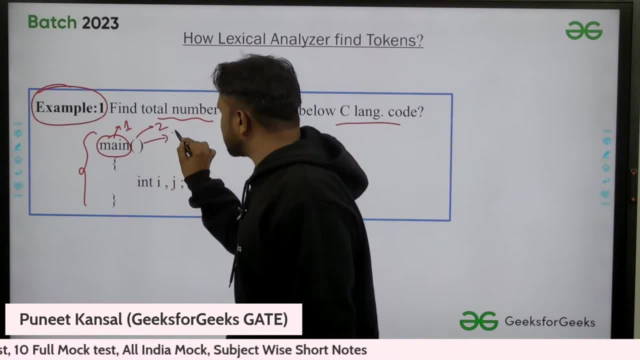 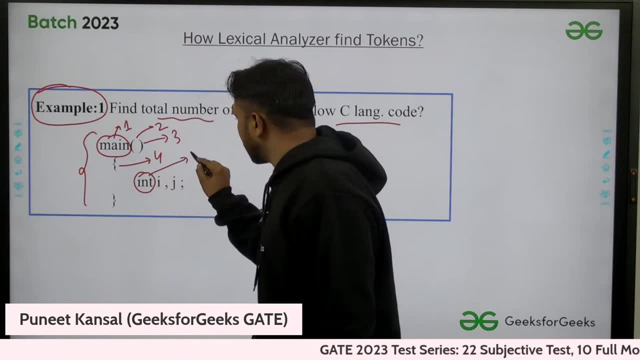 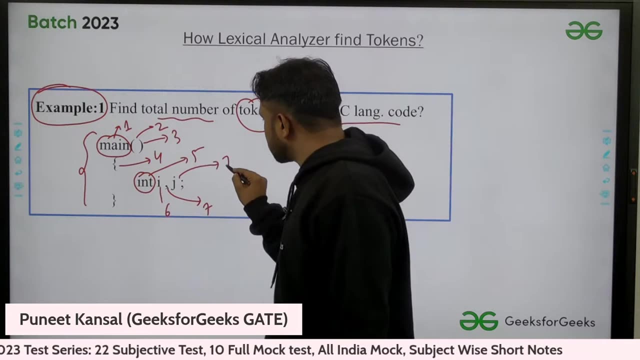 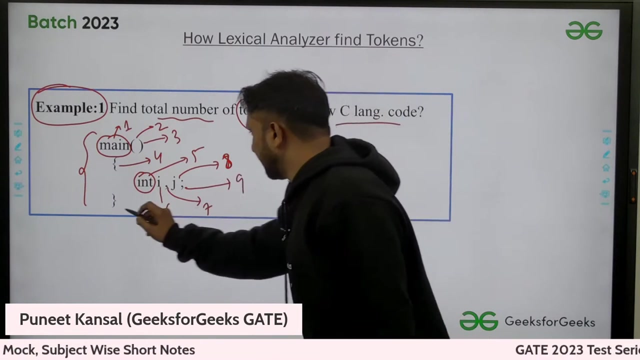 opening bracket is another token. this closing bracket is another token. this curly braces- opening curly braces- is another token. This is this. int is another token. I is another token. comma is another token. J is another token. 6,, 7,, 8,. this semicolon is another token and this is the last one. so total number: 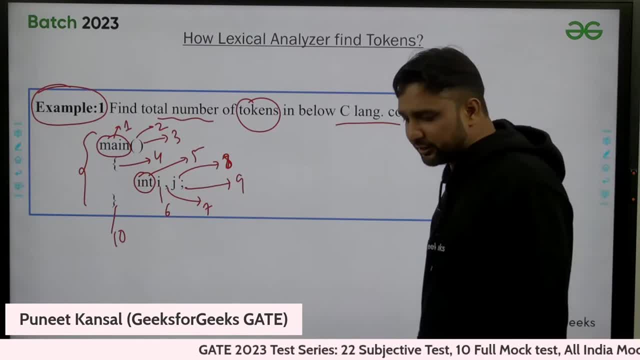 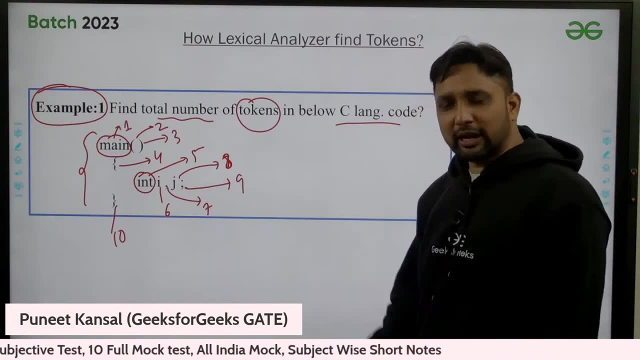 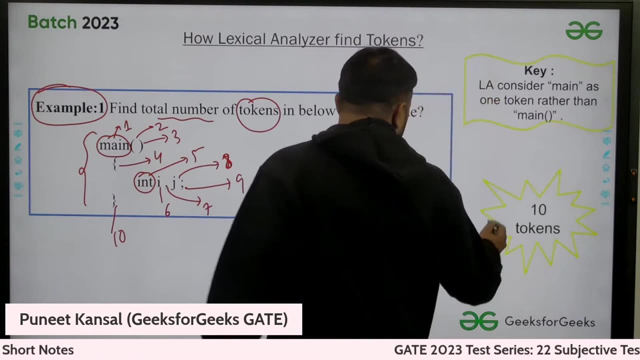 of tokens are 10 here. total number of tokens are 10 here. so any doubt in this? please ask one doubt may be there, one doubt. Let me generate a doubt from my side. so one doubt may be there. token: okay answer is: 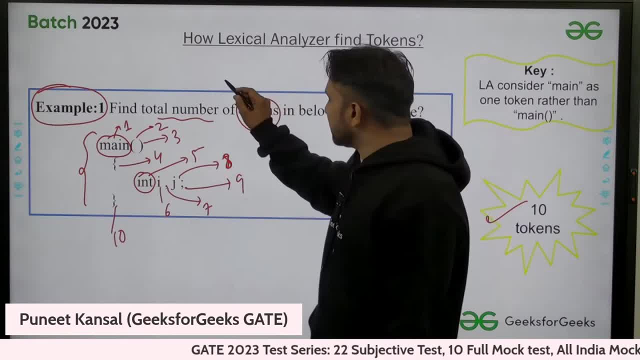 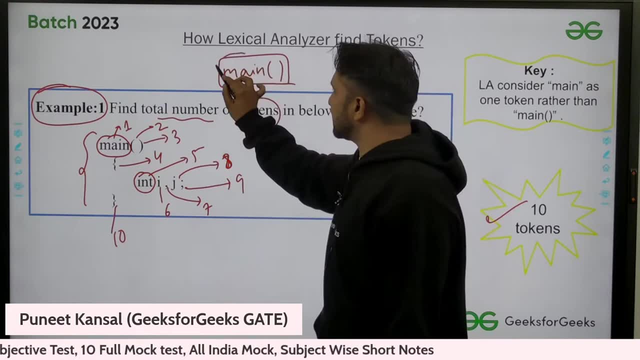 10 right. one doubt may be there. some people, if they are trying first time, they think that, okay, this is one token. this is one token. see, this will be considered as 2 tokens. 2 different tokens- this is main- will be considered as different tokens. this opening bracket. 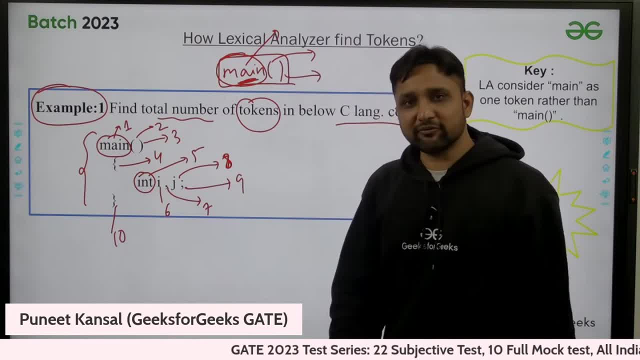 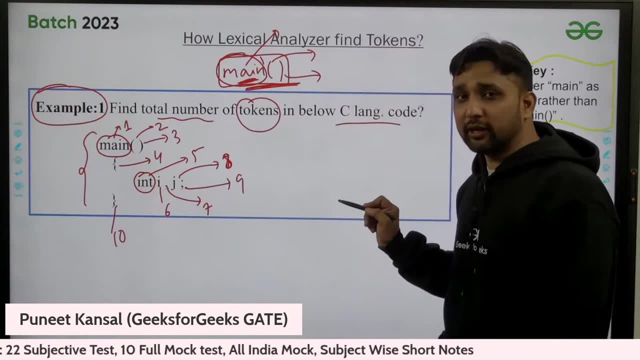 will be considered as different token. this closing bracket will be considered as different token. okay, So if we are defining a function, this is how the tokens will be counted. okay, So why this is counting like this? why this is not considered like this? see, this is not. 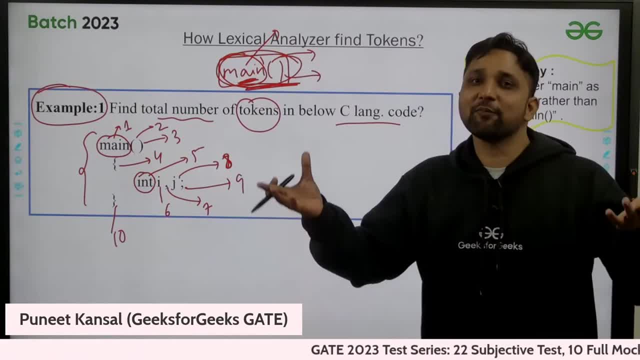 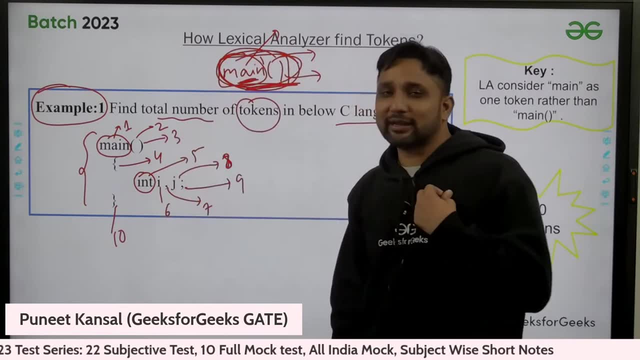 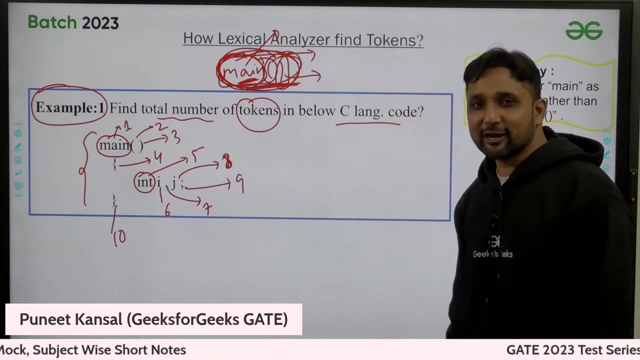 my fault. this is how the compiler is designed. this is how compiler is designed, how they are counting the tokens. okay, If I have generated the compiler, I may make it as one token, but they consider it as one token and opening bracket as another token and closing bracket as another token. okay. 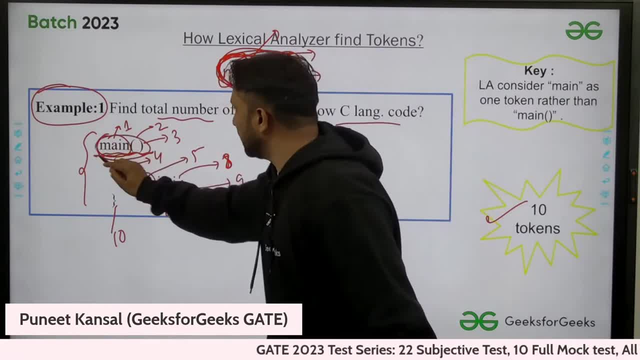 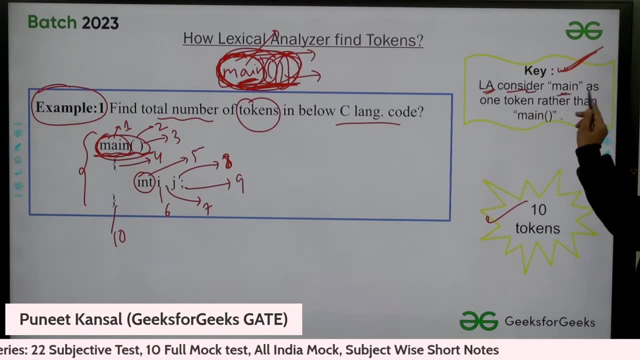 So these are 3 different tokens. this is not one token. this is what we are telling. this is the key which you can take from this program, actually, Lexicon analyzer. consider main as one token rather than this. okay, that, consider function. 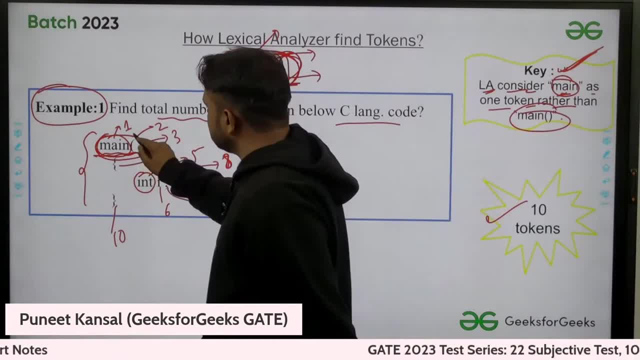 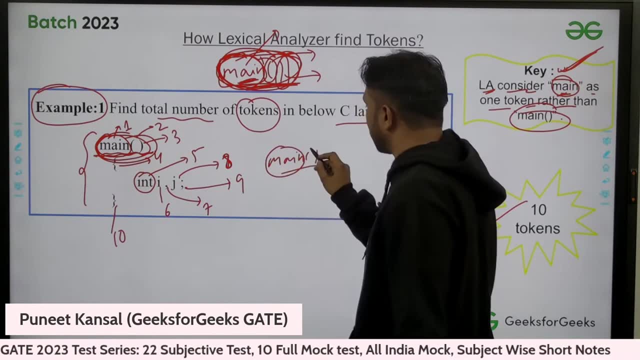 name as a one token, rather than this complete, Although this complete have some meaning. this is a function we know, but still, that is considering. this is one token. this is another token. this is another token. So some, there are some important points. 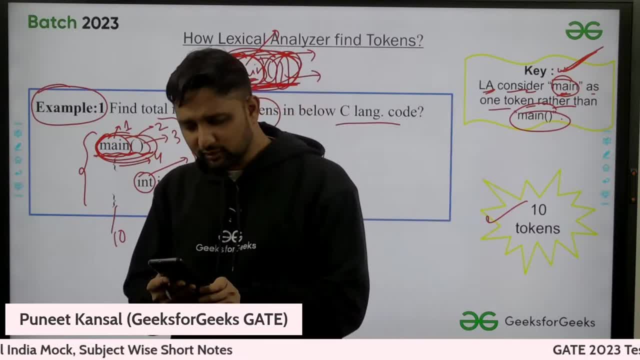 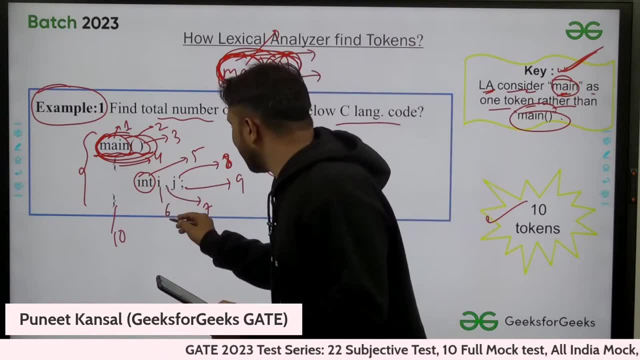 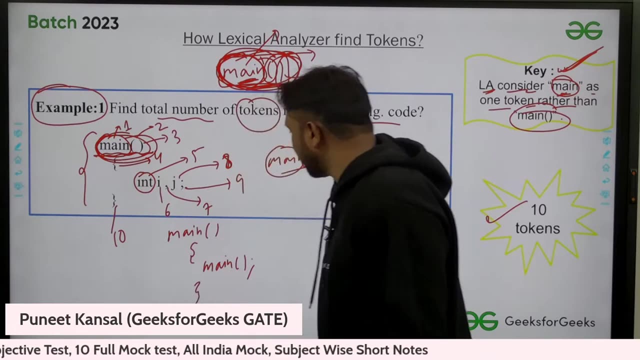 We will cover one by one recursive function call. may kaise karein recursive function call: may kaise karein tokens count. can anybody tell me this is recursive call? okay, please tell me how many tokens are here. you people please tell me. please write in the chat box. 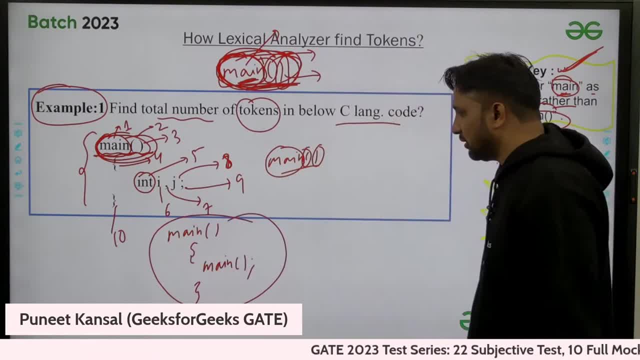 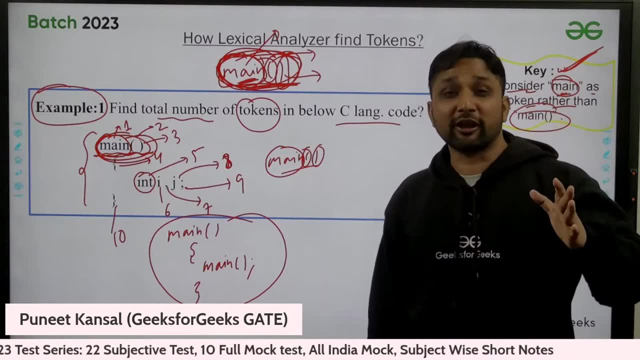 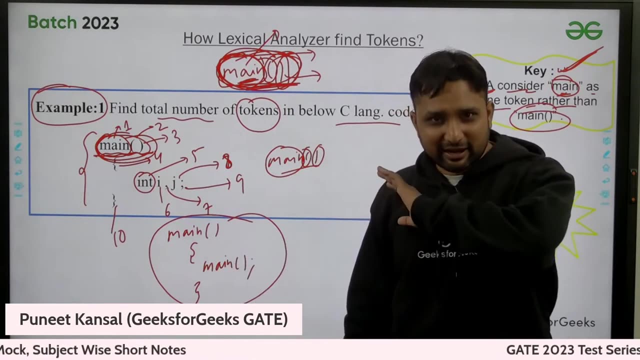 how many tokens are here? this is a recursive call. how many tokens are here? Lexicon analyzer is not worried. Let me take a note down: lexicon analyzer is not worried about what the hell you are doing in the program, whether your program is working fine or not. lexicon analyzer is. 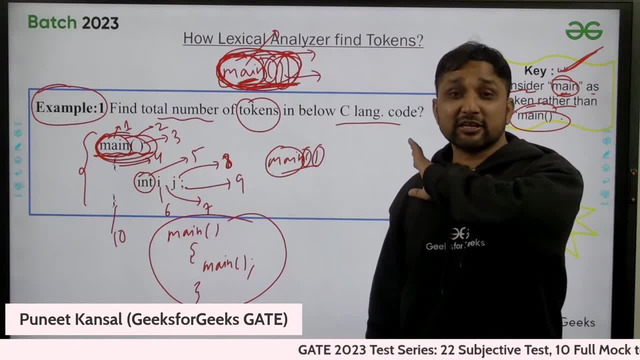 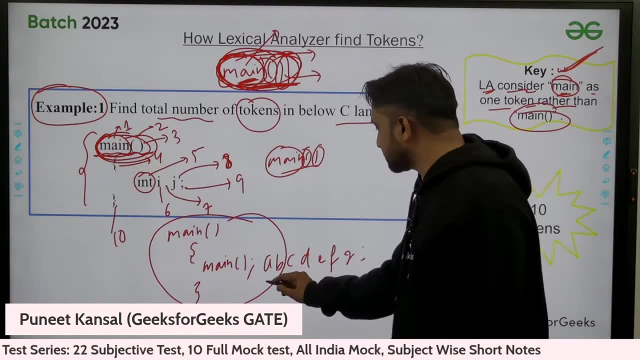 not bothered about the meaning of the program. lexicon analyzer is not bothered about the meaning of the program. If I write, say that A, B, C, D, E, F, G, H unnecessarily, I am writing this thing. Lexicon analyzer, first phase of the compiler. pass this code on. this will send this code. 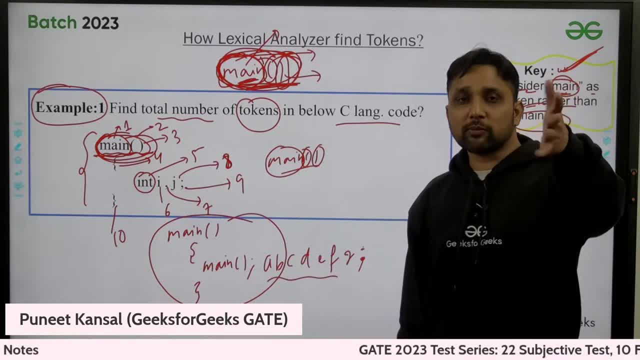 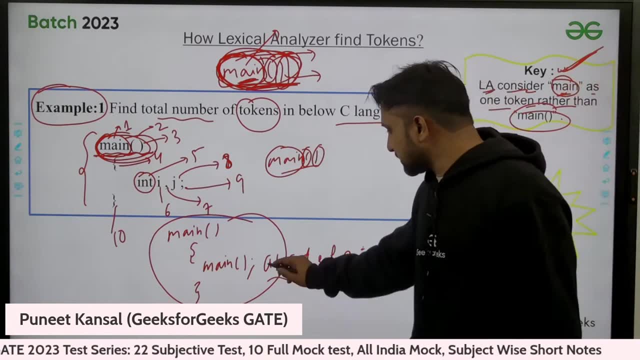 to the second phase of the compiler. That is not. Lexicon analyzer is not bothered about the syntax. who is bothered about the syntax second phase of the compiler, syntax analyzer? okay, So lexicon analyzer is not bothered about, so do not bother about how this program will. 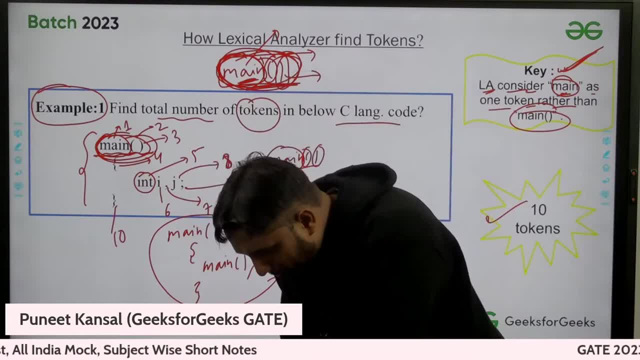 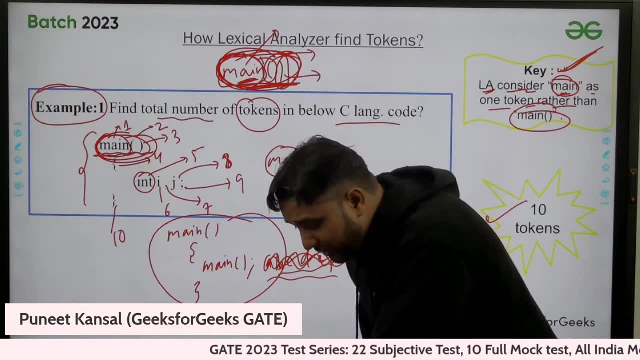 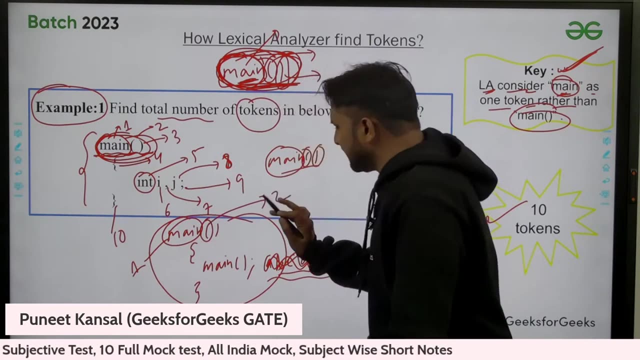 work. just simply tell me how many tokens are here. So sign up saying 9 and Jerry is saying 18,, 18, okay, so let us see 1,, 2,. no one thing is clear In this lecture. everything will be clear. one thing, this thing is clear, if any doubt. 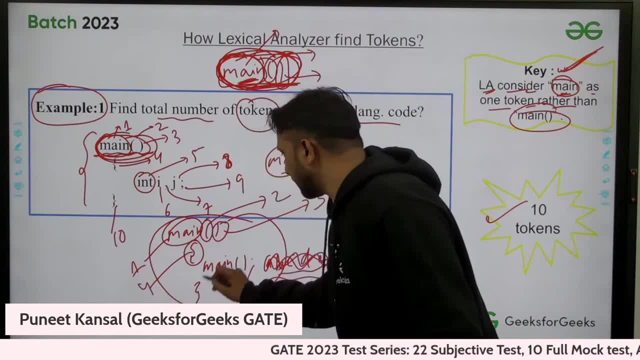 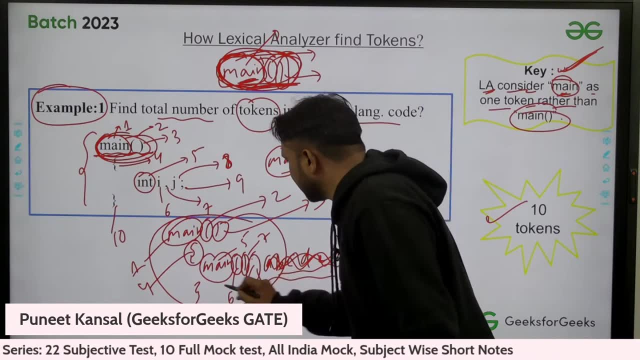 please ask me. you need to ask the doubt. 4th token, 5th token, 6th token, 7th, 8th and 9th. that is it. so these are the 9 tokens we have. 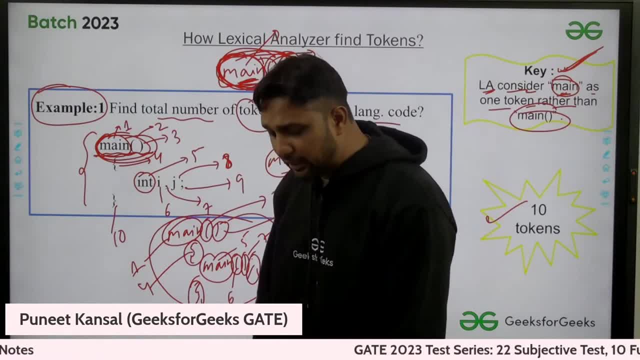 Keep asking the question. if you have any doubt, please keep asking the question. keep replying if you are replying the answer. if you already know the answer, please help other people. if you have any doubt, please keep asking the question. keep replying if you are replying. 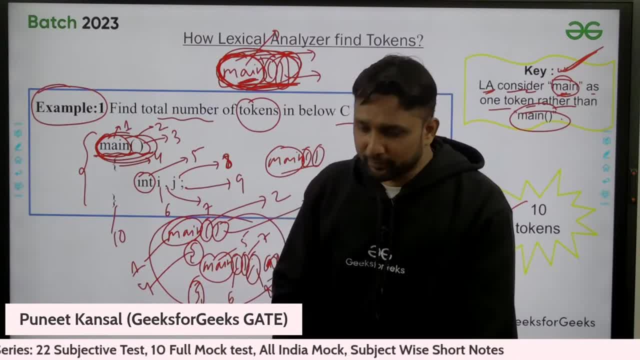 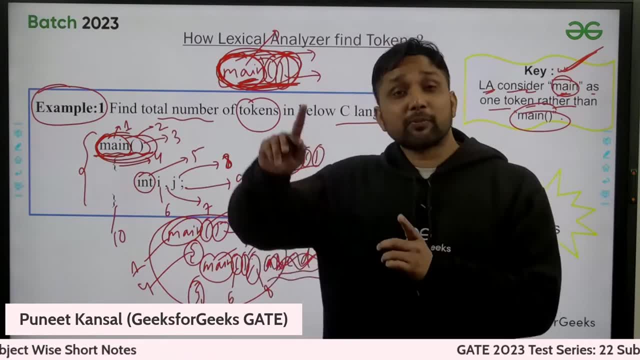 if you will reply, other people also will get benefit from that, okay, so please keep replying also and if you have any doubt, please ask the question because, you believe me, other people also have that. many people also. other people have same doubt, but they are. 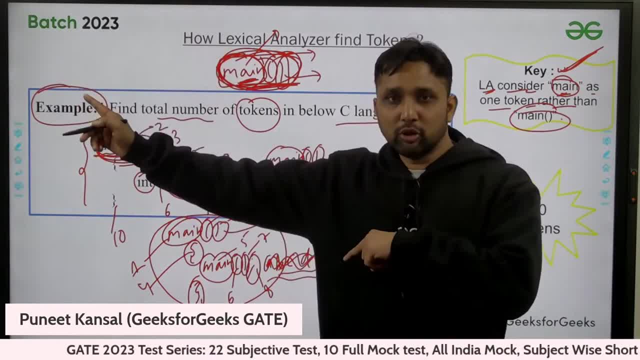 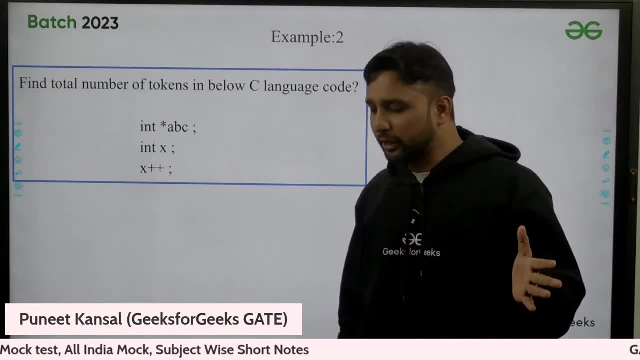 not asking. if you are asking, you are helping other people also. both way you are helping. if you are writing the answer, you are helping. if you are writing the doubt, again you are helping. okay, so another question, please, please, tell me how many tokens are here, please? 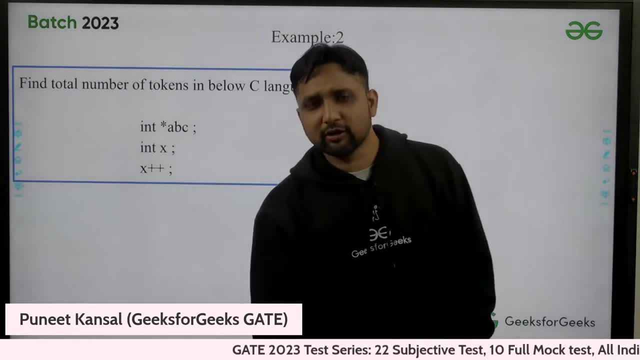 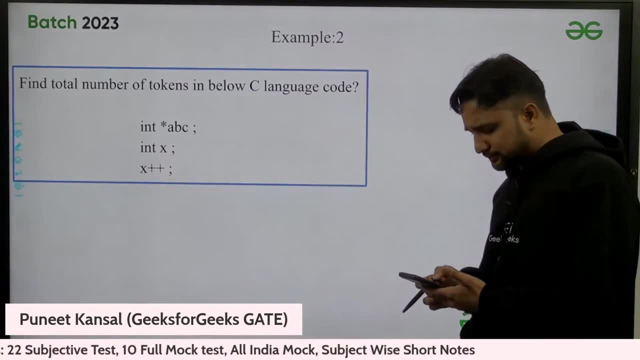 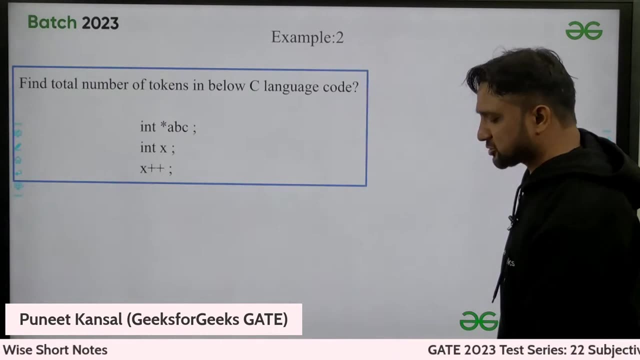 tell me How many tokens are here. try to count. even you are trying it first time. please make a try, give a try. please find out how many tokens are there in this code. find out, please. We will finish this topic. we will not left anything and they cannot ask out of the out. 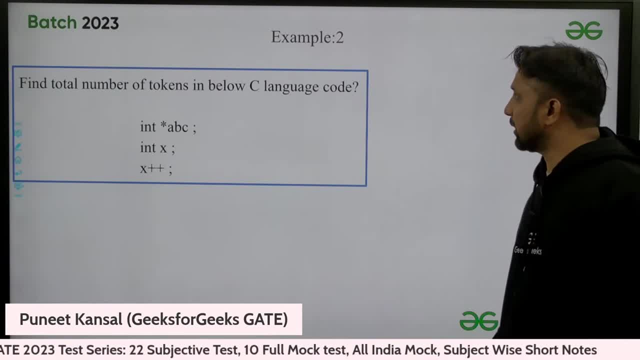 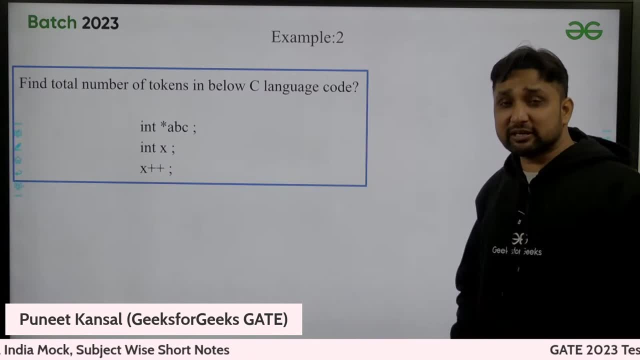 of the concepts. actually, we will cover each and everything from this concept and this is one of the most important one. We have lots of great questions from this topic. We will cover right now and you will see that they are asking the question from here. 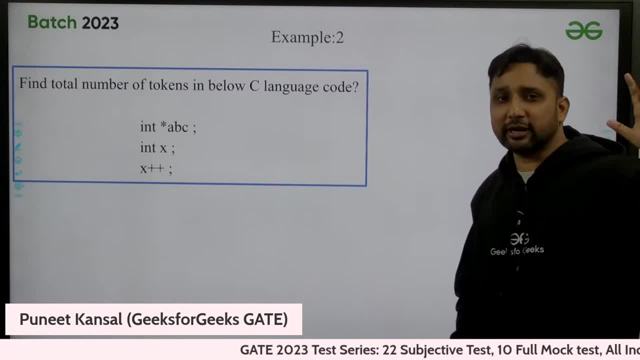 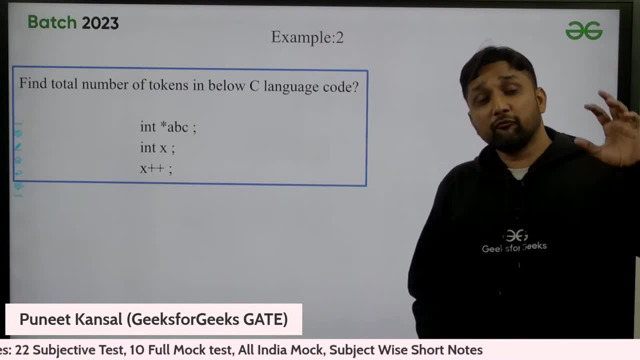 We are covering 5 most important topics in compiler in every subject. Why we are covering 5 only? why we are not covering 10 or 15 or 20? because we one thing is, we have selected. out of 20, we have, we come to 10, then out of 10, we come to 5, and 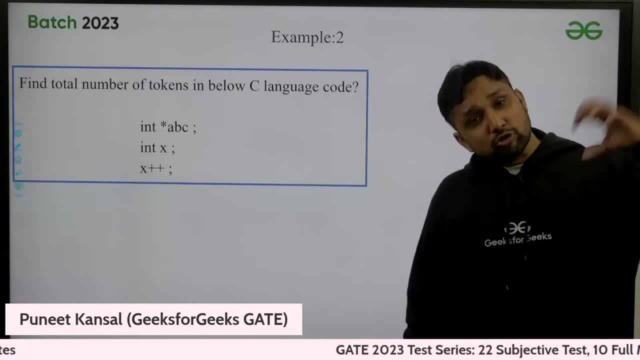 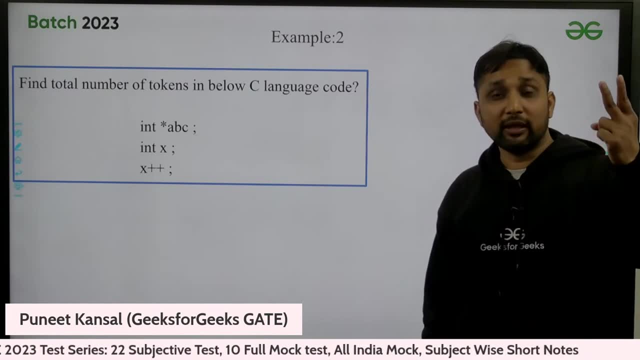 these are 4, those 5 topics. from everywhere, question everywhere, question is coming on, so maybe they can skip 1 topic, 2 topic, 3 topic. Now we have 2 topics out of 5, if 2 questions are coming from these 5 topics, I think you. 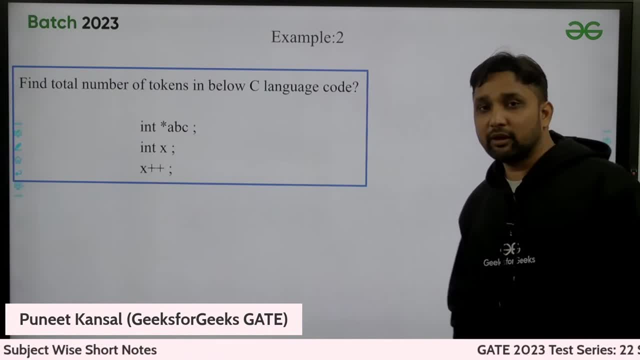 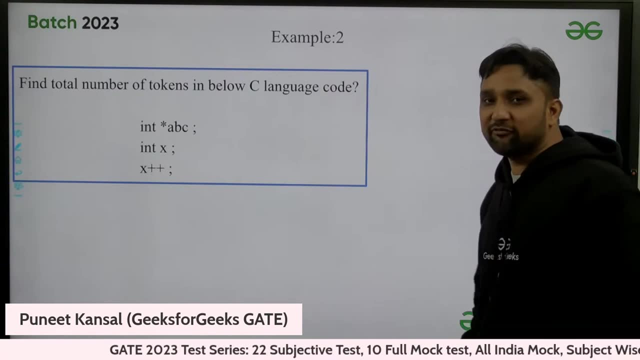 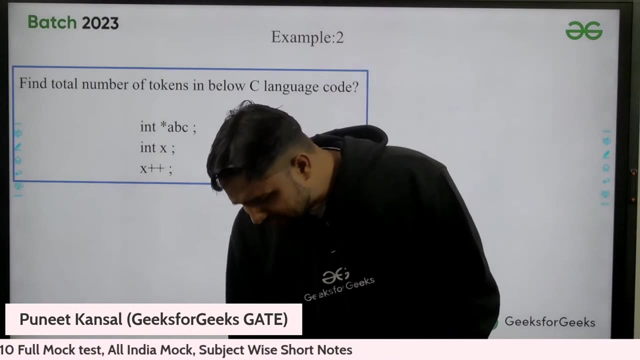 can easily clear the gate gate exam. If you get benefit after gate exam, please come back and write, write in the comment section. you get benefited. That will be the fee of this lecture, actually of these all series actually. So we get answer that is 12, so let us try to find out. 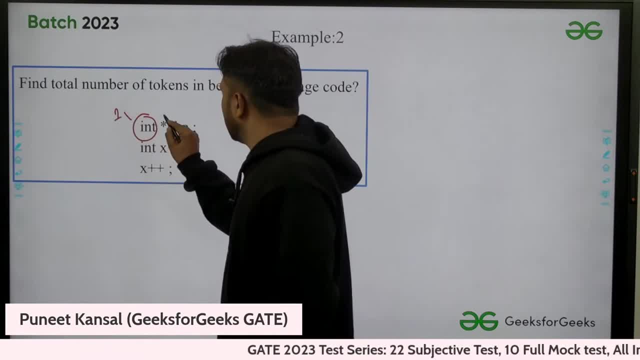 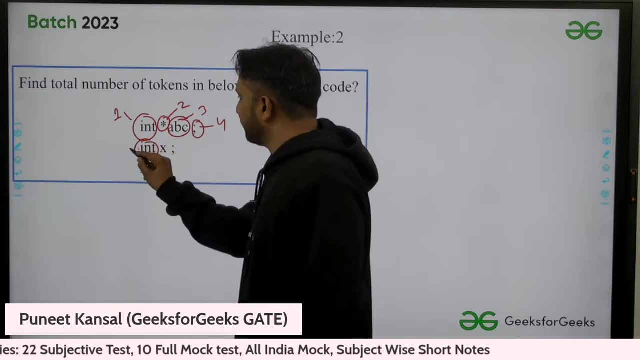 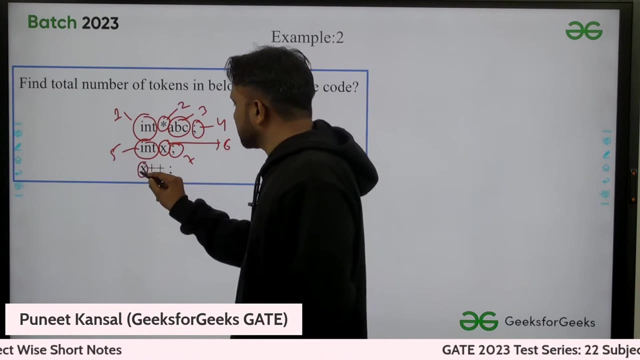 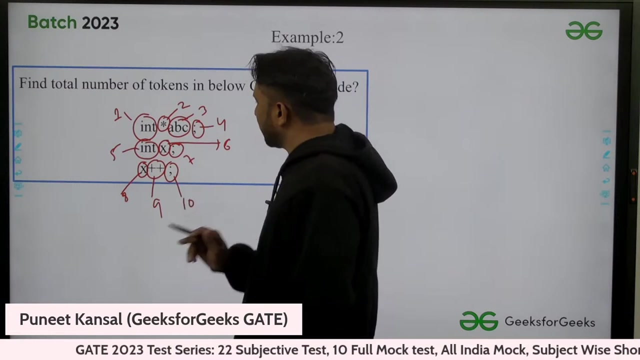 1 token, 1 token 2, 3,, 4,, 5,, 6,, 7,, 8,, 9, 10,. all doubts will be clear, do not worry. all doubts will be clear here. so let us check out if I am right or wrong. yes, there are 10, 10. 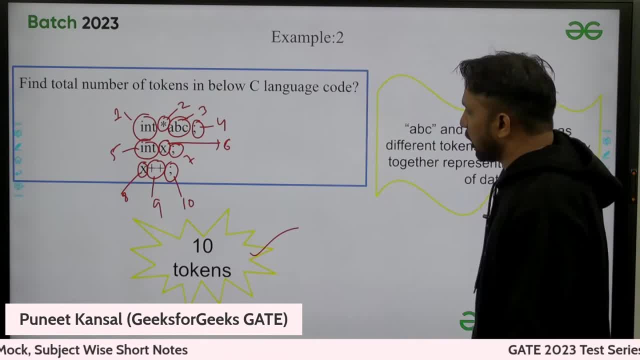 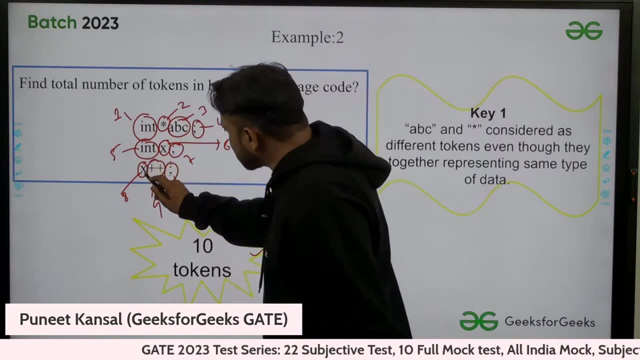 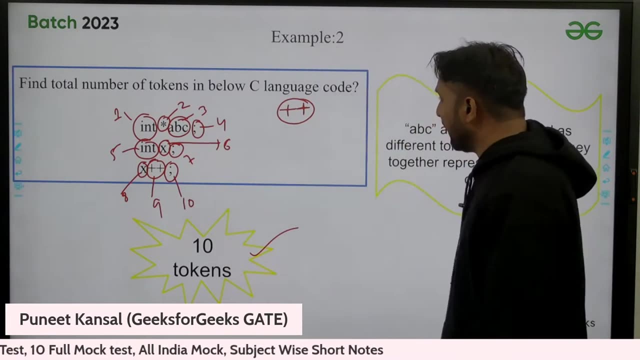 tokens only. So how I am counting here. now you may have 1 doubt. 1 doubt can be like that: ok, why I consider plus plus, plus plus as 1 token, plus plus as 1 token. ok, why I am. I do not. 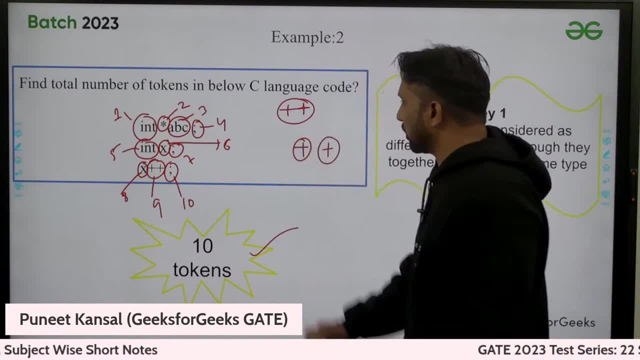 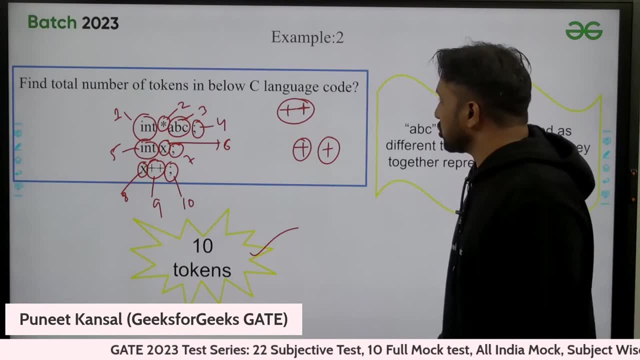 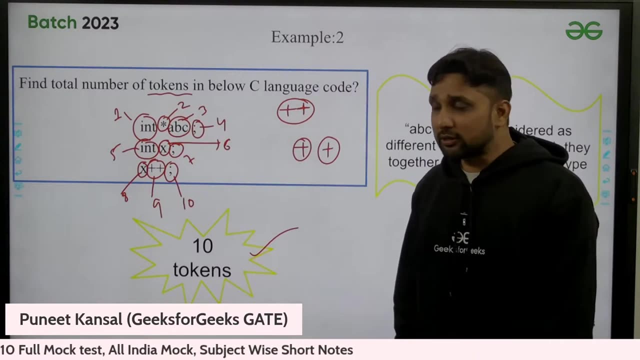 consider 1 plus as 1 token, another plus as another token. ok, why not like that? one question can be this: this, which I think can be asked here, So you can note down one important line While finding the tokens- actually, while finding the tokens- your lexical analyzer. 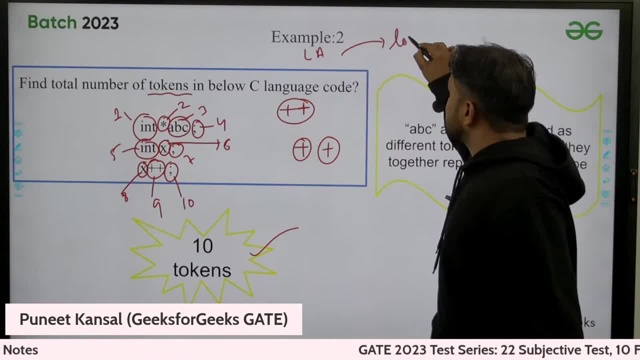 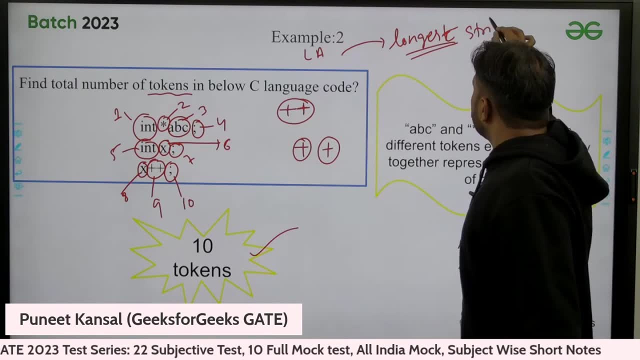 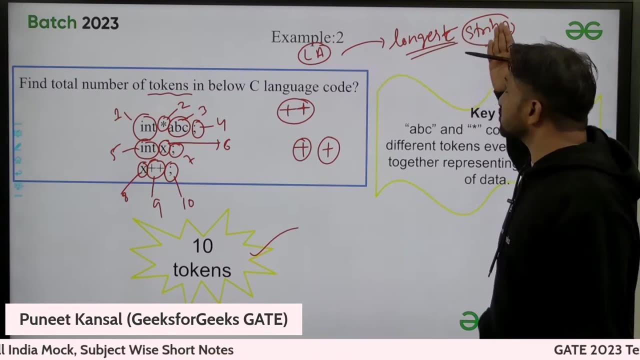 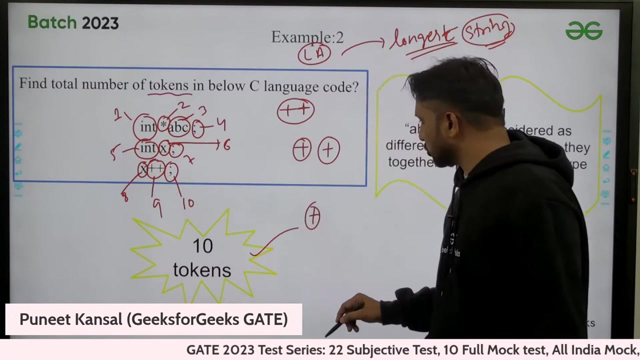 will try to find out the longest, longest, longest string. he will try to find out this person. this lexical analyzer will try to find out the longest string which he knows actually. ok, For example, He knows, He knows plus, definitely he knows plus also, but he knows plus plus also. so to whom he? 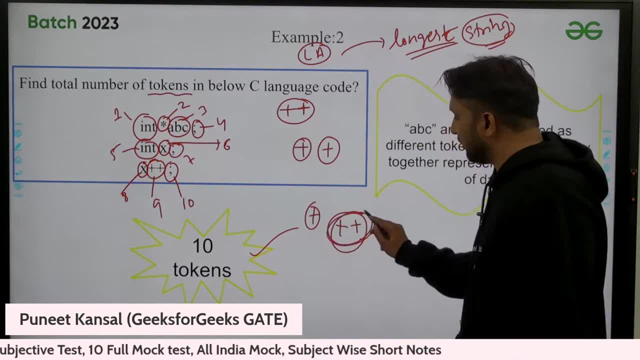 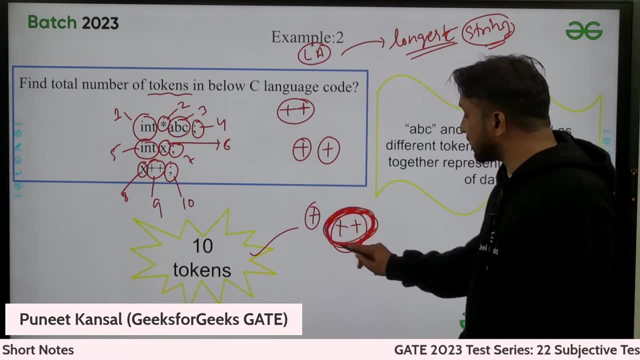 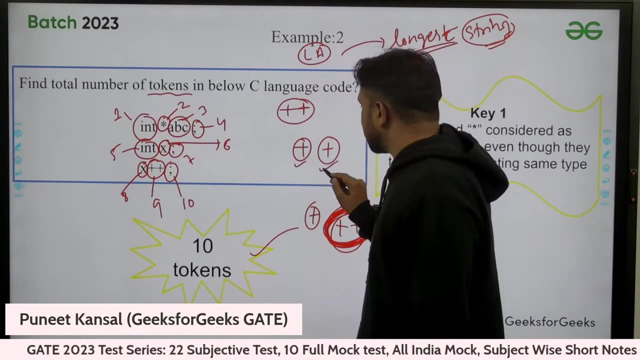 will recognize. he will recognize the longest string. he will recognize the longest string as a as a token. ok, that will recognize the longest string as a token, longest string. so plus plus will be recognized as the 1 token rather than single plus rather than 2 tokens. 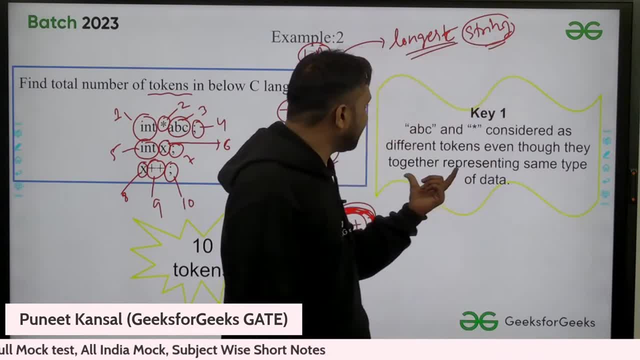 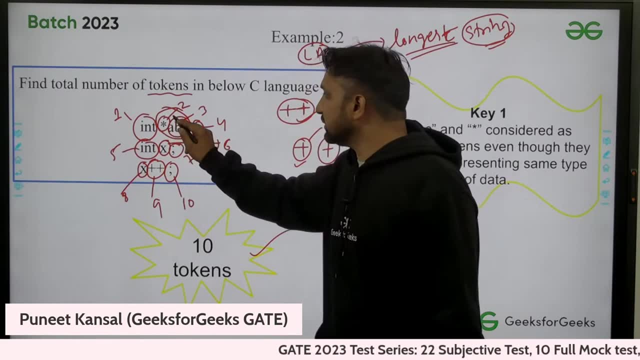 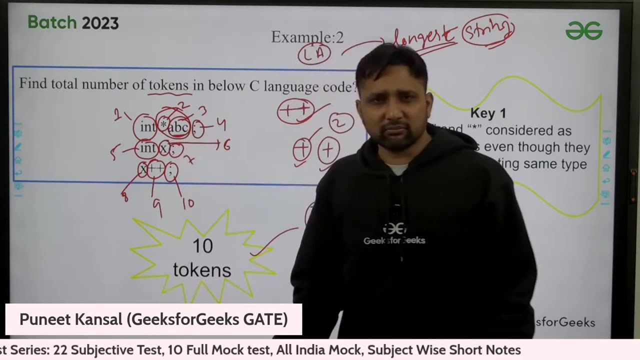 this will be recognized as a 1 token. so these are. same thing is written here. one more thing actually written here. another doubt can be. another doubt can be why I consider these are 2 tokens here. if you are actually, we know that abc is a pointer. abc is a pointer. 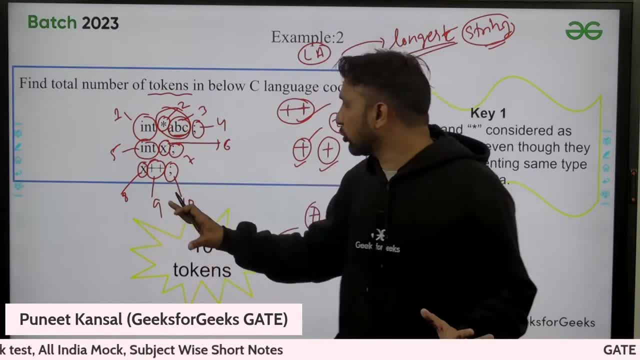 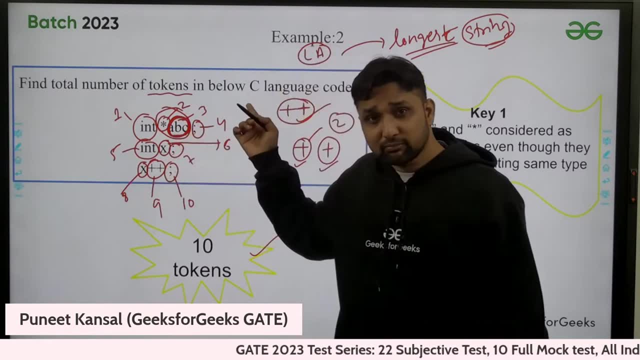 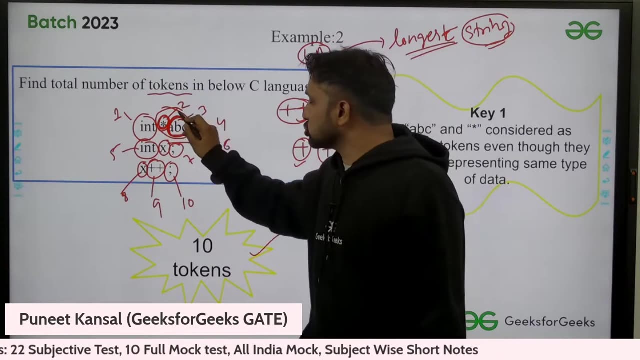 ok, but this is how compiler is finding out ok. compiler is finding out ok. abc is taking. he is taking the name of the pointer as a different, different token and this star as a, this star as a pointer. So this will be considered as a different token. again, the same question may be asked. 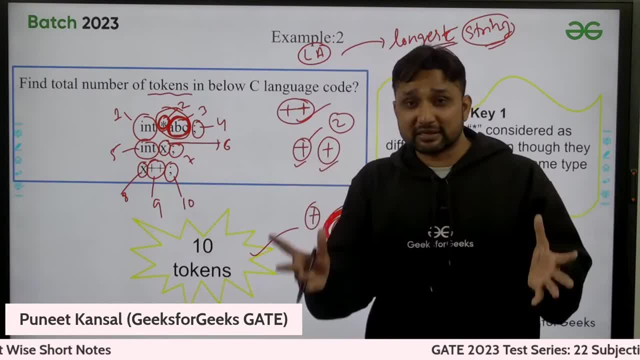 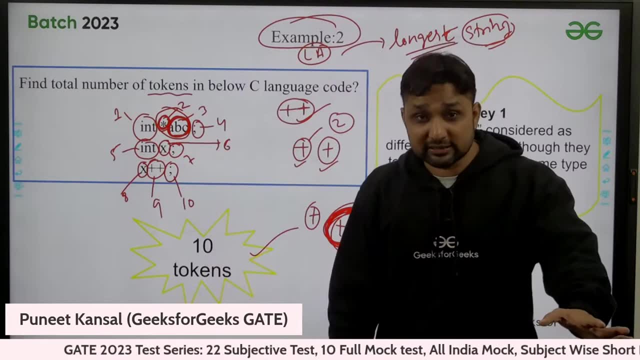 ok, why that is doing like that. this is how the compiler is designed. there are some unique cases which I am trying to cover with the help of these examples. I will cover all the cases. you will be left with no other cases. I will cover all the cases which are the exceptions. 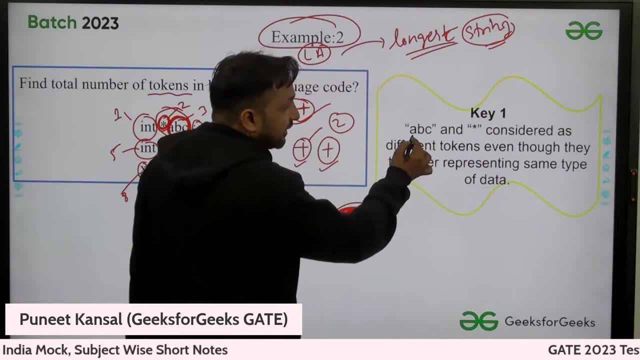 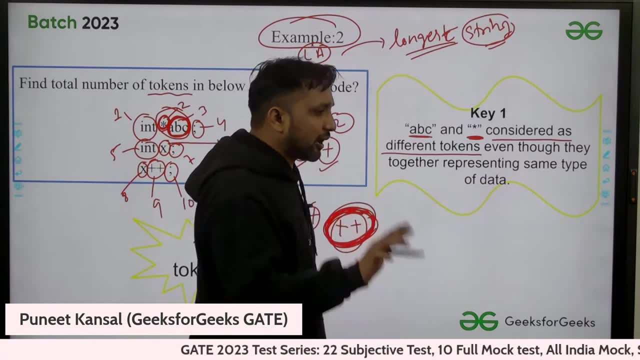 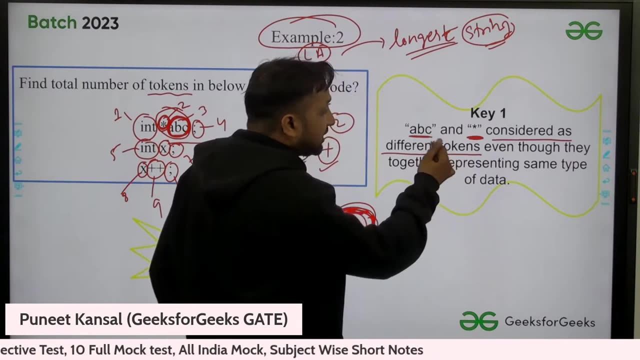 I am covering. that's why I am writing here keys. so here what is written there. here, abc and star are considered as different tokens. This is how your compiler is behaving. we are talking in the context of C compiler, which is your BTEC syllabus. actually, in BTEC syllabus we discussed about the C compiler, only that. 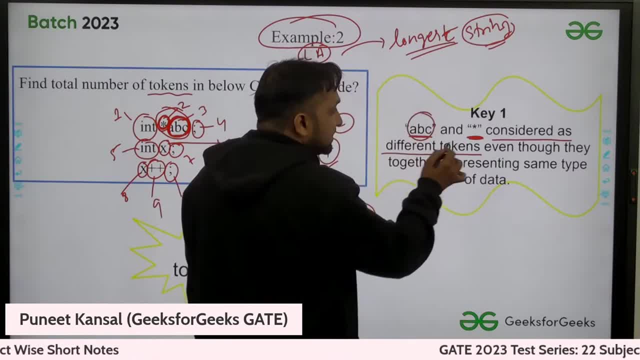 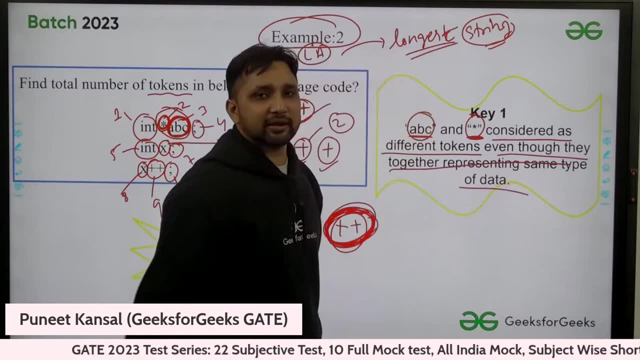 is given in the Ullman book. so here abc and star are considered as different tokens, even though they together represent the same data data type. they are together, they are together representing. what they are together representing is a. their. abc is a pointer, ok, but compiler. 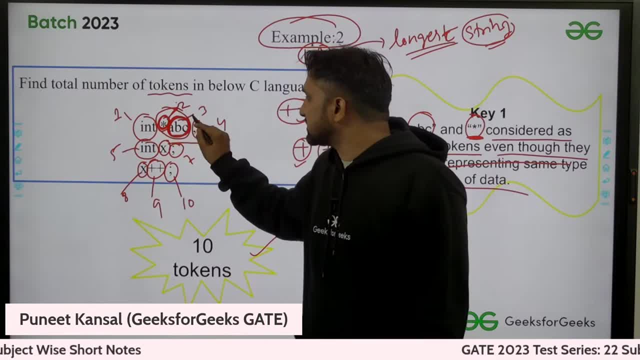 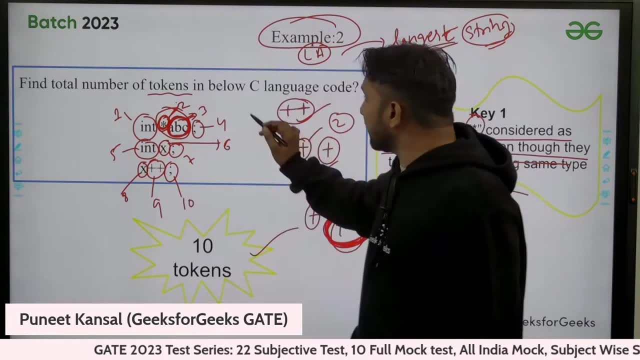 ok, The compiler consider this as different token, this as different token. we cannot fight with the compiler. this is how the compiler is designed. C compiler is designed similar way we done in the previous example. also this is considered as different token. this: 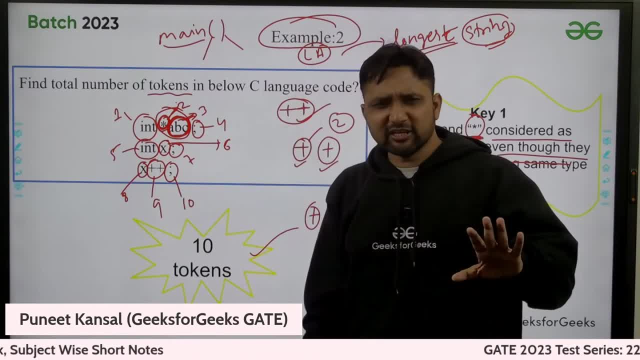 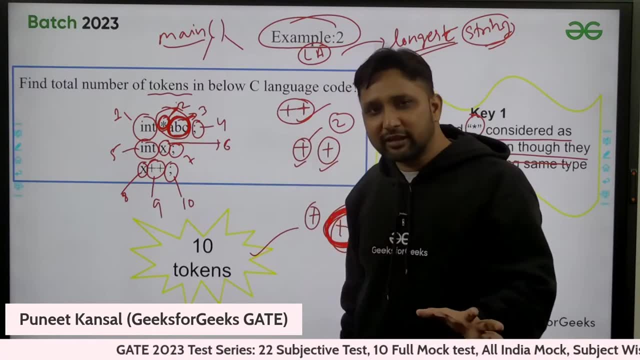 is considered as different token. this is considered as different token. One thing is sure: we will cover all the different this type of concepts. ok, we will cover every. all these keys, All these keys we will cover with the help of these examples. 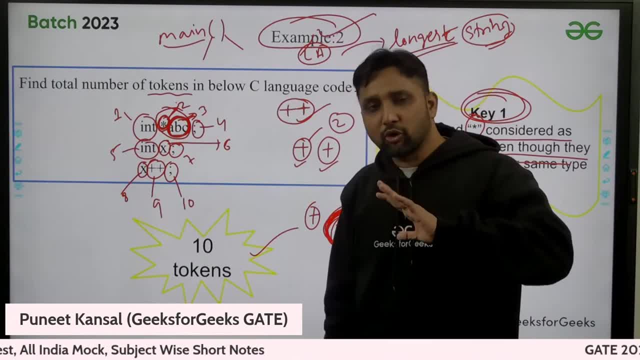 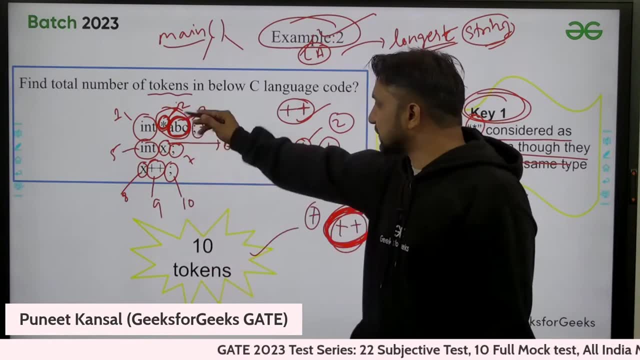 You will be left with nothing, So do not need to worry about that. So you will be able to solve the questions. every question, Okay, Because we will cover all the concepts. These exceptions will be covered. So let me check out. 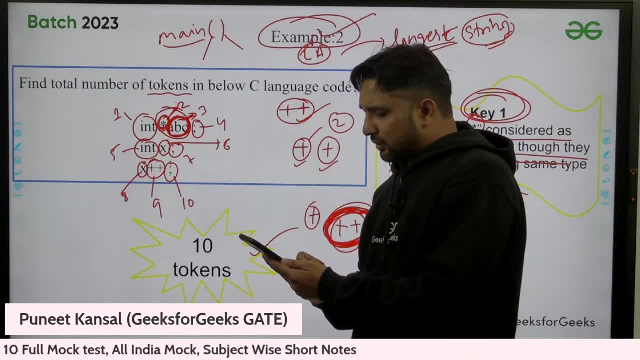 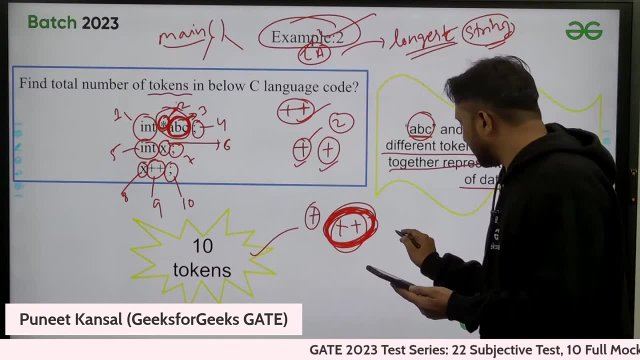 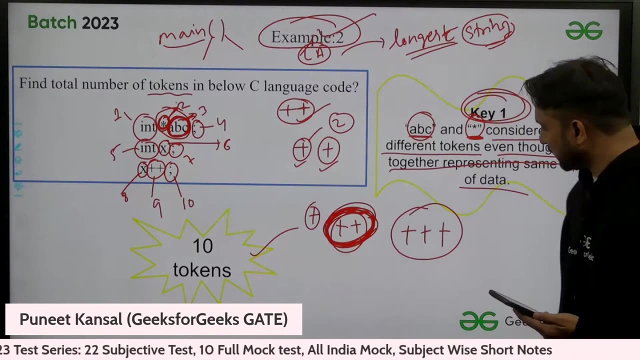 Plus plus. Okay, You are asking, Harsha is asking, Harsha is asking If we have plus plus plus. If we have this thing, then see, We are starting from left, Starting from left, Finding out the longest operator. 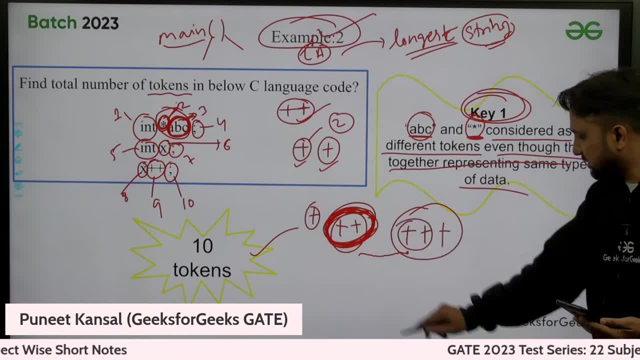 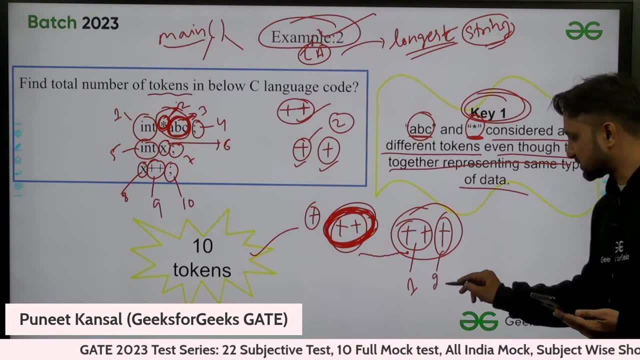 Longest operator, Which is the longest operator Plus plus, This is the longest operator. This will be considered as one token, And then we are left with one plus. This is considered as second token. Okay, So we have two tokens in this. 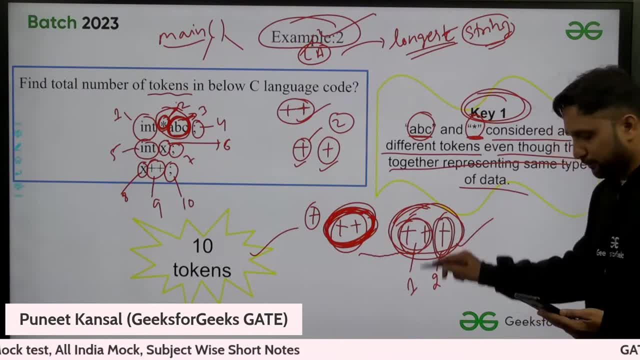 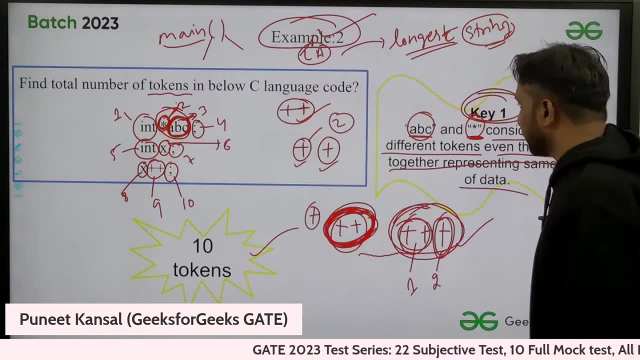 We have two tokens in this. One is this, One is this. Please ask the question. Please ask the question. You are clearing not only your doubt, but many other people's doubt. Okay, So we have lots of examples, Don't worry. 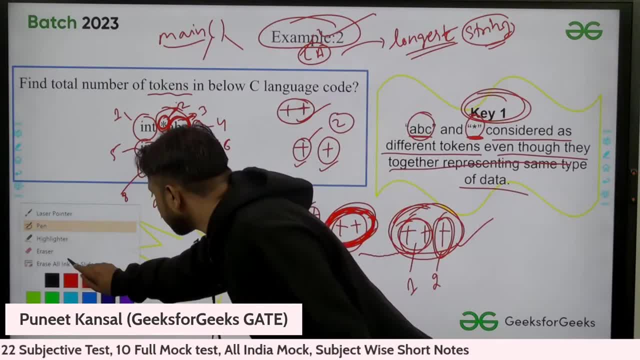 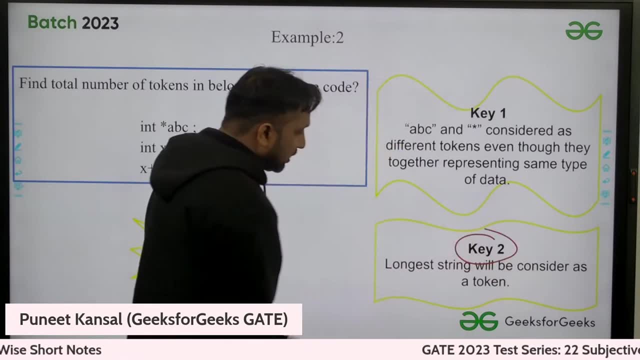 We have lots of examples also. So before moving on, I think there is another point also here. Yes, there is another key which we already discussed. That's why I write it here. Longest string will be considered as the token. 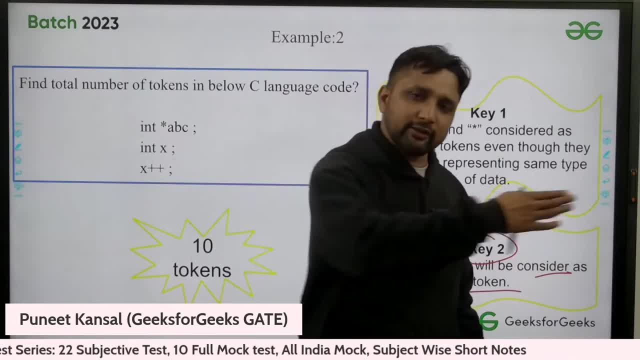 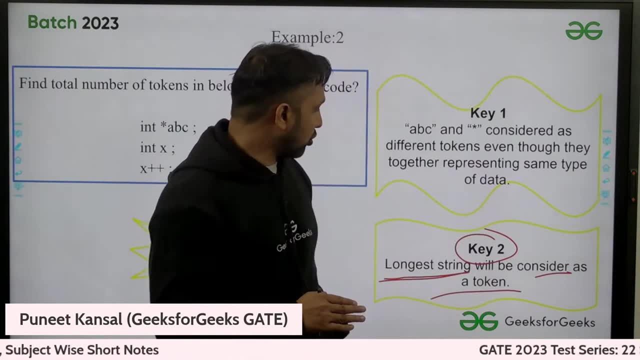 Longest string will be considered as the token. You are moving from here, You are moving from left to right and whichever the longest operator you are finding, that will be considered as a token. That will be considered as a token. Okay, Longest string will be considered as a token. 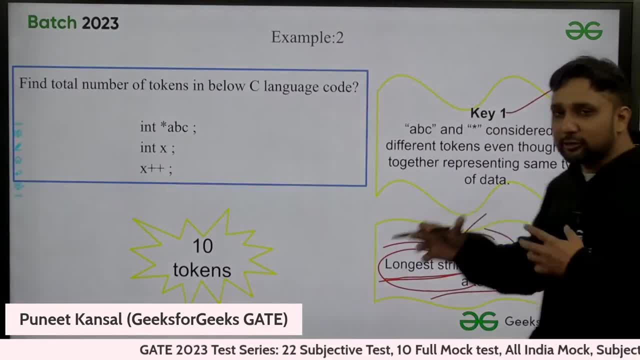 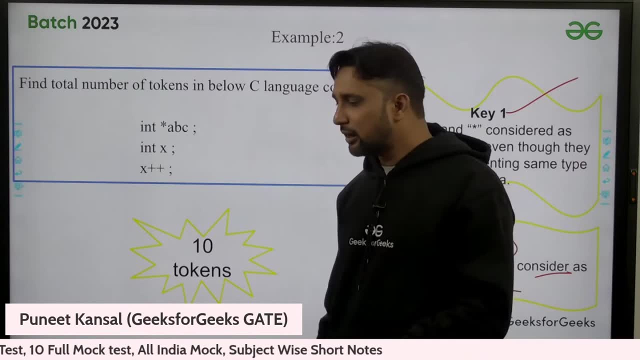 Now they are using these concepts only and they are making the question. they are trying to make the question tough, But if you know these concepts, they cannot make fool of you. You just need to do practice little bit and we will do practice here itself. 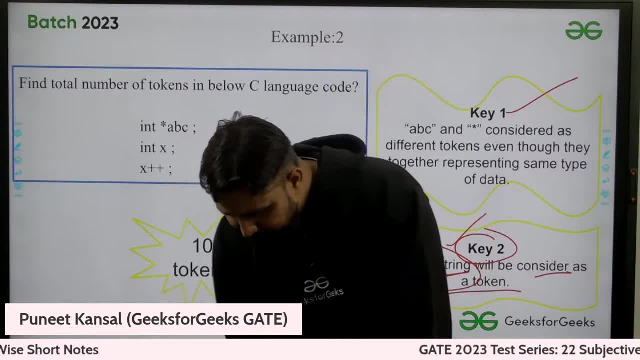 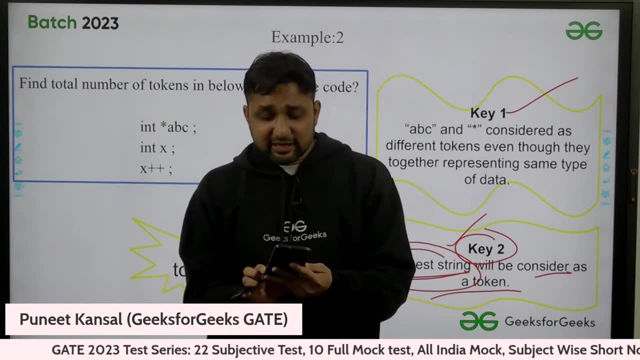 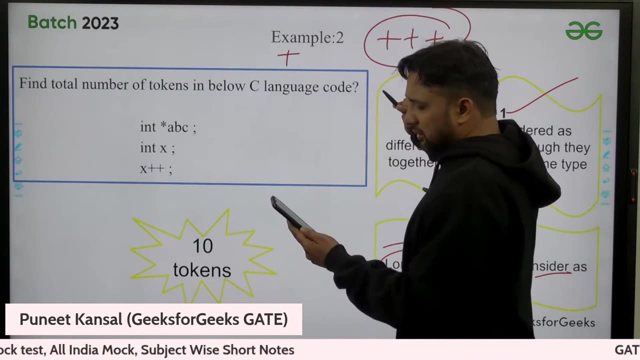 We have lots of time with us. One more hour we have. Okay, again one question Sainath is asking: but sir, in programming, this is this, is this. never happens, This, this, we will cover the PYQ also. 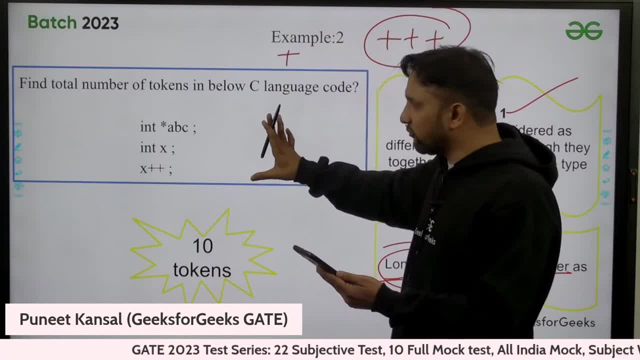 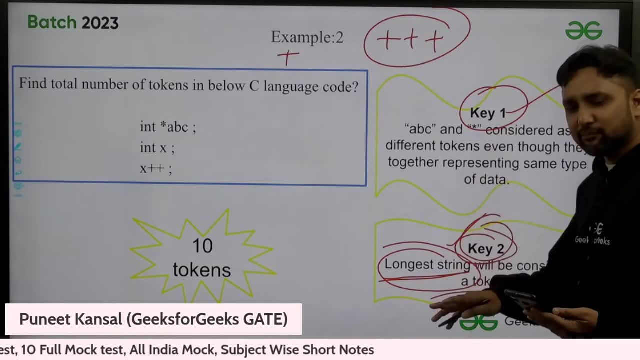 Okay, Sainath, we will cover PYQ, lots of PYQ, we will cover, and you people will solve it yourself. I am just clearing all the key points, which is very important. If we will directly jump over there, then you will actually. 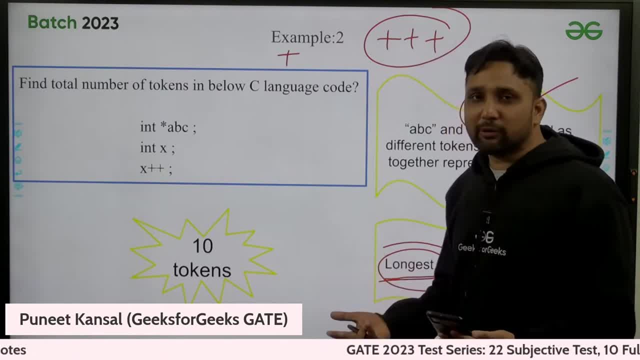 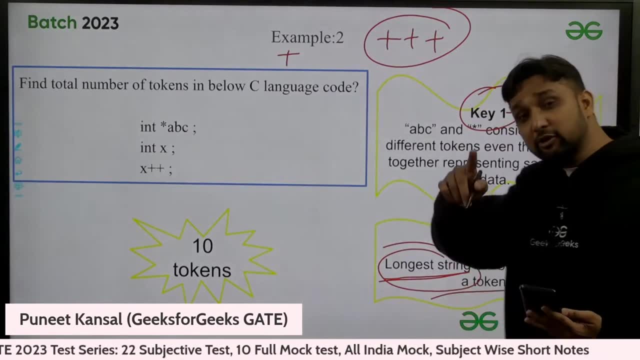 what will happen is that you will think that I am not able to solve the question. You will make this assumption in your mind. But if all the concepts, all the keys will be known, that will make easy for you people. Okay, because you know already. 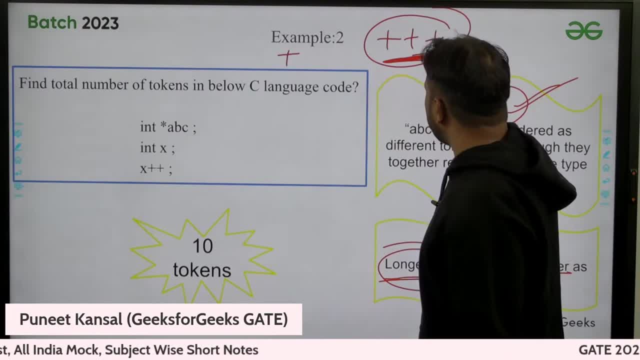 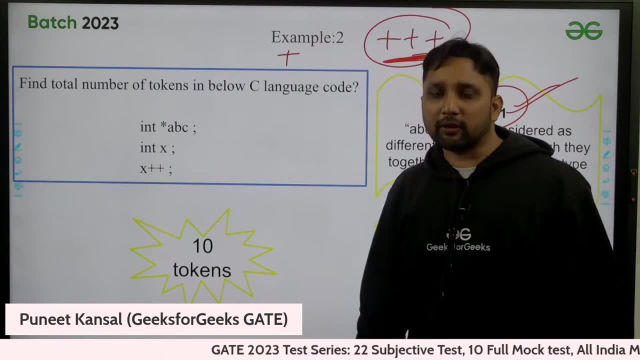 So the question is, this is not in the language, in any language, then how this can happen. Maybe, maybe the person is first time he is programming, First time he is programming, he don't know. He don't know that. okay, this is, this is some operator. 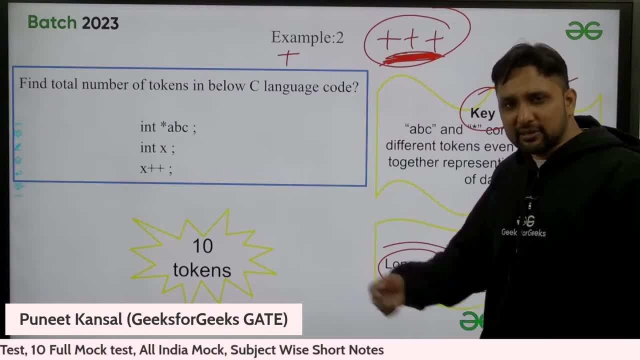 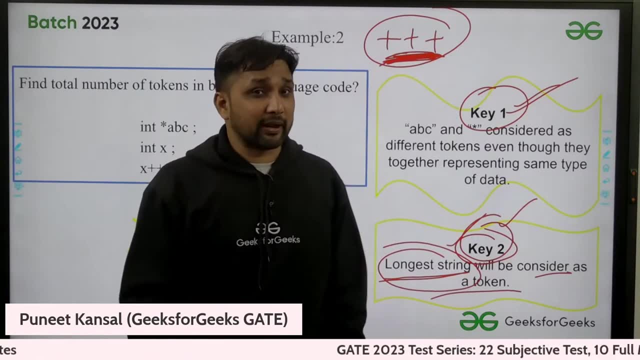 He know that this is incremental, This is incrementing, this is incrementing by one. by mistake, he write: okay. Now, important point here is that lexical analyzer phase, first phase of compiler, will not find out this syntax error. This is a syntax error. 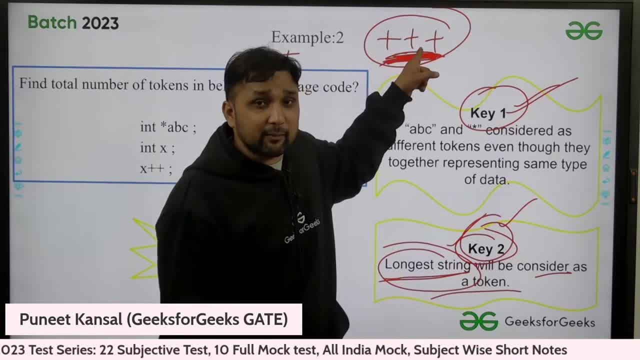 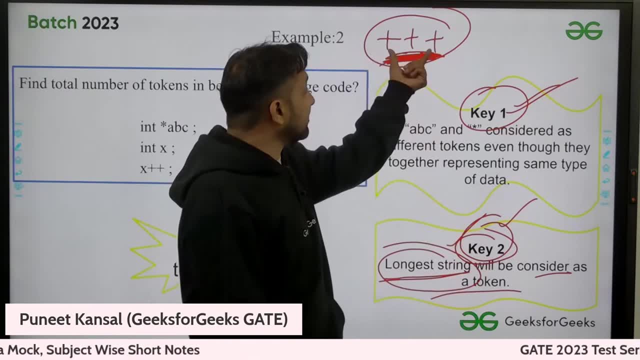 You are right, This is a syntax error. This is not defined in the compiler. plus plus, plus lexical. This is not the duty of lexical analyzer phase to identified something is wrong with this. He will pass on. he will pass on this thing. 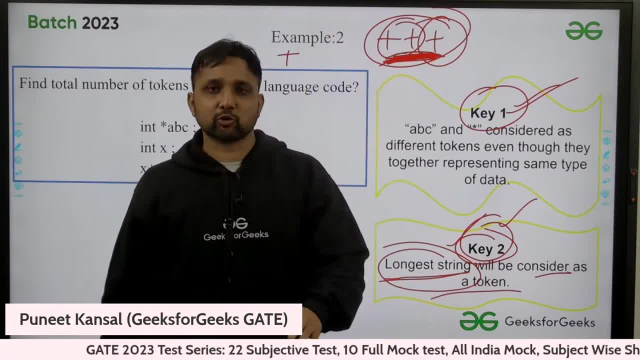 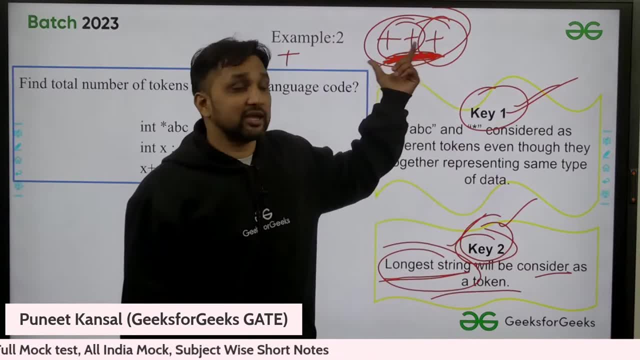 He will count the tokens He will pass on. okay, So who will find out the syntax problem? Second phase of the compiler: syntax analyzer phase That will identify that. okay, this is. this is not the right syntax. That will generate the error. 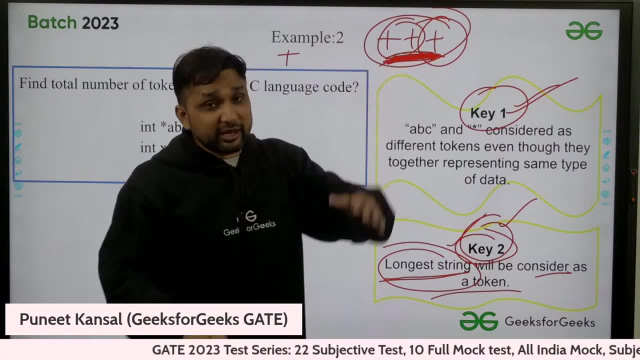 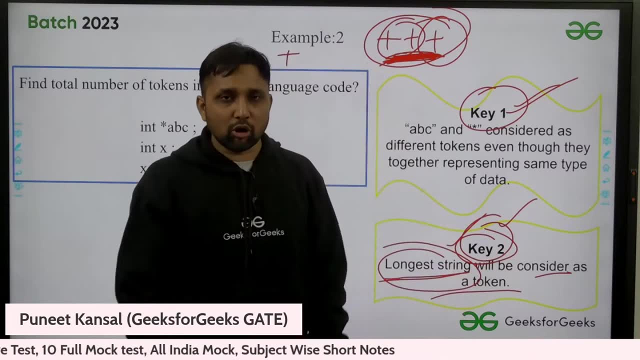 That will generate the error, not the lexical analyzer. They can ask the question to you. They can give you wrong something wrong- okay, They can write the something wrong. They can give you something wrong code and they give you one option: none of the above. 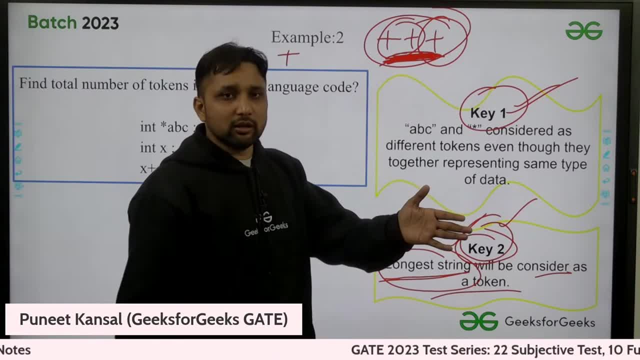 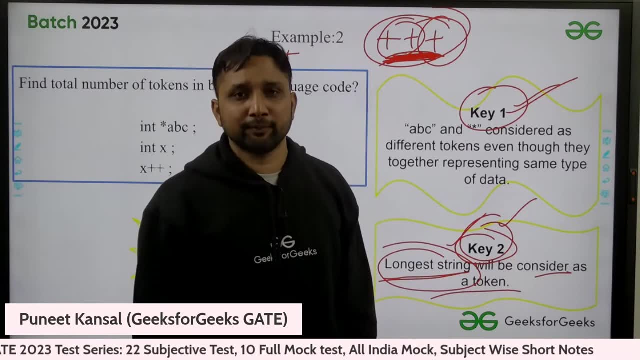 Or maybe they give one option: Syntax error. Syntax error is given by the second phase of the compiler, not the first phase. Lexical analyzer: don't give the syntax error That. do not give the syntax error. That is given by the second phase of the compiler. 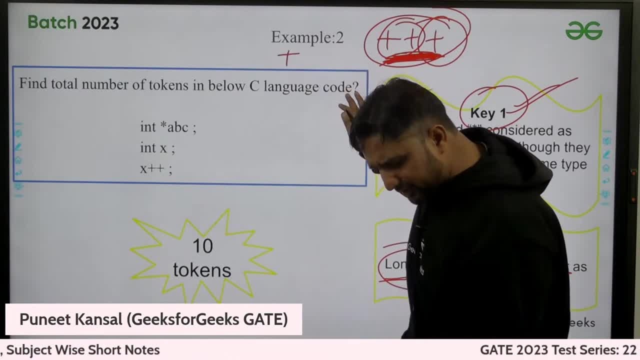 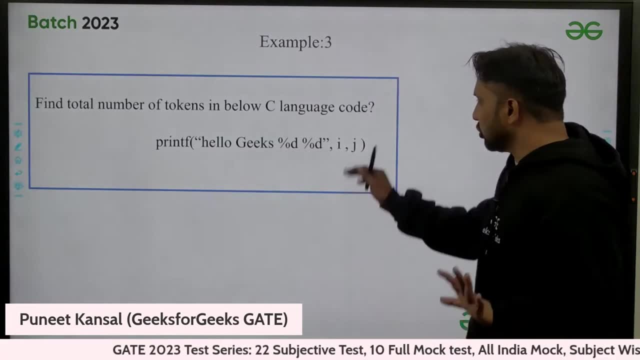 So lexical analyzer is not bothered about the syntax. We will cover this thing also, okay? So let me move to another question. Then I will move to the chat box. So you people, please try this question yourself again. Please try this yourself. 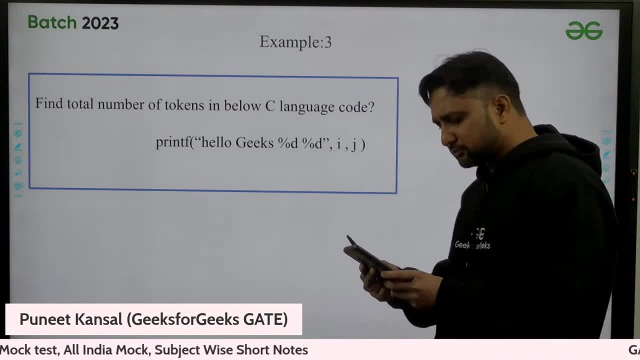 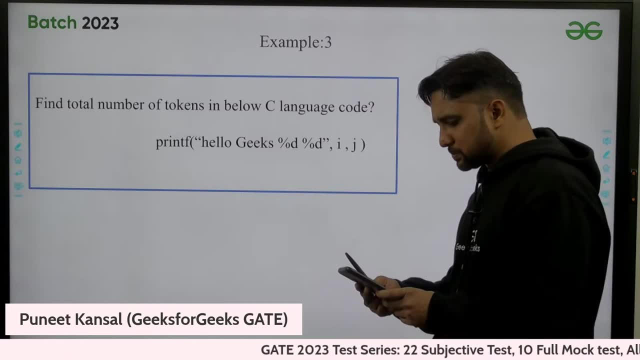 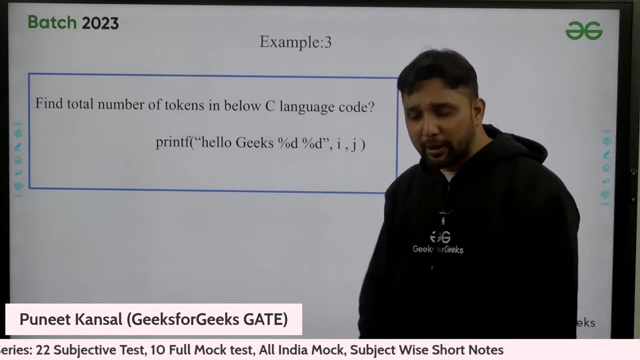 And meanwhile, let me check out the chat box. Yes, Harshay Lexical analyzer is not bothered about the syntax. Yes, Second phase of the compiler is bothered about the syntax. Please give me the answer of this question. Please try it. 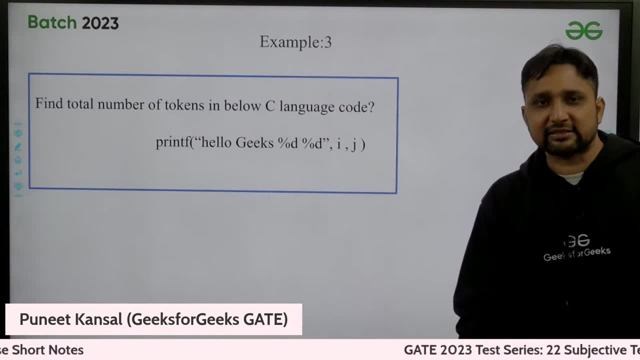 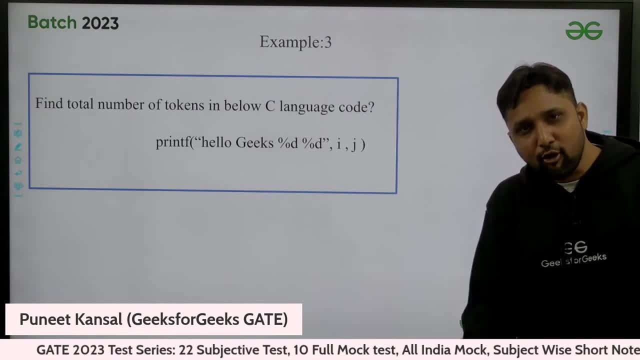 Right or wrong doesn't matter right now. Right or wrong doesn't matter in this class. That will matter in the exam. Okay, You are here. You are wasting your time with me because you don't know, If you already know, why you are here. 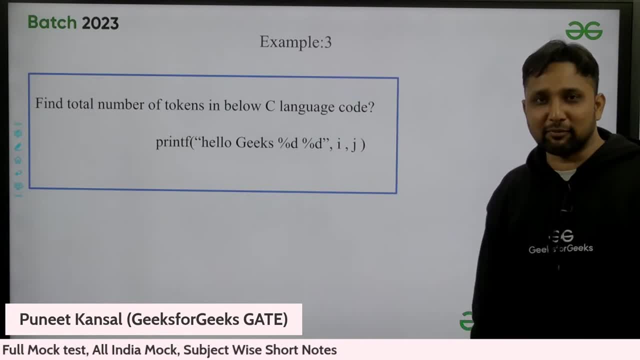 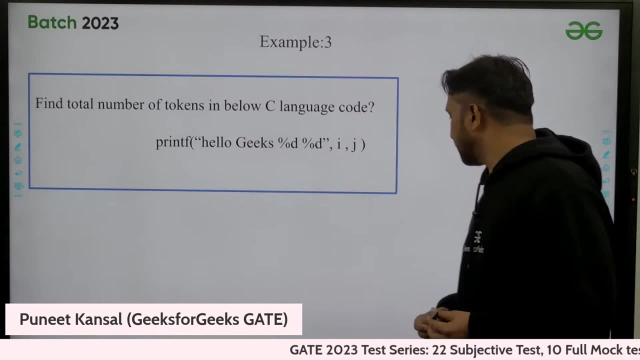 You must be watching something on Netflix Why we are wasting time here. Because we don't know. And if you don't know, please ask the question. Okay, And please try this. Please try it. Please write the answer. Whatever you are writing, that is the important thing, is you please give the answer? 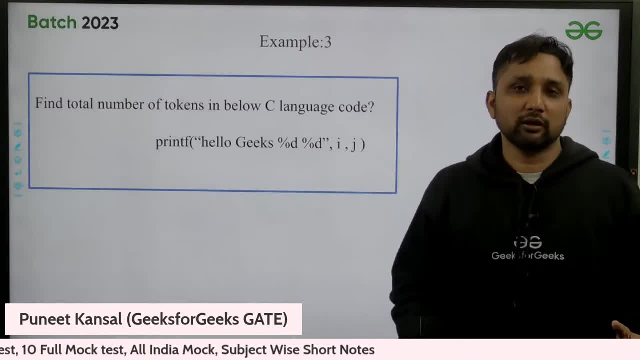 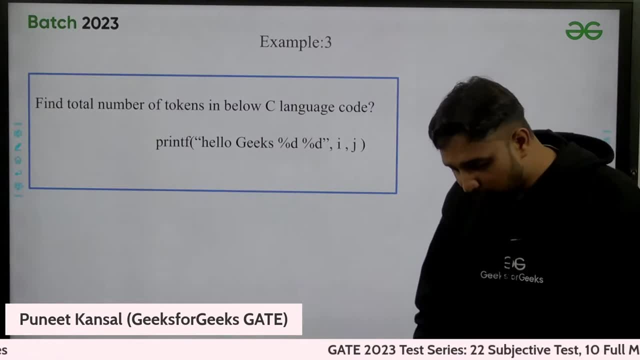 Important is not that you are giving wrong or right answer. Believe me, that is not required right now. Even you will give wrong answer, you are still learning. We are learning here. We are not proving ourselves right now. We will prove in the exam. 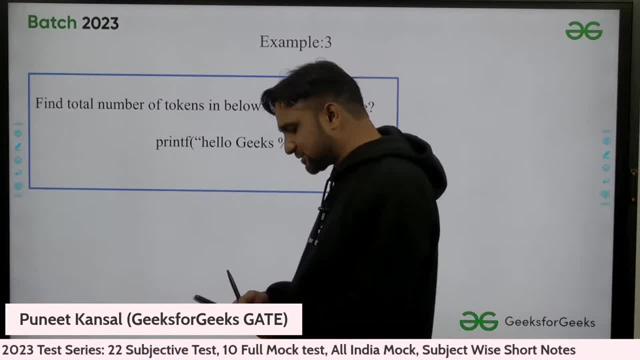 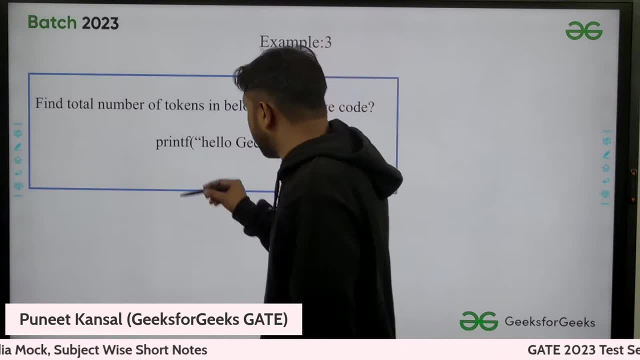 So many. all the people are saying 15,, 15,, 15.. Some are saying 8 also. Keep trying, Keep trying. Okay, Let's try, Let me try also. So this is one. Wrong or right doesn't matter. 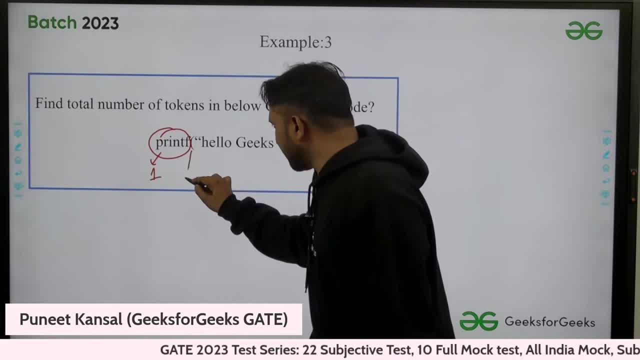 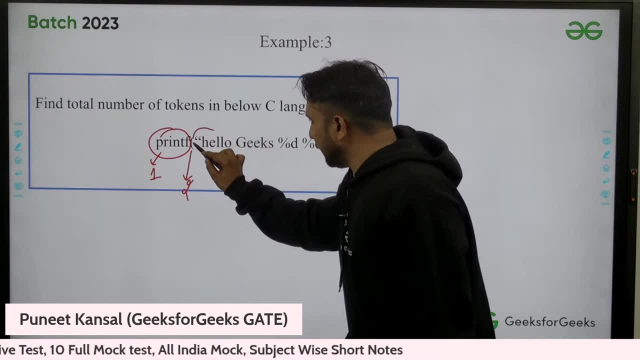 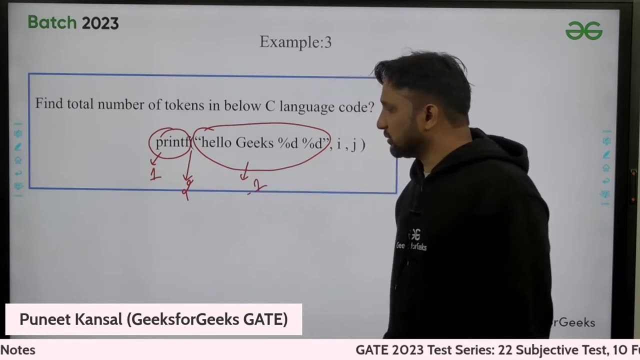 Doesn't matter at all Right now, that it doesn't matter In exam, that can matter. Second token: See, This will be considered as one token. Everything in the court, everything in the court will be considered as one token. Already we get, I think, one right answer also. 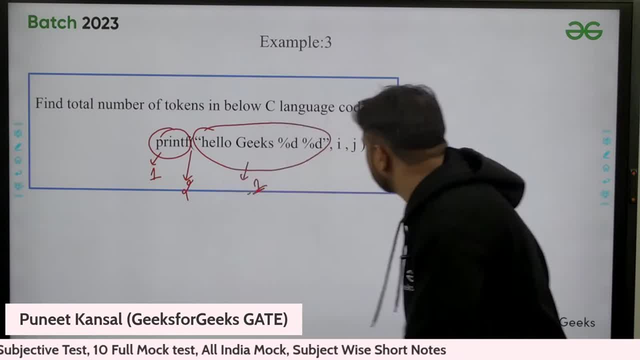 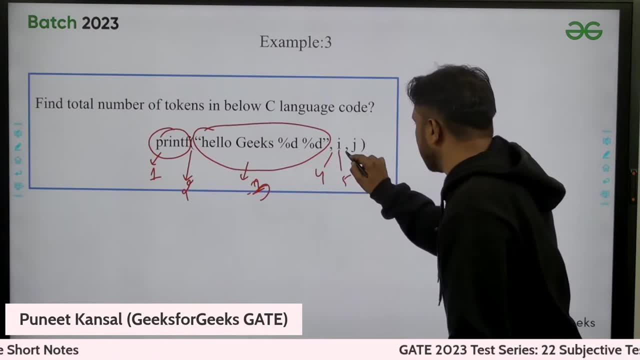 One or two From Anku and Kavya. Let's check out. So this is the third token. we get Fourth token, Fifth token, Sixth one, Seventh one And this is the eighth one. So we have eight tokens here. 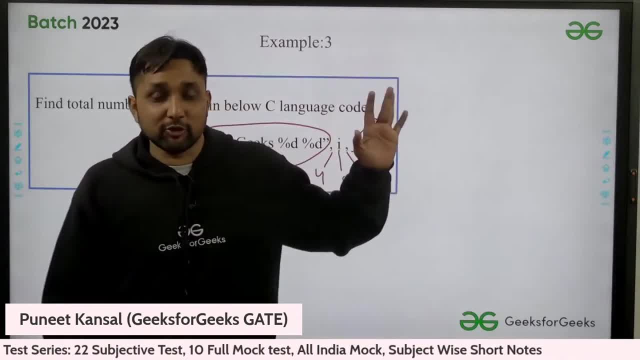 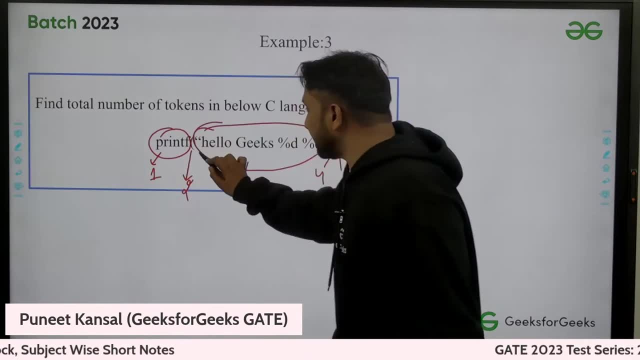 So we get one more key. We get one more key. You try it yourself, So you will keep remember. now You try, You write the answer, So you will keep remember that. Okay, Everything inside the courts will be considered as a one token. 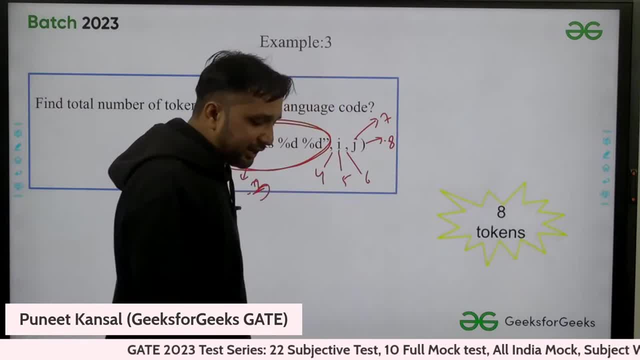 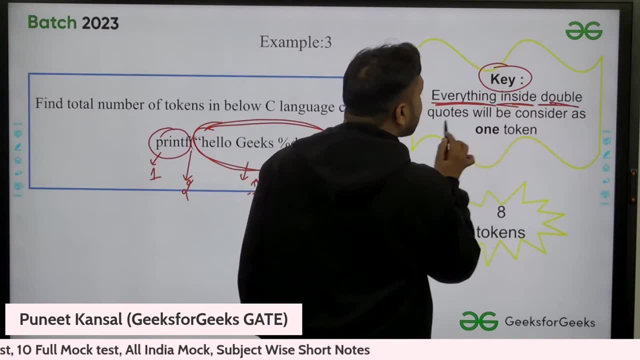 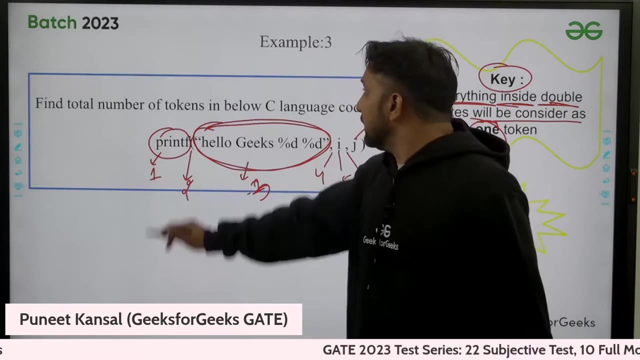 This is how compiler is behaving. This is how compiler is designed. So eight tokens are here And the key is: What is the key? Key is: Everything inside the double courts will be considered as one token. Everything inside the double courts will be considered as one token. 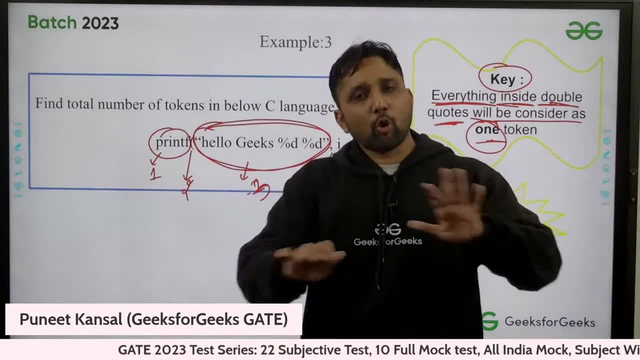 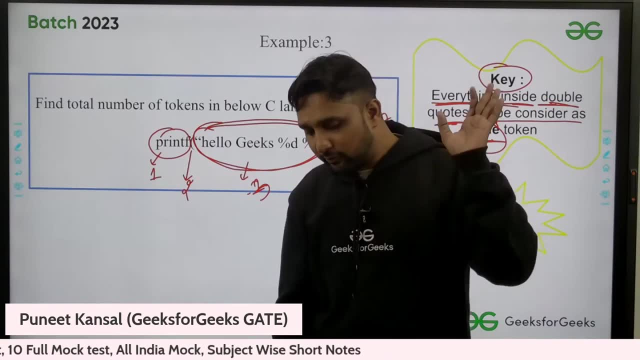 With the help of- Again, I am repeating, With the help of these examples, we are covering all the keys, point Okay. So we are covering all the. We will not left even a single one, Okay, And after that you will be able to solve any gate question. 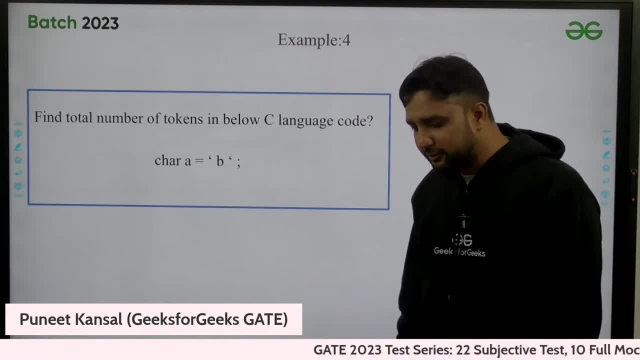 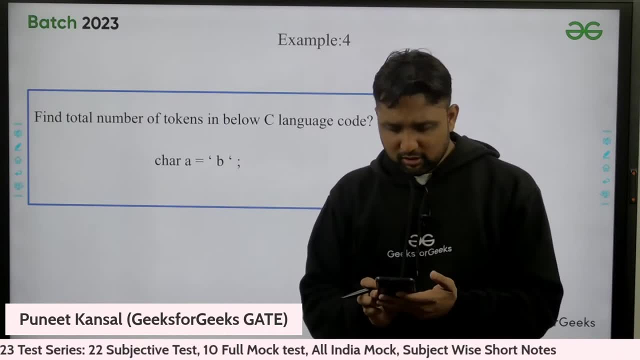 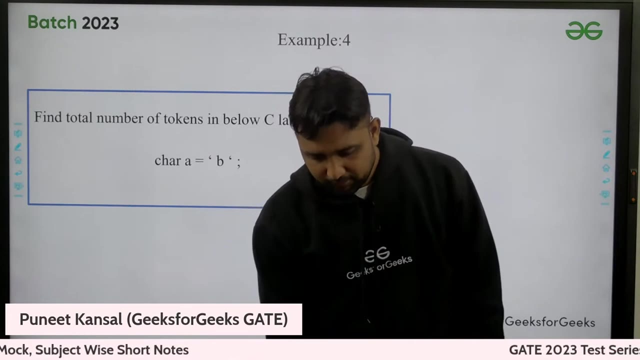 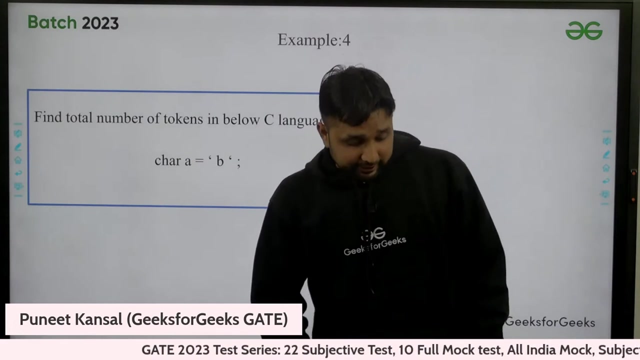 So next question: Please try it. Please try it. Please write in the chat. Please write in the chat Everyone, please. We will cover all the key points. You will left with nothing. Take this complete gate, crash course. I am giving you surety. 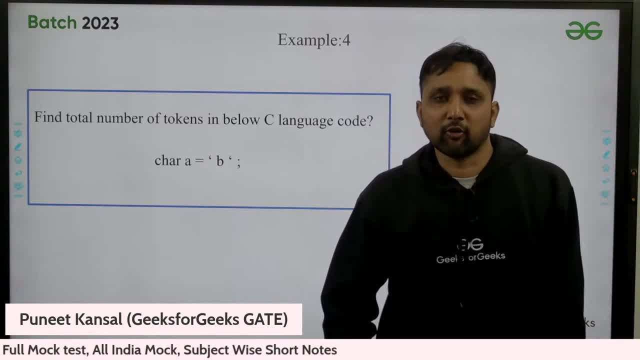 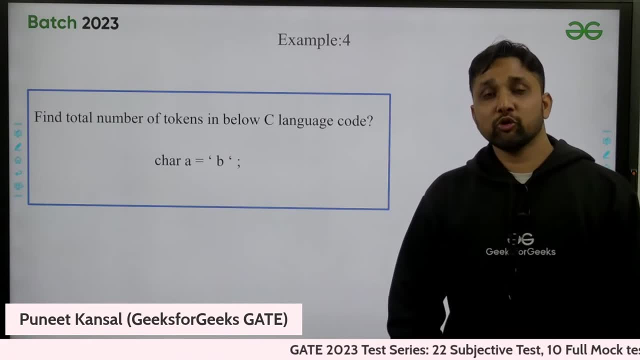 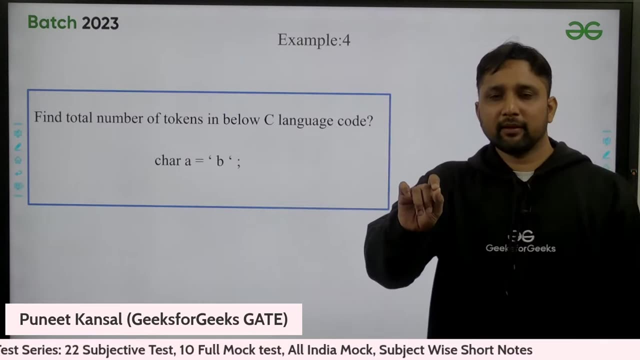 You will clear the gate exam, at least If you don't know anything right now. If you already know, Please attempt again this. Please attend this gate series. Your most important topics will be revised. Everything we are covering, Each and every point we are covering in every lecture. 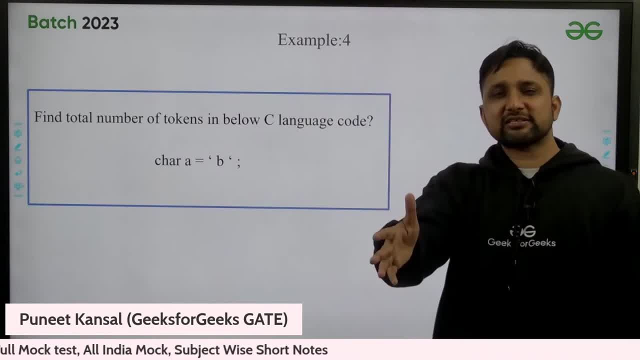 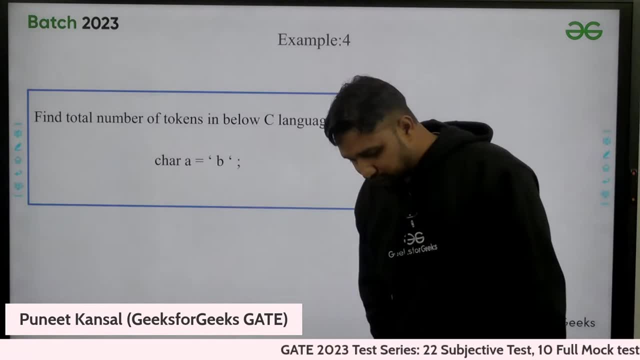 And we are not relating that lecture from previous lectures. Every lecture is just like individual lecture. Okay, So attend this series and you will get benefit. So it's a gift from GeeksforGeeks for you people. GeeksforGeeks is always helping the students. 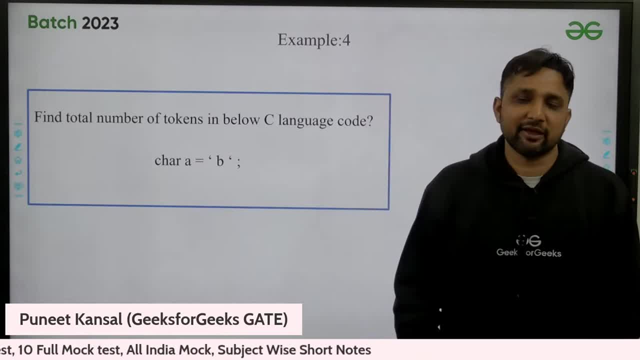 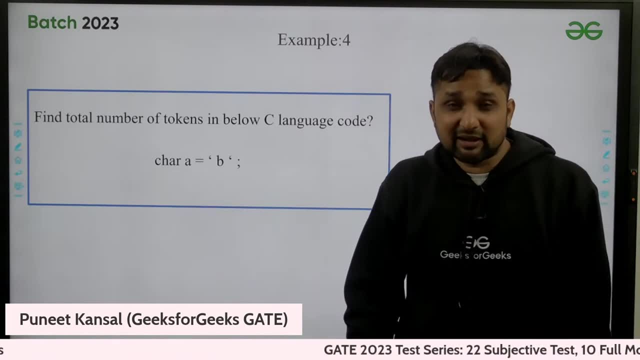 That is always trying to help the students in every way. It's not because I am working here. It's because I have already. I have myself also used GeeksforGeeks. It's not because they are paying to me. It's not like that. 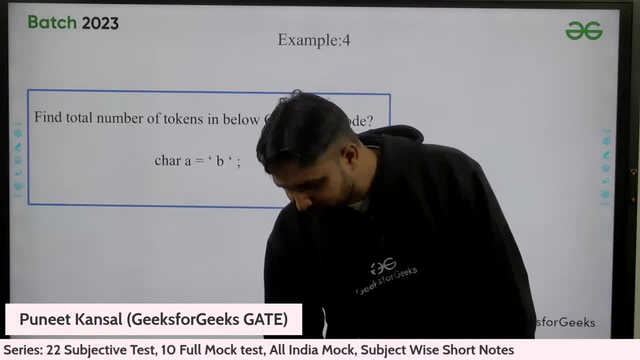 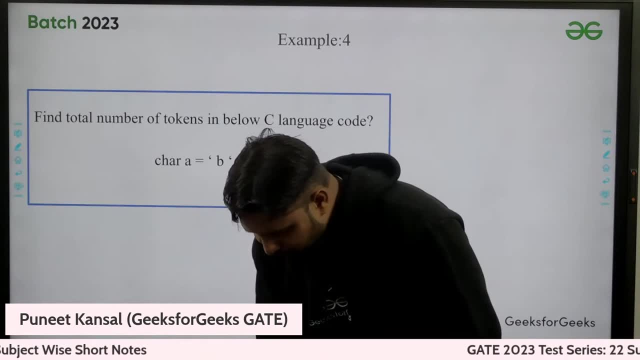 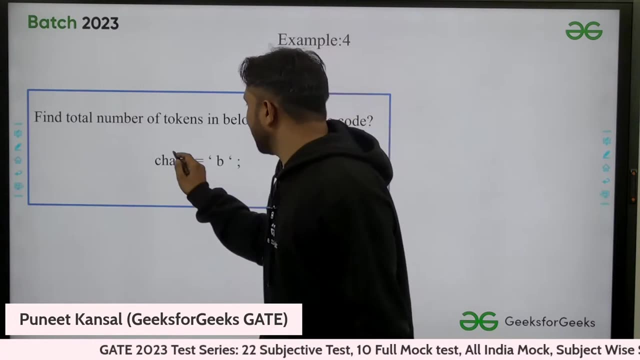 But you already know that. Okay, We get same answer: Divyanshu, Sainath, Arshay, Jerry and Kavya. Everyone is saying five. That must be right. That must be right One, Two. 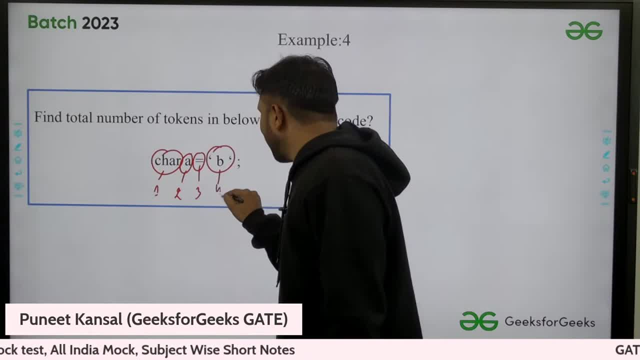 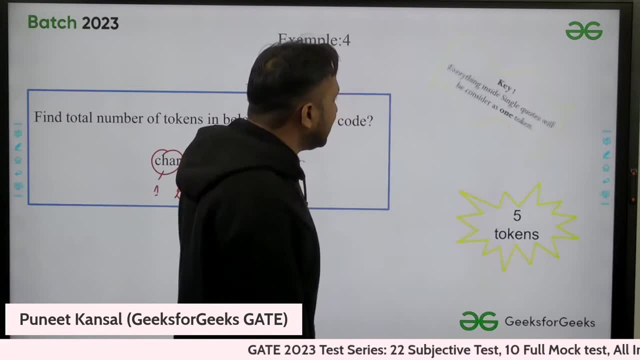 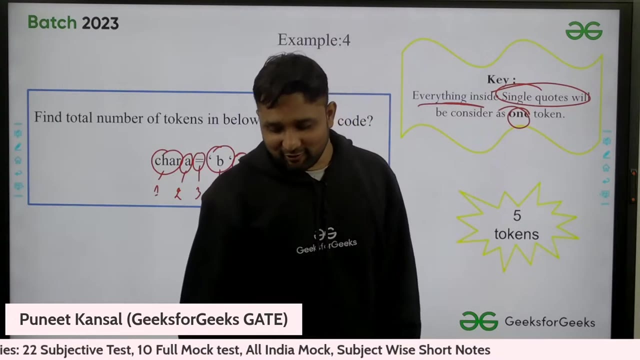 Three, Four And you get the point. actually, You get the key point. You get the key point here. Everything, Everything inside the single course also will be considered as the one token. You already know this thing now. You already know. 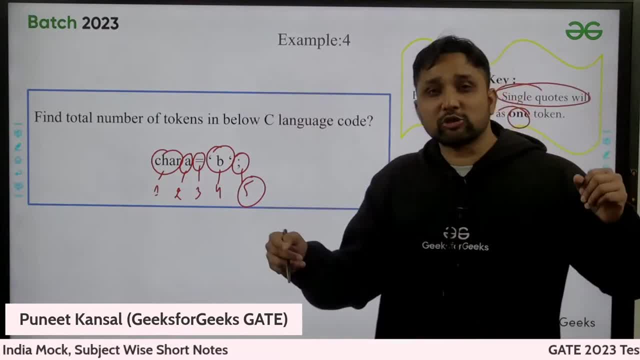 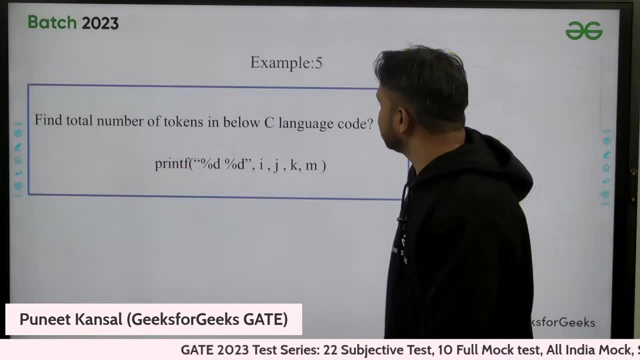 You already check out this thing: Everything inside double course is also one token, And everything inside single course also is considered as one token. Okay, Great, Great. Another example: Please find out the tokens. Please find out the tokens. Please write in the chat. 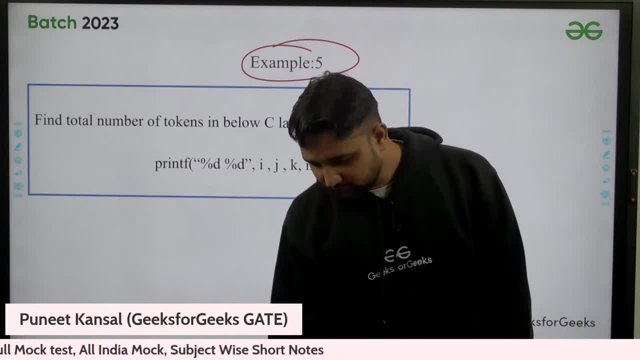 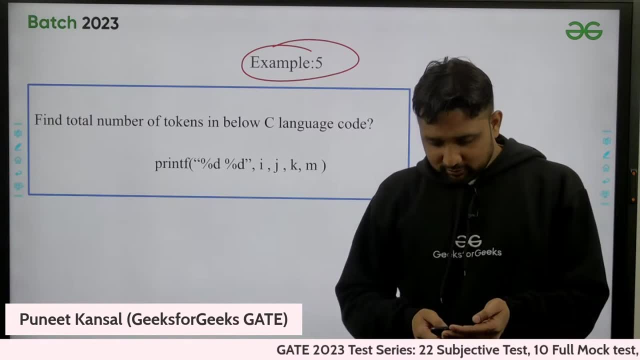 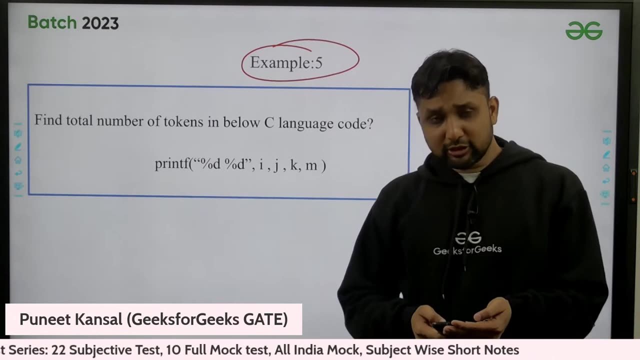 Everyone, Please. I know you people may be hungry- It's lunch time, But I am also hungry. Believe me, You will take the food. Believe me, You all will sleep. I will also sleep If I will eat the food right now. I will also sleep with you. 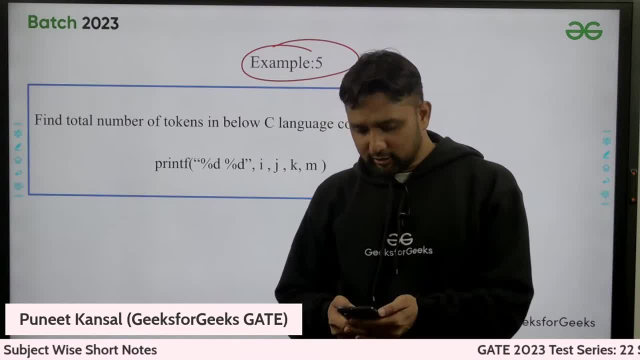 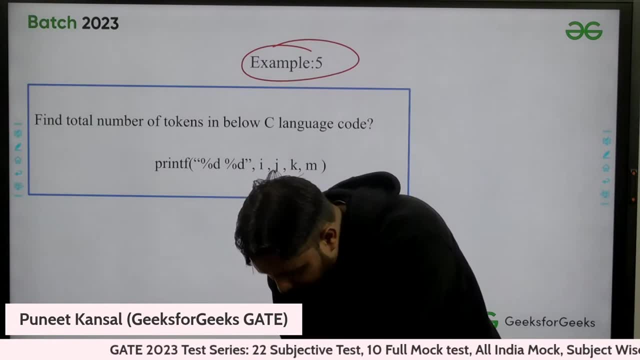 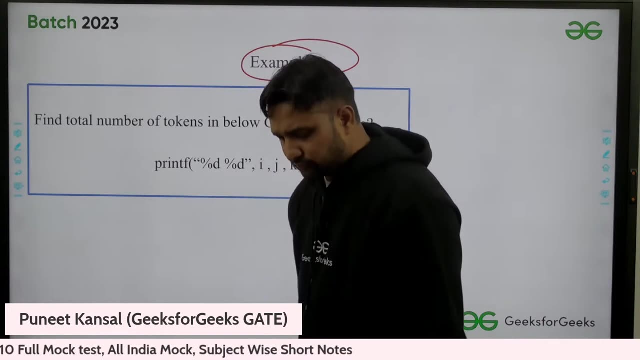 And we will spend one hour in sleeping only. So twelve, Twelve, Twelve. Many people are saying twelve. Keep trying, Everyone. Please keep trying. Please write it in the chat box If you already know, If that's easy for you. 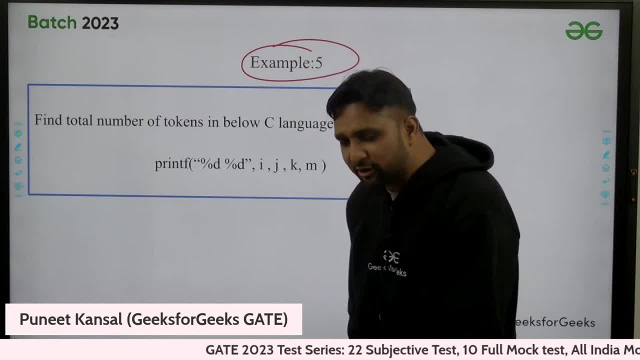 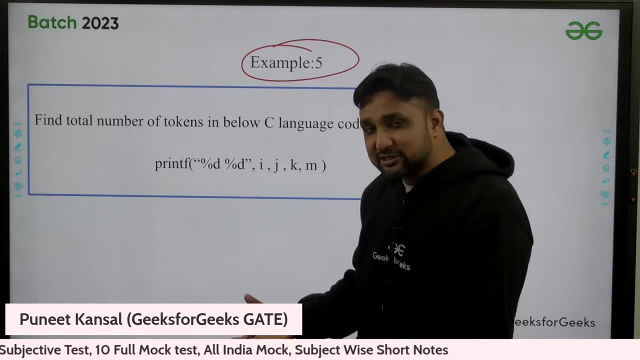 Please write, Please help other people. If you don't know, Don't worry at all, Nobody is going. Nobody is going to. Nobody know here to us. At least we can share right now here. Okay, Nobody know us on this chat box. 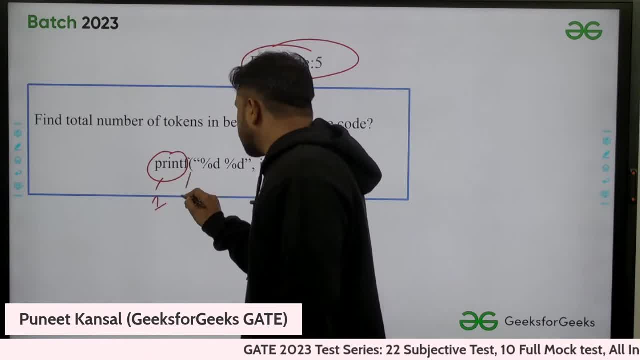 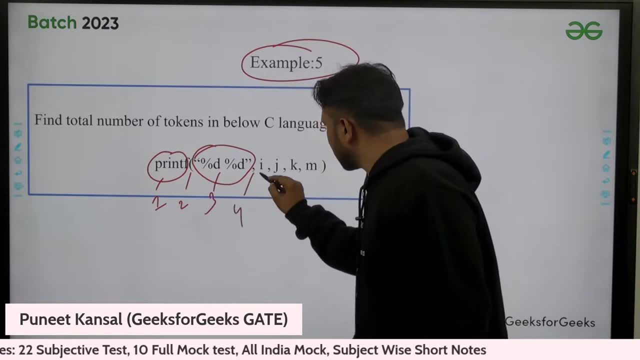 Okay, So this is first one, This is second one, So double course. This is third one, This is fourth token, This is fifth one, This is sixth one, This is seventh one, This is eighth one, K is ninth one. 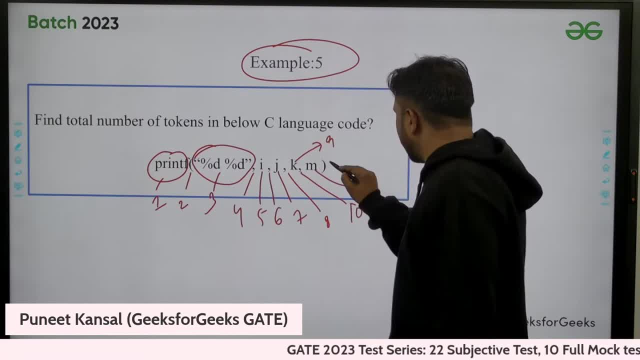 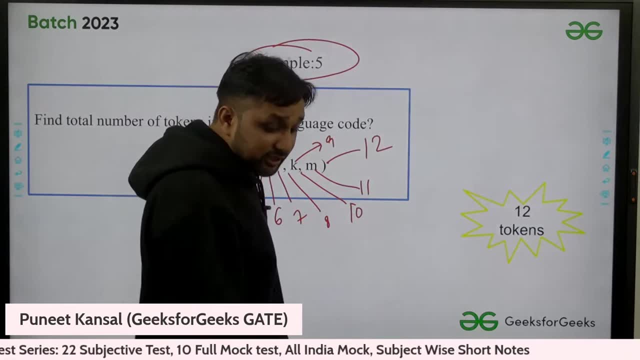 This comma is ten, This M is eleven, This closing bracket is twelve. So all the people are giving the right answer. So twelve tokens are here. And what is the key point why I give this example? Actually, you already know this key point. 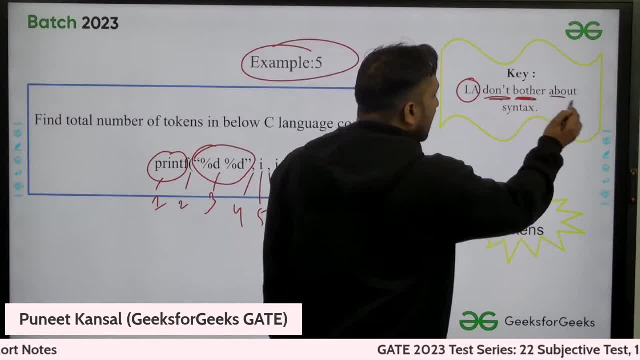 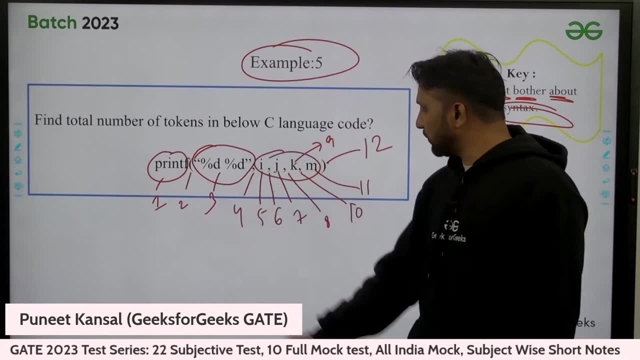 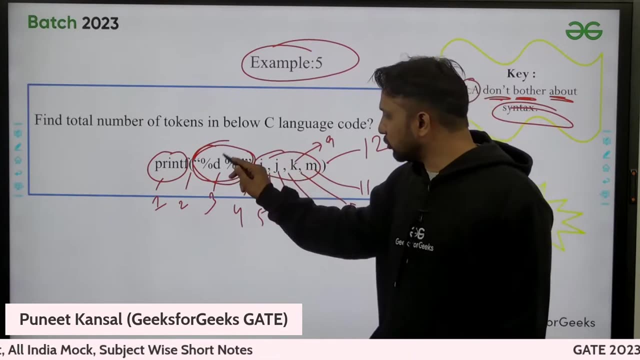 Lexical analyzer. do not bother about the syntax. You can see here if you know C language. We have written here four variables, But I need to write percentage D four times. If I am printing four variables, I need to write percentage D four times. 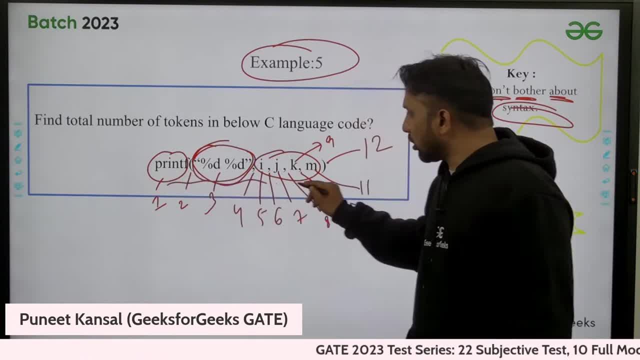 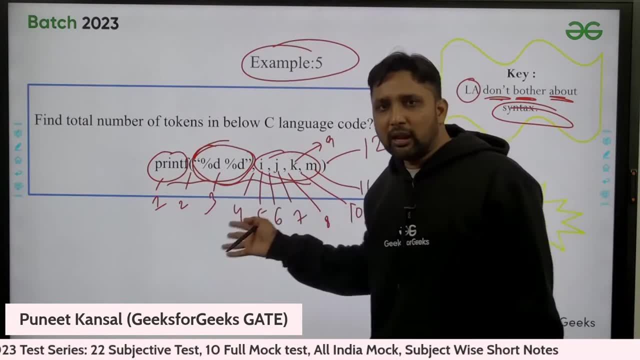 If you know C language, So this syntax is wrong. But syntax analyzer is not bothered about the syntax. It will count the token, Store the variable into the symbol table And pass it to the second phase of the compiler, syntax analyzer phase. This is the duty of syntax analyzer phase. 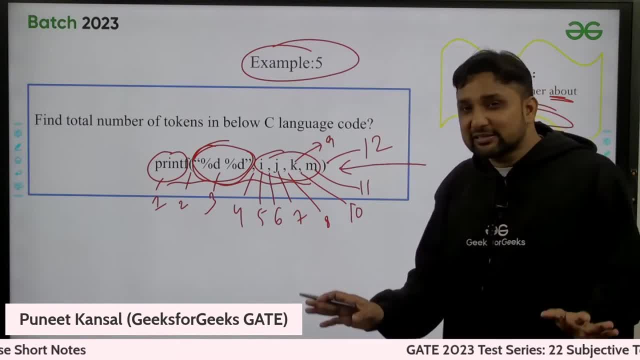 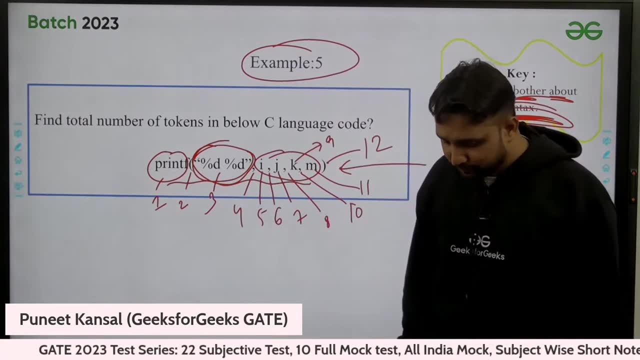 To check if the syntax is right or wrong. Lexical analyzer is not bothered. Lexical analyzer is not bothered about the syntax. He will simply count the tokens and pass it. Let's move on to the next example. Sixth example: Please find out. 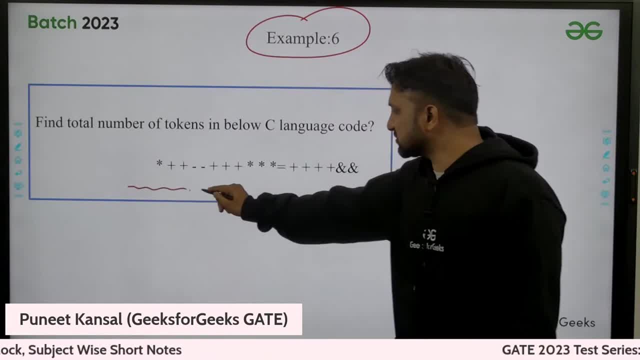 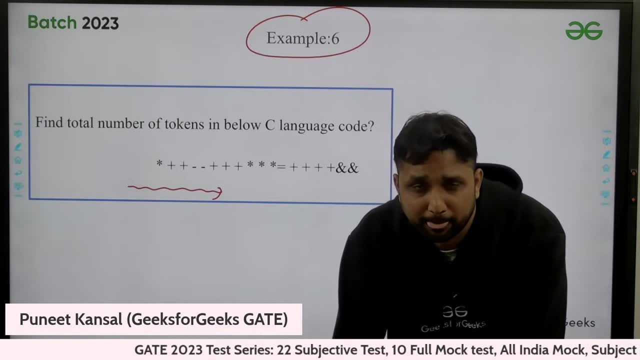 We are not bothered about the syntax. Please find Start from here. Please find out number of tokens. You will be able to solve every question. Keep trying. You will be able to solve every gate question. Please keep trying. Please try it and write the answer in chat box. 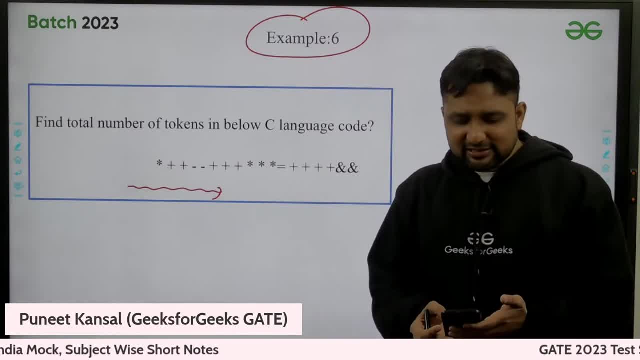 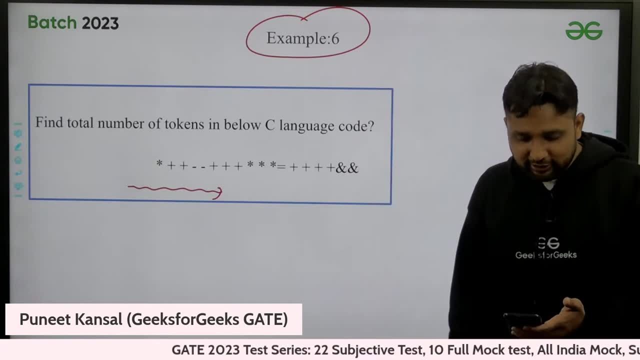 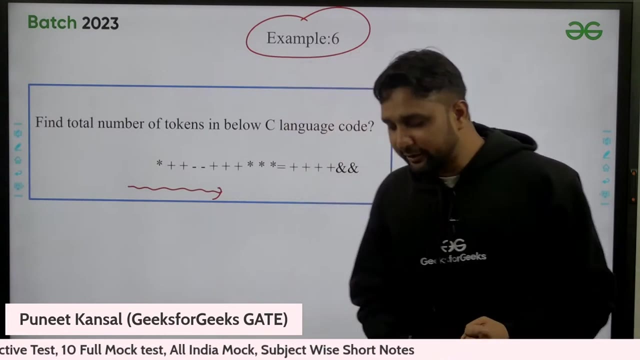 If you like this session, Please give some time to give a thumbs up. That will boost my confidence for the next lecture. I will put more energy, I will put more good content in that. Please give a thumbs up also. Please give a thumbs up also. 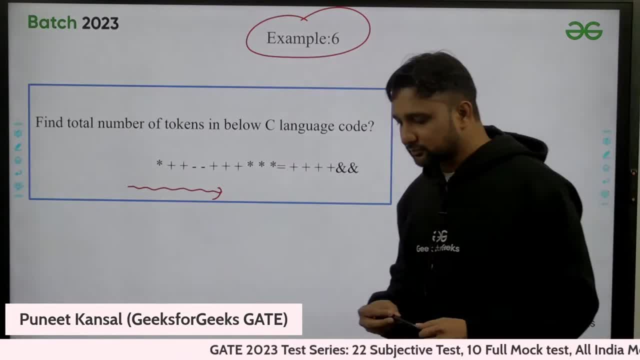 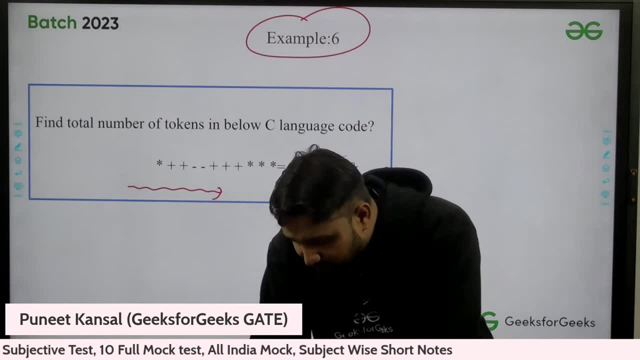 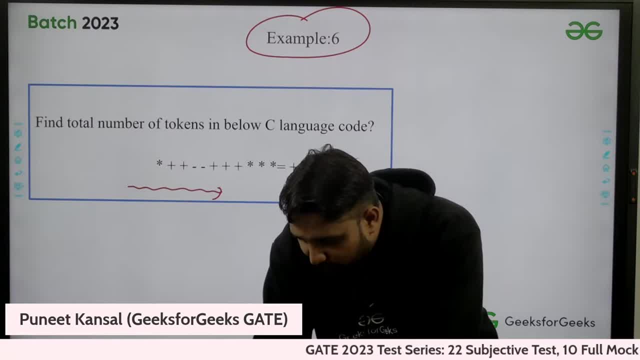 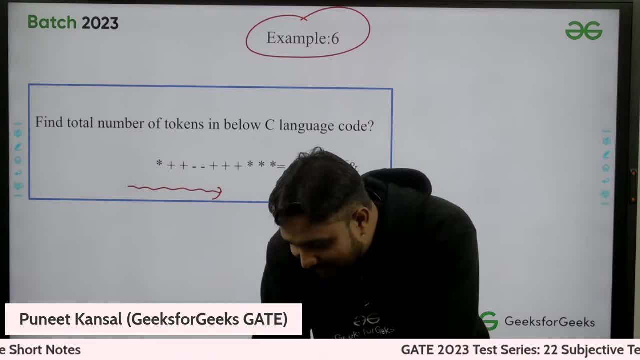 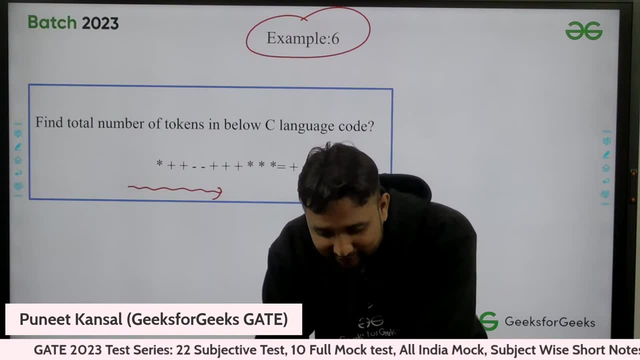 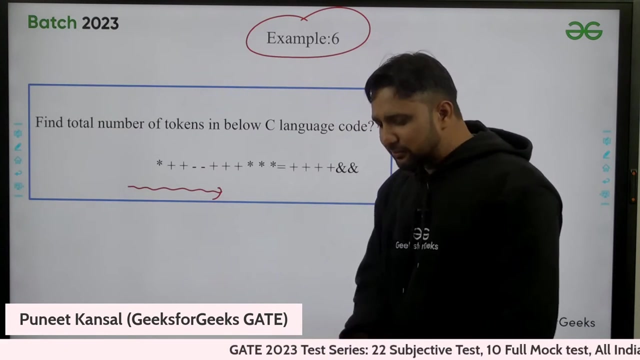 Please like the session. That will boost my confidence for the next session. I will put more energy. Maybe I will take the keyboard and I will break the keyboard in front of you. I will show more energy I have. Okay, okay, So let's kind, let's try to find out. doesn't matter answer. doesn't matter right or wrong. 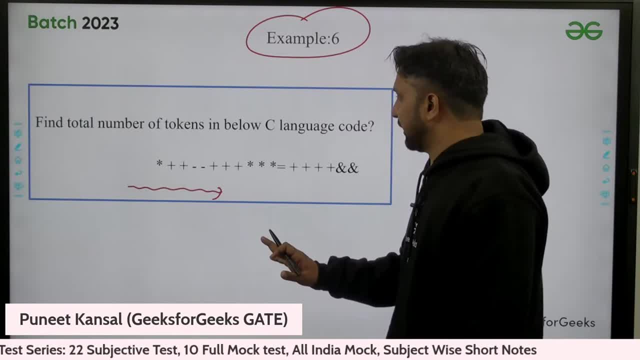 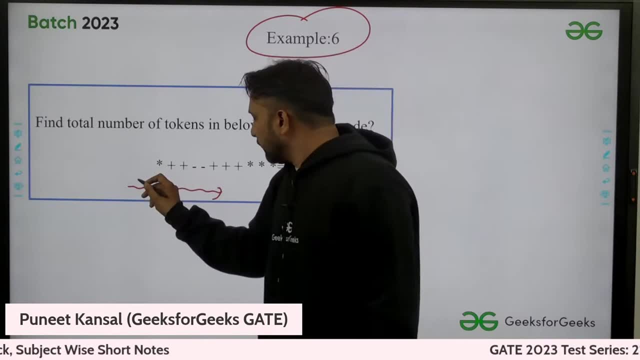 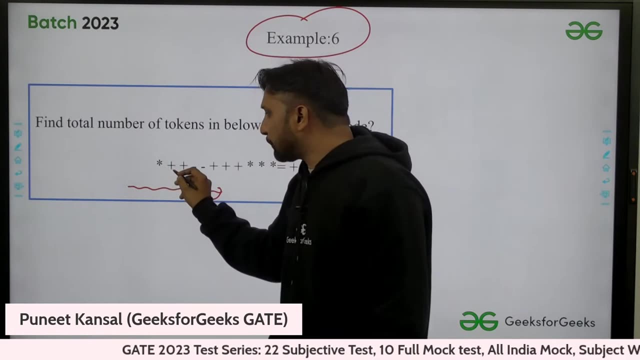 What matter is, right now we are trying because we are learning when we are trying. okay, okay, again, same rules, we will apply, keep applying which we learn till now. okay, We are finding the longest, we are finding the longest operators. okay, So after: multiply plus is not operator. this is not not any operator. okay, multiply n plus. 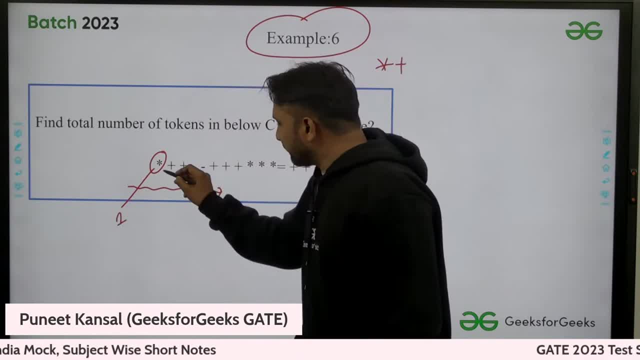 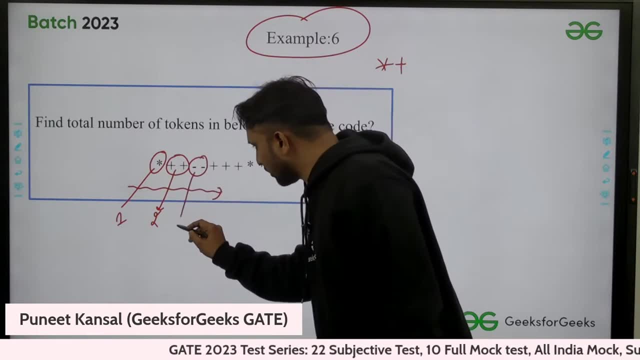 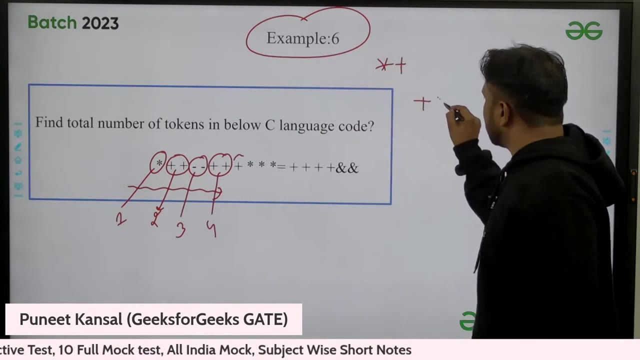 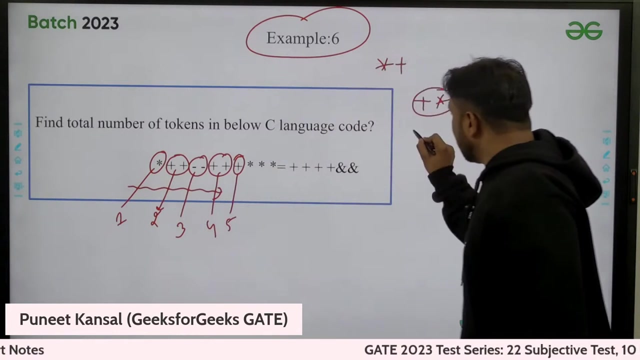 So this is one token. After that longest operator, This operator is plus plus. this is another token. this is another token. this will be another token. see, plus multiply is not not any operator in C actually. So plus is another token. multiply, multiply is not any token, okay. 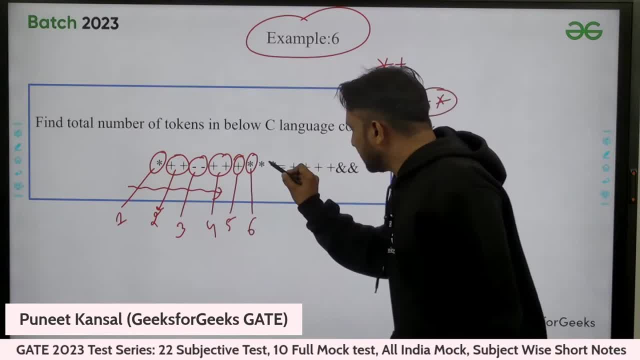 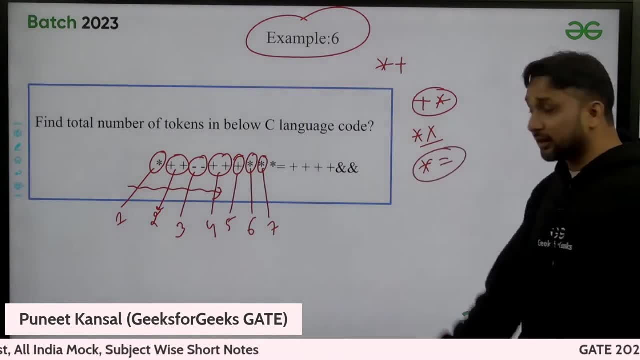 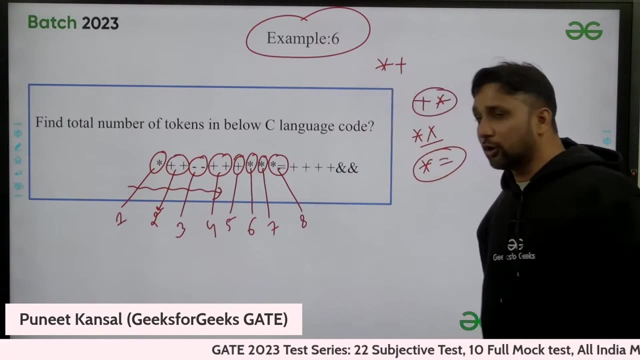 So we need to consider single as a one token. again, single multiply as another token, see multiply equal to. This is a one token. This is a operator, this is a operator in C, we know. so this is one token. we need to take the longest one. we need to take the longest one plus plus another token again, plus plus. 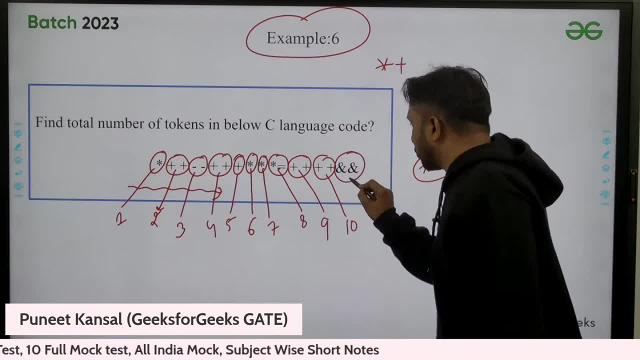 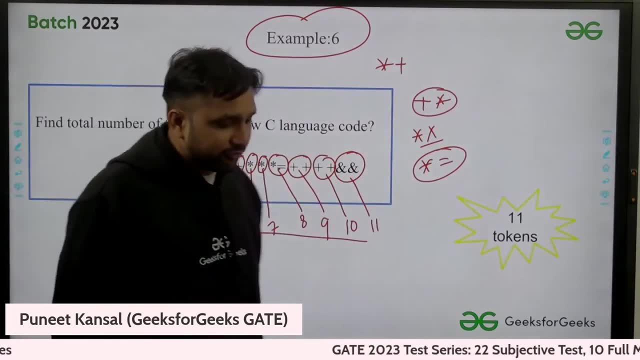 another token and this is one token. again, this is and operator in C, So total we have 11. let me check if I done it right. yes, we have 11 tokens here. we have 11 tokens here. The only rule I apply here is that. 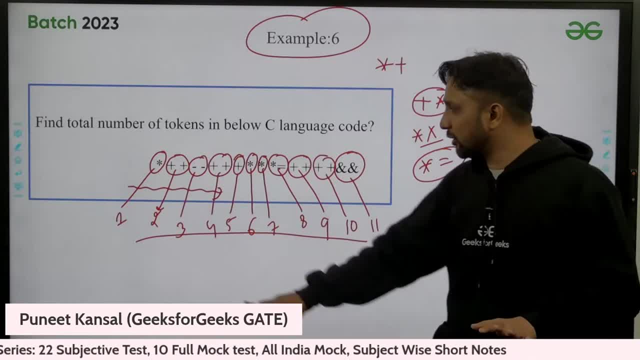 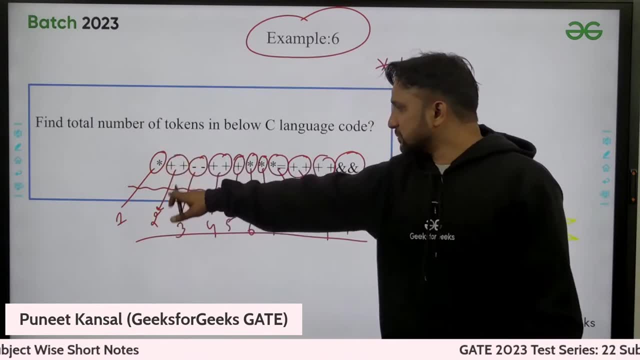 I try to find out the longest one. every time I try to find out the longest one. multiply plus was not making any operator, So multiply, I left it. and plus plus then minus minus, and plus plus then plus and multiply, multiply. multiply equal to was there. this can be little tricky. 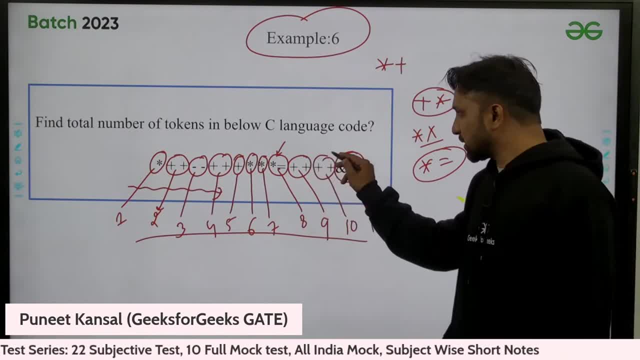 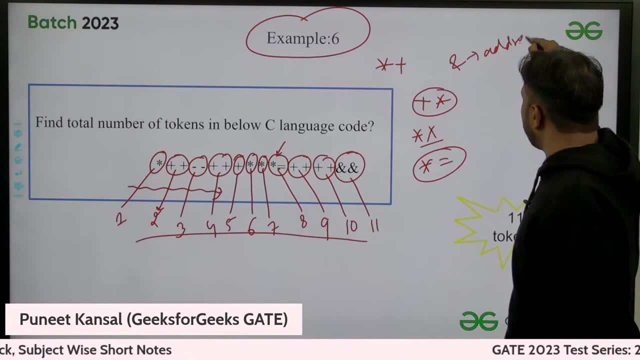 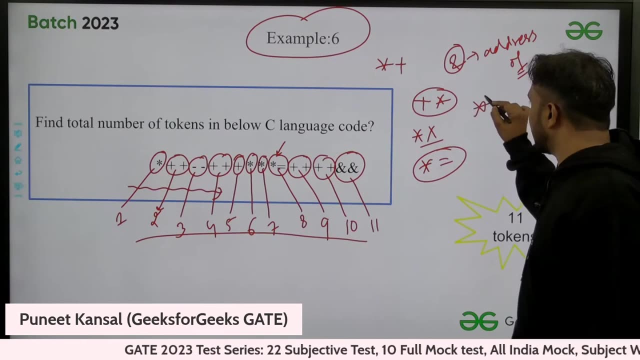 So multiply equal to: was there plus, plus, plus, plus, and this was: this is also and operator. okay, And single. this is address of. this is address of operator. okay. okay, if you want to find out the address of something. okay, if you want to find out the. 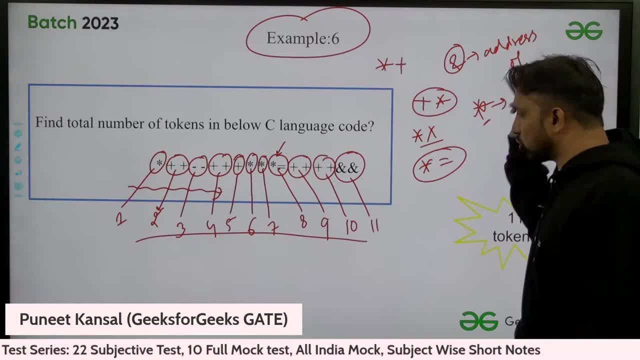 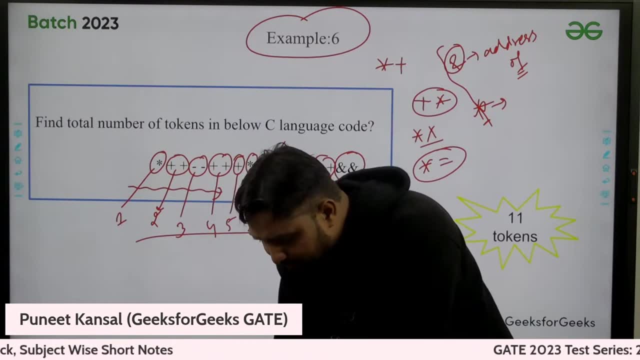 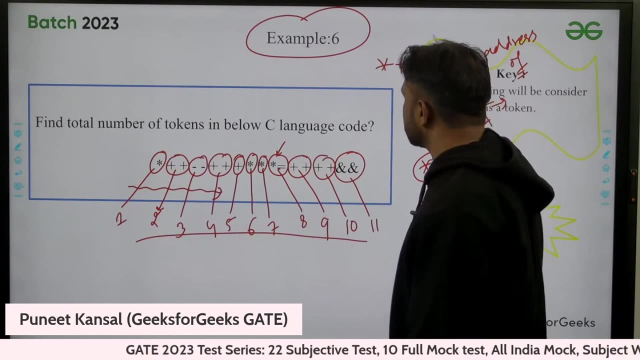 value, then this is: can be single, can be used for value also. okay, that is different thing. any doubt in this? please ask any doubt. important is that: keep clearing your doubt, because now i think examples are almost finished after that gate, uh questions we will cover. so this is the. 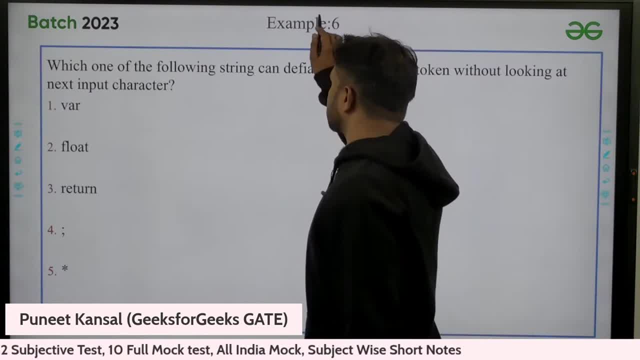 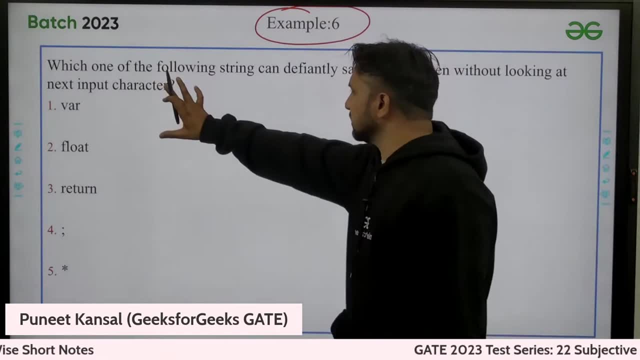 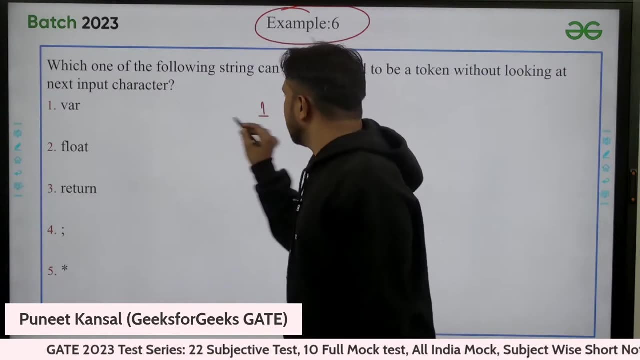 last example. i think, yes, after that, your, you need to solve the questions. i will sit and you will solve the question, please. uh, try to find out, check out the question and uh, you need to give true or false. okay, so you can write like this: for first, is this true or false? second, true or false whatever. 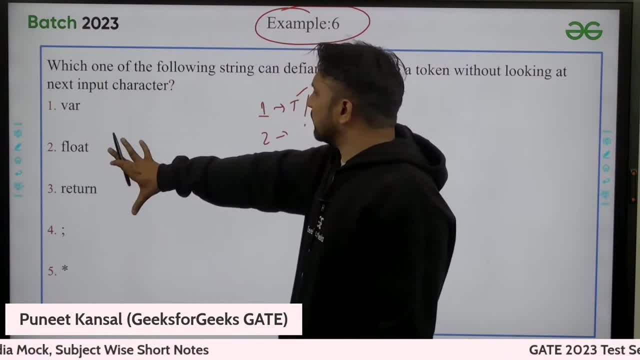 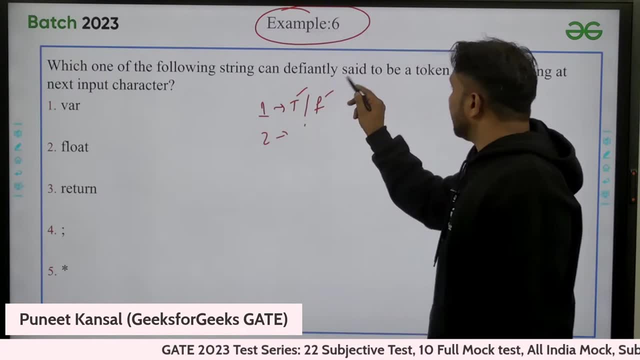 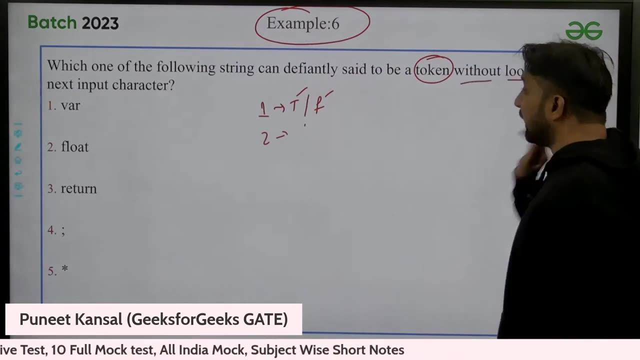 is that you need to write. so what is this question? okay, let me read which of the following string out of these six string, which of the following string, can definitely set to be a token, which can be set to be a token, definitely can be set to be a particular type of token, without looking at the next input character. 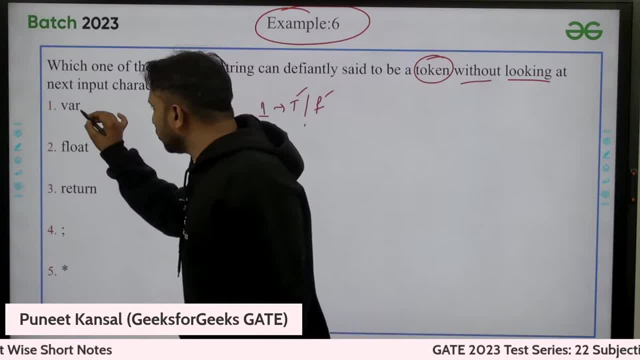 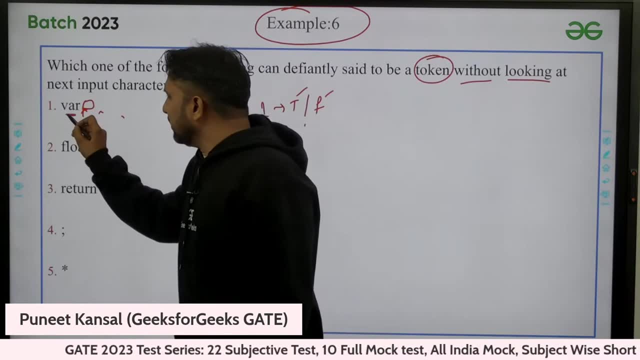 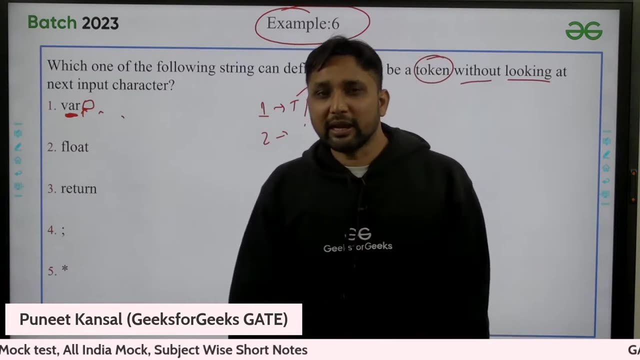 okay, without looking at next input character, without looking at next here. what is the next is coming? what is next is coming? without looking at here, can i tell which type of token is this? is this a operator? is this a function? is this is a keyword? can i tell this thing without looking at next character? next vector: here, maybe here, maybe here. 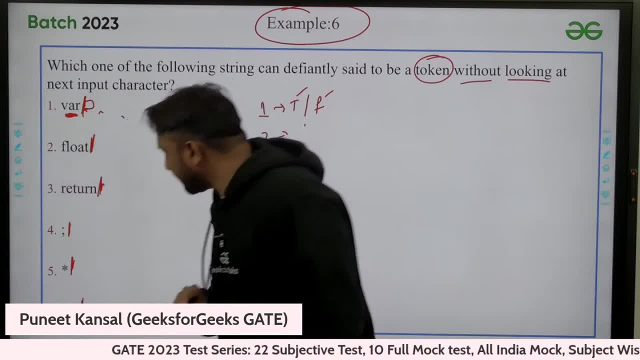 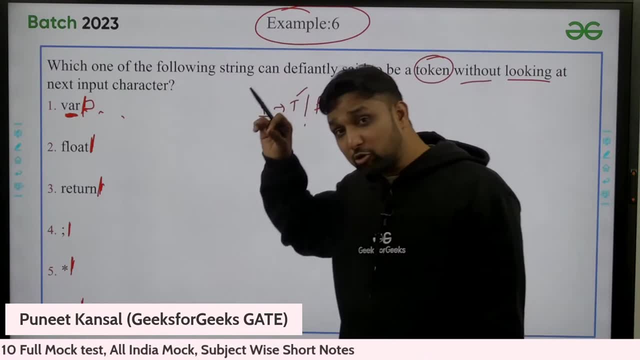 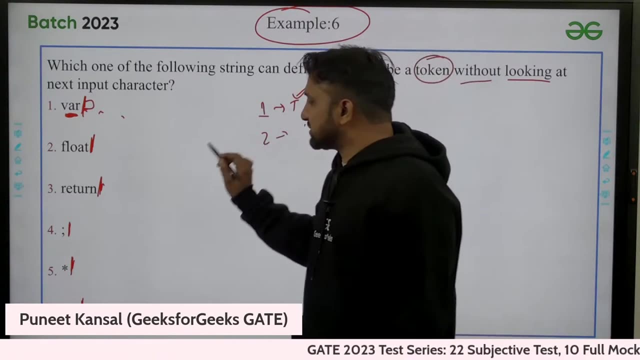 maybe here, here, next vector, without looking at next character, which of the strings here i can ensure that, okay, this is a particular, this type of token. so if you can tell, then say true, i can tell. otherwise, said false, i i cannot tell. without looking the next next. 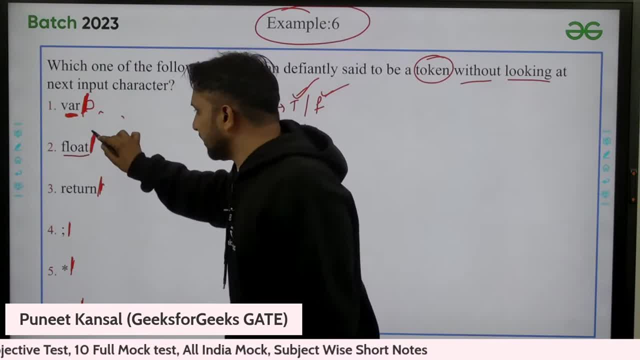 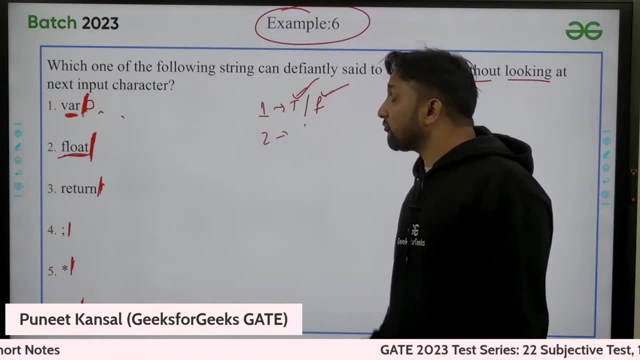 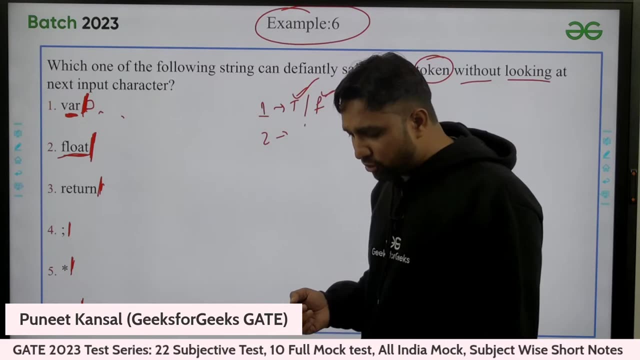 after? what is the next factor here, after, after this plot? if i, if i am not able to read what is after this, can i tell what is this plot is? is this is a token or not, or what type of token is this? can i, can you surely tell this thing? so i hope you understand the question. if you don't understand, 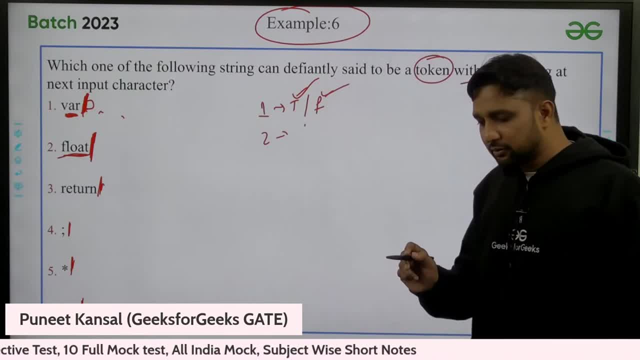 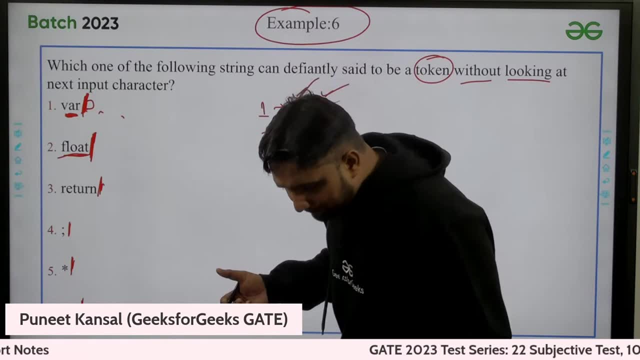 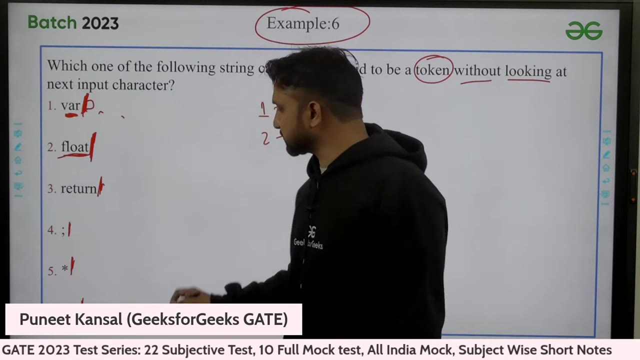 you can ask this thing also, sir. i don't understand. you can completely ask, sir, i don't understand the question, or you can ask something, but you don't understand. please let me write his name. six is not visible. that is plus plus. six is plus plus. let me write six here. uh, let me write sixth here. sixth option is: 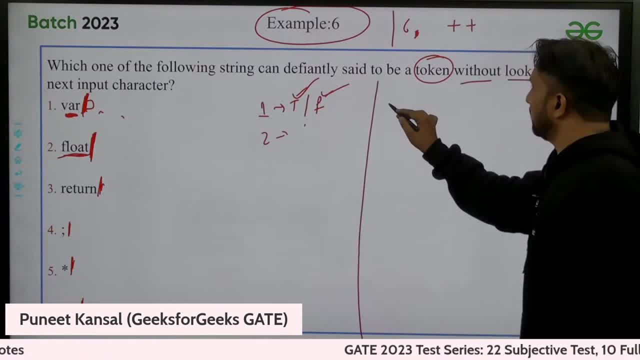 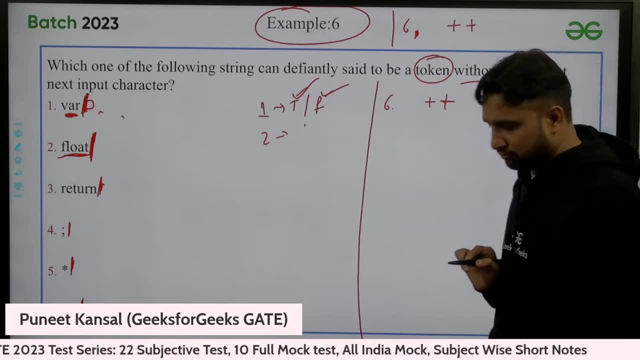 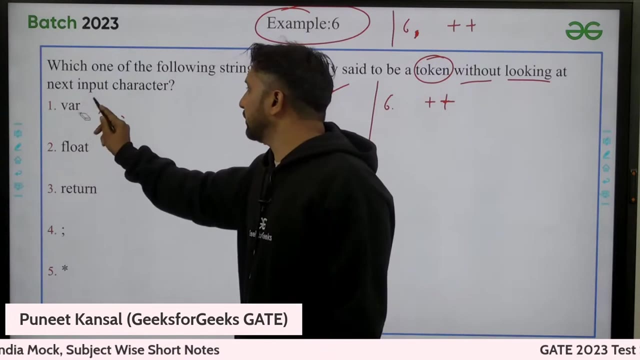 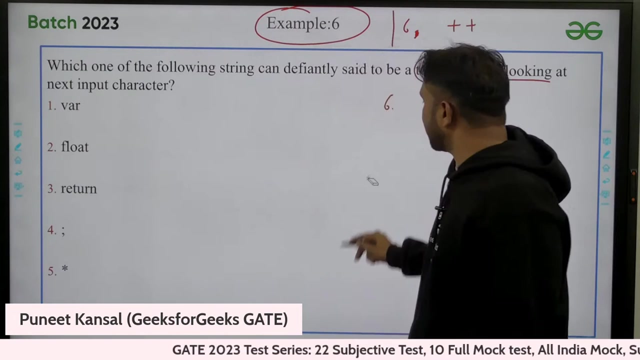 uh, let me write: six is plus plus. so let me write here: six number is plus plus. please try it. what is important is: you are trying or not. that is important, important, let at least. let let at least make sure that we will clear the gate, exam at least. 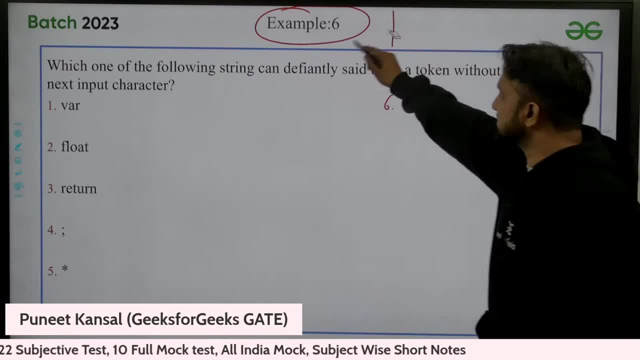 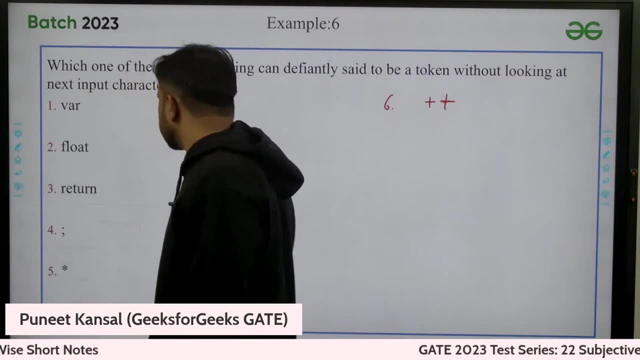 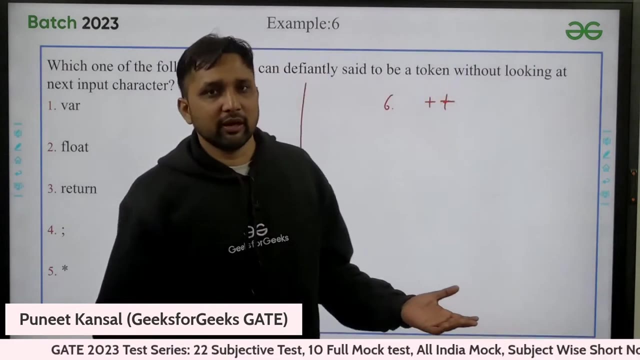 clearing the gate exam. we will ensure with this series. I am not giving you the surety for 60 marks from this series, but I can ensure you because we are covering the most important topics only, which are every year is coming and we are covering everything. we are writing. 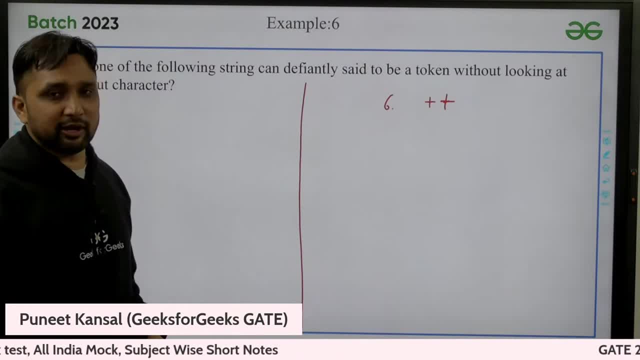 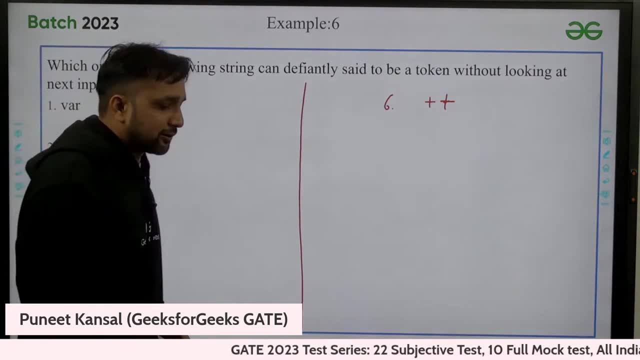 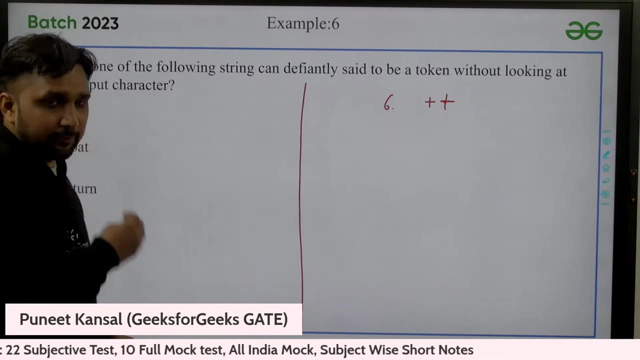 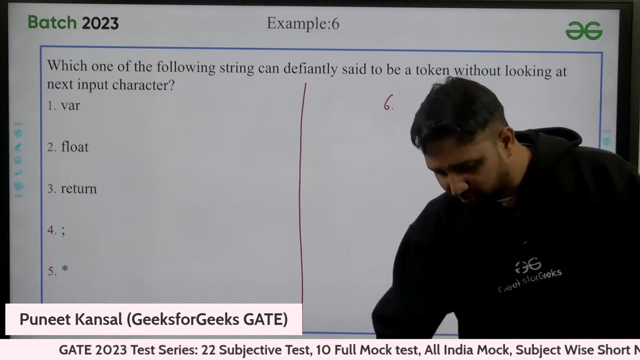 complete over there, otherwise no every anyone can claim claim on us how you are writing complete. we are not completely covering the topic. GFG cannot do like that geeks or geeks cannot do, cannot give the false promise that is a brand. so so please try write the answer, everyone, please try. right or wrong doesn't matter at all, right? 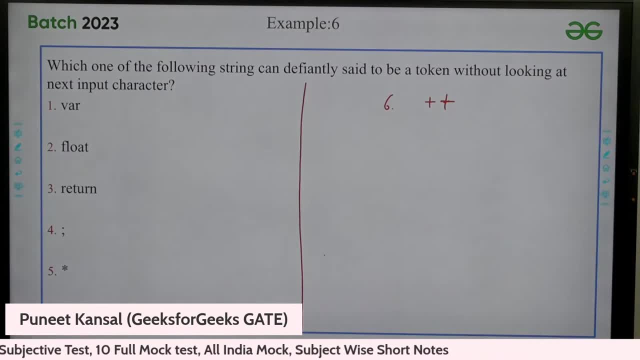 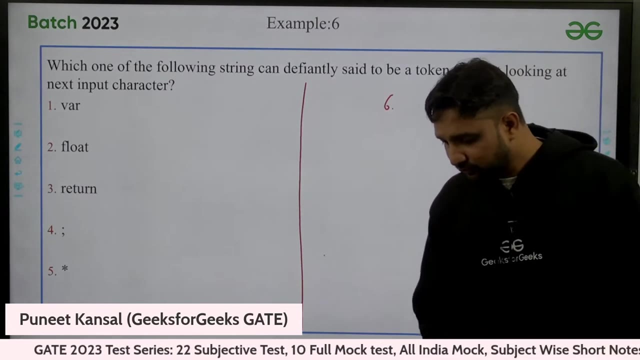 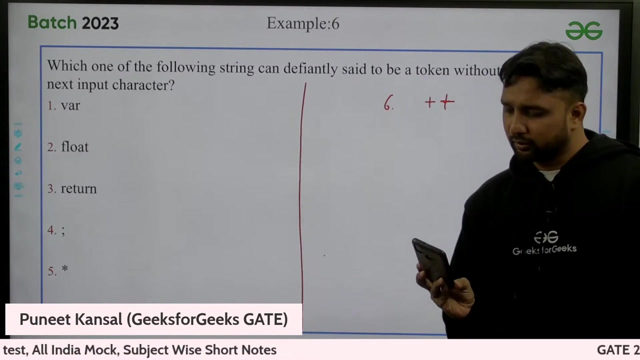 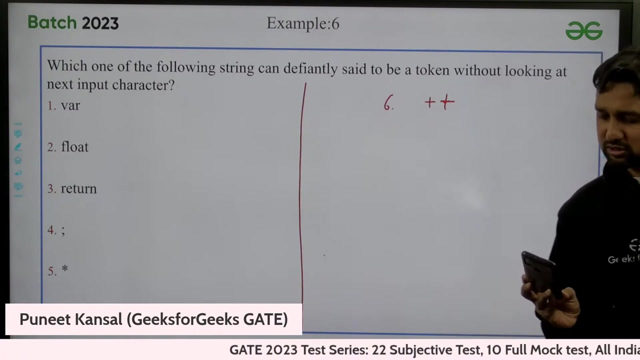 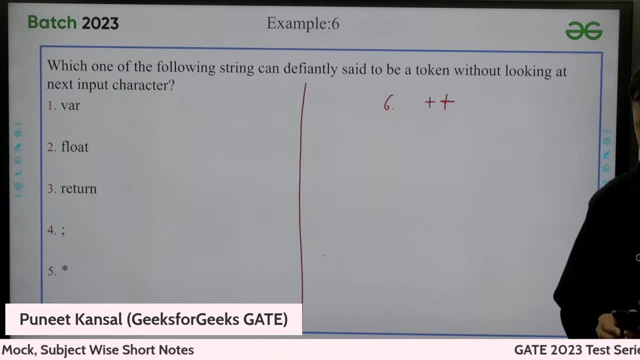 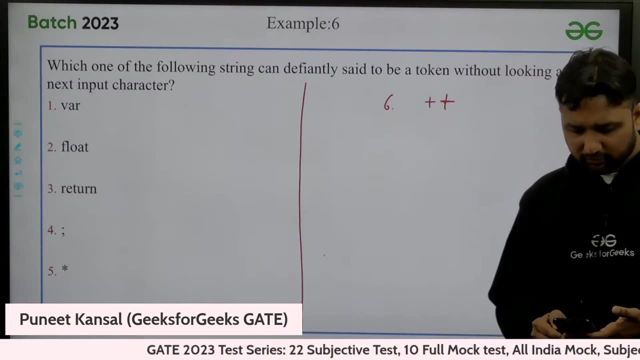 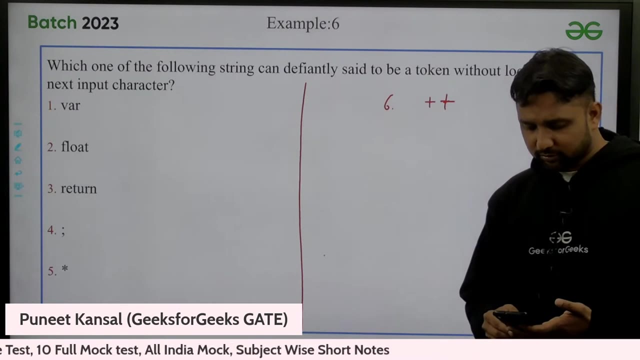 about dividions 0 to 0: 0. this through to to. you are saying the fourth and the 6 or false, and cover it. you also have and cover you also writing 5. what is 5 means 5 is true. So let us check out and this is: 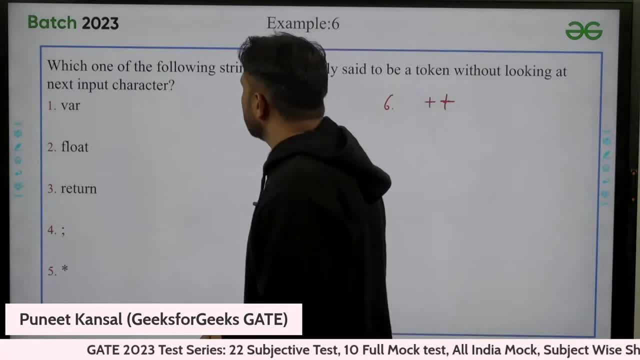 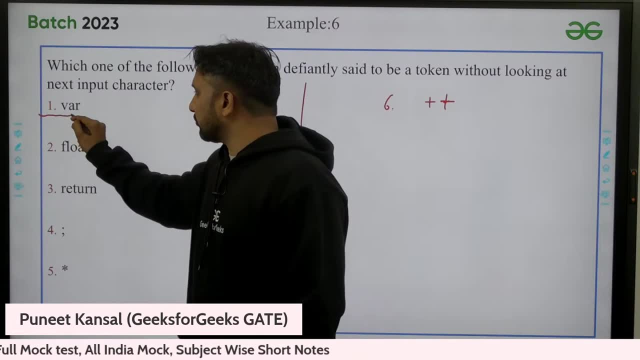 the last question. after that we will cover the gate questions. So we are. we are saying that our lexical analyzer is moving from here moving on, moving on, moving on character by a character, that is, scanning character by character. after reaching at here, at R, he is: 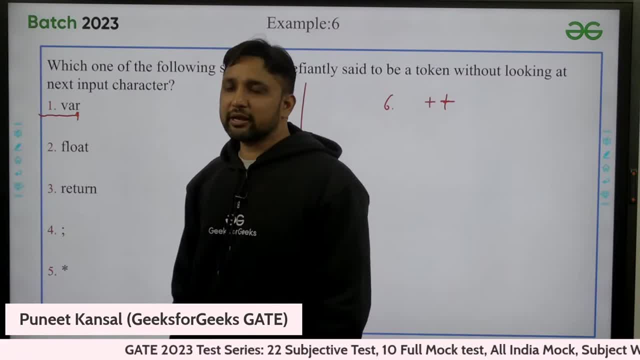 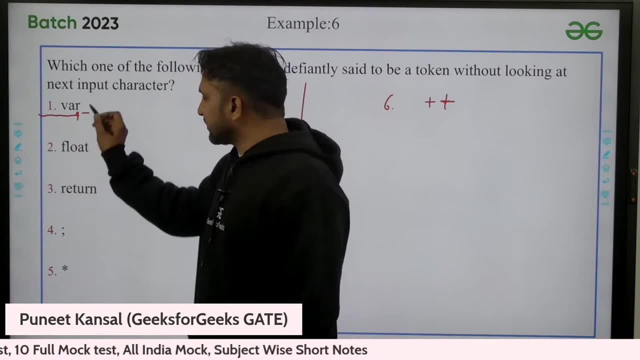 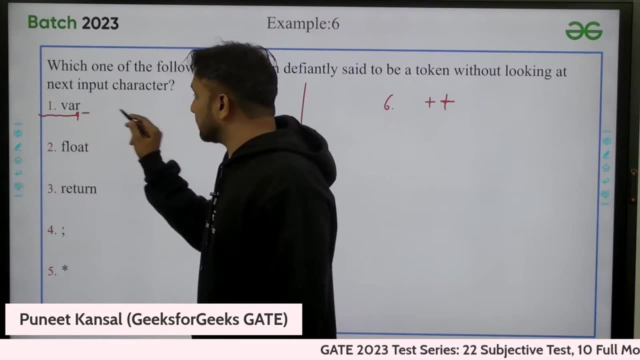 not allowed to go further. see, he cannot decide. he cannot decide where is the identifier. he need to scan the next character. after scanning the next character, if he find out there is a space here, there is a space here. if there is a space after, where? then this is an identifier. 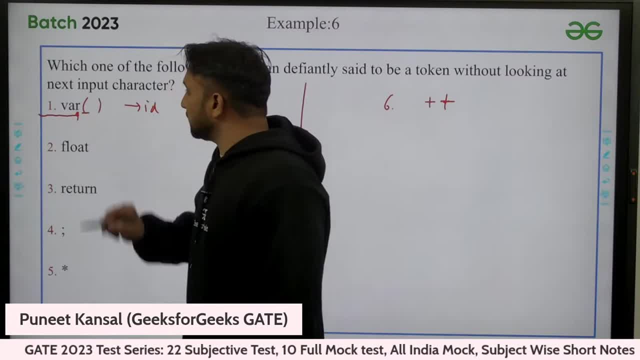 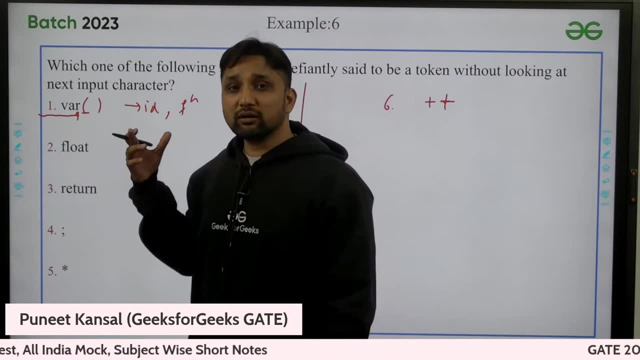 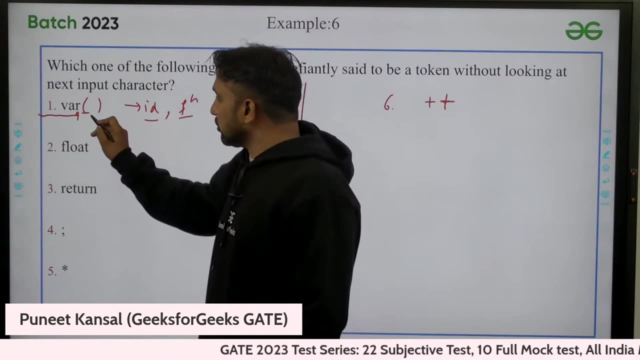 but if there is a, if there is a bracket here, Then this will be taken, become a function, okay, and maybe that can convert it to some keyword also. i don't know, maybe there that that can make some keyword, at least that can make these two things. so until unless i cannot, 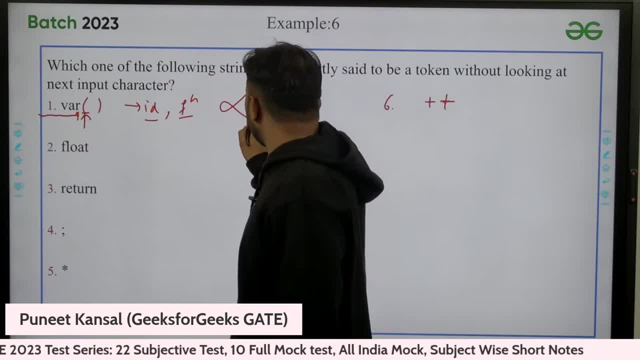 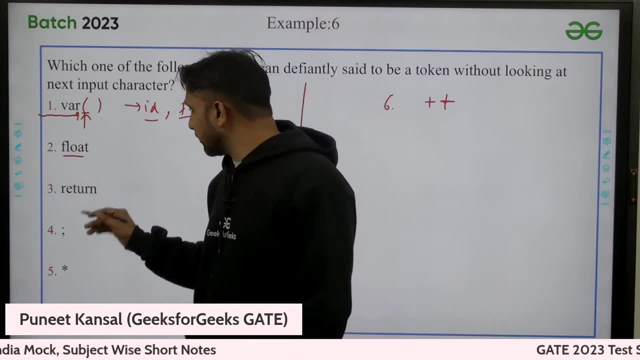 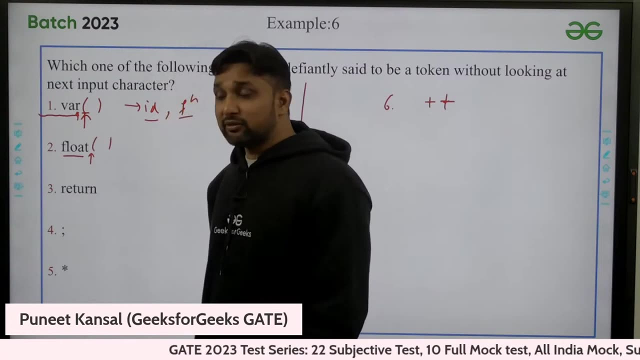 look at here i cannot make sure. so this is false. i cannot identify. i cannot identify here. same the reason here: after float, this is a keyword. no doubt float is a keyword, but without looking at the next character i cannot say float is a keyword, because maybe there is a bracket here, if there is. 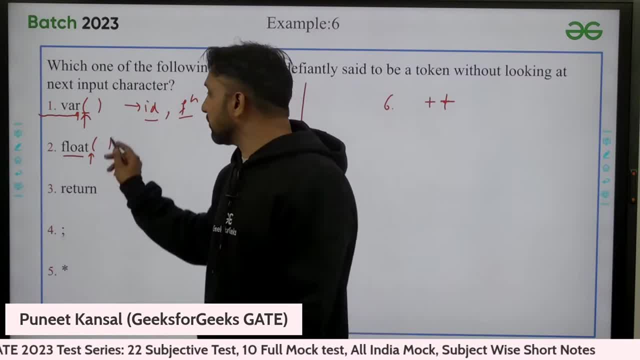 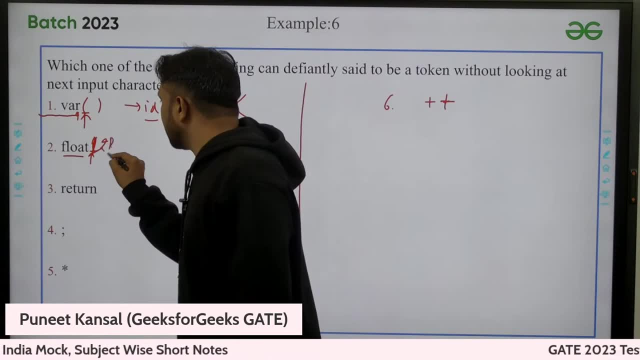 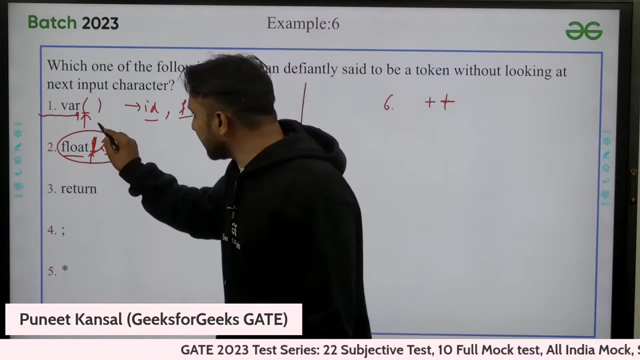 a bracket. now this is not anymore, is a keyword, this become a function, this become a function. or maybe, after float, i get float one, i write float one, two, three. so now this become a variable, this become a variable. float one, two, three. this is not anymore a keyword. so, without looking at this, 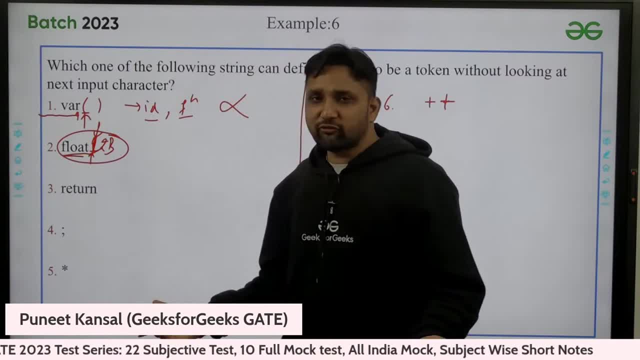 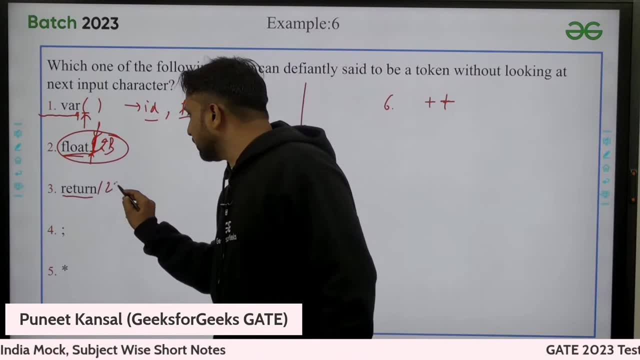 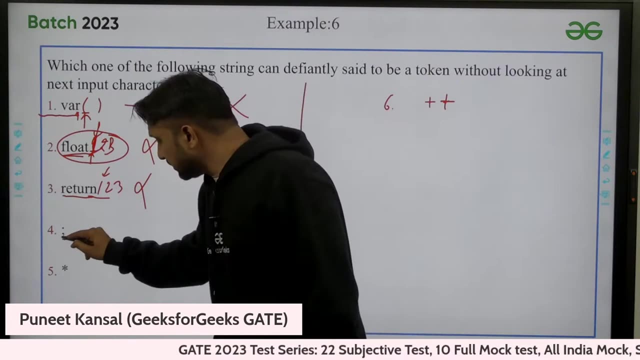 particular. next character immediate after this, i cannot find out. which type of token is this? okay, and what about? this? same reason apply here also. i can write one, two, three. now this become a variable, without looking at next character. i cannot say anything here. also, what about this? see after this semicolon. after this semicolon, nothing happens in c, if you see. 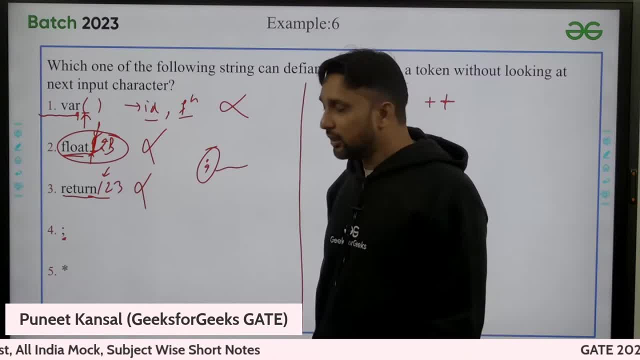 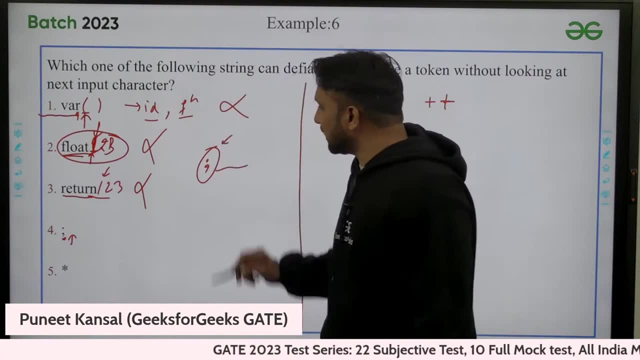 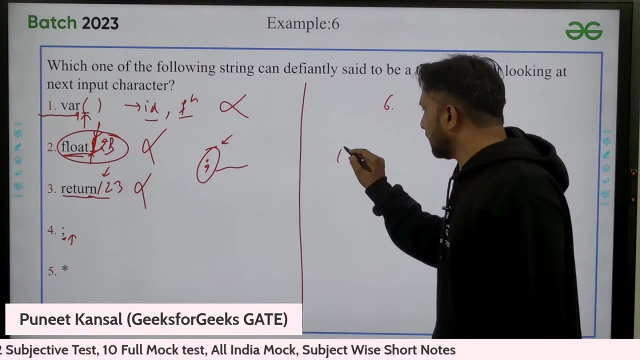 that we terminate every statement with semicolon only. okay. so here, even we do not read the next character, even we don't read anything, i can say that this is, this is a token, this is a semicolon token, this is a that's what. let me write one statement. can you tell me what the meaning of this? i equal to 5. 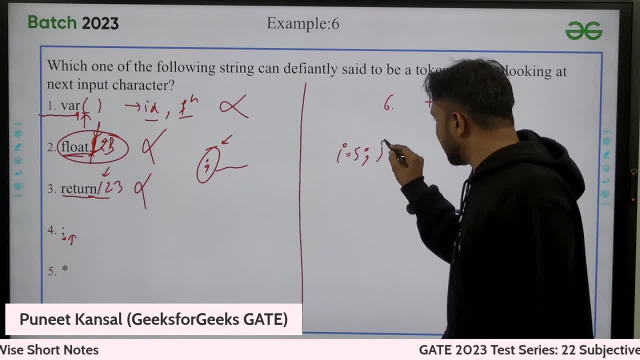 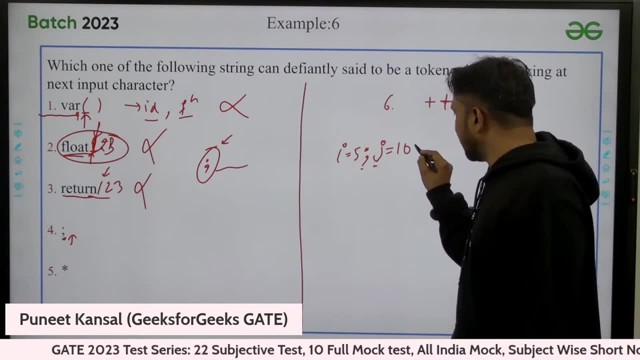 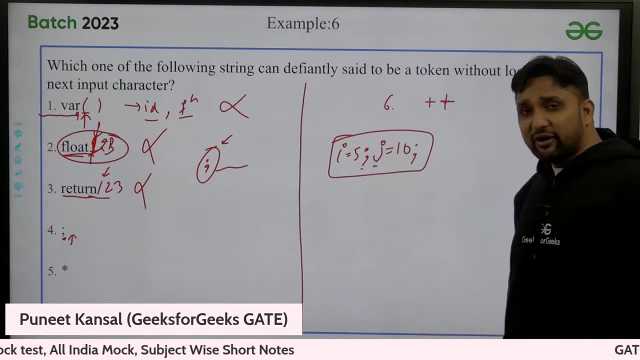 now i'm writing c. this is in c. i'm writing j equal to 10. immediately after, immediately after semicolon, i write j equal to 10.. so is this will give some error in c? no, this will not give error in c. this will completely find executed. 5 will be stored in the i. 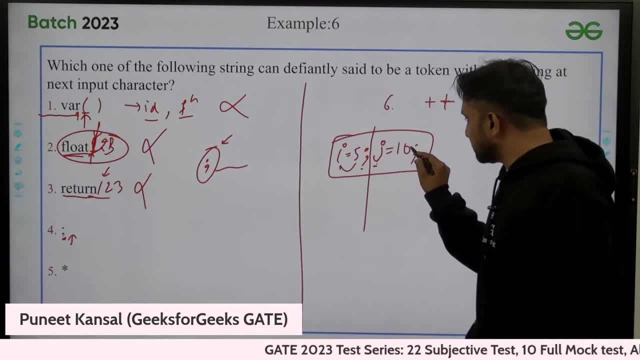 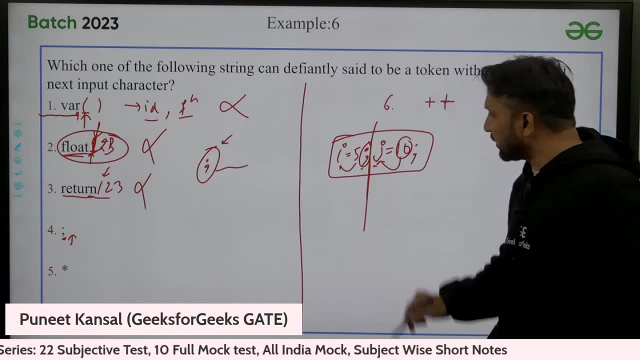 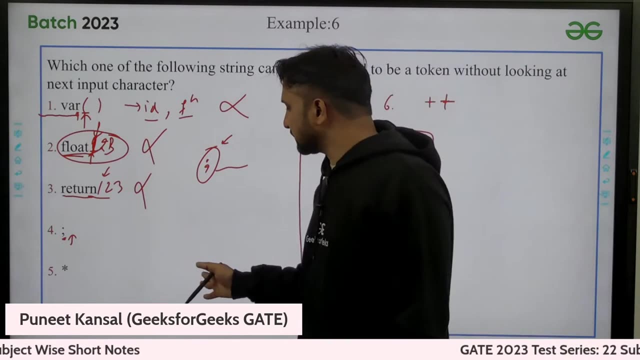 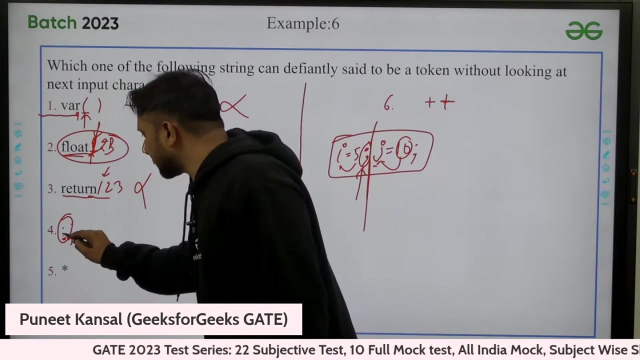 and the statement will terminate and j 10 will be stored in the j. okay, so this semicolon is sufficient in itself. we do not need to look at the next character. this is showing the end of a statement in c language, okay, or c plus plus or java. so this is sufficient in token in itself. so, without looking at next vector, i can. 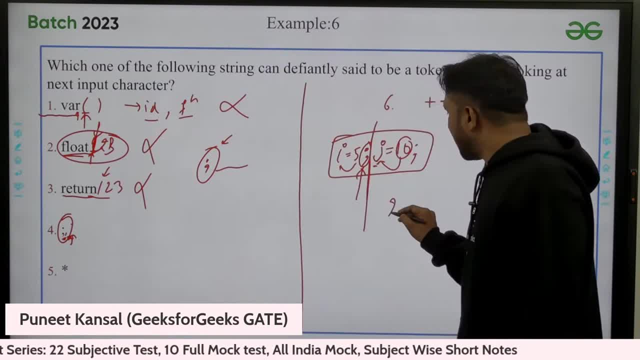 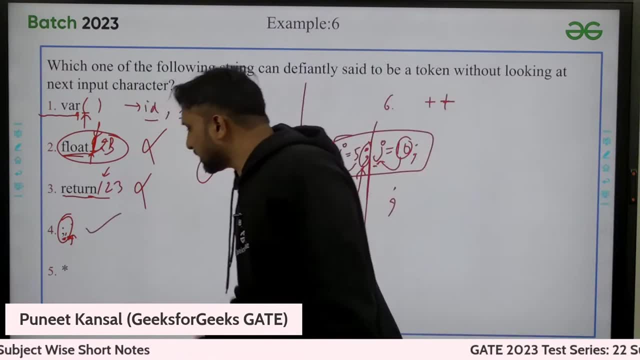 say: okay, this is a token, because this is not making any other, any other other, this is not using, instead for simulating any other, any other symbol and making something else also okay. so, yes, this is a. i can say that without looking at next, next after, i can say: this is a token. what about this? 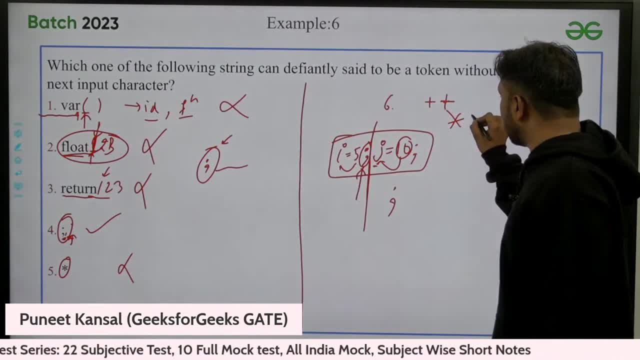 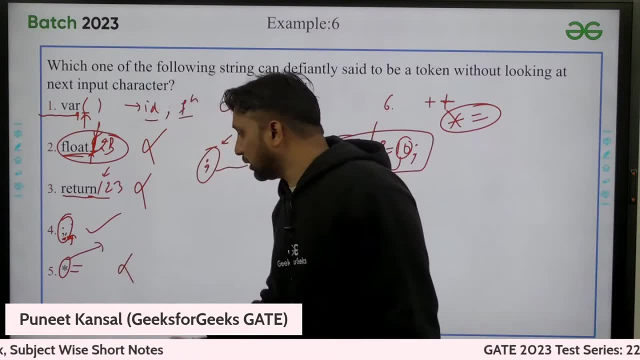 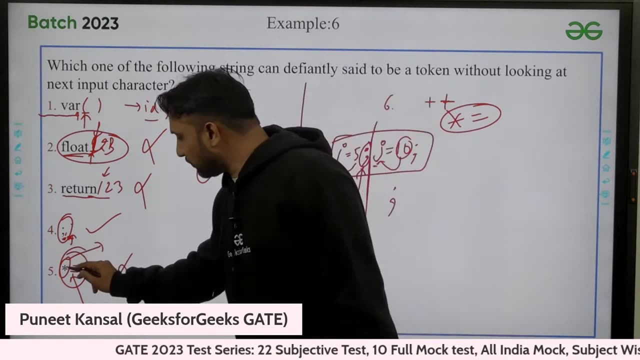 here. i cannot say why, because there can be. there can be multiply equal to, there may be equal to after this, if there is equal to after this. now this is not more a token. this is a token now. this is a token i i need to look at here. i need to look at here. 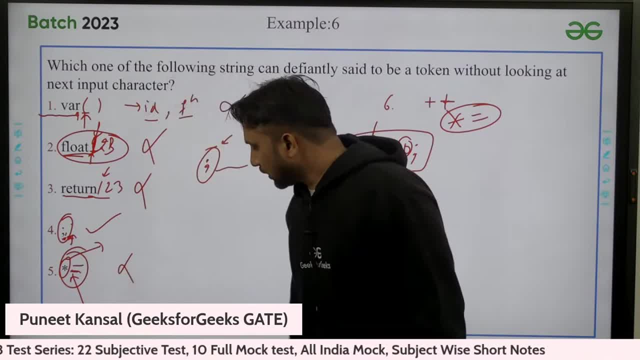 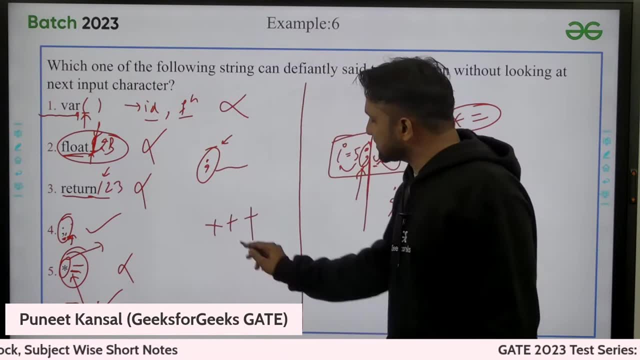 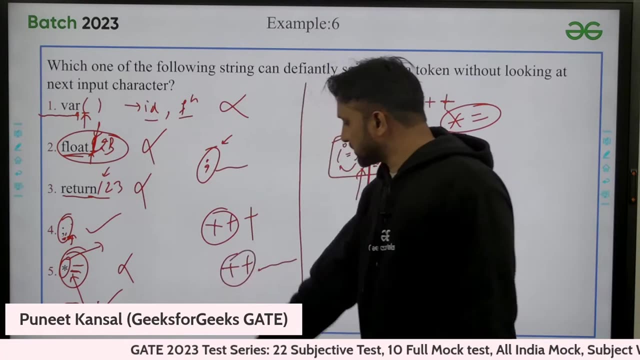 making a statement. okay, i need to look at here. and what about this? this is a token. why this is a token? because even i have one more plus. still, this will remain a token. whatever you can write after this, whatever you can write, that will not bother this, this person, and this is a token. 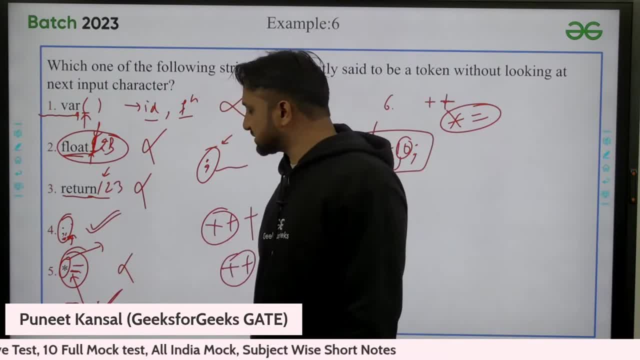 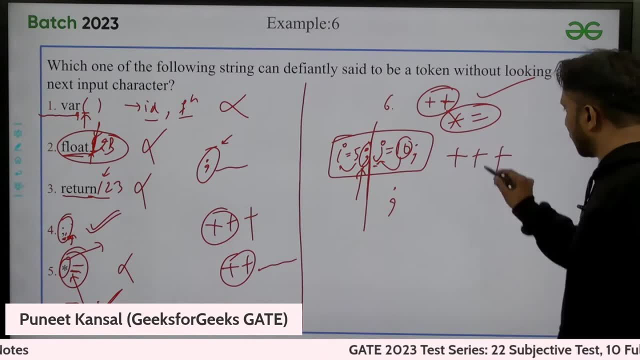 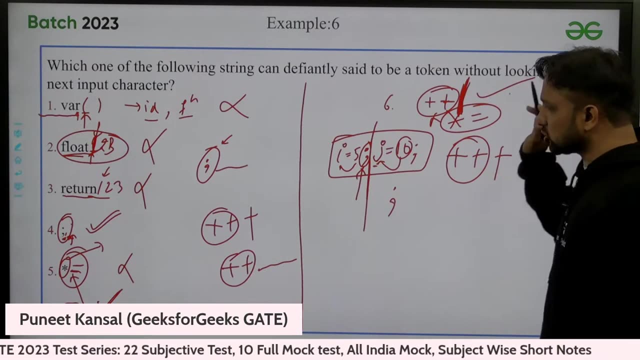 actually yes. so fourth and fix six. fourth and sixth. i think six is not visible. so six is also a token, because after plus, plus, if i'm writing one more plus still, this will remain a token. i do not need to bother about what is. what character is coming after this. so six is also right. fourth: 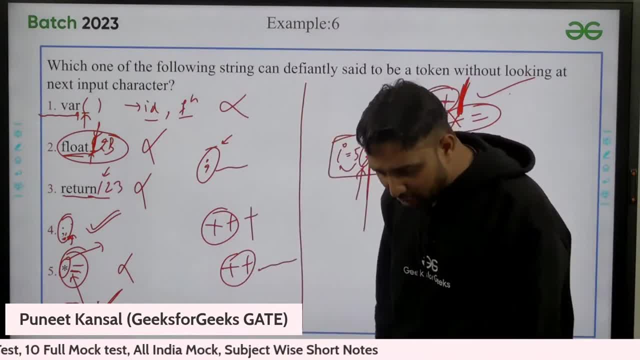 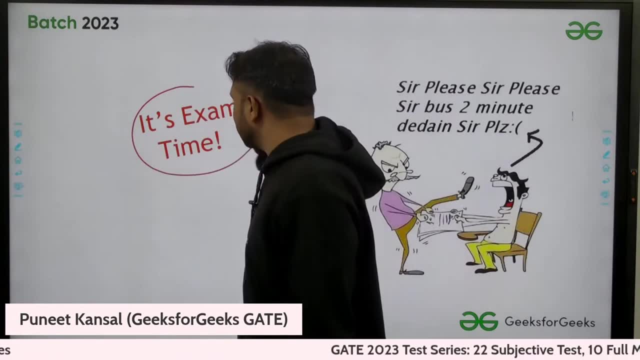 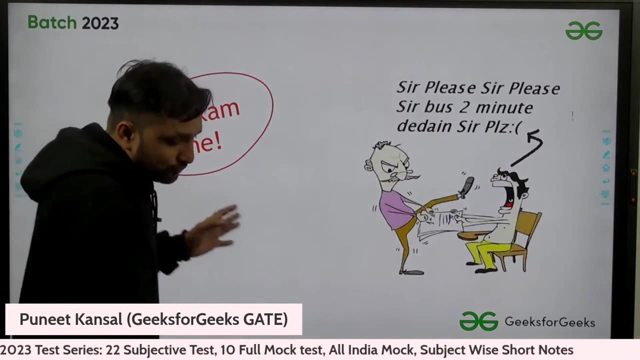 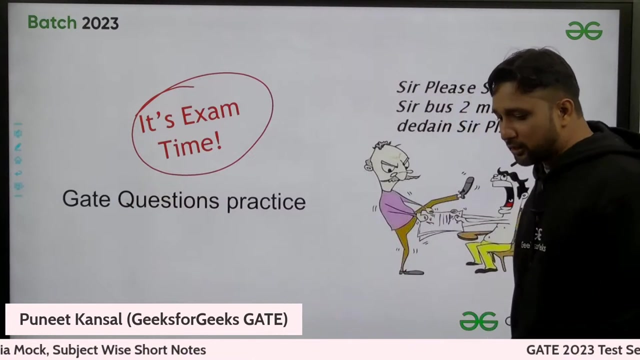 is also right. all others are false. any doubt? please ask any any doubt? please ask otherwise. now it's your exam time, it's not my. now we have covered everything about the lexical analyzer. you people need to solve the gate questions, so get questions. we will do right now. 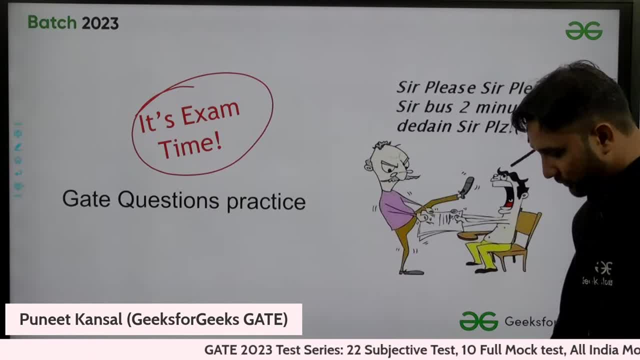 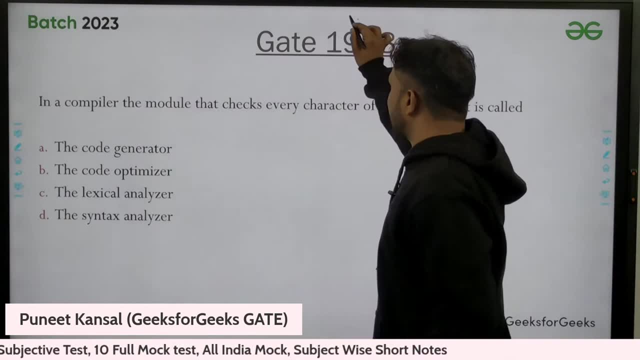 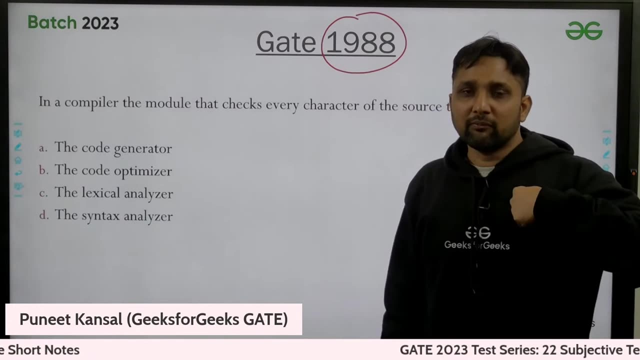 so let's move to the first gate question, gate 1988. please try it yourself. if you will, you people will solve the question yourself. you will get the confidence. if i will solve, believe me, you will not get the confidence. please try to solve this question now yourself. 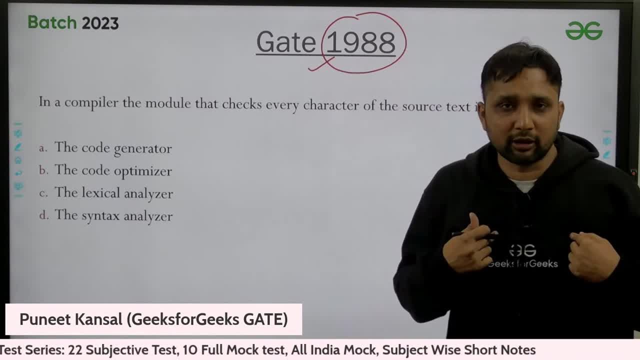 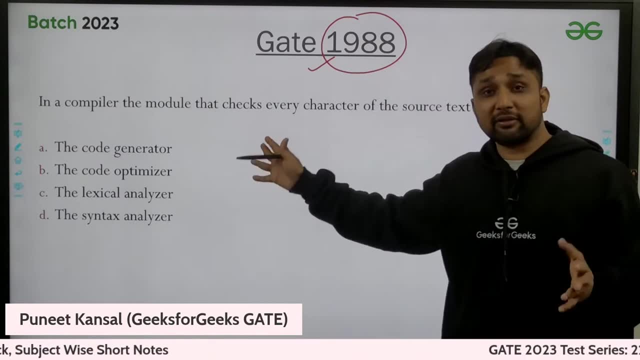 these are gate questions. these are not designed by me or any of any of us from geeks for geeks. these are gate questions, so this is the level you need to achieve: actual level. these are the actual questions you need to solve in exam. so i'm going to cover many questions. please keep keep trying. 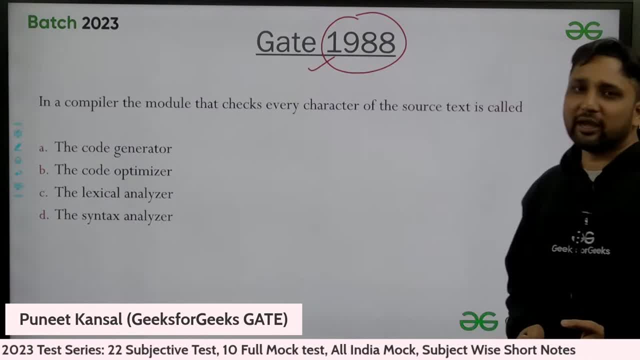 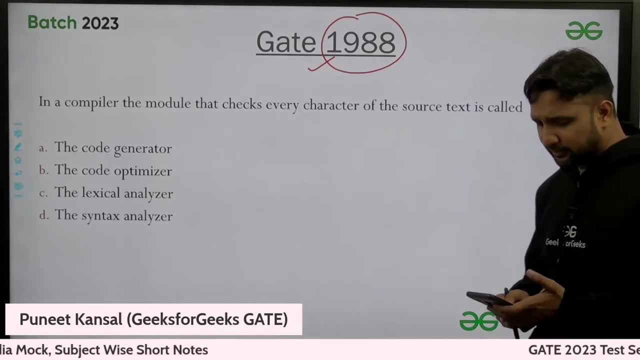 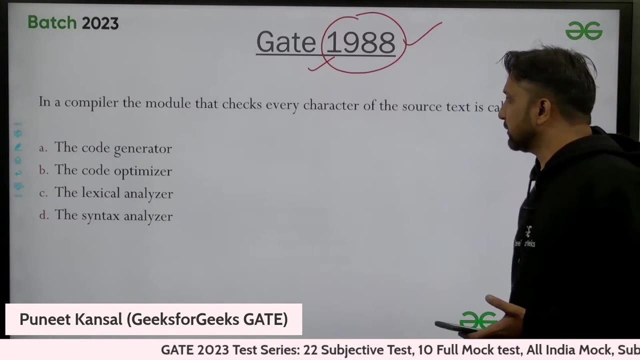 all these questions yourself. please try them. wrong or right. again i'm saying: doesn't matter wrong or right, doesn't matter right now, that doesn't matter. please try it. that's why you people are here. that's why you people need to raise your level up to these questions. please try it. 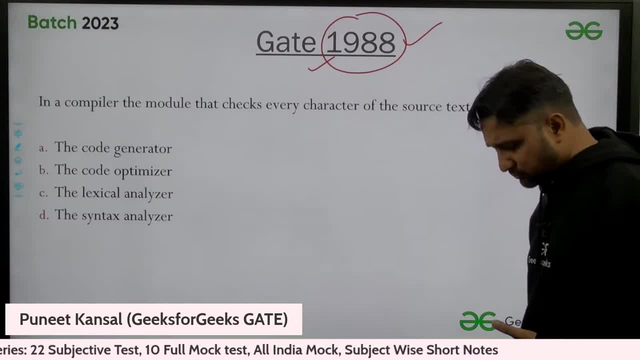 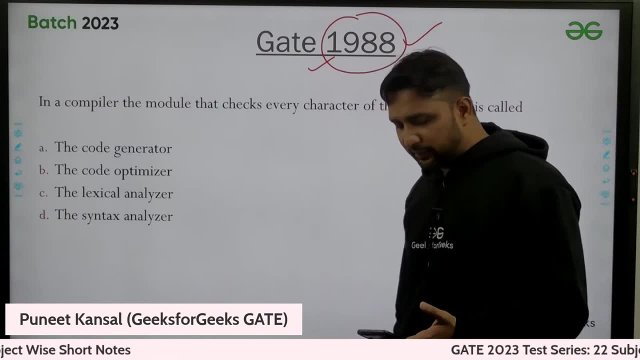 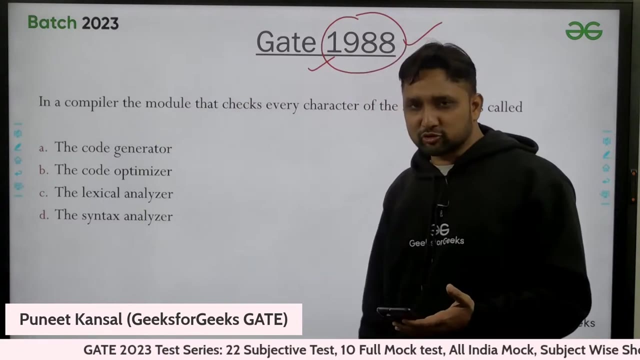 everyone, please, everyone, all, all people. please try it, please. please give the answer in the chat box now you are solving, uh, i'm, i will increase the level of their difficulty also, don't worry, if you are too much comfortable, don't worry, we have too much comfortable, don't worry, we have too much comfortable. don't worry, we have. 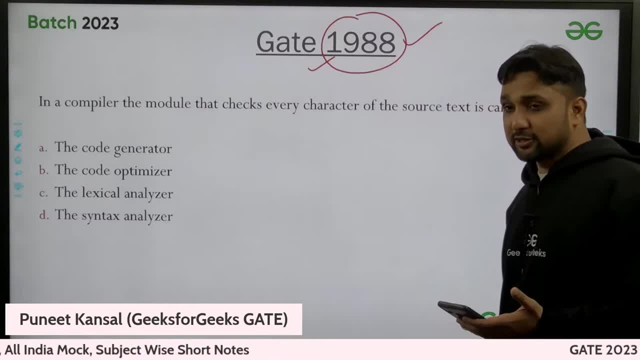 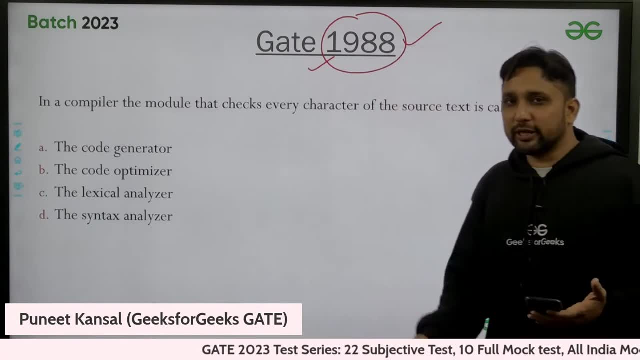 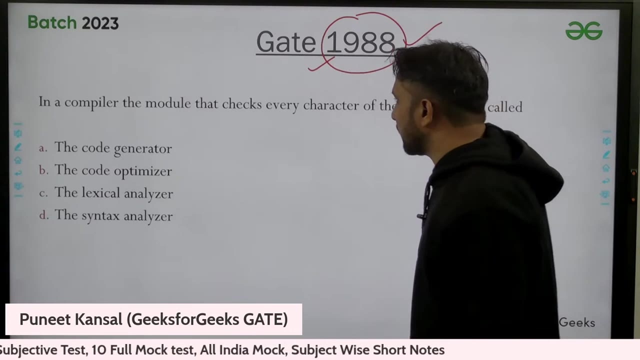 higher level of questions also here. but one thing is sure: you will be able to solve all the questions. these are: uh, they can make little bit modifications and all that, otherwise they cannot change the concept. so maximum people is giving the c answer and you people are right actually. 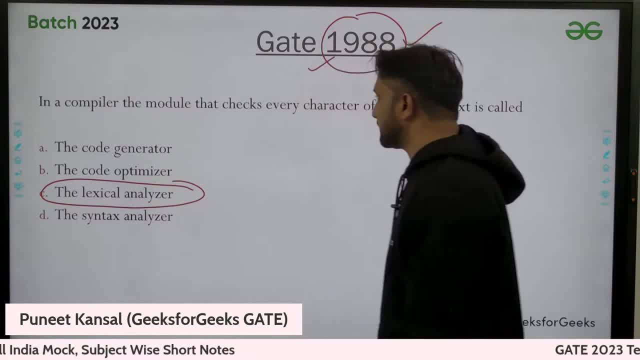 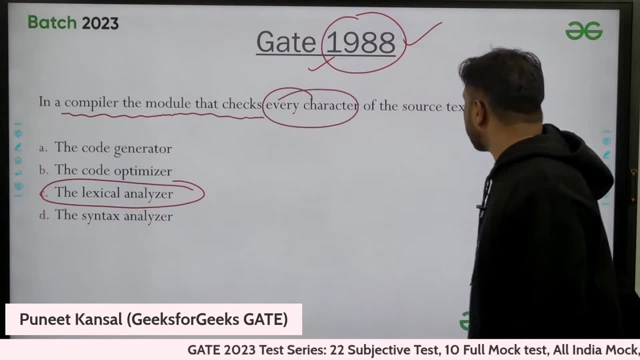 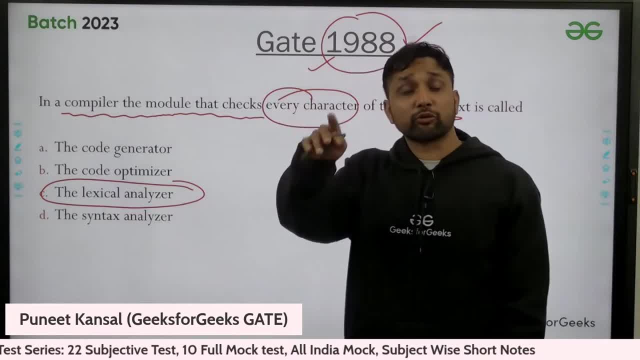 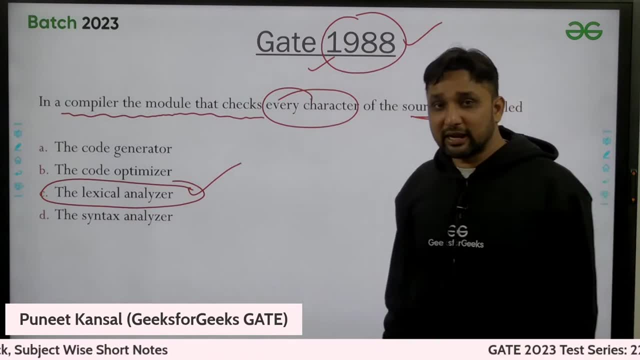 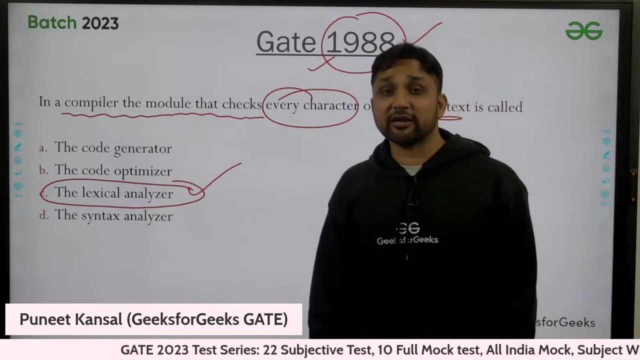 who checks the every character, every character note string? i am talking about character by character, character by character. that will keep moving on. that is done by the lexical analyzer. okay, that scan character by character. who is scanning character by character? there is a machine which is working behind that, which that that is finite state machine, actually finite state. 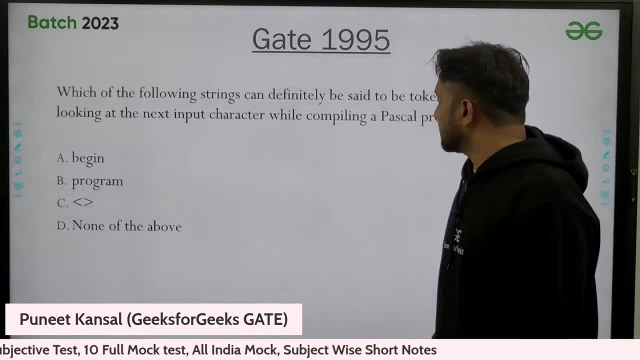 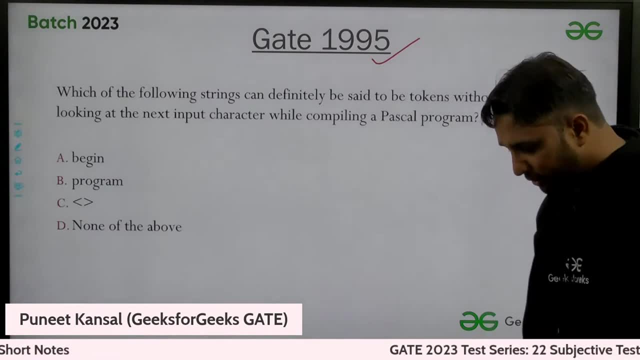 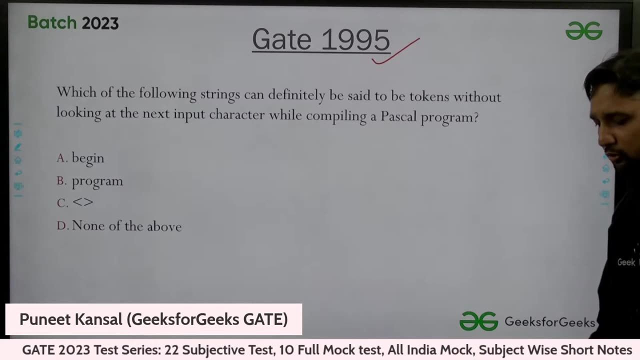 automata is working behind the lexical analyzer. second question from 1995. please keep trying these gate questions. that's why you people are here. that's why you people are here. that's why you people are here. you need to raise your bar right in the chat box. everyone, all the people. 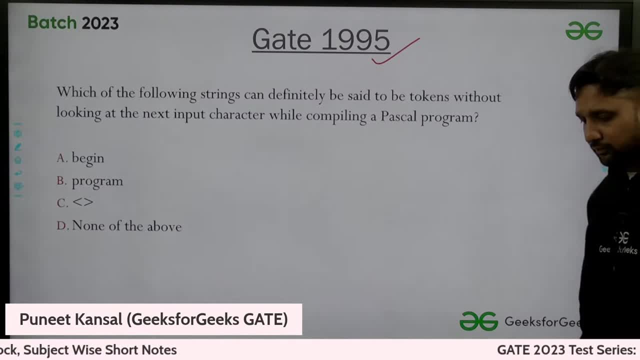 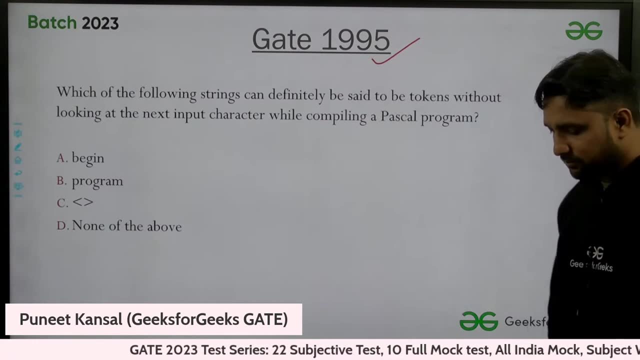 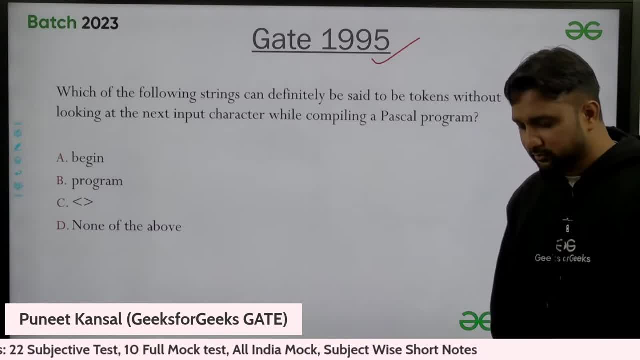 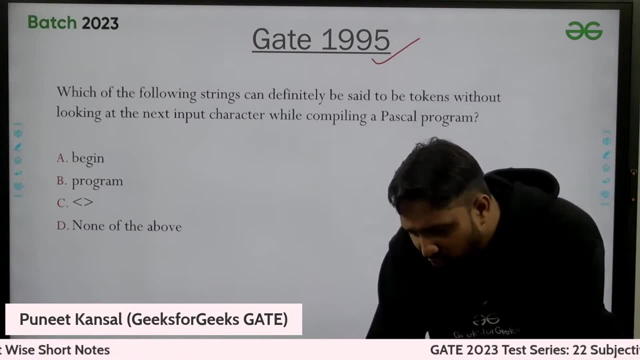 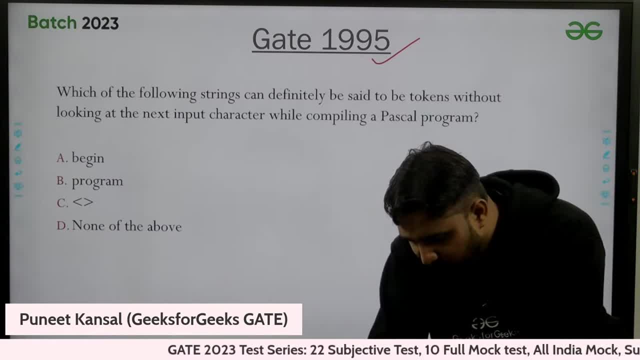 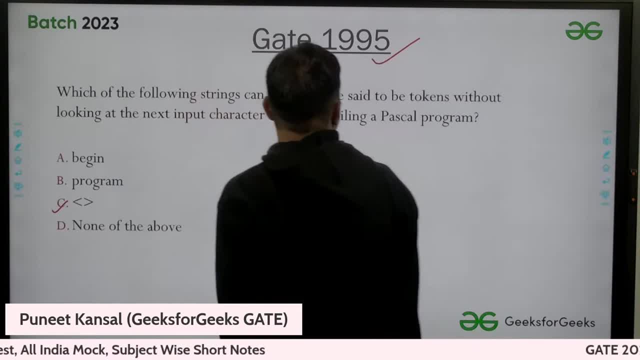 so all people, you people, all are. so all people, you people, all are right. the answer is c right. the answer is c right, the answer is c. and actually this is talking about, and actually this is talking about, and actually this is talking about pascal, and actually this is talking about pascal. 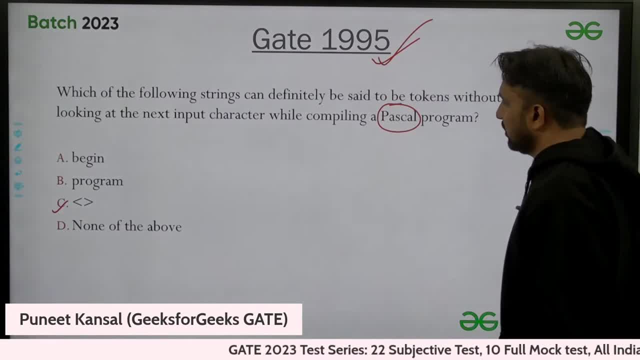 and actually this is talking about pascal language, language, language. this is the old question actually. this is the old question actually. this is the old question actually, but we are not that much bothered about, but we are not that much bothered about, but we are not that much bothered about this pascal language also. 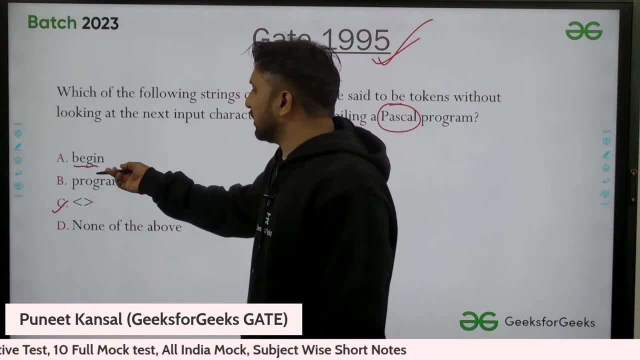 this pascal language also, this pascal language also, uh, this is actually keyword in pascal. but uh, this is actually keyword in pascal. but uh, this is actually keyword in pascal. but again, if again, if again, if i don't know, i can put something bracket. 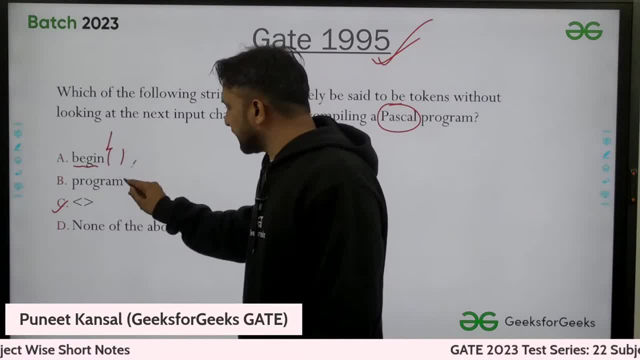 i don't know, i can put something bracket. i don't know i can put something bracket here and i can make it function here, and i can make it function here and i can make it function. so i need to look at next character next. so i need to look at next character next. 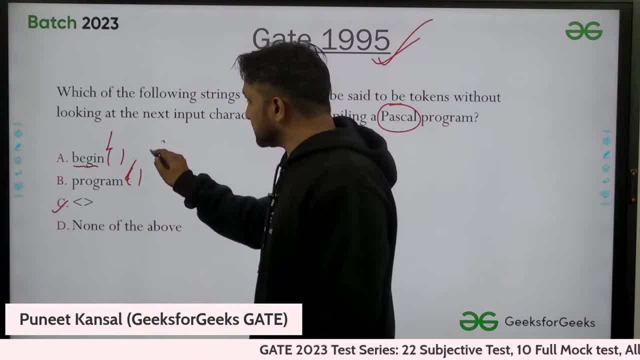 so i need to look at next character, next character, character character: here also this can also be a function. so here also this can also be a function. so here also this can also be a function. so these are wrong, these are wrong, these are wrong. this is a not not operator, not operated. 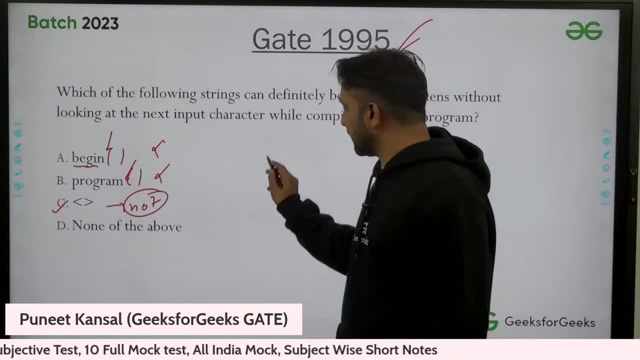 this is a not not operator not operated. this is a not not operator not operated in pascal. if you want to write not in pascal, if you want to write not in pascal, if you want to write not in pascal, then we use these angle brackets. 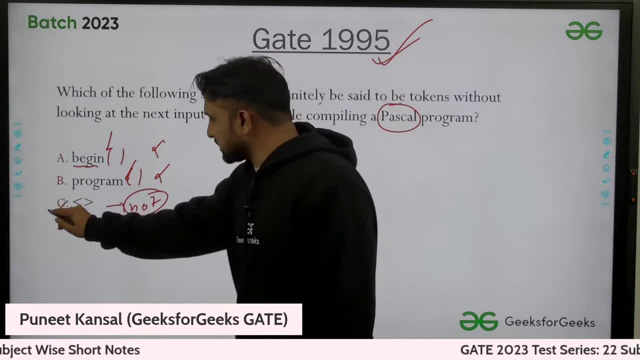 in pascal, then we use these angle brackets. in pascal, then we use these angle brackets. this is this means not. this is this means not. this is this means not, and so this is the right answer without. and so this is the right answer without, and so this is the right answer without looking at next factor here. 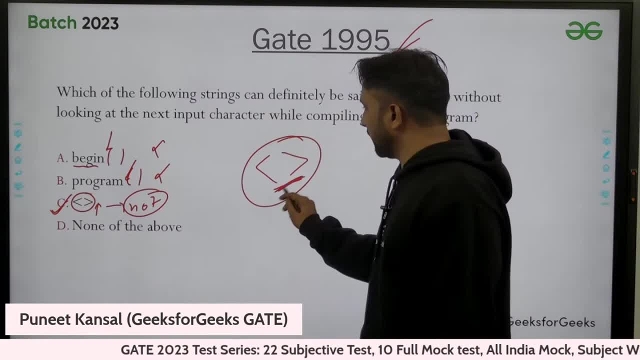 looking at next factor here. looking at next factor here, i can say that this is a token, this is a. i can say that this is a token. this is a. i can say that this is a token, this is a not, not, not- okay, okay, okay, okay, okay, okay. so let's move to the next question, this: 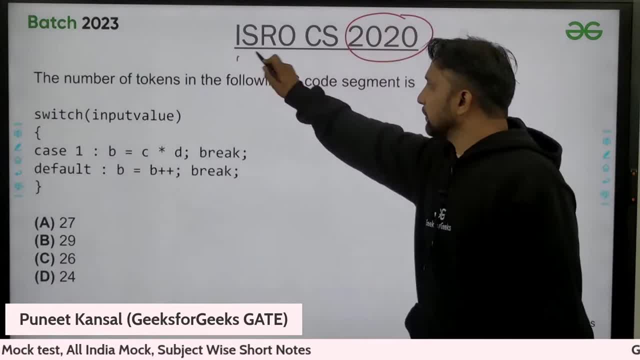 so let's move to the next question: this. so let's move to the next question. this is isro cs 2020 question. isro cs 2020 question. isro cs 2020 question. please try to solve it yourself, you people. please try to solve it yourself, you people. 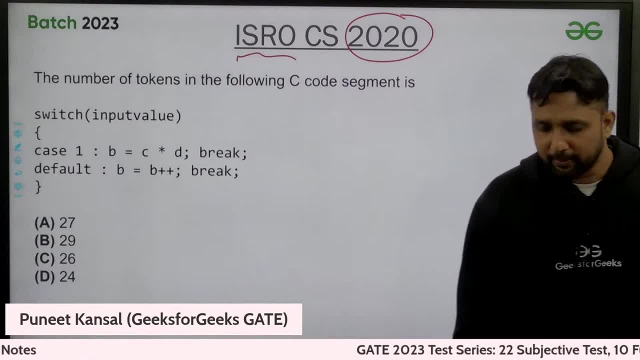 please try to solve it yourself. you people can solve it. you people can attempt can solve it. you people can attempt can solve it. you people can attempt all these questions, okay, all these questions, okay, all these questions. okay, you have covered the topic, that's it. you have covered the topic, that's it. 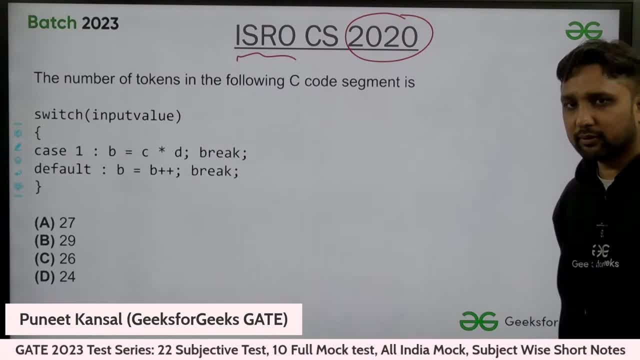 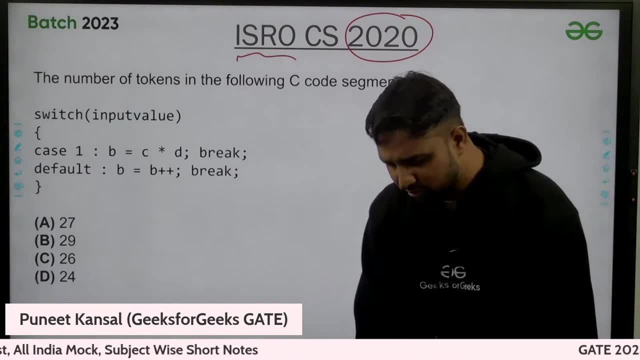 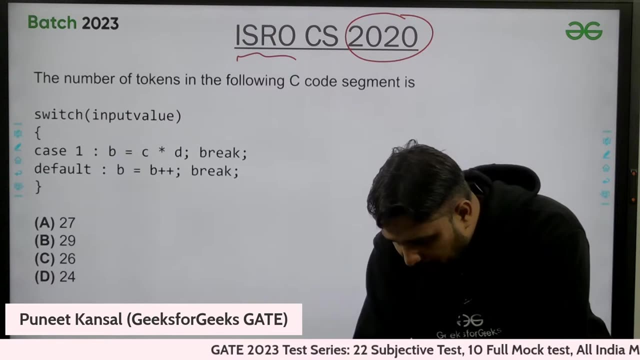 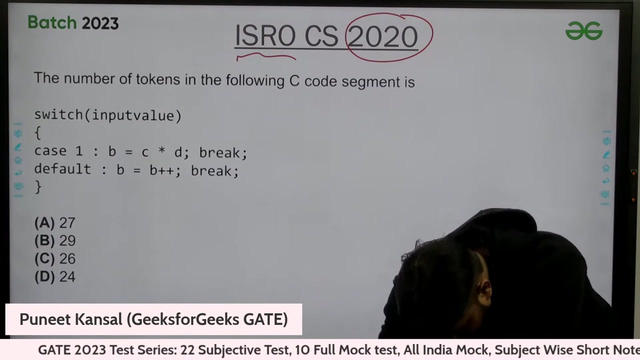 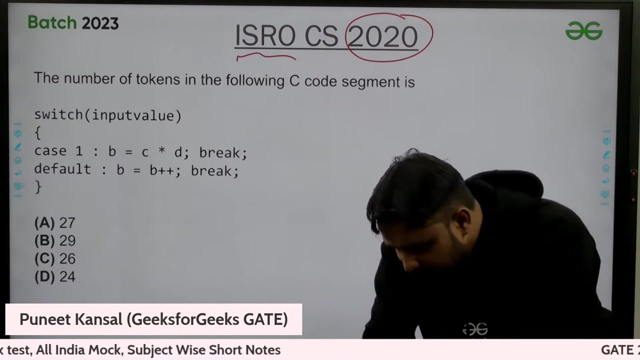 you have covered the topic. that's it. now you can appear for any exam actually. please write the answer in chat box. now you can appear for any exam actually. you have covered the topic, that's it. now you can appear for any exam actually. so, so, so, so. 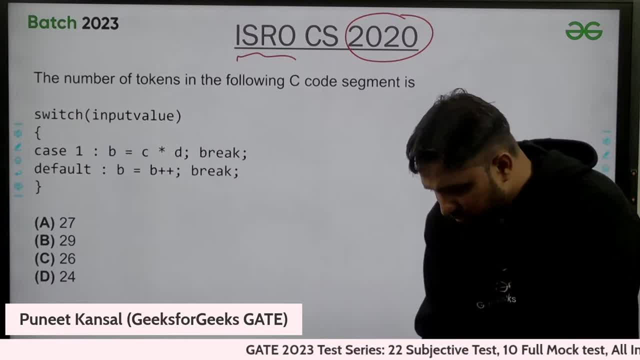 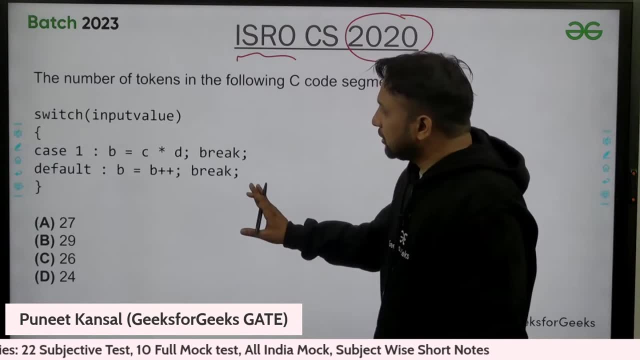 so, so, 26, we are getting from many people. i, 26, we are getting from many people, i, 26, we are getting from many people. i think, think, think, uh, uh, uh, uh, if, if you, if other people are trying, please keep trying it. see if i am explaining it and you. 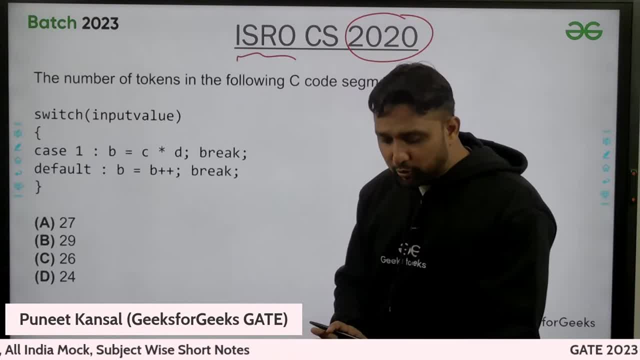 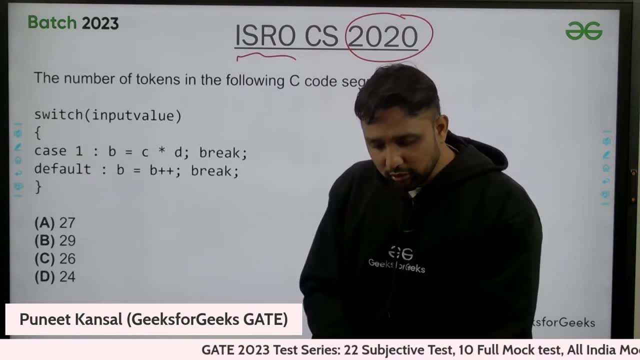 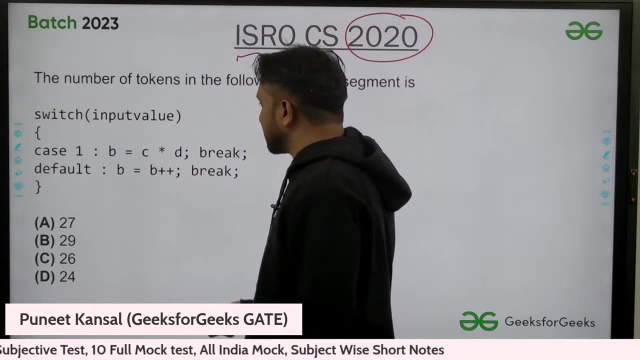 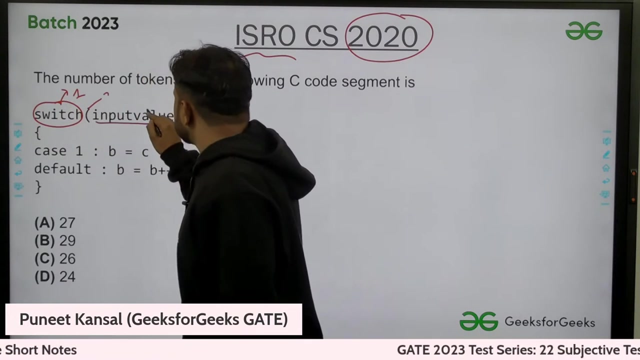 are still trying. please, you, you keep trying. okay, that is more important than whatever i was explaining here. the new information is not that much important as compared to if you are trying it yourself. that is more important, okay, so you must be right. actually, your finding is 26, so let me try also. this is one, two, this is three. sector token this: 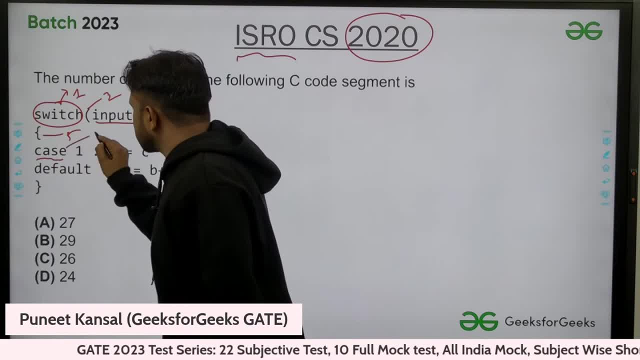 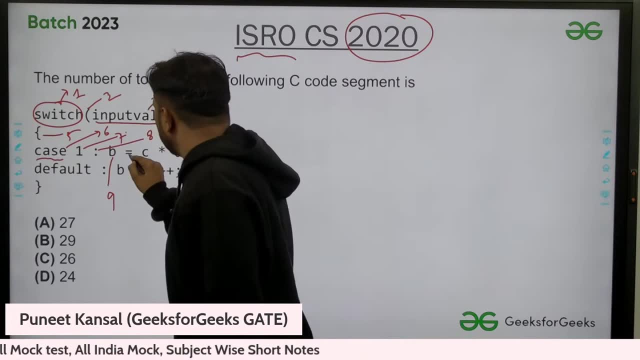 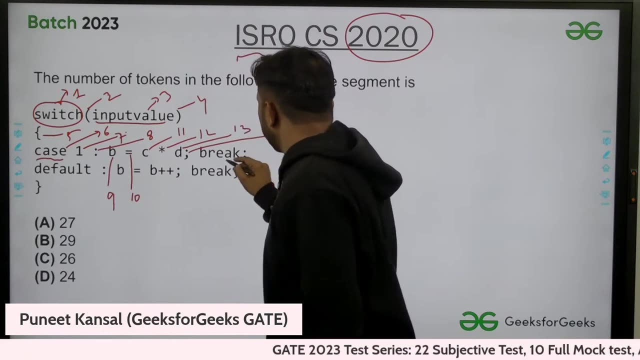 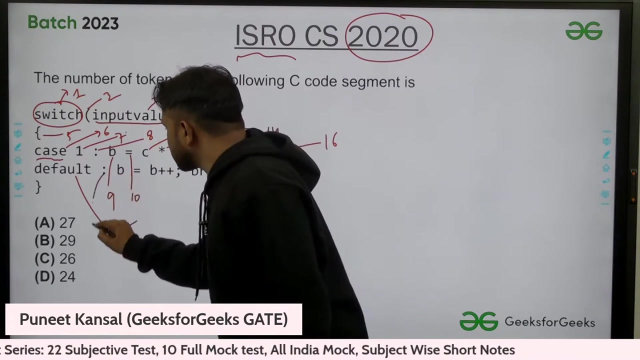 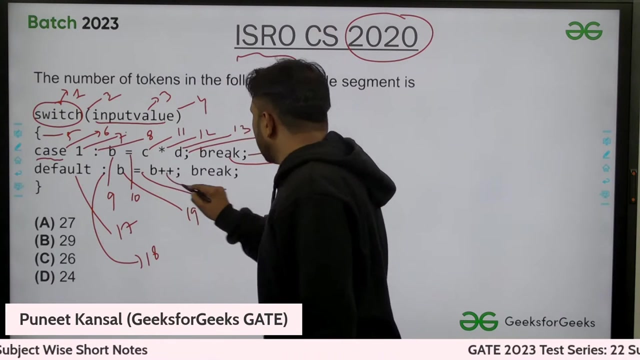 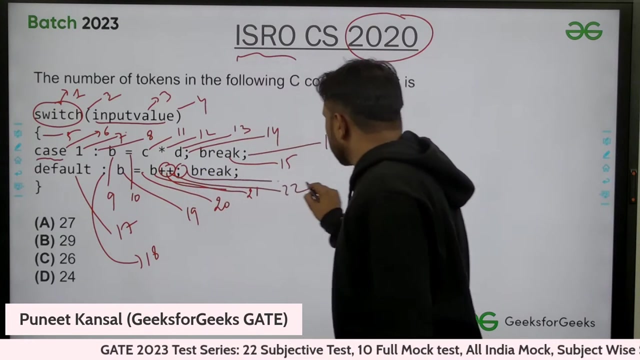 is fourth token, this is fifth one. this is sixth one. this is seventh one. eight, ninth, ten, eleven, twelve, thirteen, fourteen, fifteen, six, seven, eight, nine, ten, eleven, twelve, thirteen, sixteen. default is seventeen. this colon is eighteen. this b is nineteen. twenty b is twenty one. this plus plus is twenty two. this colon semicolon is twenty three. break is twenty. 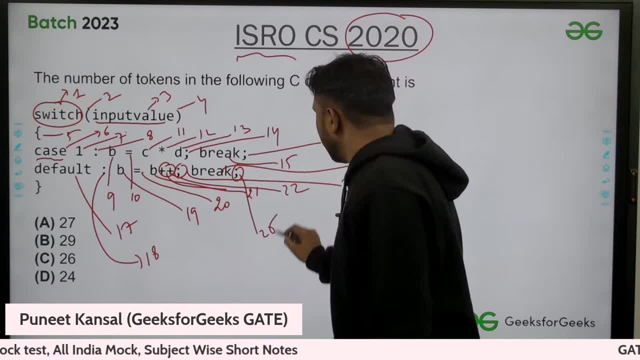 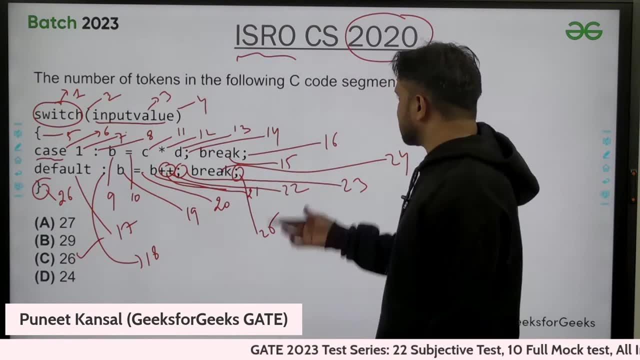 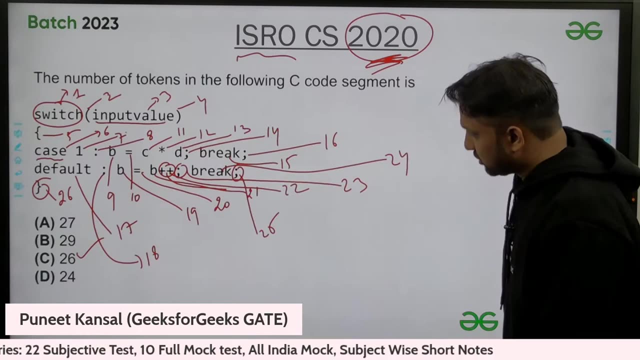 four, this is twenty five and this is twenty six. so you people are right, all are right, you are. this is not too much old question and you have attempt it. that is. answer is twenty six. that is c. you are right. let us move to the another. this is also: 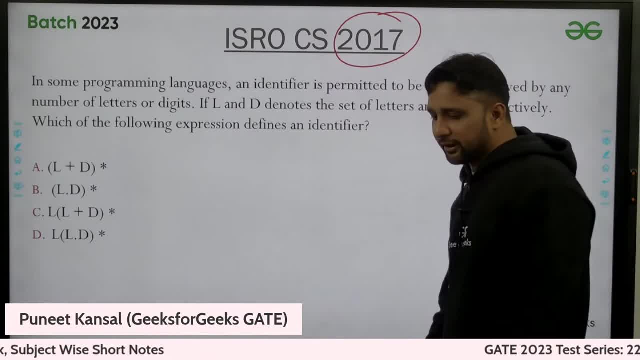 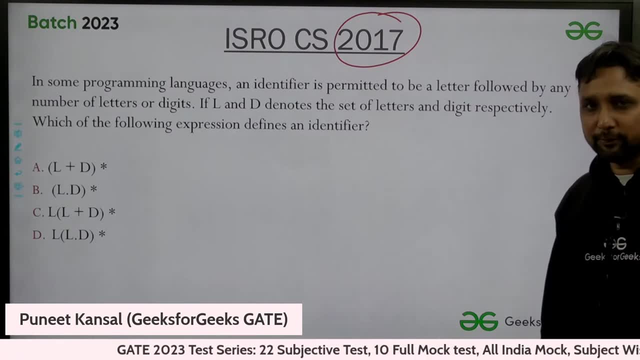 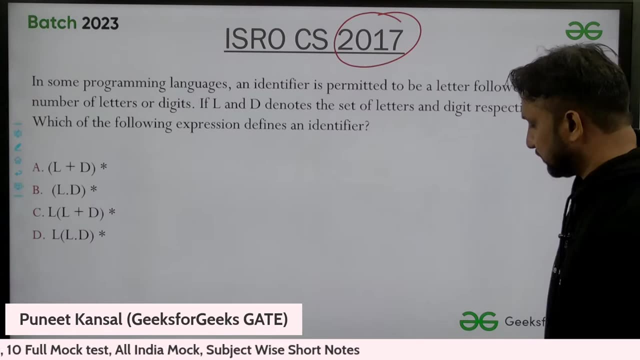 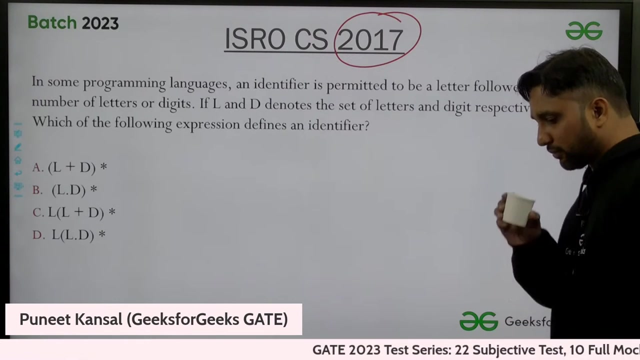 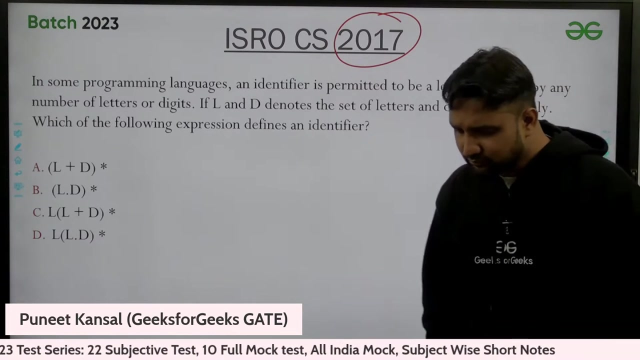 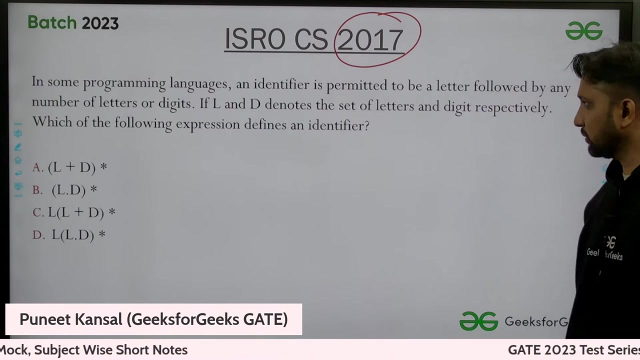 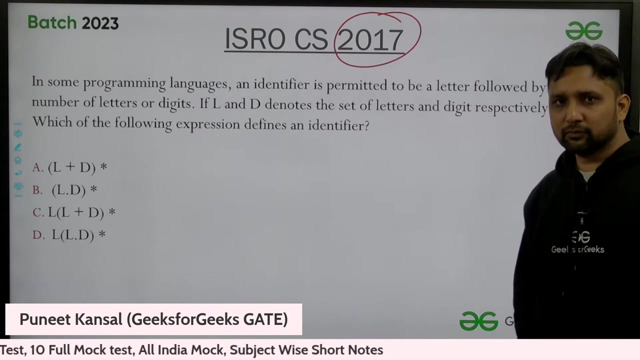 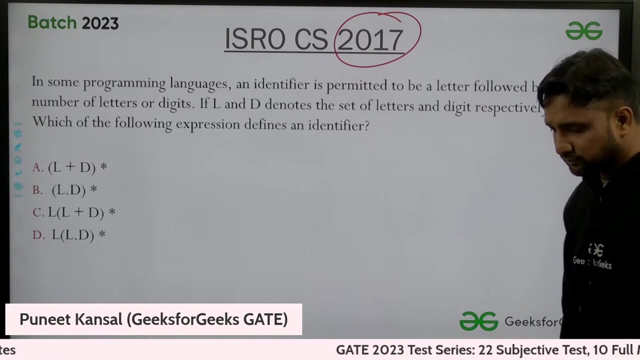 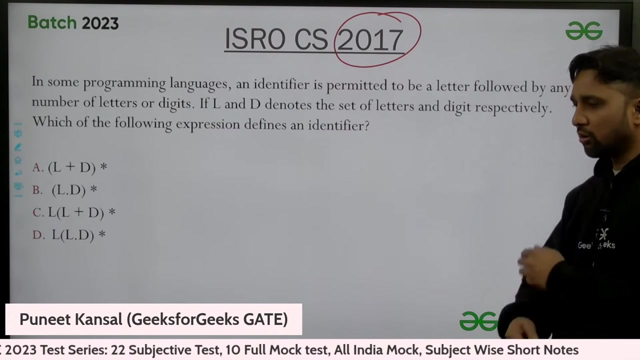 a slow question. twenty seventeen, please try it yourself. little modifications they are making okay, but read it carefully and try to solve it. okay. if you will think yourself, then only then, only you will be able to solve the question in exam. think yourself, think over it. wrong or right doesn't matter. 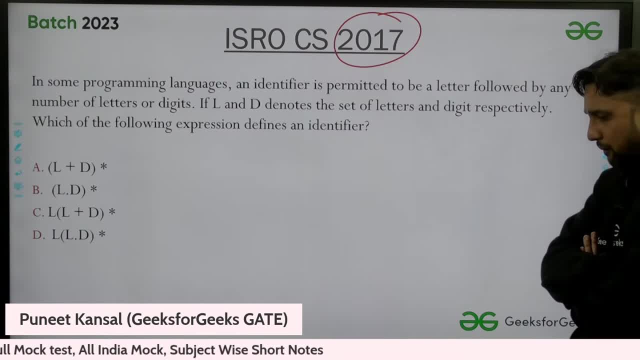 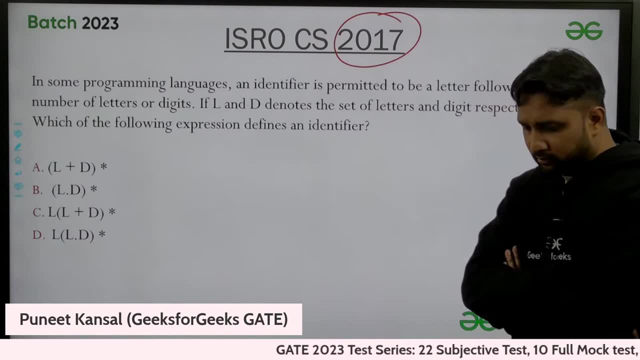 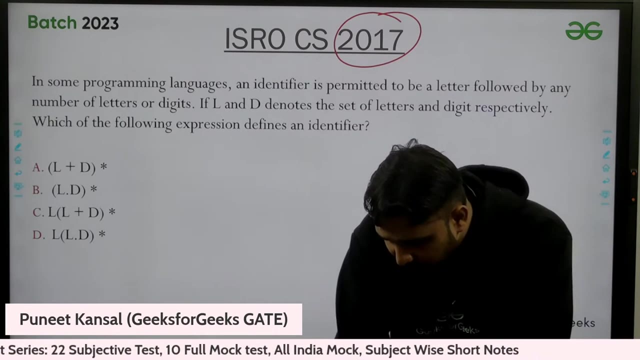 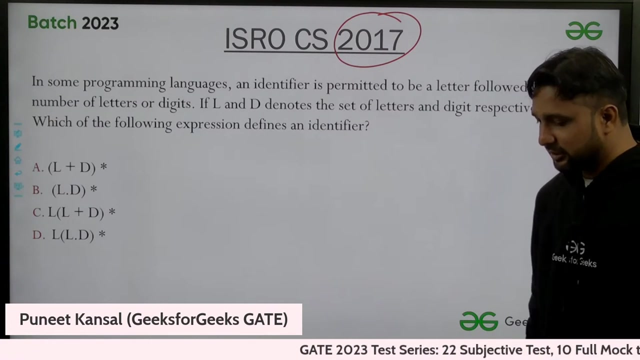 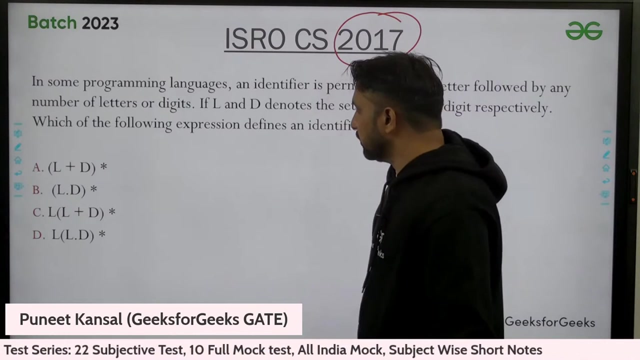 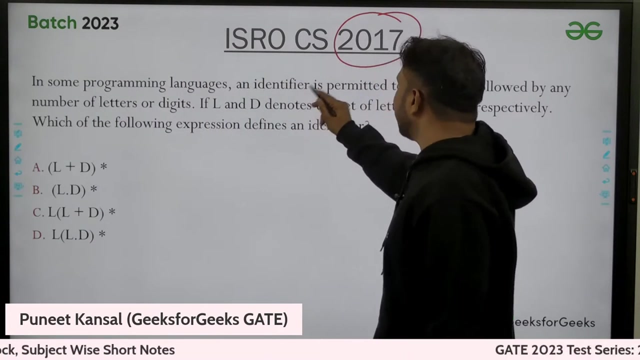 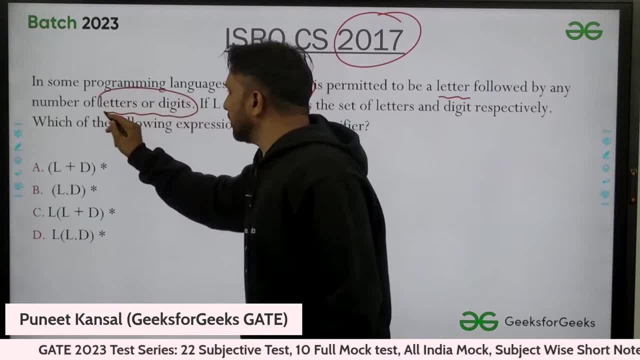 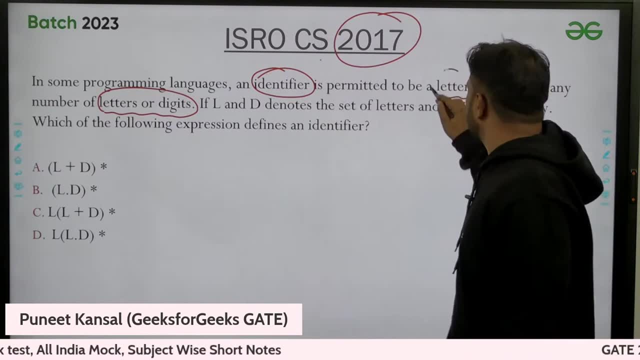 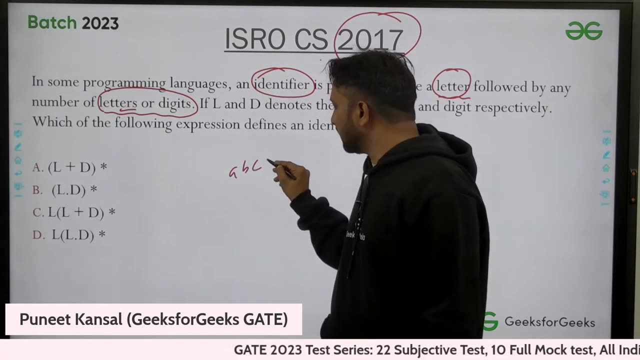 all get together by can you actually happens in almost every language- if you want to declare some variable that start with a letter and that can followed by any number of letters or key or digits. actually, like I can write ABC and then I can write the digits, also like this first character. 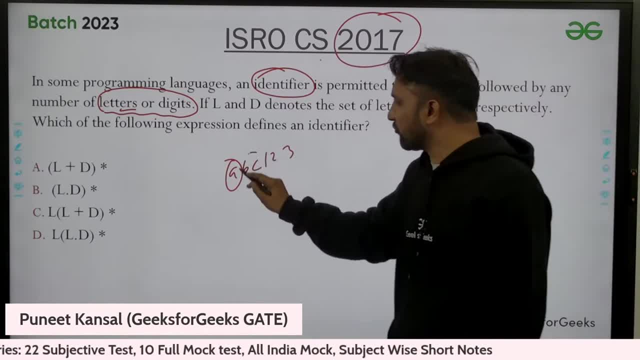 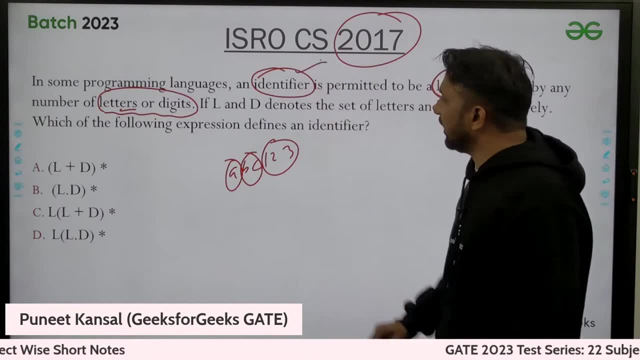 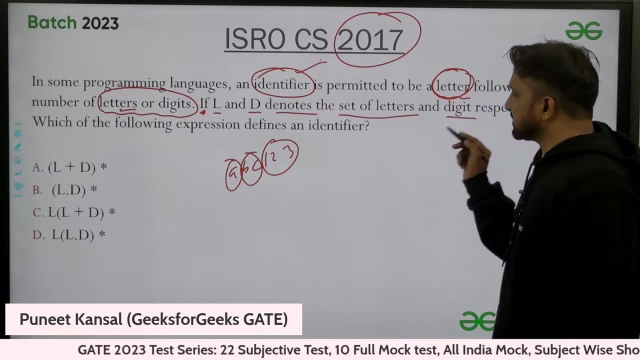 must be the letter. okay, after that, I can write any number of letters or digits. okay, so this is. this is happening with almost every language identifier. if L and D denotes the set of letters and digits, yes, this is representing the letters, L is representing letters and D is representing. 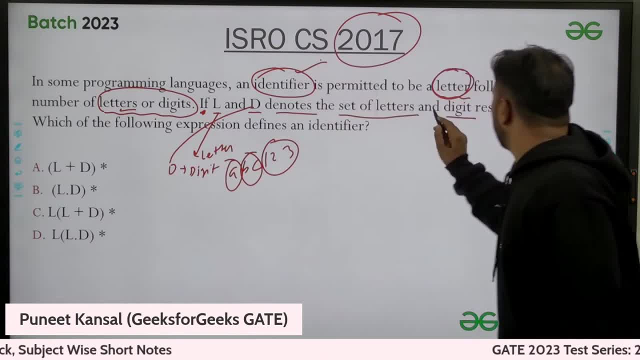 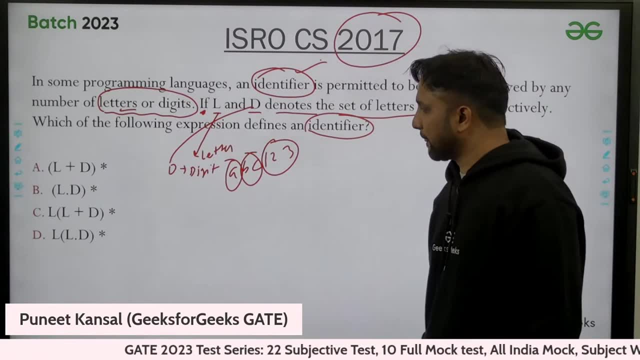 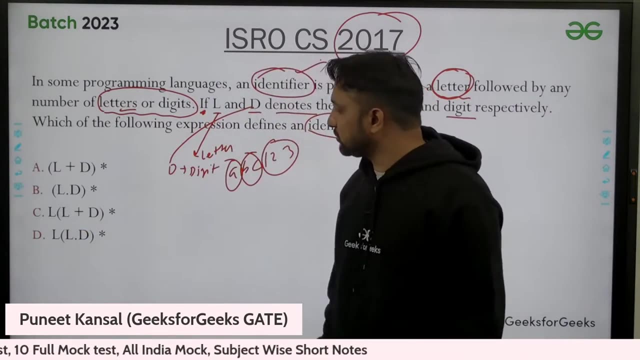 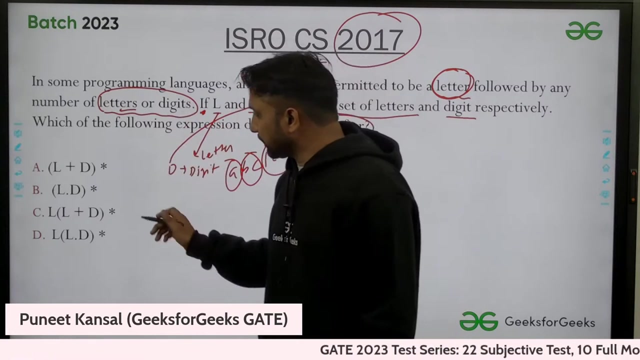 digits, okay, okay, then, which of the expression defines an identifier? then which of the expression is defining an identifier? okay, So this question is actually mix up of, like you can say, automata, and here to this lexical analyzer also, because lexical analyzer is also finding out the identifiers, okay, and 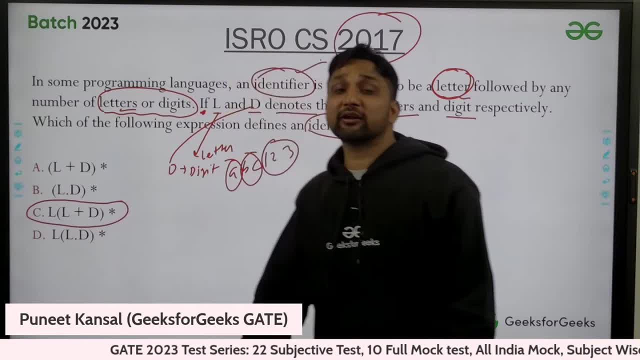 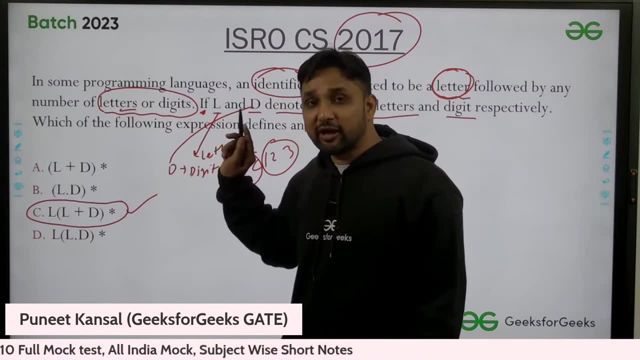 this is the. this will be the DFA for finding identifiers. we need to make the DFA of like that, this type of machine we need to make to find out the identifier in lexical analyzer. why you people are giving the maximum people are giving this answer is because we are saying: 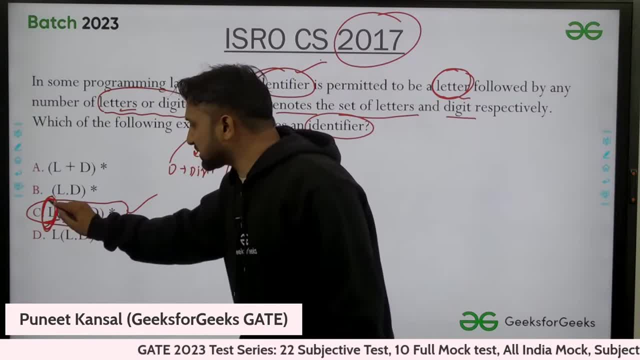 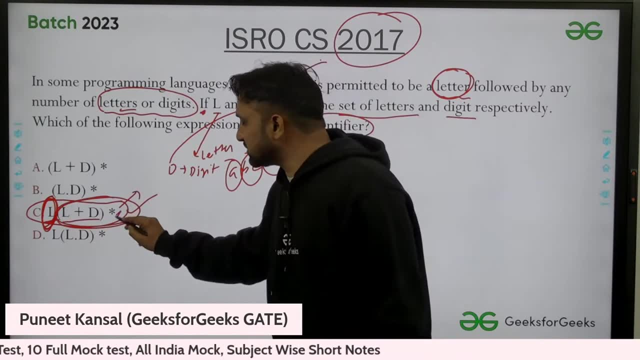 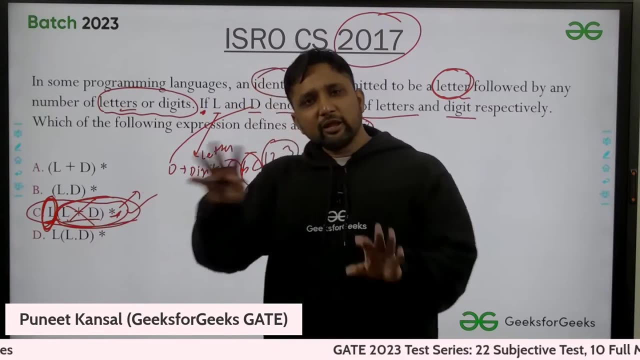 that one letter is compulsory. L is compulsory. one letter is compulsory after that. I don't know how many letters and this can be there. even there can be zero also. this star means, this star, closer, says that the value can be zero here or there can be any number of any. 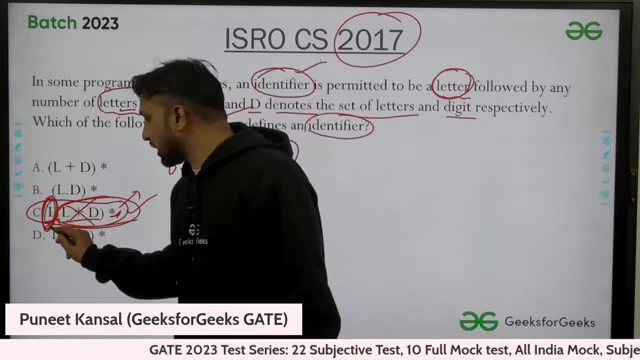 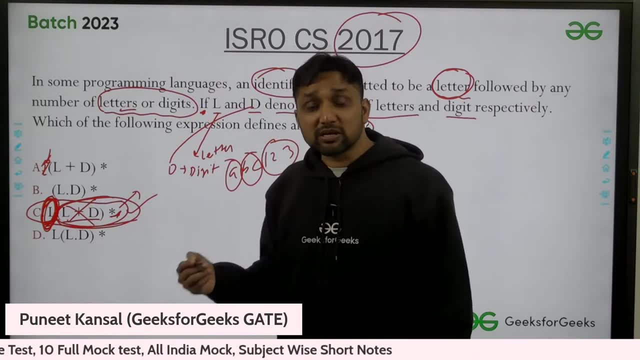 combination of letter and digits. but one thing is sure: that you start with one letter. okay, here we do not mention L, here we do not mention L. so see, identifiers must have some. first of all, Identifier must have some character in that. okay, so here I can have null also, and other. 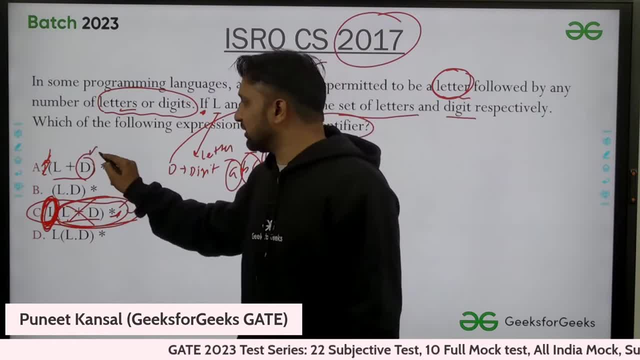 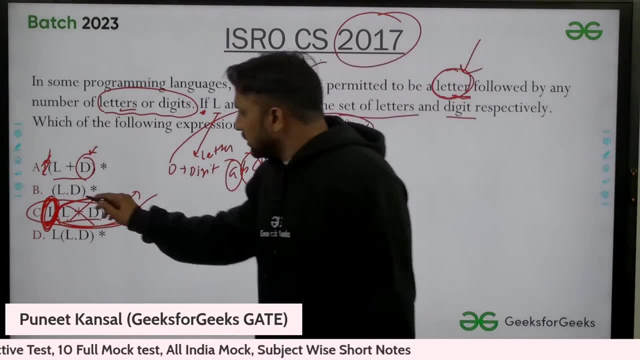 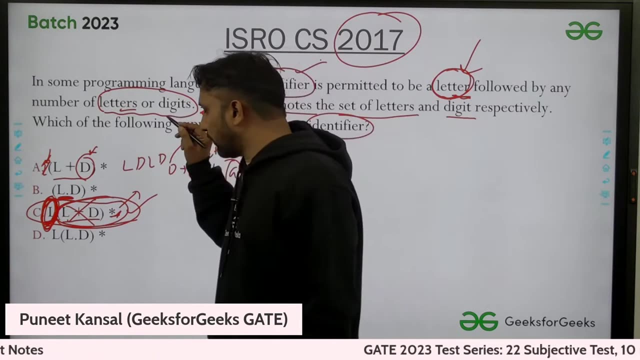 thing. I can start from digit also, so I cannot start with digit. we have given the definition of the identifier that must start with the letter, then must start with the letter here. this is the. this is: this will be like this: only LD, LD, LD. this is binding also to us, okay. 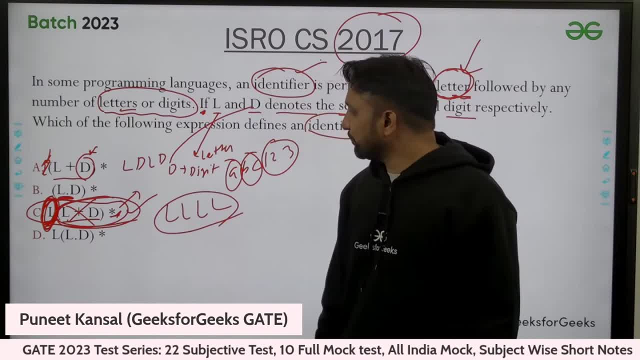 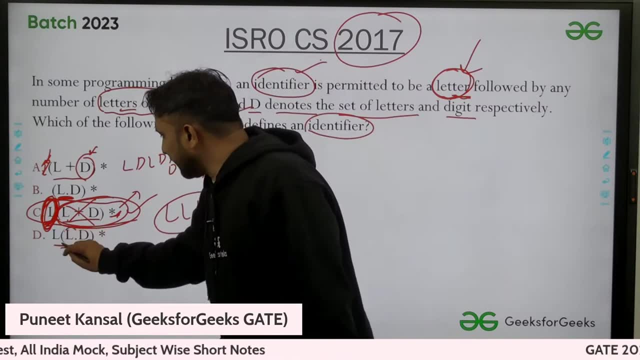 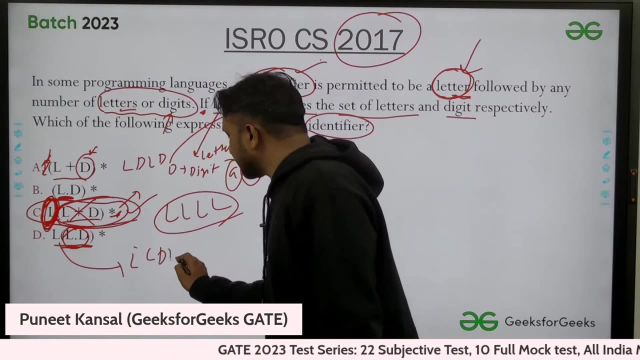 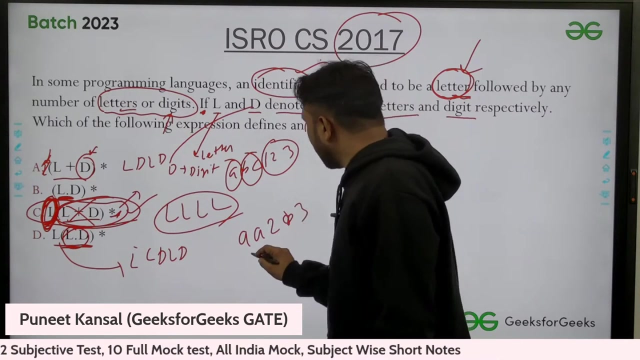 we can have L, L, L itself also as a identifier. Okay, Like only letters. we have, why we have. we need to have digits here again, that is binding, that, okay, that would be in this sequence, that will. that is starting with L, with letter, but after that he is saying that that should be like this LD. LD means like A, A2, like B3, but 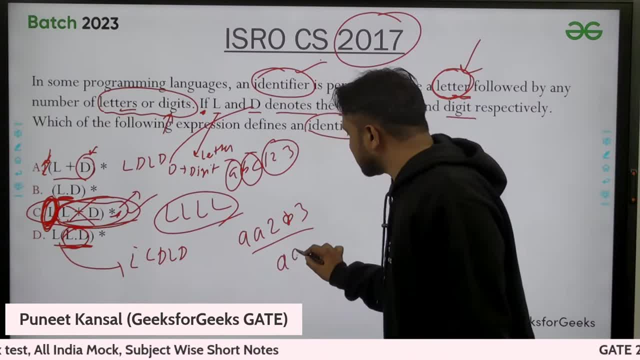 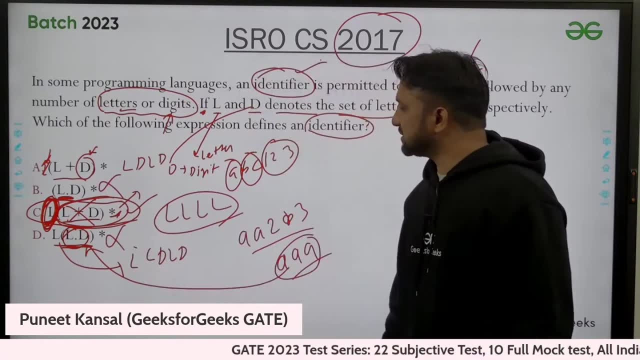 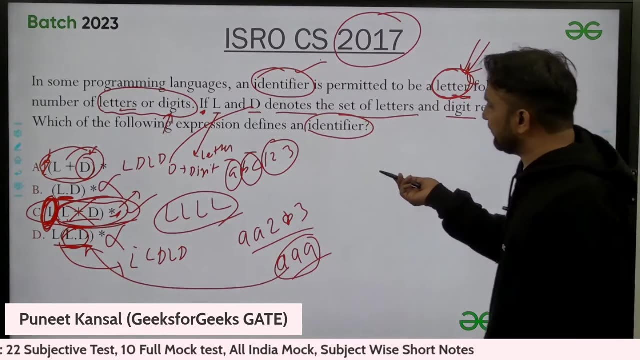 if I? what about if I want identifier like this: AAA only? so this cannot be achieved with this, and this also B and C, and this is in this. I can start with digits also, but start should be with the letter. this is happening with every language. in every language, we start with the letter, after that. 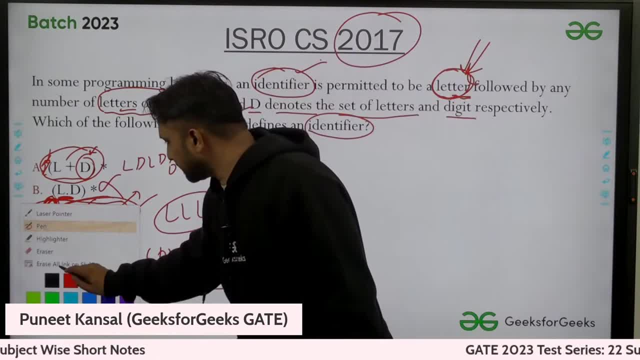 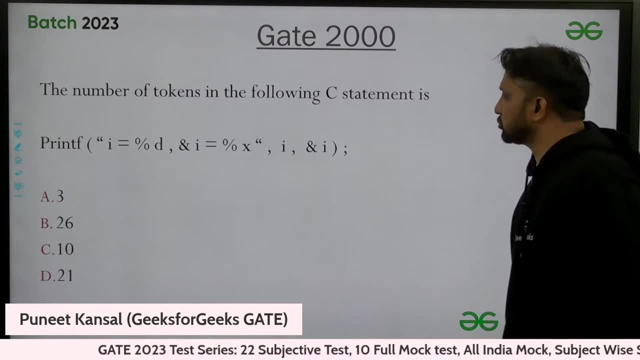 there can be any number of letter and character. so C is the right answer here. you people are right: C is the right answer here. let us move to the next question. please try it, gate 2000 question. we need to find the number of tokens in this C statement. please try it. 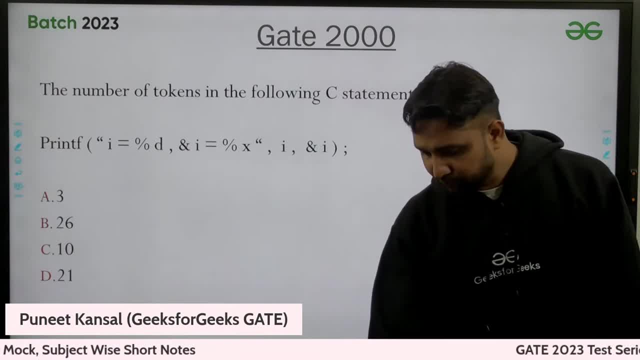 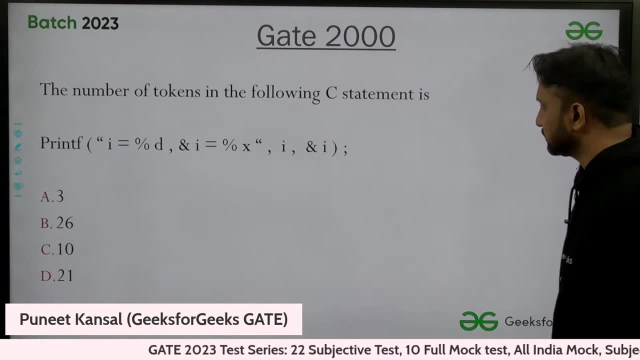 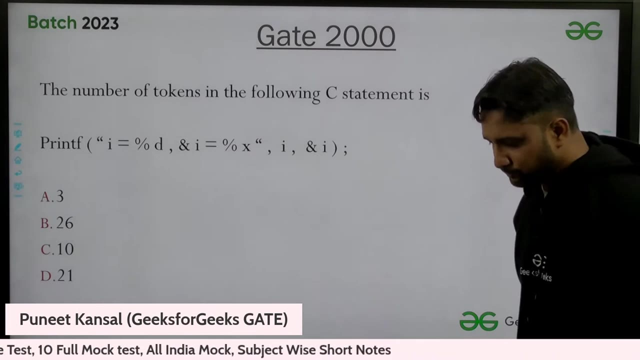 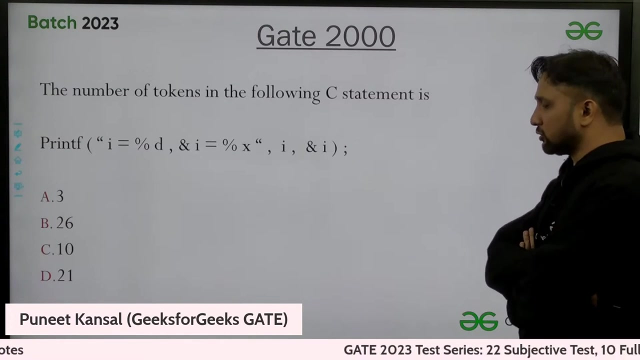 Okay, Okay, Okay, Let us try it. please keep trying it. These questions are not designed by me. these are gate questions we are taking. we will take out all the questions. okay, don't worry, we have lots of gate questions with us, isro or? 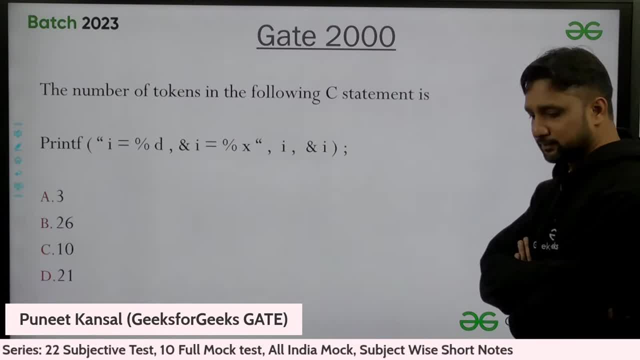 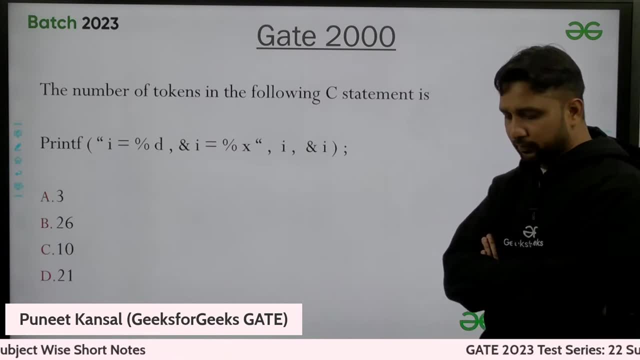 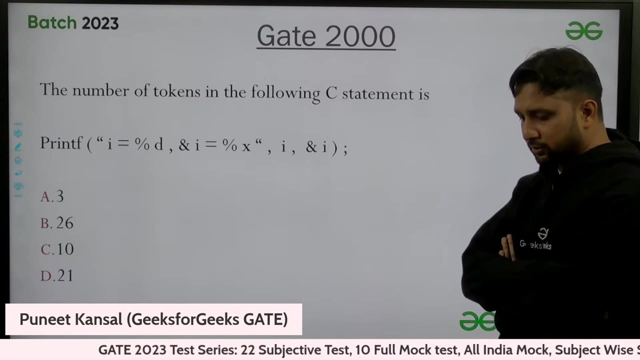 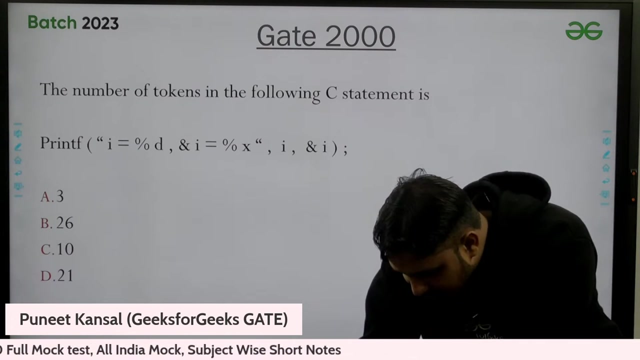 gate questions: Isro, Isro, Harsha, Vir, Divyanshu, Kavya, Jerry. all give the right answer, Varun also give. So all are giving the same answer. so you people must be right actually. 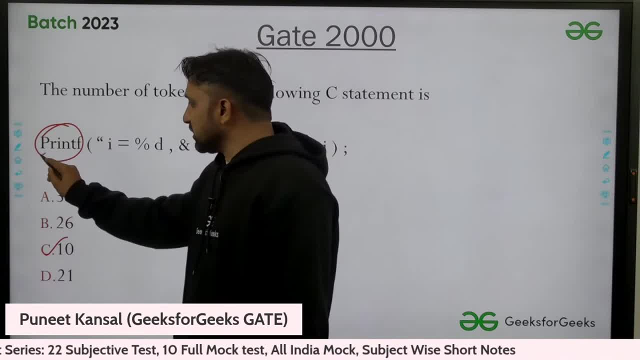 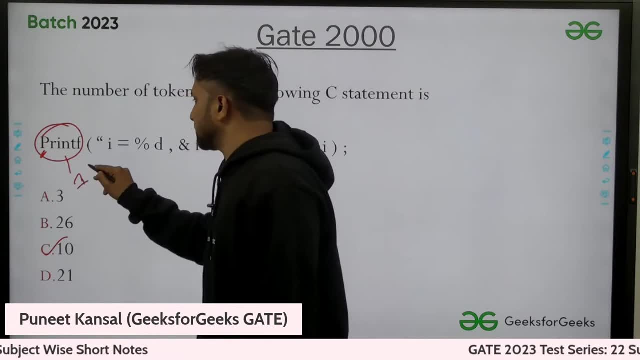 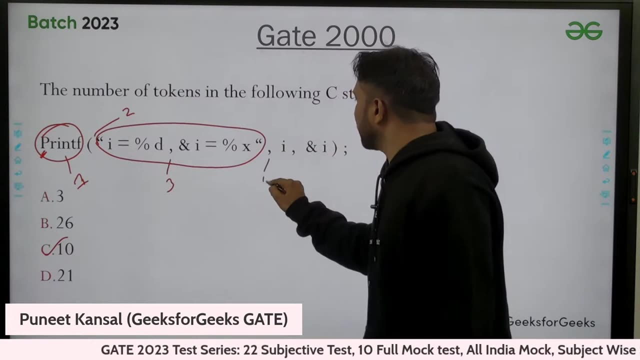 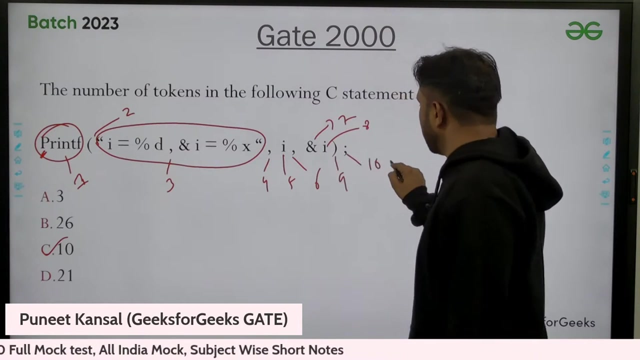 So this is one token. you can say that, sir, in C printf do not start with capital letter. but KalexicalAnalyzer is not bothered about the syntax, he is not bothered about the syntax 2, this is her token. 4th one, 5th one, 6th one, 7th one, 8th, 9th, 10th. yes, you people. 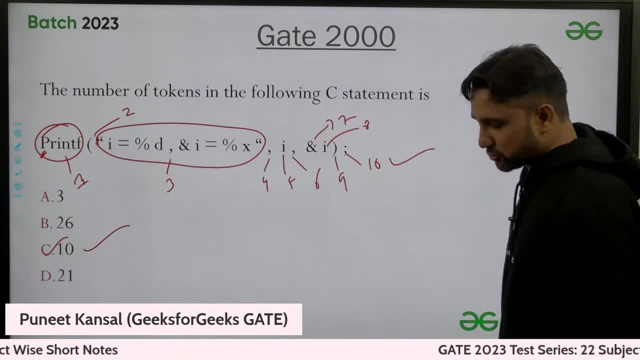 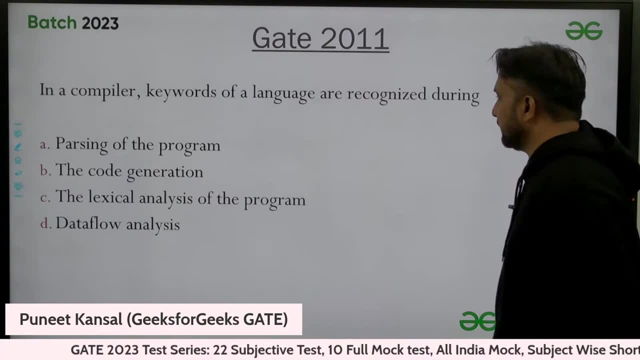 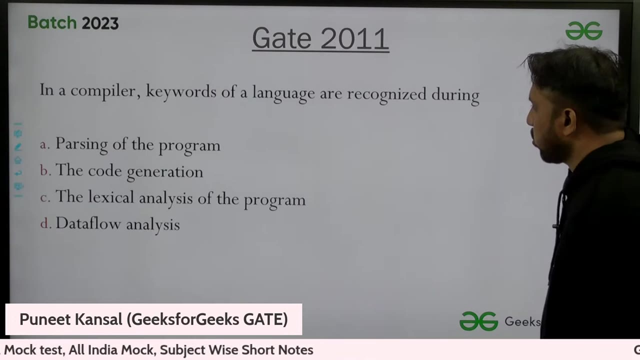 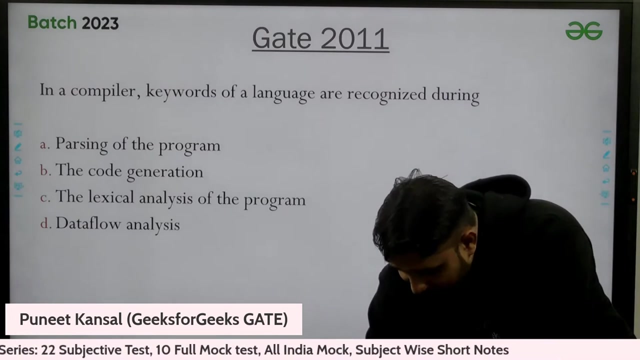 are right. She is the right answer. let's move to the next question. any doubt? anyone you can ask 2011 question. try this From so many questions, from examples also, you can check out in the chat box we are. 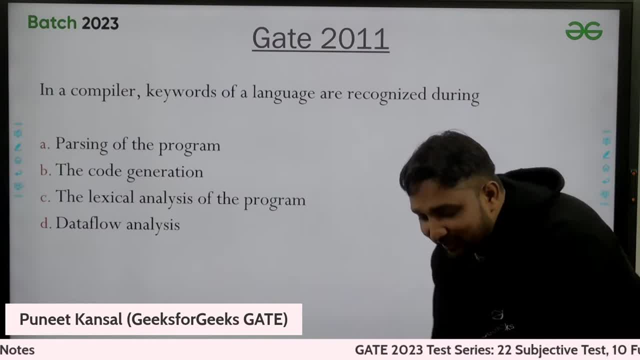 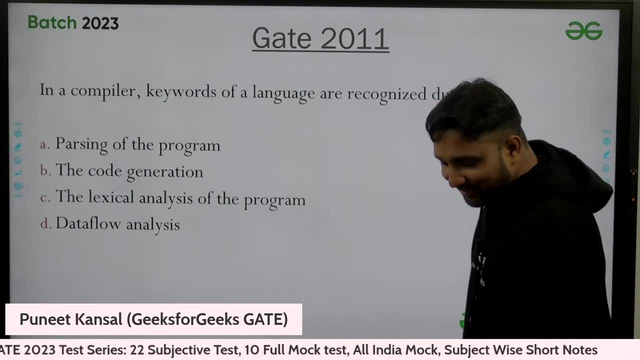 giving C as the right answer. So don't think that in exam you need to write C every time. so I have, I think, taken C as the option everywhere. that doesn't mean that C will be the right answer if we don't know. 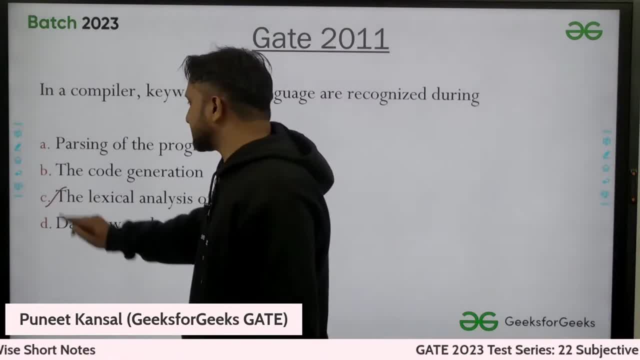 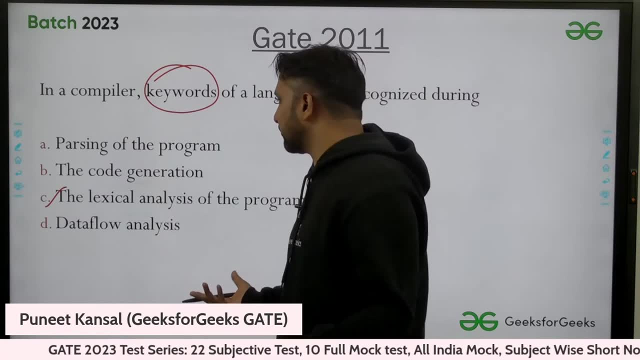 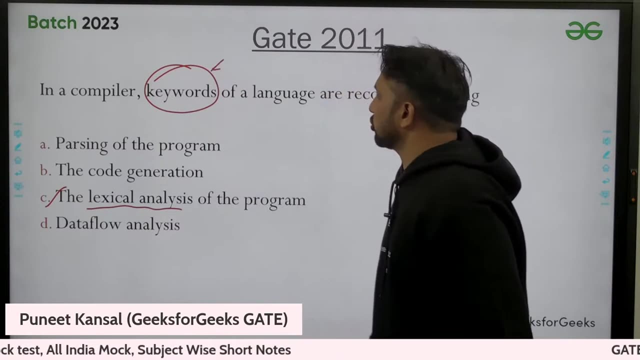 the answer. we are going to click C. So C is the right answer, you are right. so keywords, if for switch, these are the keywords. any other keywords are all find out by the lexical analyzer. Lexical analyzer is finding out. these are also tokens. these are also tokens, one type. 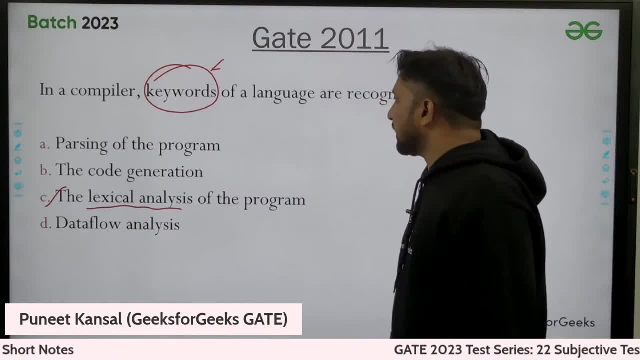 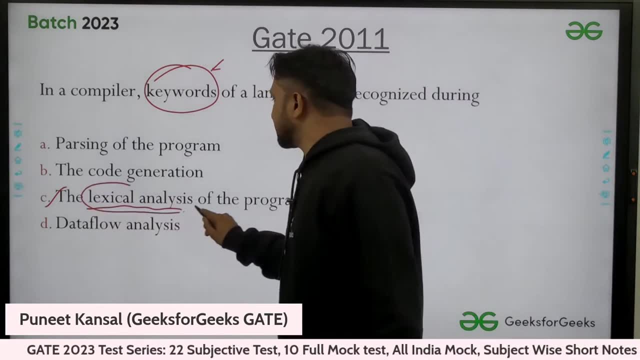 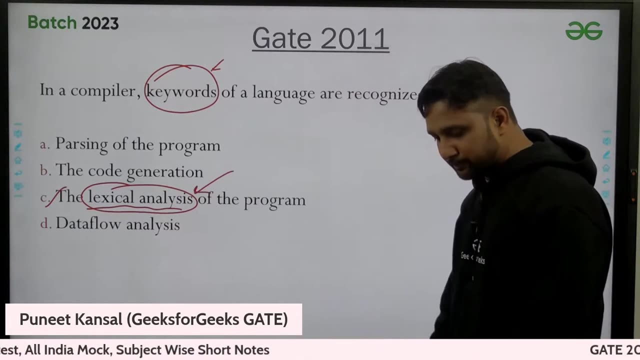 of token, one type of token: their identifier also. they can put identifier also here. they can put operators also here. all are recognized, while the lexical analyzer is. all the symbols are recognized, everything is recognized, while this phase only Okay. 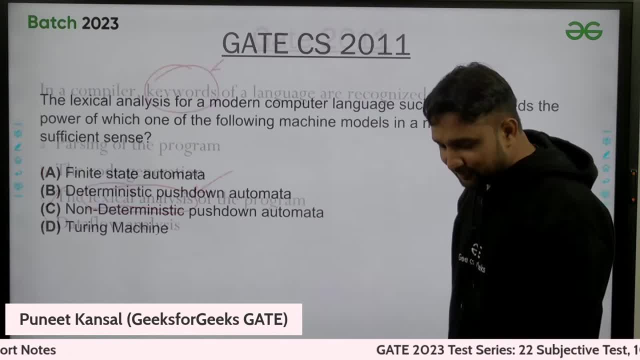 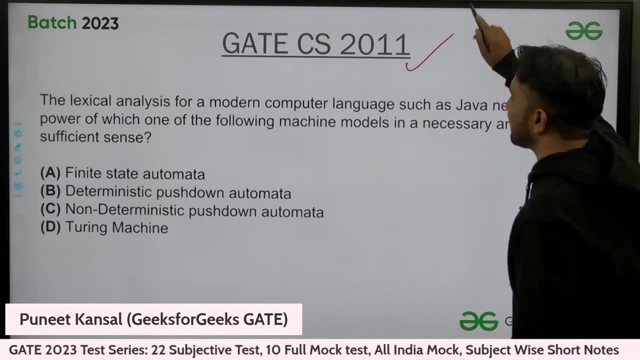 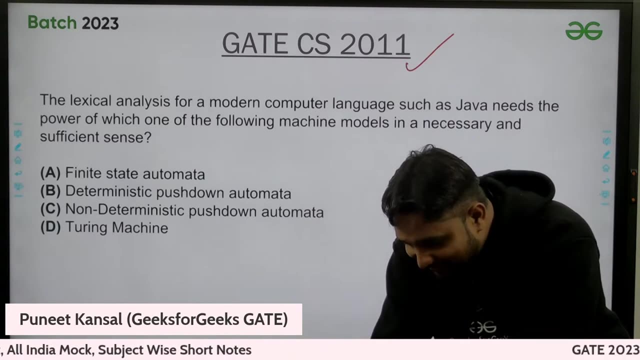 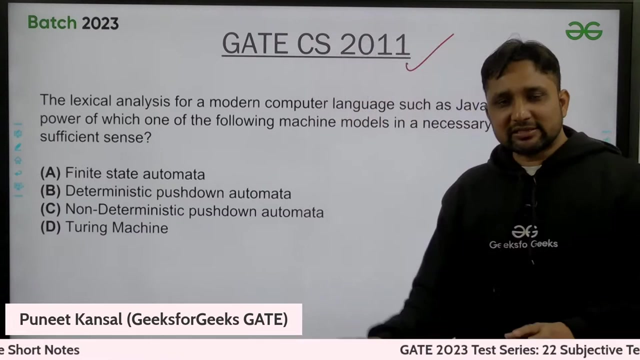 Deepayanshu says: Jaya Mata Di C. that's right, Okay. 2011 question: try this. Please try this, Okay. So Sainath is asking about the notes. The notes of all the lectures, all the lectures in this series, is available on, on, on the. 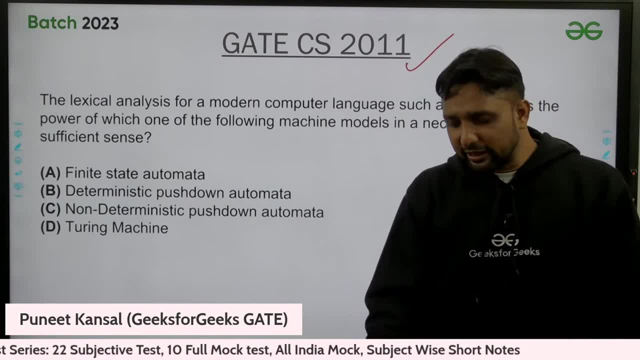 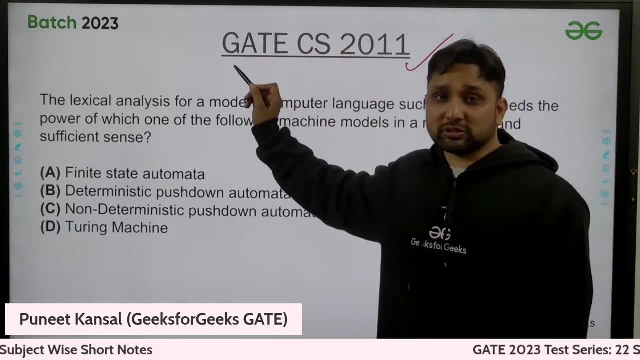 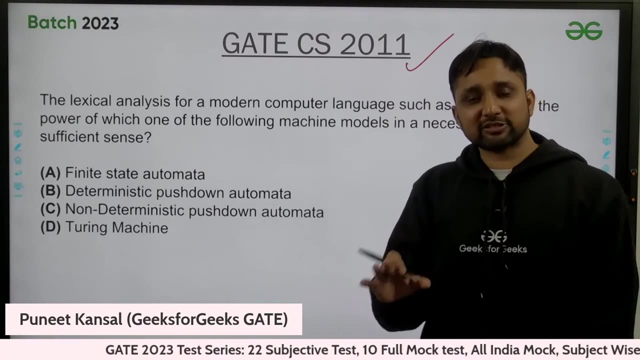 on the page. actually, on the get crash course page, You can find out the link in the description. actually there is a link link to the this complete course, not only this lecture, but complete course. Okay, So this course notes are provided. every lecture notes are provided on that particular. 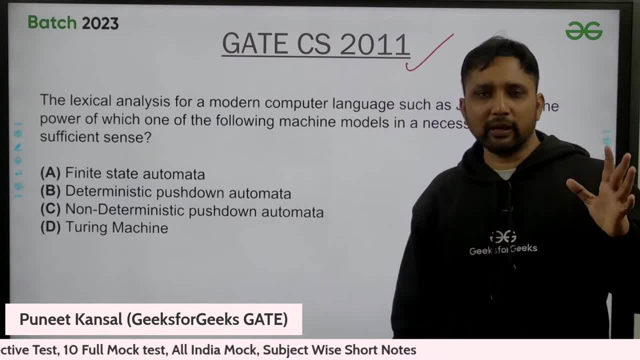 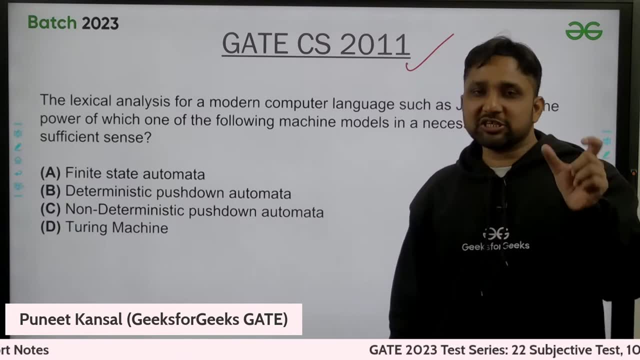 page. only that is free. only this course is free for you people. You need to, just you need to. if you want to access the content, all the notes also, then you need to register over there. That's it. This is what you need to do. 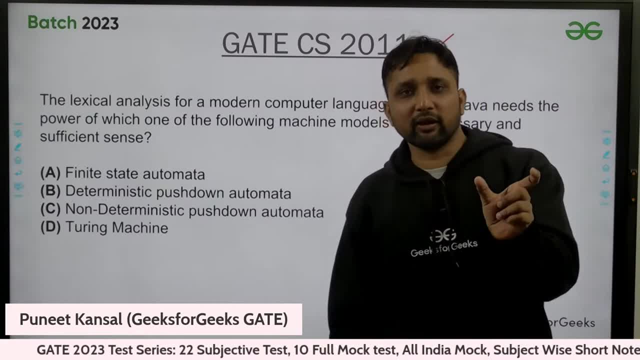 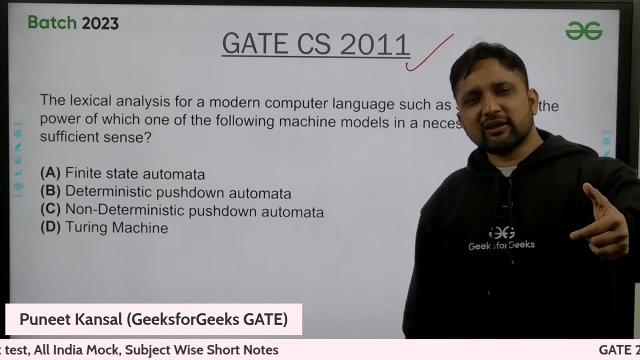 You need to register over there for this course so that we can- you can authorize yourself. Okay, You are, you are just just for authentication. So register yourself, Okay, And you will find the notes for all the lectures, not only this lecture, this lecture also. 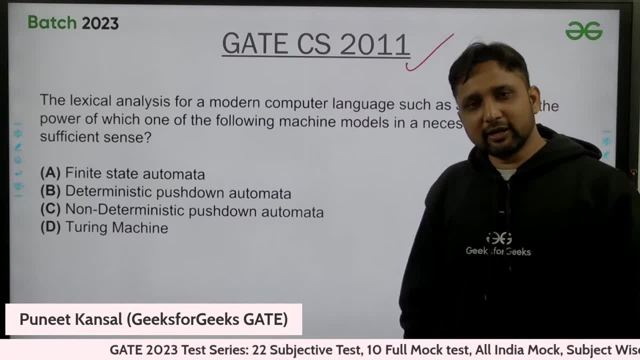 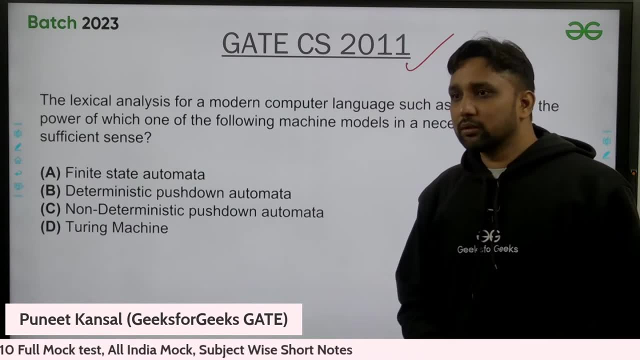 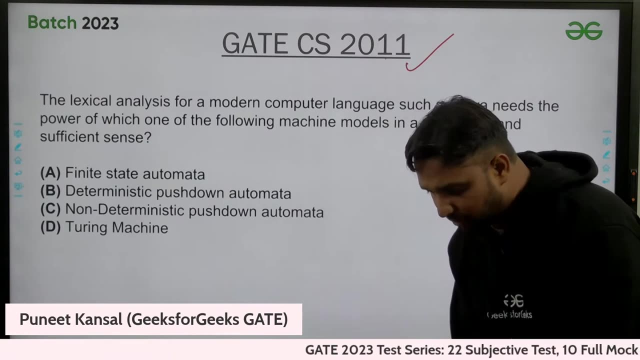 all the lectures notes you will find out there- And all the content- previous lectures also, which we have already done. all everything will be in a managed way And if I can show you here also, okay. so let me give me some time, let me you try. 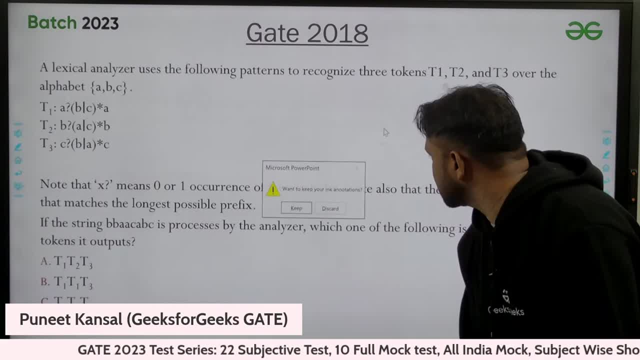 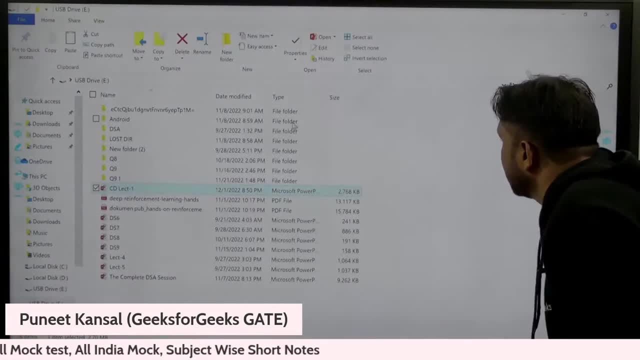 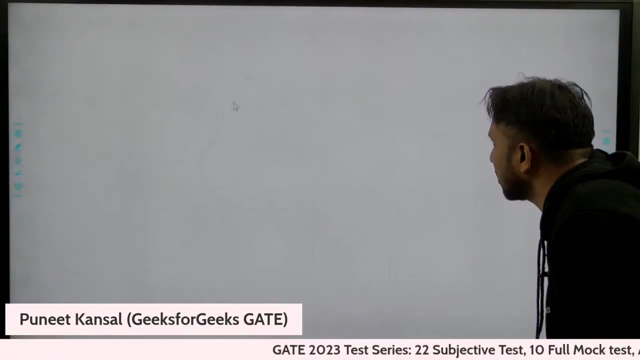 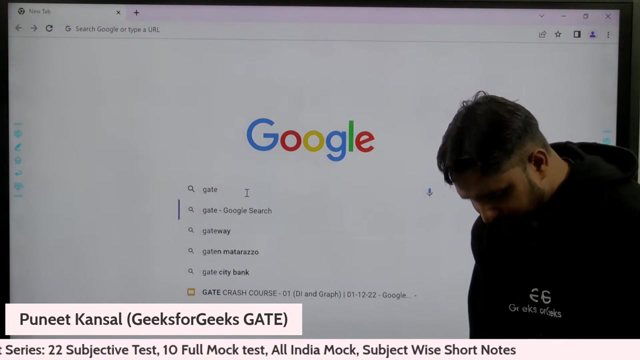 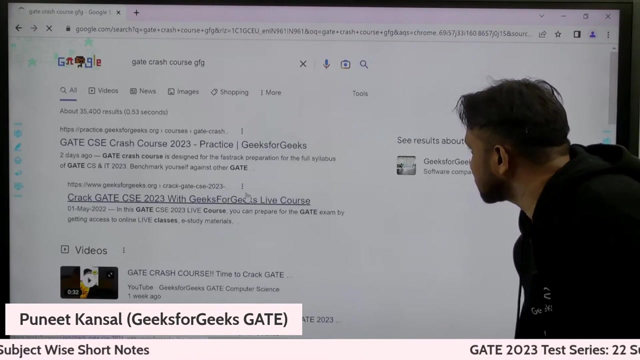 this question. So let me show, show you this Here also what you need to be done. you can check out in the description or even you will write in the Google: also get crash course GFG. you can write like that: great crash. 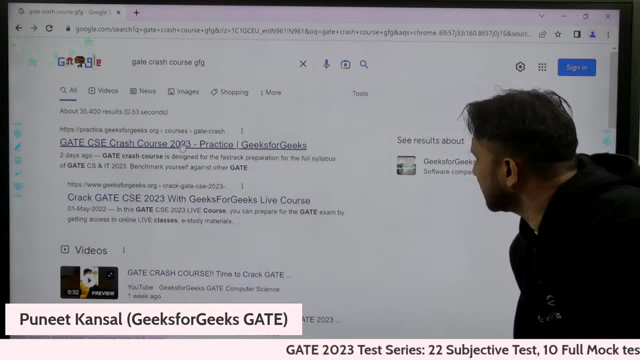 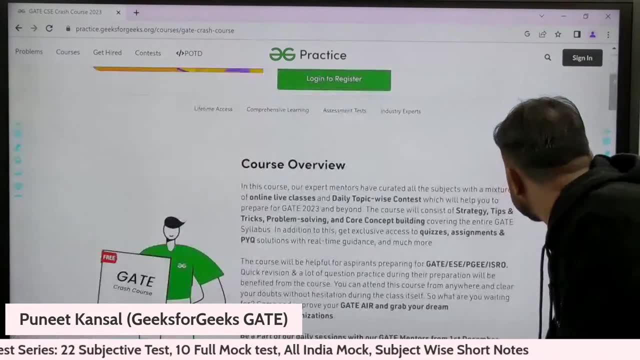 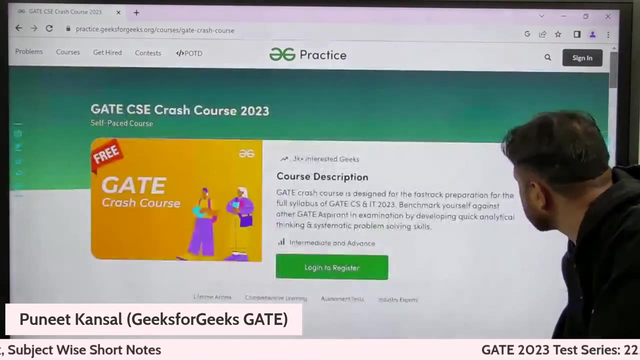 course. So here. so this is the first thing you are getting, see, first thing itself you are getting. So this is the complete crash course, which is, you can see, that is free of cost, no price, zero pricing, with zero pricing. complete course is there. 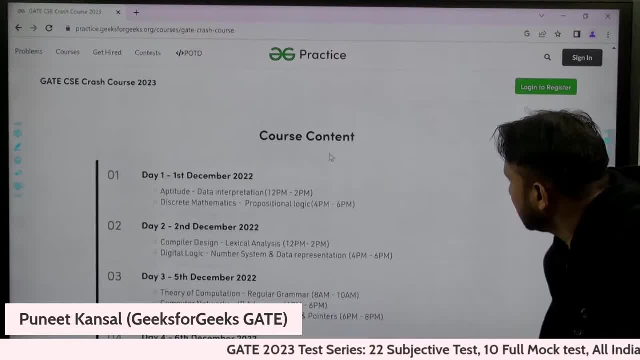 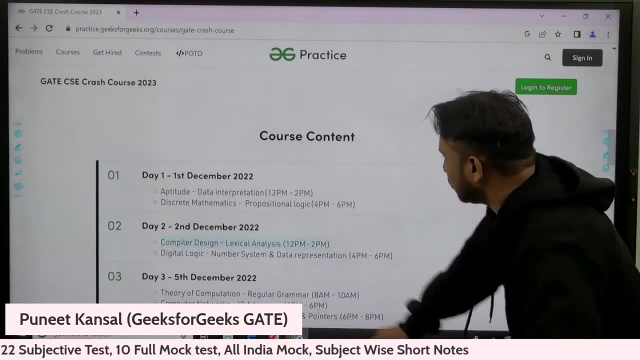 And we will find out all the detail. This is the lecture is right now going on. lexical analyzer- this one, this lecture is going on right now, 12 to 2.. And today itself there will be lecture for from 4 pm to 6 pm, of digital logic. 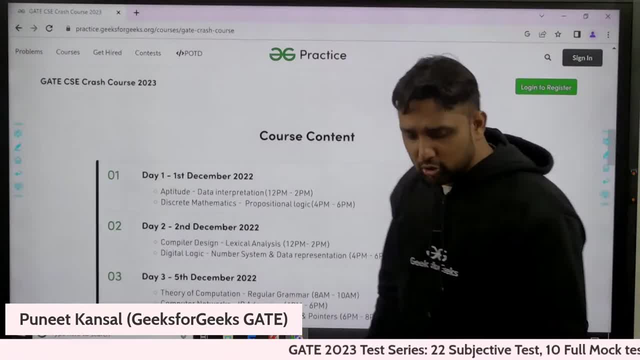 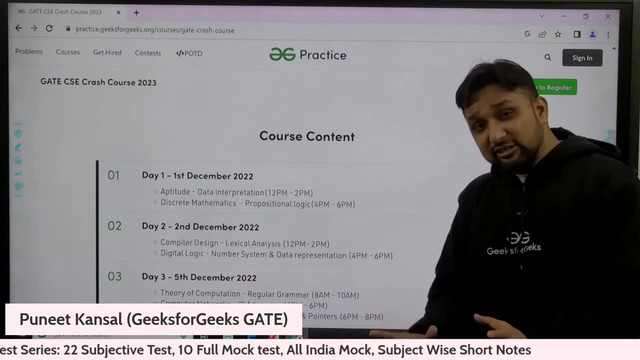 Actually, that will be from Biple, who is from IIT Kharagpur, so he will deliver that lecture today from for digital logic, Everything will be. all topics are individual. okay, we are considering that. all you do. 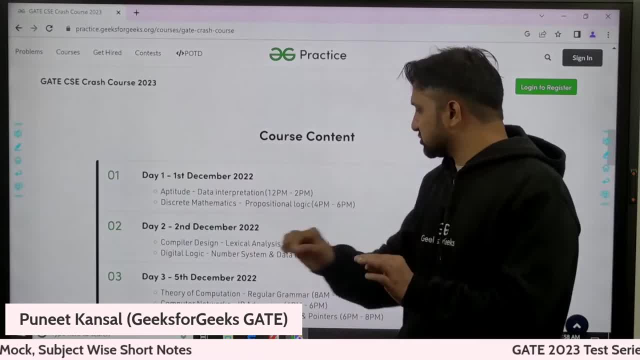 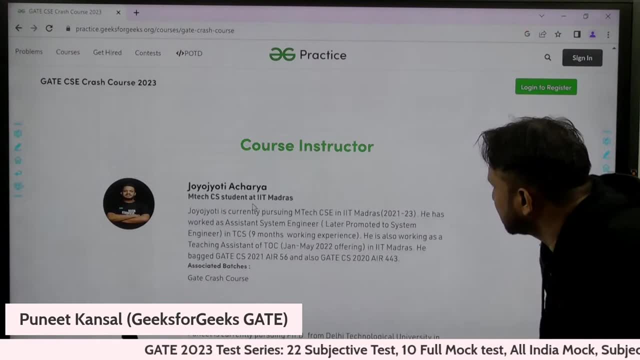 not need nothing you need prerequisite is zero, that's it okay. And all the schedule is given here you can check out. These are the mentors, Like Joya Jyoti from. he is right now in IIT Madras you can check out. this is me. 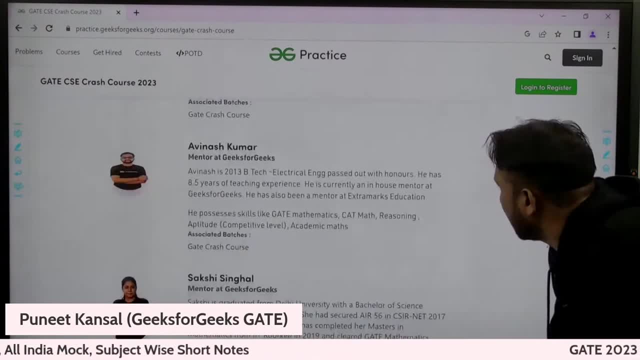 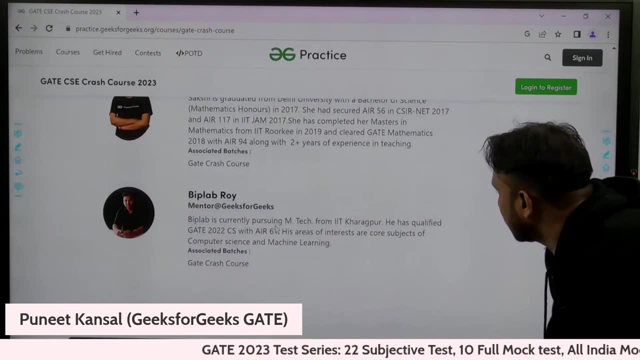 I am pursuing my PhD from DTU Avinash sir, who is very senior faculty, Sakshi, who is very good at mathematics, and Biple, who is from Kharagpur IIT, Kharagpur. so these people. 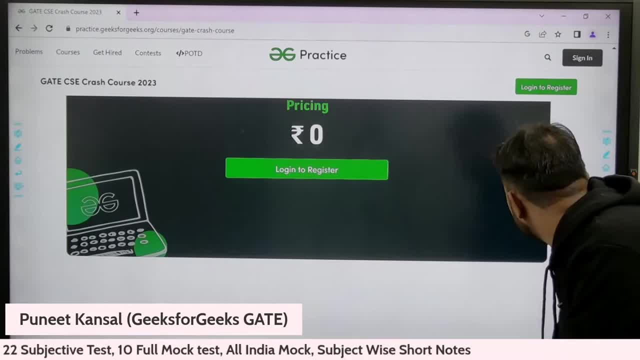 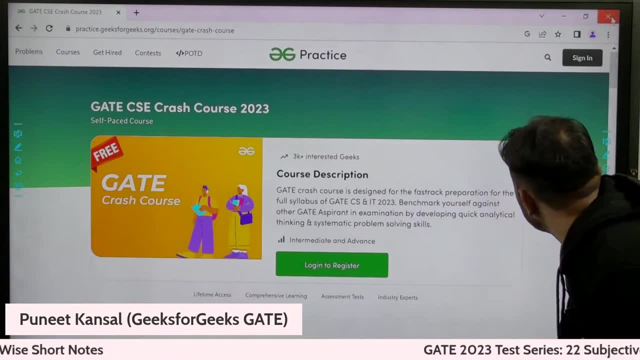 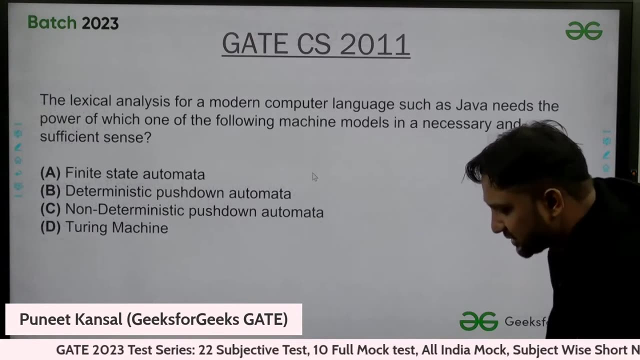 are going to help you. you need to just register here And you will get the complete notes here- only complete notes- after registering. okay, Okay, So let's move. Let me close this and let's move back to our to the next question. I think yes, this. 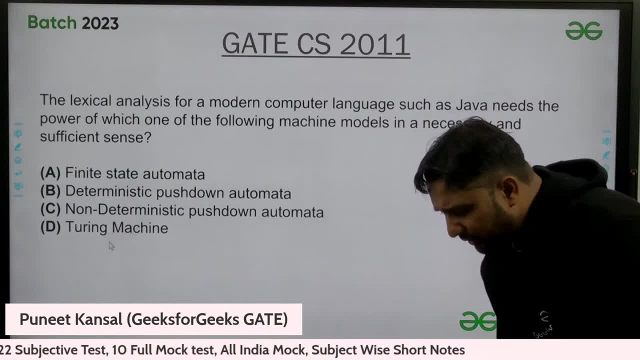 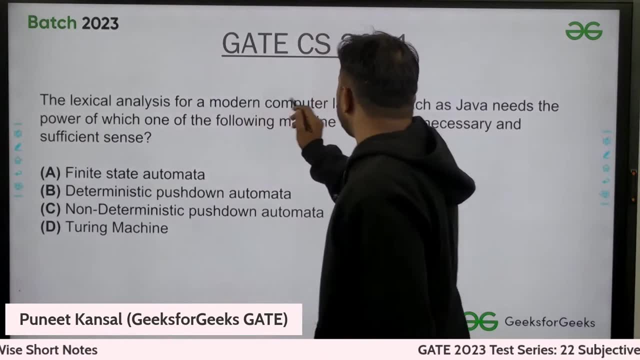 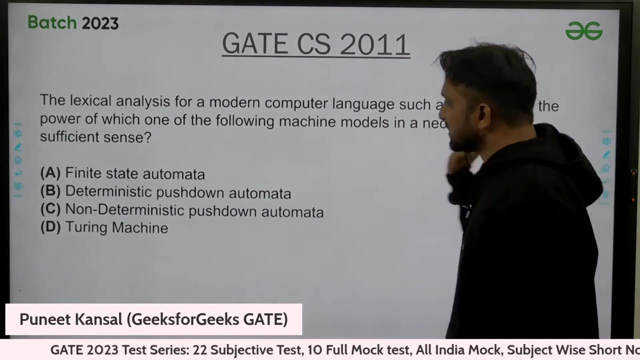 is the, so you have already given the A answer. A is the right answer. so a lexical analysis of a modern computer language such as Java need the power of which of the flowing machine model in a necessary and sufficient sense? okay, this is needed for lexical analysis. 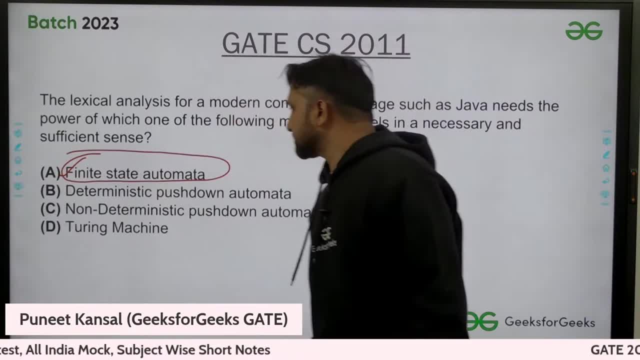 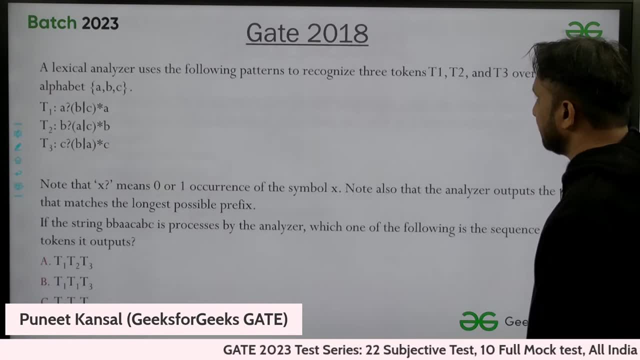 phase: This machine is working. behind that, okay, finite state: automata: This machine is working. 2018 question: try it yourself. little little, little bit hard one, but please try it, please, everyone try it. try it okay. 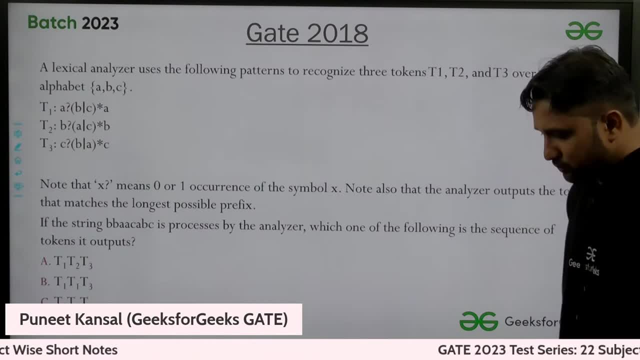 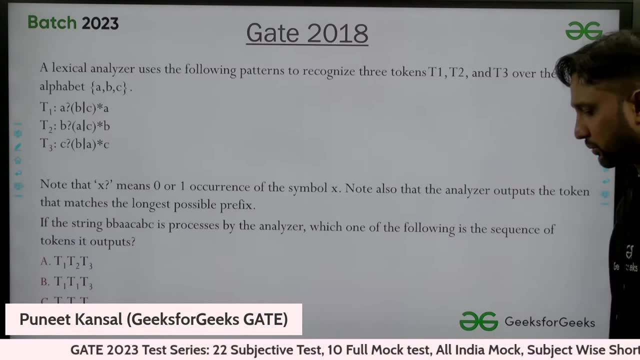 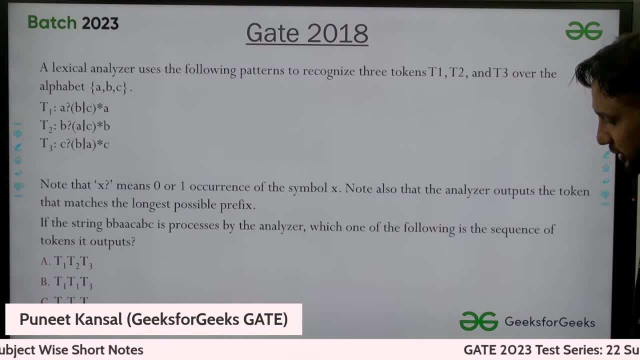 Okay, So let me, let me get aside so that you can see the complete screen. You can ask me anything. You can ask me anything, How Dude? Yes, Okay, Varun says that last option is not visible. last option, let me write here: D option is: 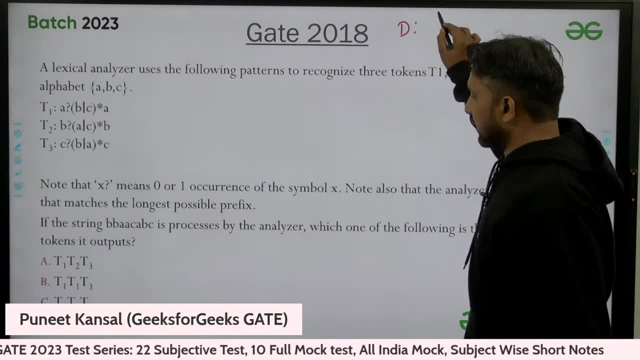 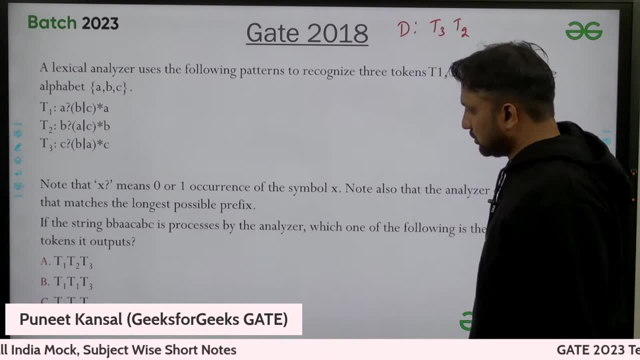 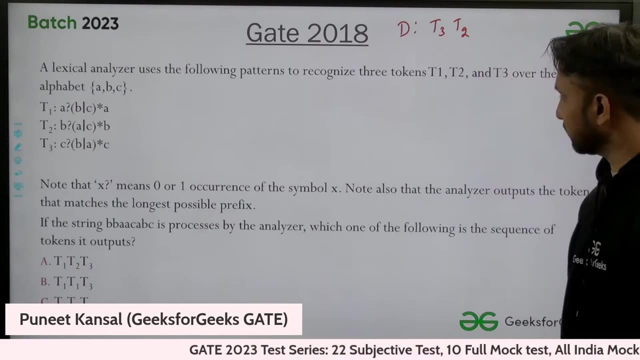 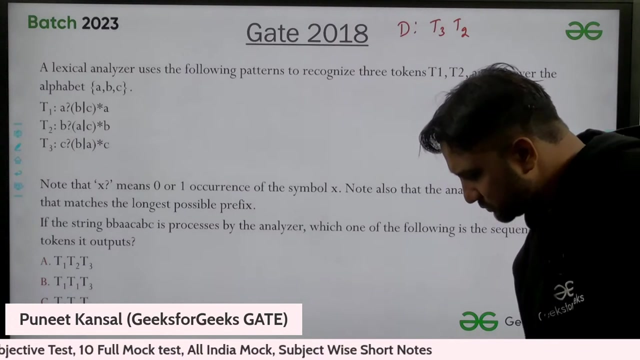 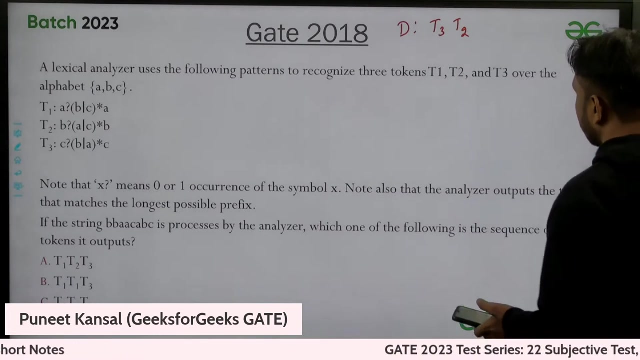 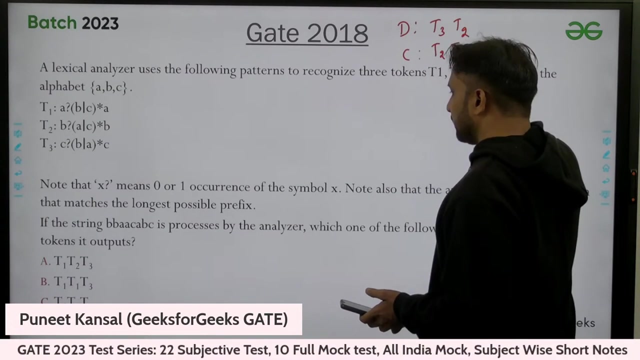 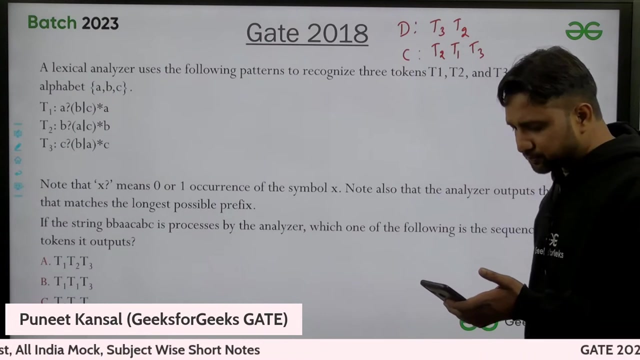 T3 and T2,. I hope that is the answer: T3 and T2.. Arshya says that she is also not visible, so C is T2, T1, T3,. I can see that many people are able to solve this question also, so this is a good question, actually good question. 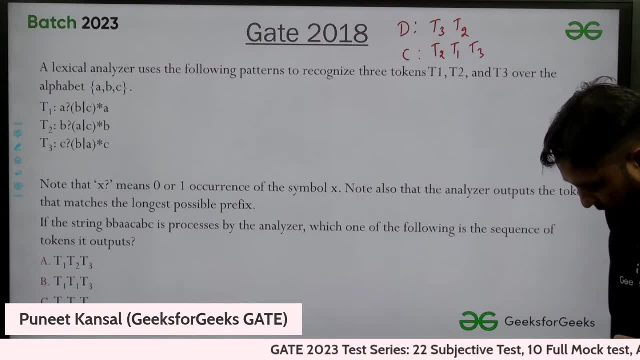 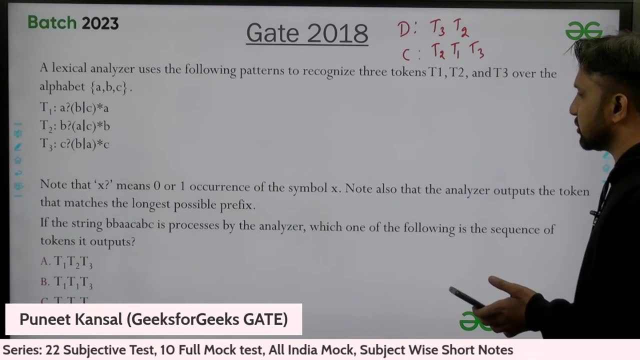 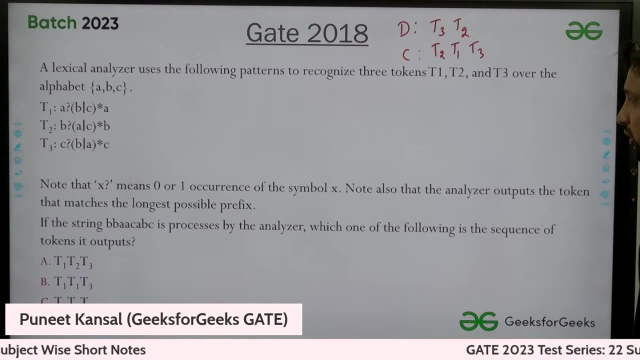 I will say that, from gate point of view, this is a good level actually. so if you people are able to solve this question yourself, What I will suggest to you people is that you please take some test series, and now you have to go through the test series also because you need to now practice lots and lots of. 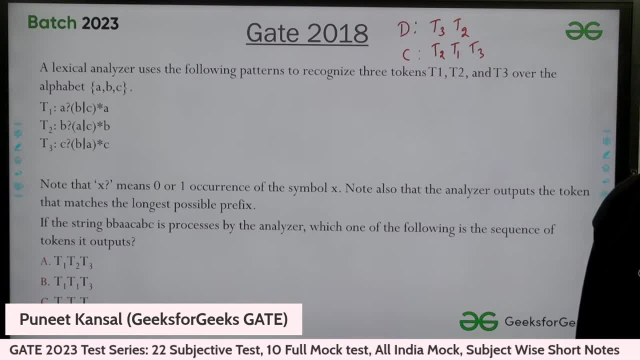 questions. it's better you take one or two test series, even I will say not only single one. take two test series which you find that. okay, that can help you and please attempt to solve the question from there. okay, If you are able to score good in the test series. 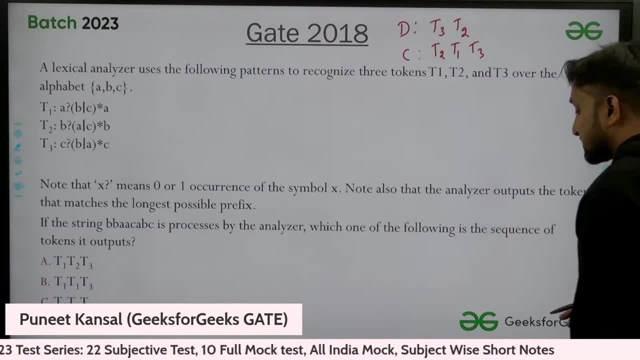 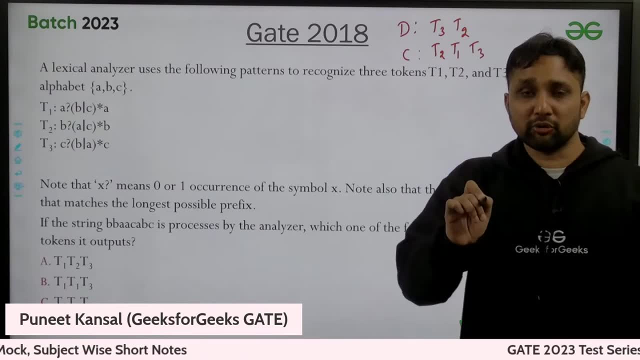 Like, if you are able to score good in the Geeks or Geeks test series, that will ensure you that, okay, you will get below 300 rank. that will make this thing sure to you if you are able to score good in that, because there are good level of questions are there? 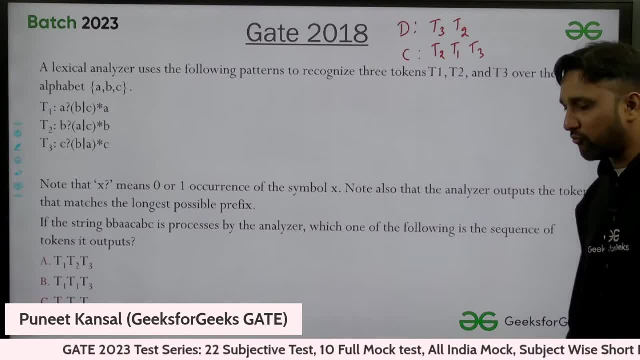 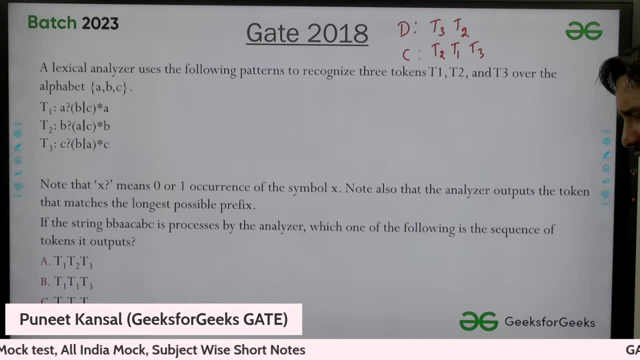 and if you are able to solve this question, then definitely you have to go for the test series because you have great chance to get rank below 300. The second test series will help you tenfold. So any official review, we can only give you a minimum manila to say six minutes and 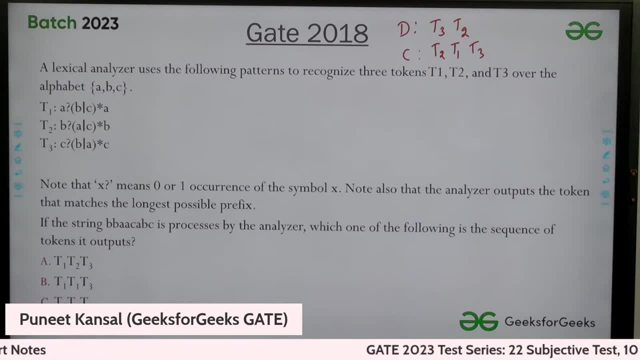 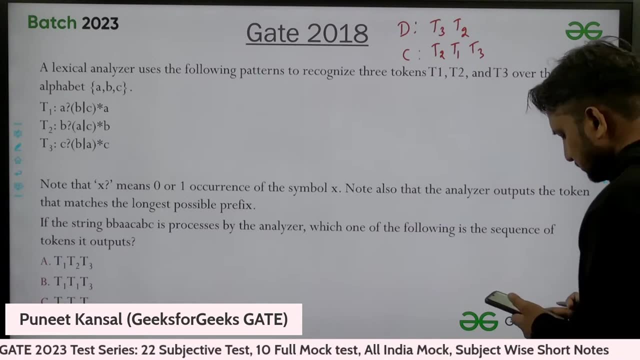 every single person able to score good. you have got to go for this test series- Product placement, perfect score. So you need to egently reflect on yourself. you need to ready yourself and make it one rule which left you in doubt that marketing is a dream and it's easy to believe it's. easy to change. So again, if the customer has no idea about the market in particular- and they understand it- you need to go for the extra part and understand the basics. There is no question. and be sure to compare yourself with anyone, and, in fact, if one of you 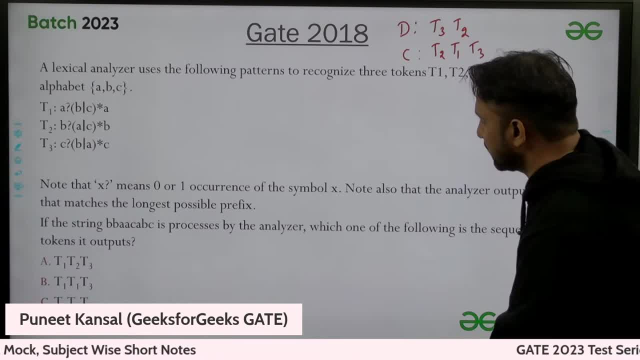 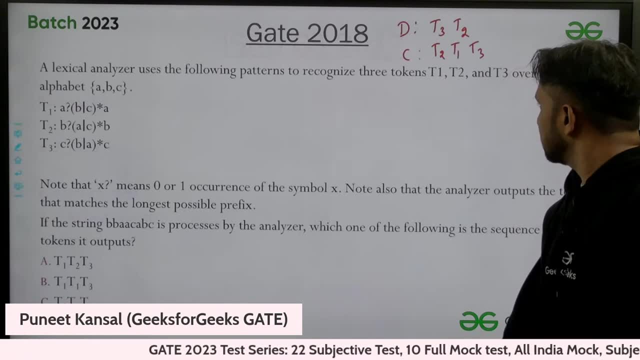 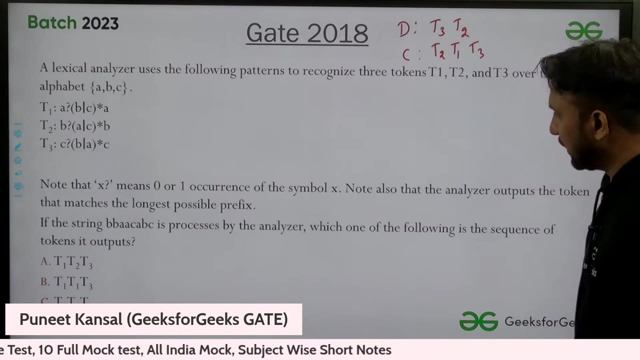 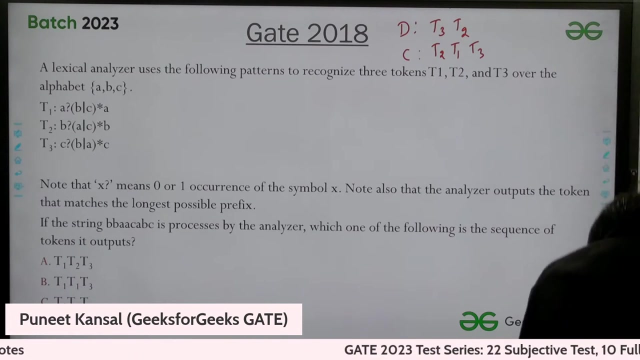 This may take little time, It's okay. So let me wait for one last minute. After that I will also try. Otherwise, you can keep trying. That is more important. After one minute I will try this, Thank you. 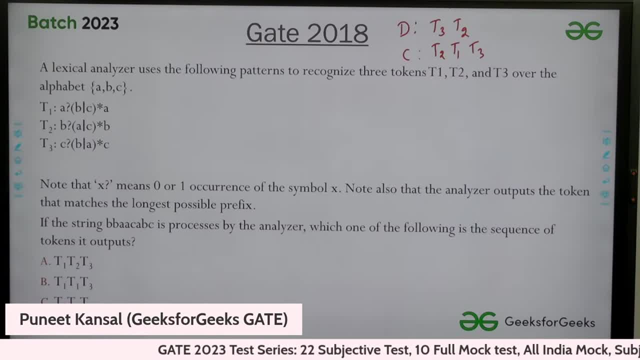 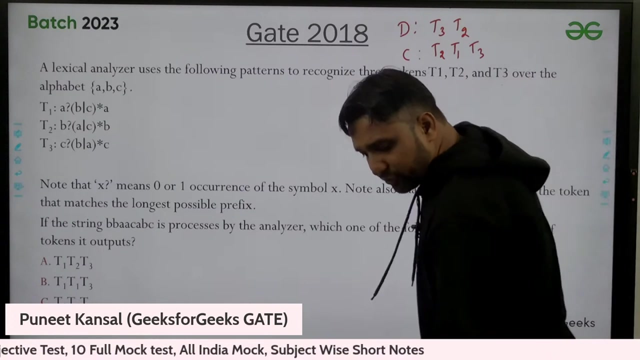 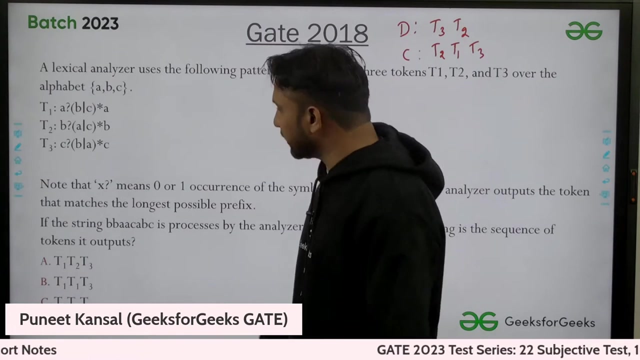 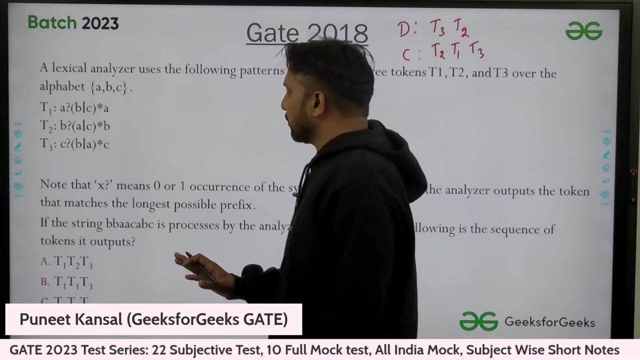 Thank you. Okay, I think I have to try now. If you people are trying, please keep trying. That is more important, rather than even listening to me, because you can find out this explanation later on, also in the recorded part. So if you are trying, that is more important. 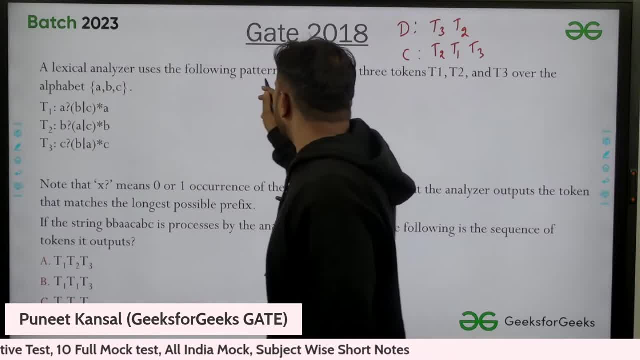 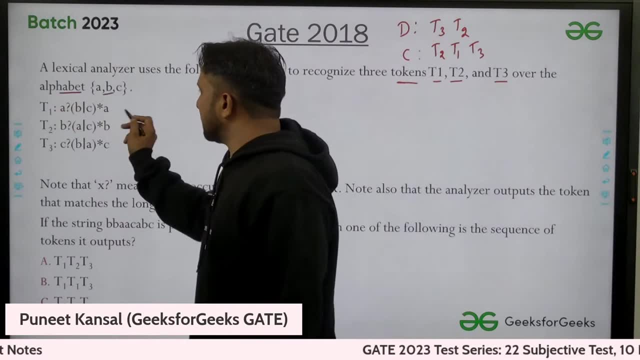 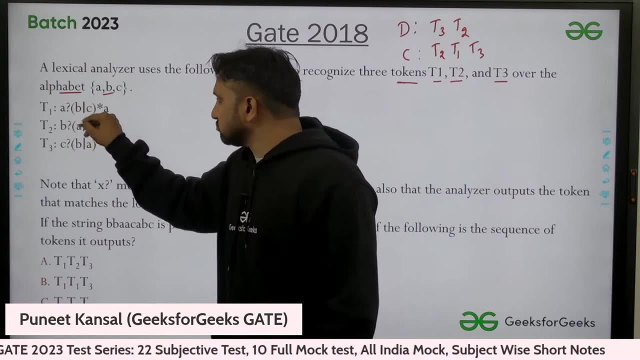 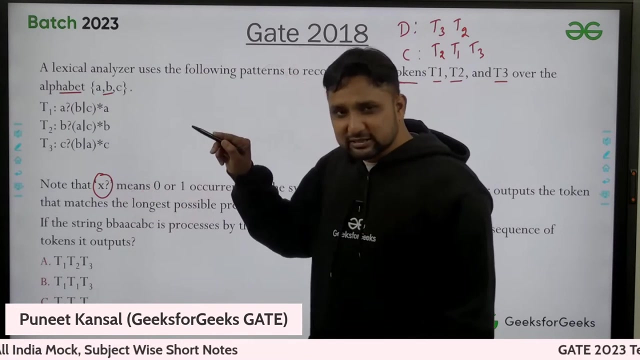 Okay, So a lexical analyzer use the following pattern to recognize the tokens T1, T2, T3.. So we have three type of tokens from these alphabets: A, B, C. And here important part is here is that they are telling us the meaning of this A question mark. Okay, What is the meaning of this? Let's suppose X question mark is. This means either I will consider X or I will not. Either I will consider A or not, Yes or no, Zero or one. 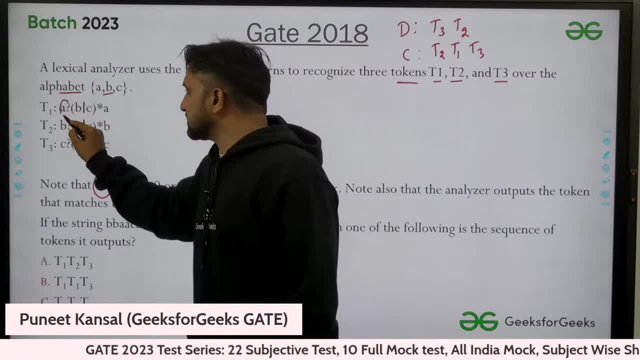 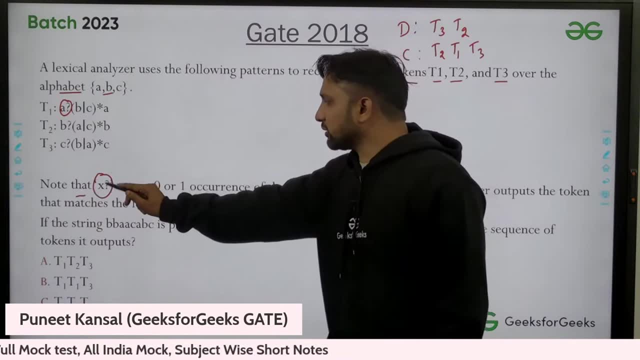 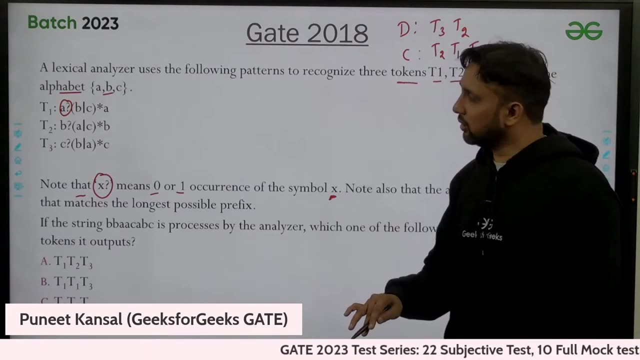 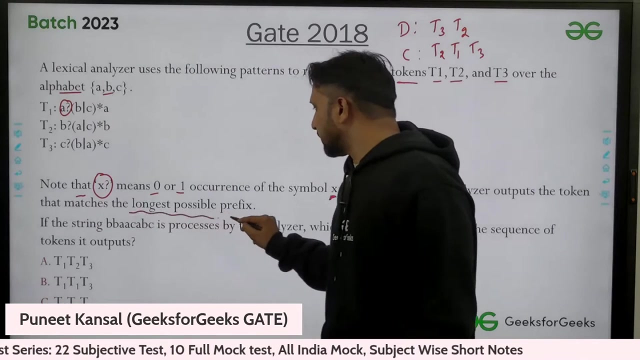 I will consider the occurrence of A. This is telling me Either I will not consider Similar for B, similar for C question mark. So this statement is telling this thing. Note that X question mark means zero or one occurrence of symbol X. Either X will occur or not occur. Okay, So note that. Note also that analyzer output the token that match the longest possible prefix. We already know this thing, otherwise, 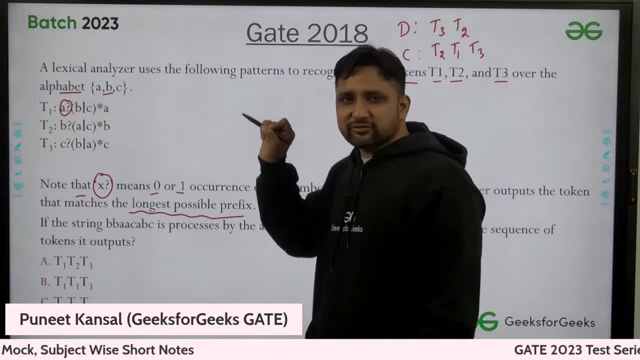 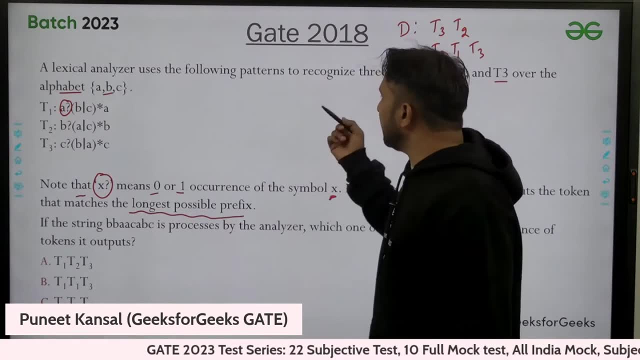 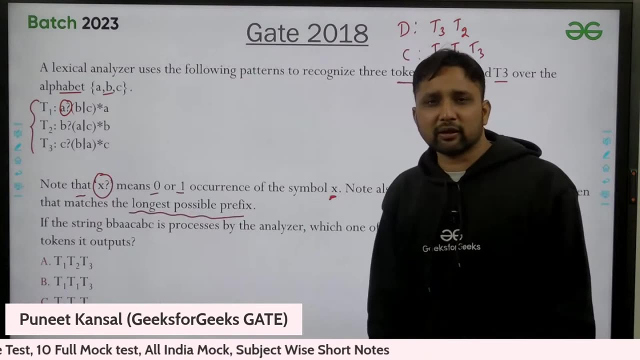 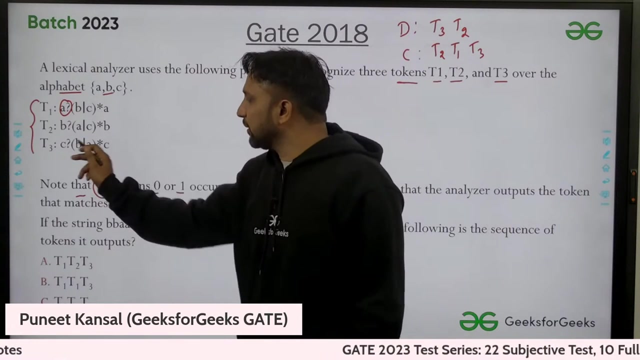 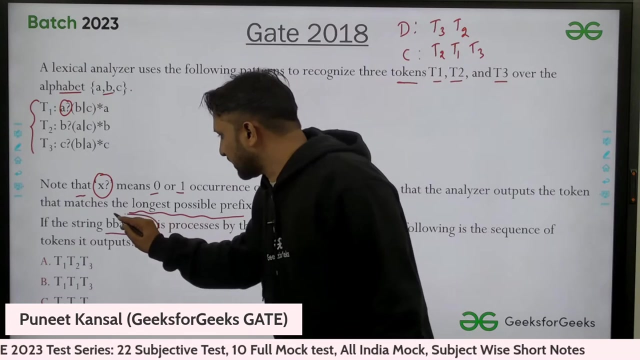 Lexical analyzer always find out The longest one, Longest one as a token, that recognize the longest string as a token which he can match. So we design a compiler, let's suppose, And we say that these are the three tokens in my compiler Compiler can recognize these three tokens. Okay, I design these machines, finite state machines, for three tokens And then I give this string, This string I give. 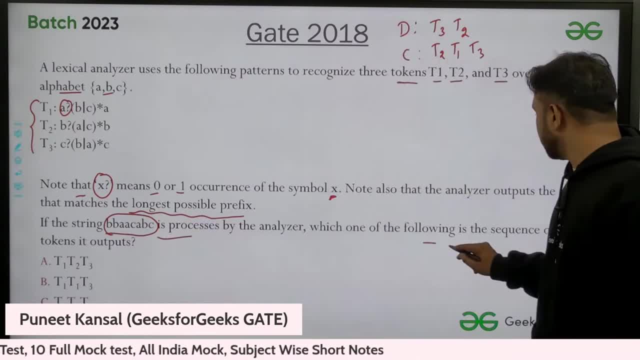 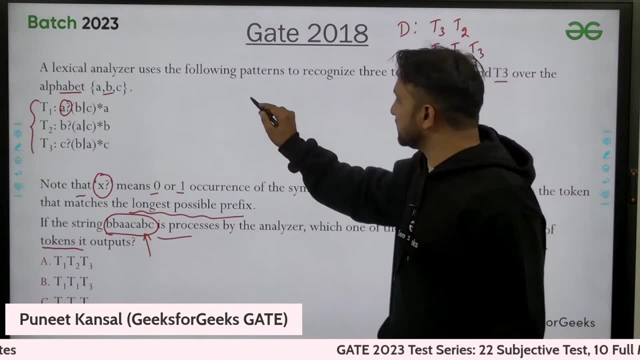 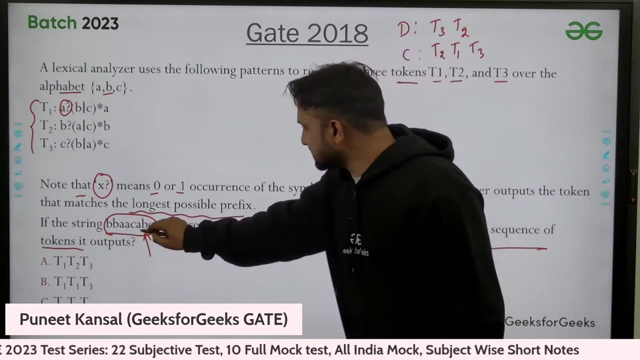 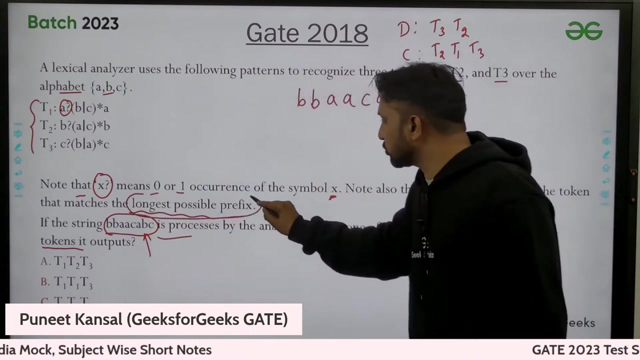 Okay. So first we need to find out. Okay, we need to find out which of the which of the tokens are there in this string. which are the tokens are there in the string? So let me write the string a little bit in big font over here: BBAA, CA and BC. Okay, so we need to find out the longest, longest possible prefix from this side, left side- and moving to the right side, and a finding the longest one can match over here. So let's say 겁니다: 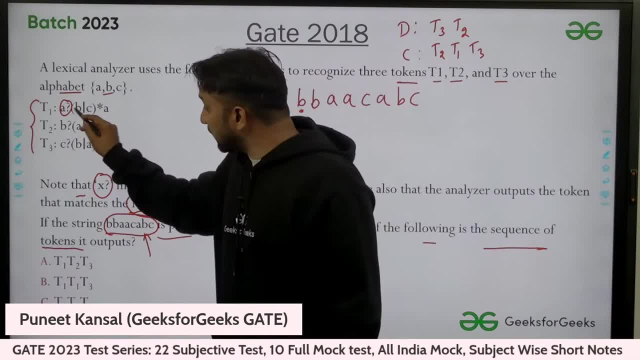 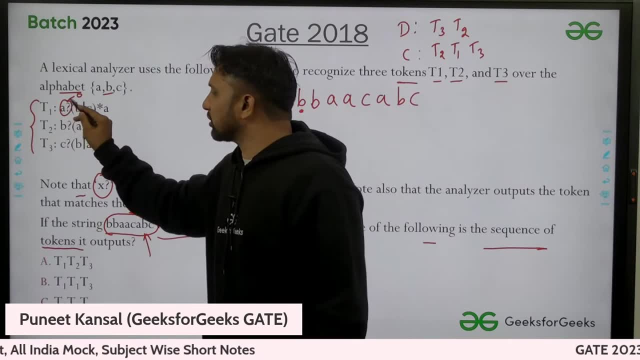 So first I get B, So B I can get from here, Yes, From here. also, how I will get B from here, I can make this as 0.. I can say that: okay, I am not considering A, So I can consider. 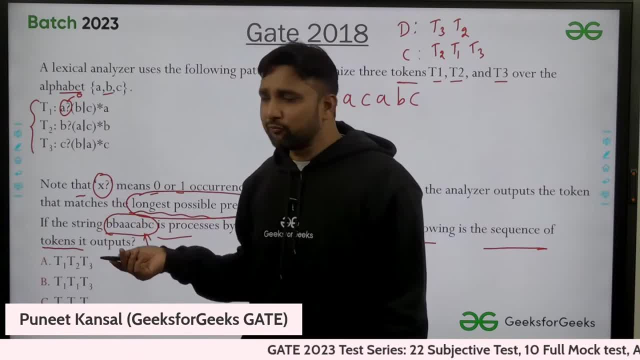 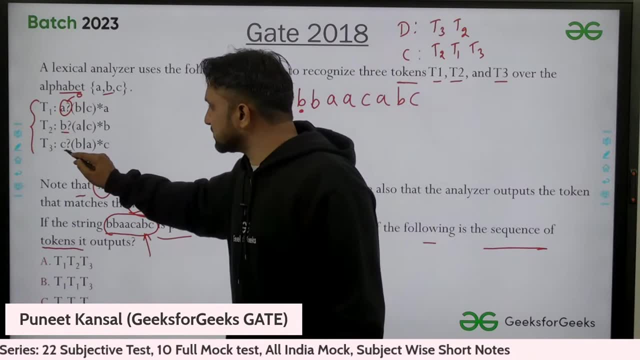 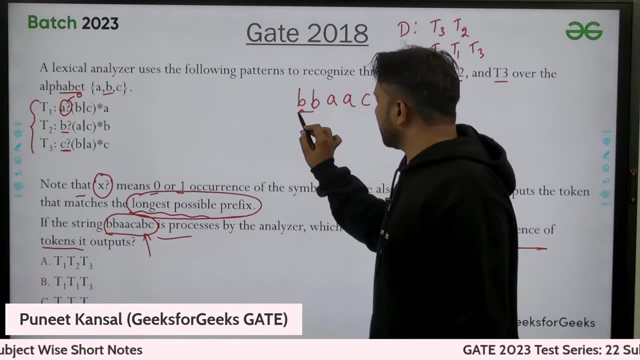 B from here. Okay, I can consider B, any number of B or C- from here, So I can consider B From here also. I can consider B From here also. actually, I can consider B. I can consider this as null nothing, And from here I can consider B. Okay, After that, but I am looking. 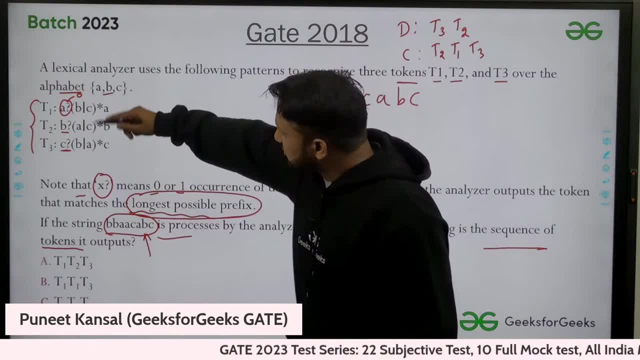 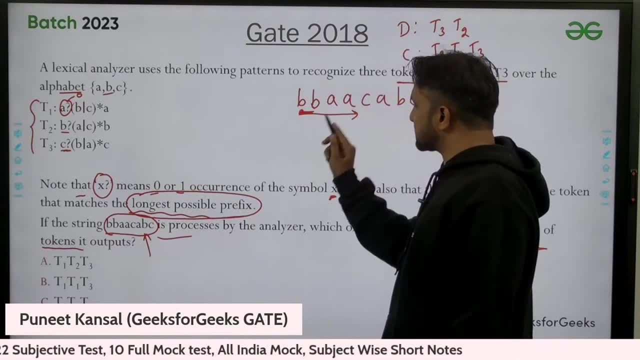 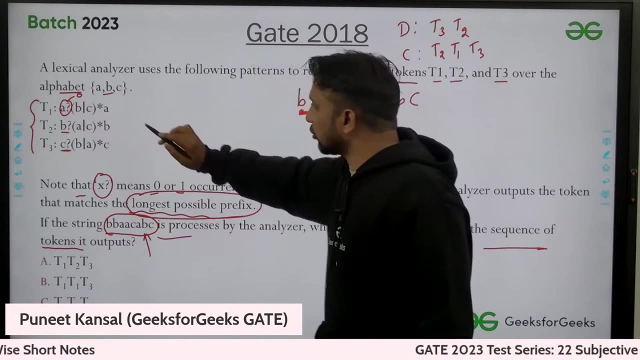 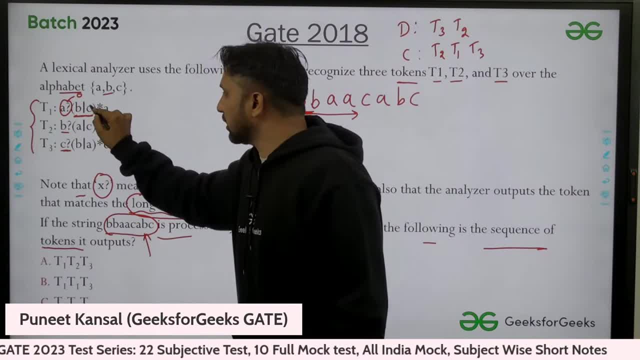 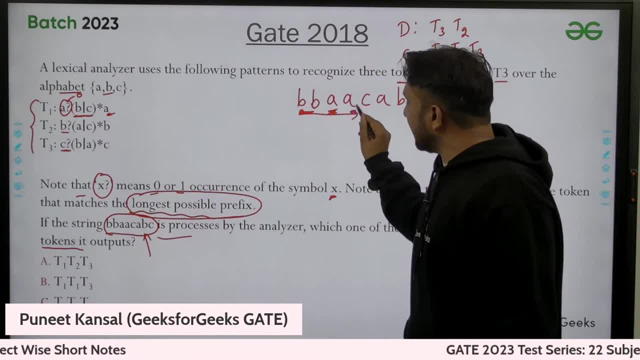 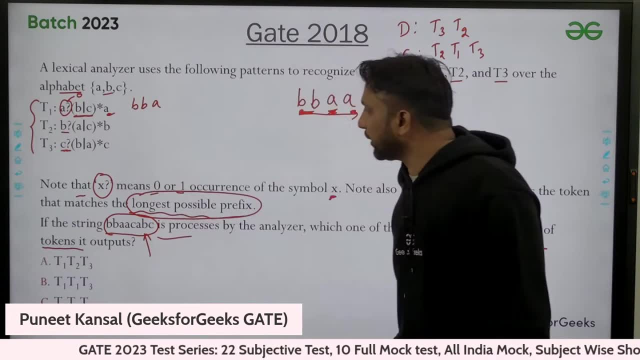 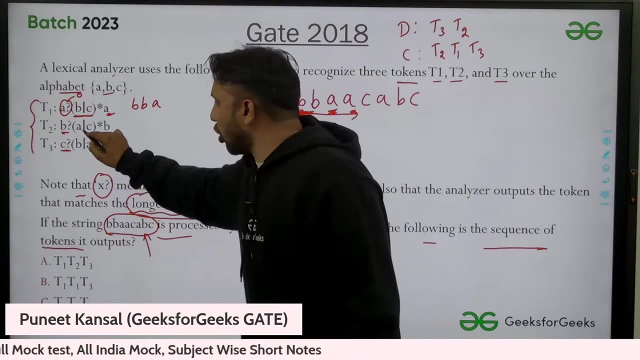 from here: this A, But the second A I cannot generate. So maximum substring which I can generate initially from this token is BBA. Okay, And let us check out from here. From here I can generate B. Yes, First B, Second B- no, I cannot. Yes, second B I can generate. 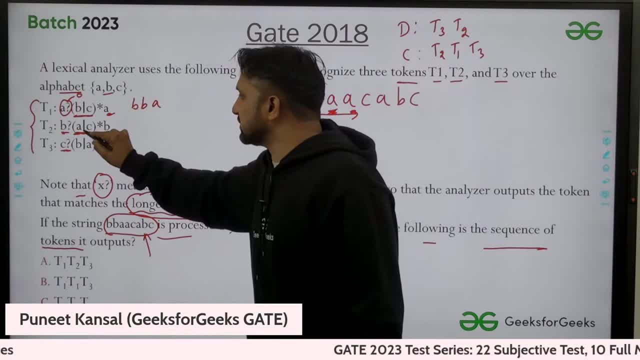 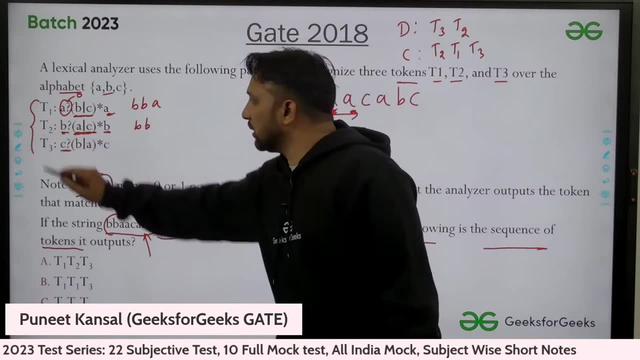 but from here I can set this to null, because star is here. So 1B, 2B, only 2B I can generate. So this is the longest substring I can generate from this token, And from this token I can set: 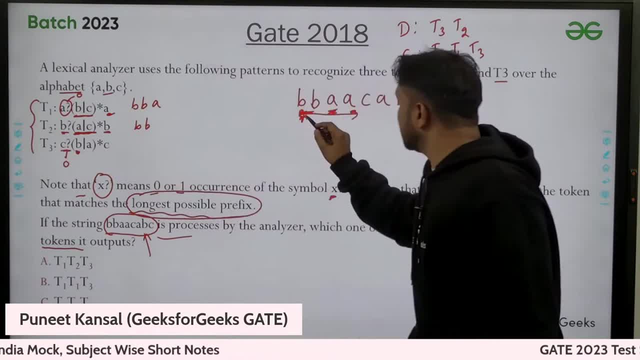 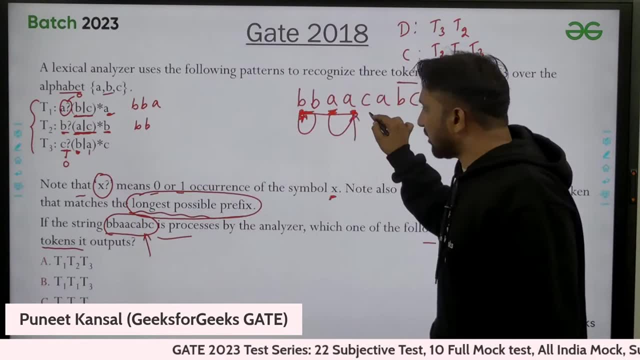 this to 0.. And from here I can generate 2Bs, first B and second B. yes, After that A. even I can generate 2A. yes, up to here. now, After that C. yes, I can generate C also after that. 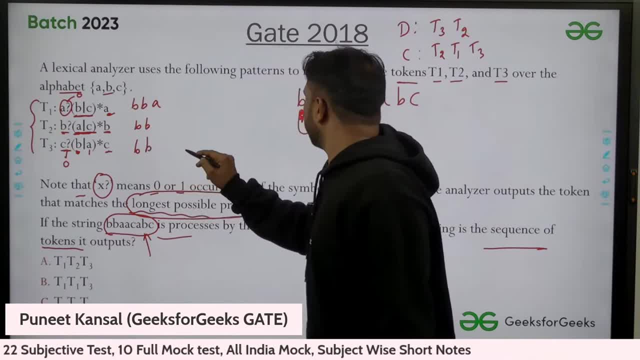 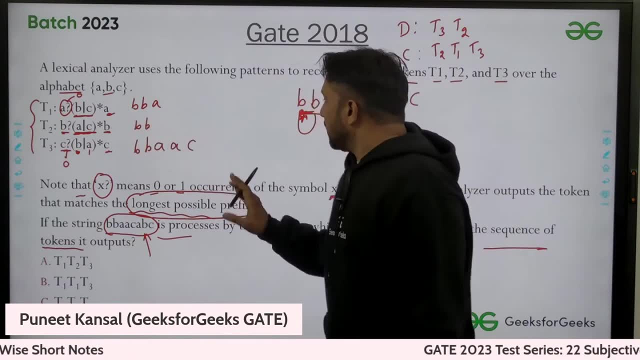 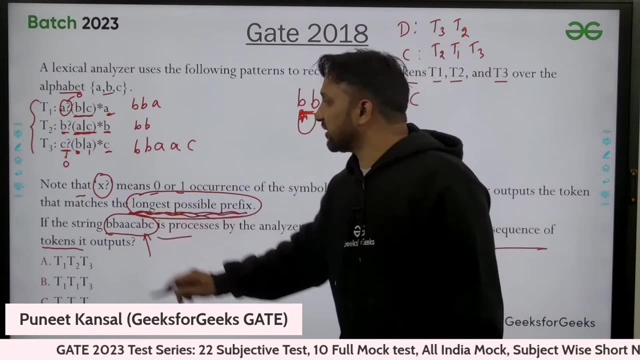 So from here this token from this machine. actually, I can generate this longest possible string, So, according to this statement, we need to consider the longest one, the tokens, which is considering the longest possible prefix. okay, So this can detect only this. 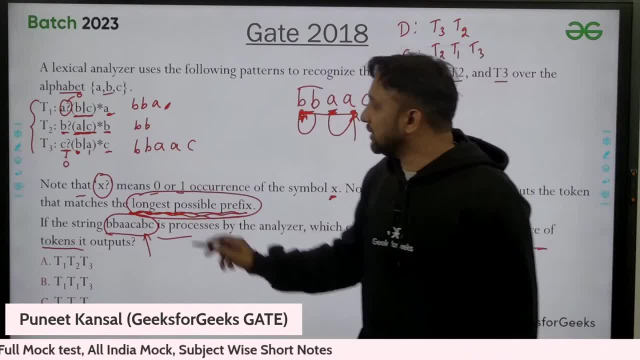 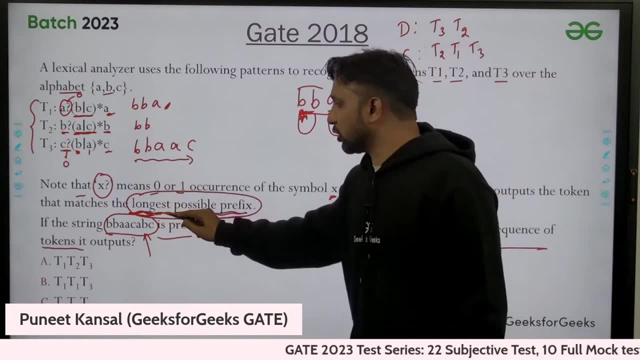 much. this can detect. only BB and T3 can detect up to this long. T3 can detect 5 character long prefix. So this is the longest possible prefix. So I need to consider the longest one. So first token, I will find out. I can say here: 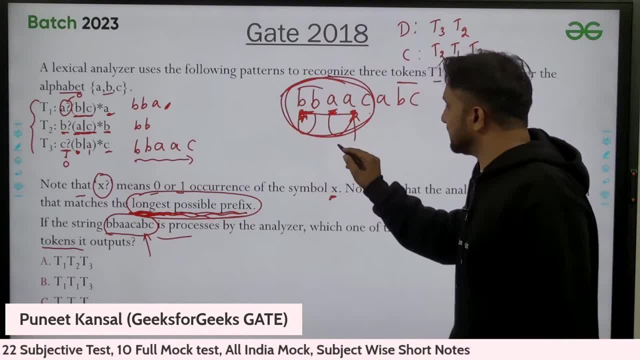 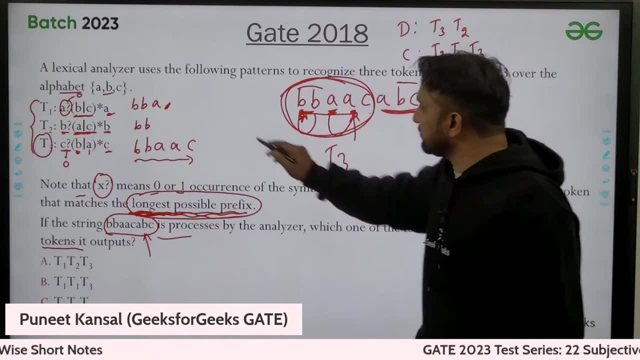 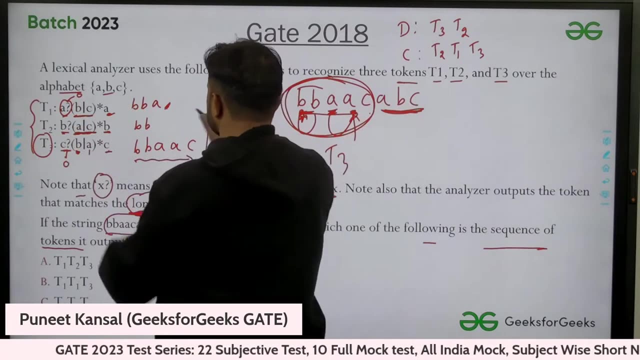 is this? First token I find out is this: This token is actually T3.. This token is T3,. okay, Now I need to find out this thing. Can I generate this thing from here? Let us see: A. A, I can find out here. B, B, I can find out C. no, not C, But A and B I can find. 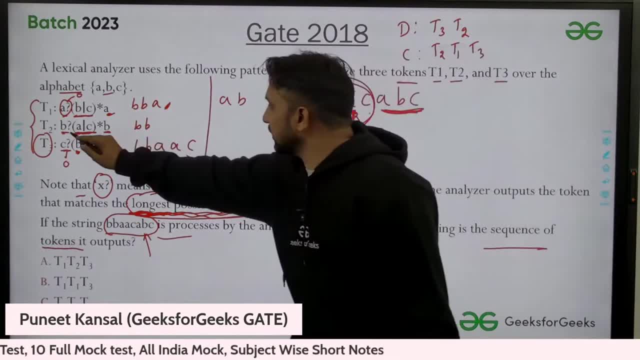 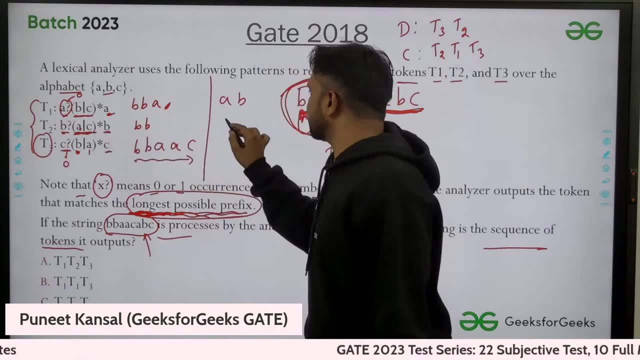 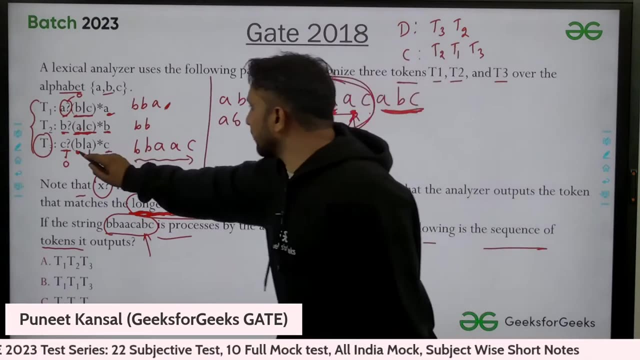 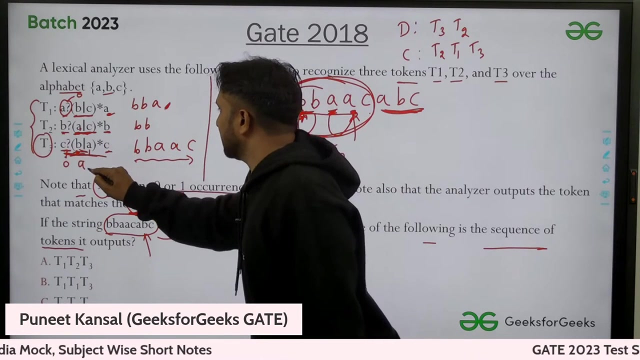 out in this: A, B, C Here. A, yes, B yes, C, no. After finding A and B, I cannot get C. So A and B here also, Yes, I cannot find out C. And what about this? A, yes, B, yes from here, C yes from here, Okay So. 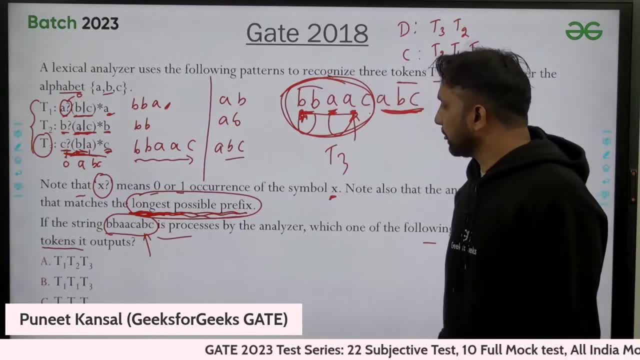 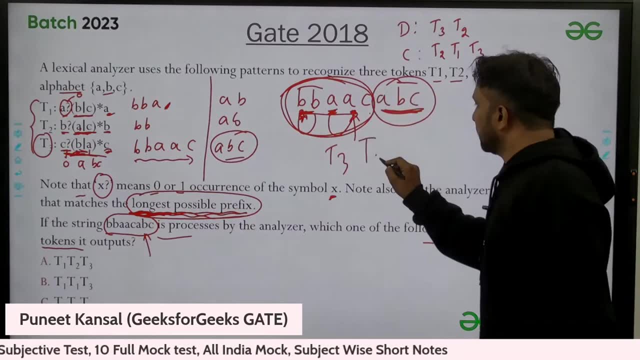 I can find A, B, C from here, T3. Okay, So longest string can be find out by T3.. Longest string can be find out by T3.. Okay, So from T2 and T1,, from T2 and T1, I can find. 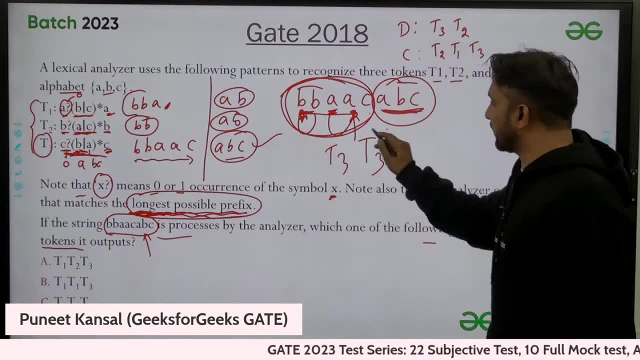 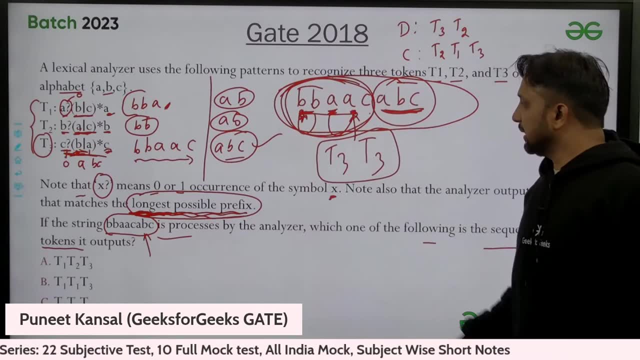 out only two characters, But longest one is find out by this one, So I will consider this one. So in this string, I can say that, according to these statements, these are the tokens I will find out. These are the longest, these are the tokens which is helping us to. 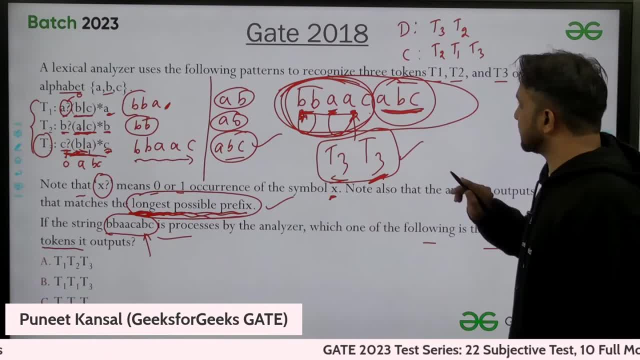 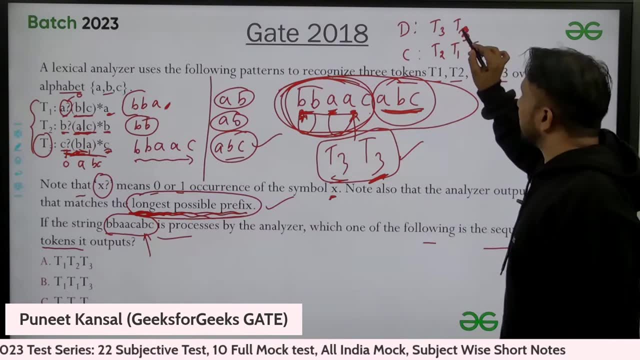 find out the longest prefix. Okay, So this is the answer. So D should be the longest prefix. Actually, 3 must be here. If we, I do not know why you are giving the D as an answer. if I write T2 here, I cannot write T2 here. T3, T3 must be the answer. T3 must. 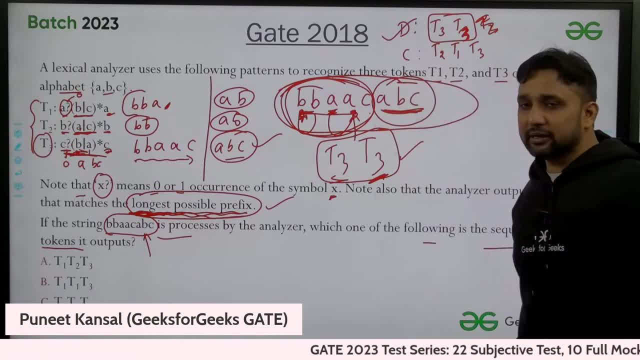 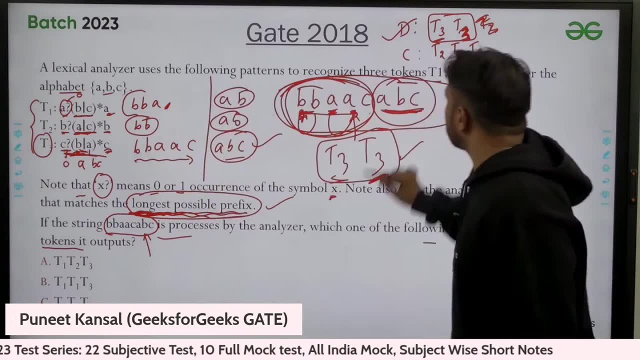 be the answer. So D is the right answer here. D is the right answer, But the option should be T3, T3.. And the option is T3, T3 only. I was not able to read here, So option is: 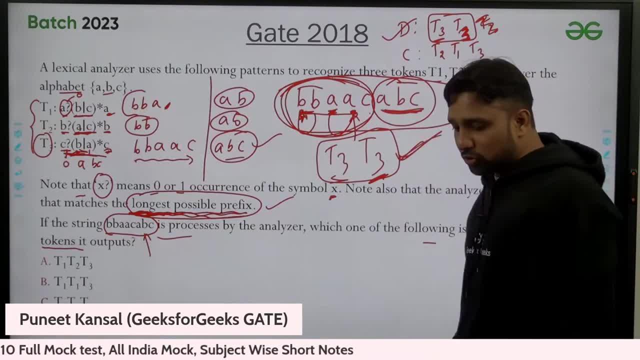 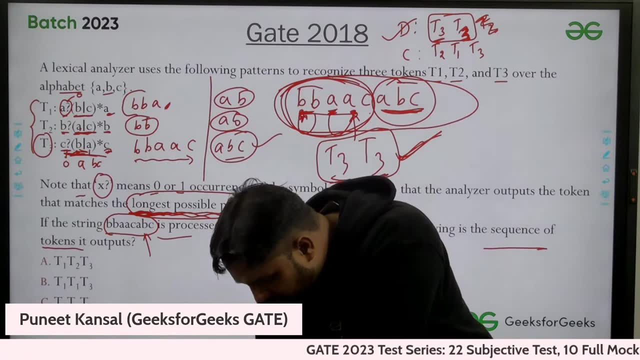 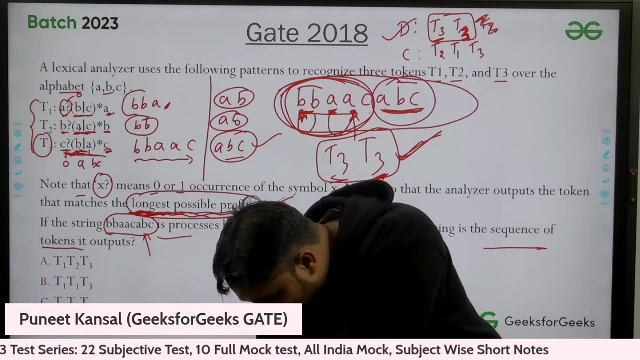 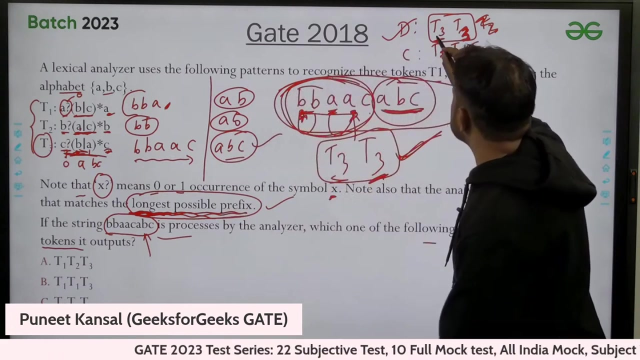 T3.. And this is the tokens we find out. If any doubt, please ask, And we what is your answer? You are wondering why your answer is not matching, but where is your answer? Let me check. Okay, you D is the right answer, but this should be T3,. 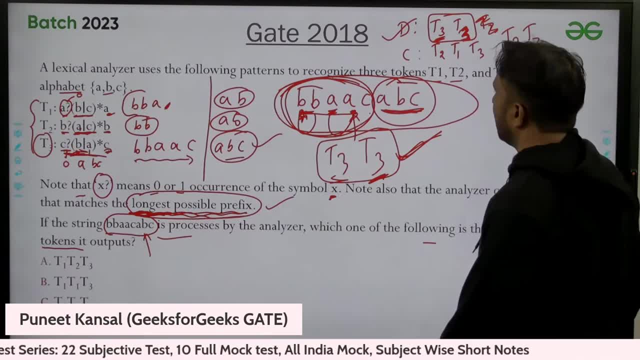 T3. But T3 and T2, you cannot say Why. Because you cannot say So. you cannot say So, you cannot say Why. If you are considering T2,, okay, you are considering, okay, this as a. 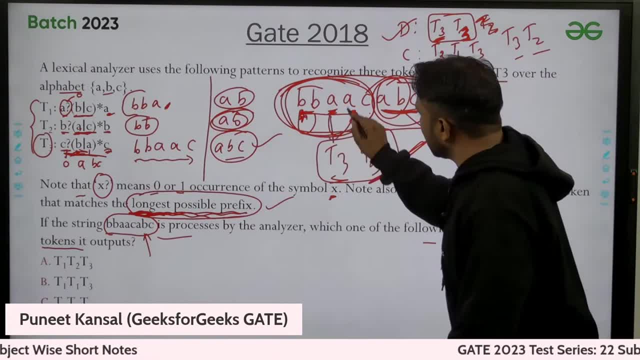 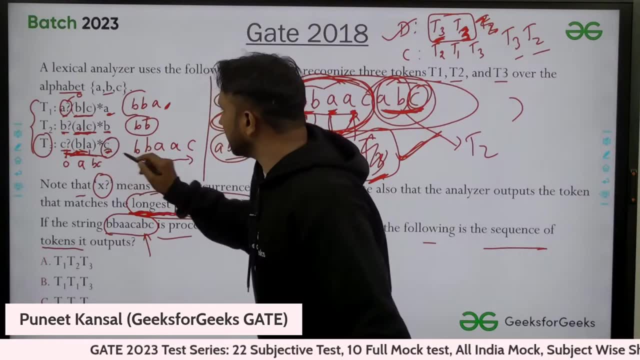 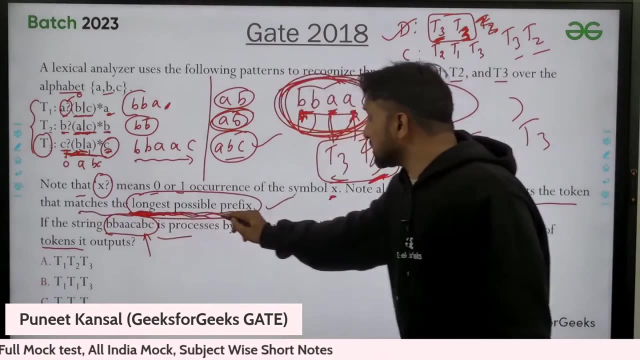 token. now. This will be T2 token. This is T3 token. this one Now for this also, you need to consider a token For this. you can take actually this token Again, T3.. But according to this statement, we need to consider longest possible. we need to consider that token which. 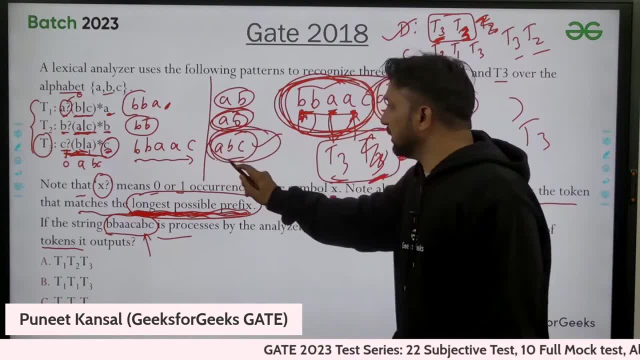 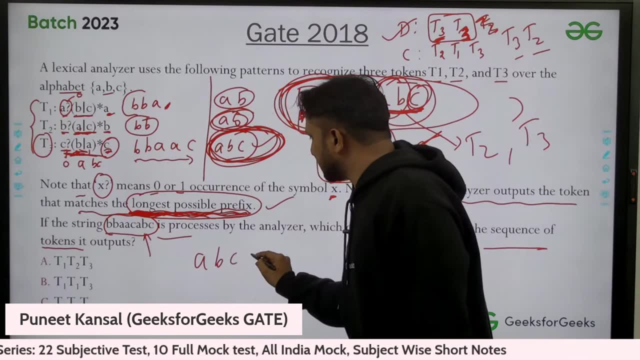 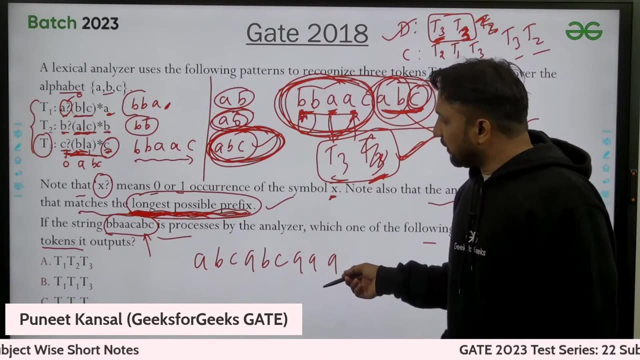 is considered longest one. Longest one is considered by the this T3.. Longest one is considered by the T3.. You can take another example also. If I write like A, B, C, A, B, C, A, A, A, I can make any question out of here. So here I can say: okay, which. 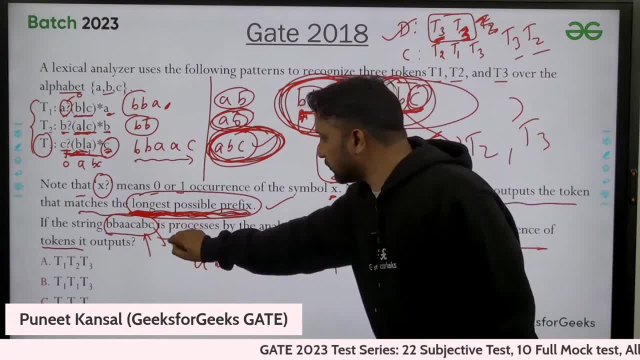 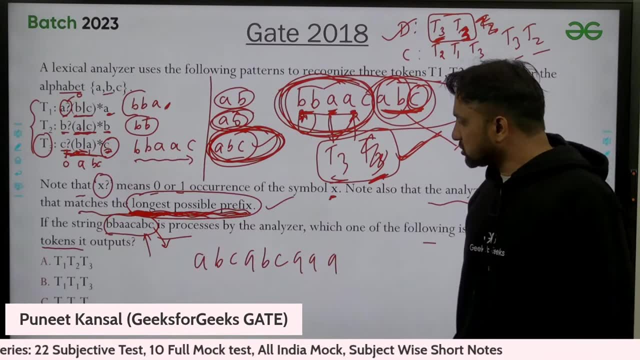 are. the long same question with this is: this is the input string. Now, which are the tokens? Can you tell me which are the tokens? Please try again. Okay, please try again. Which are the tokens? you will say that, okay, that should be the right token, Can you people? 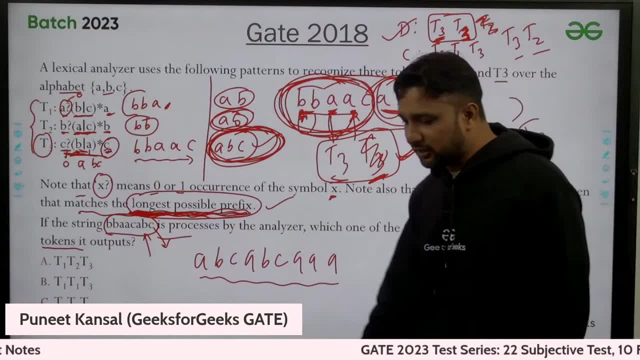 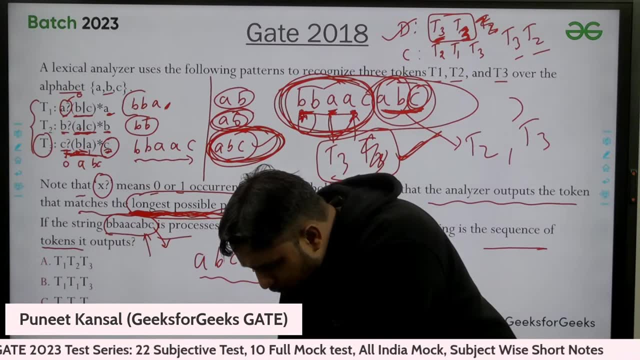 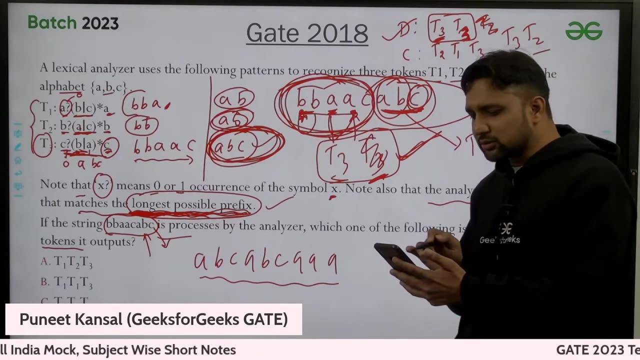 tell me For this string, please try, please try. Harshay says that if you people try this, otherwise I am taking some question from chat box. If T3, Harshay says that, if T3 and T2 are the options, then what is the possible? 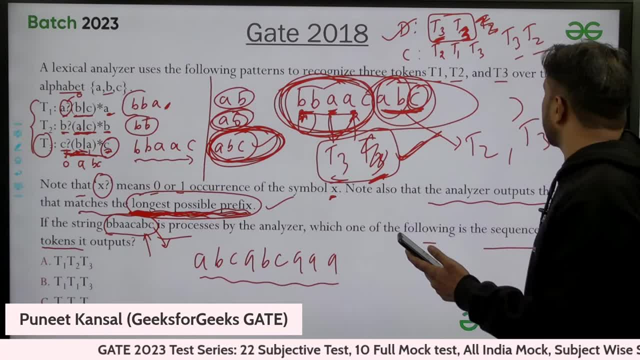 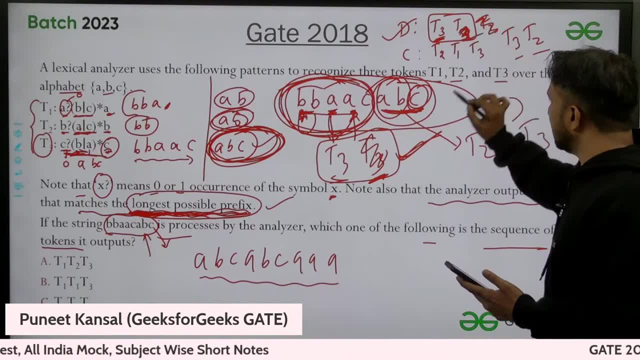 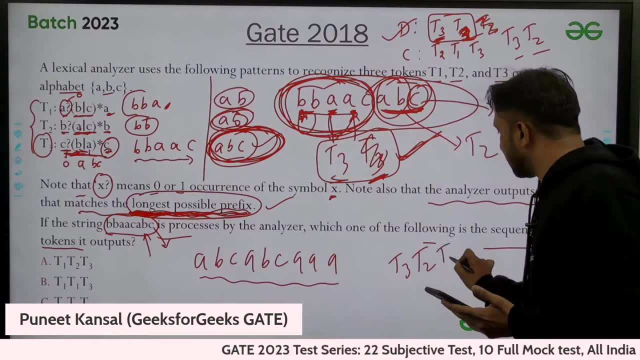 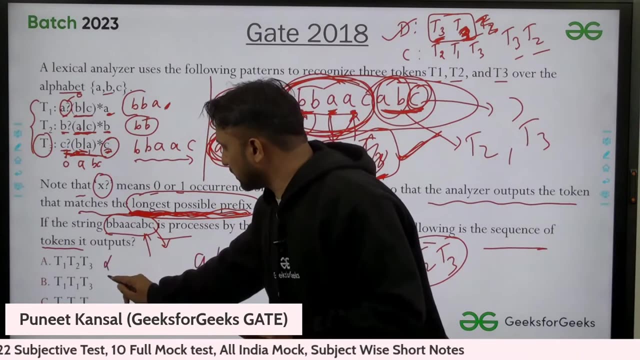 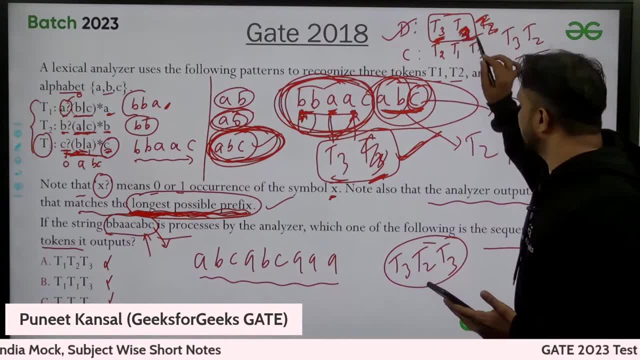 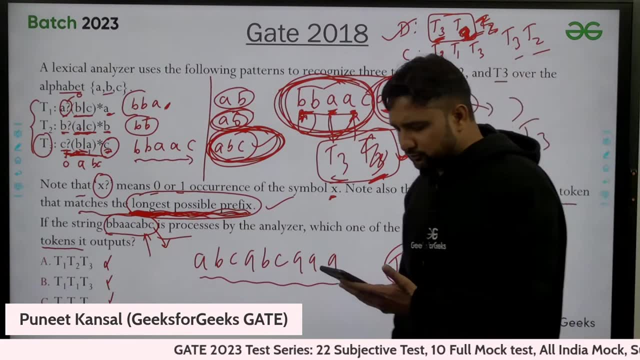 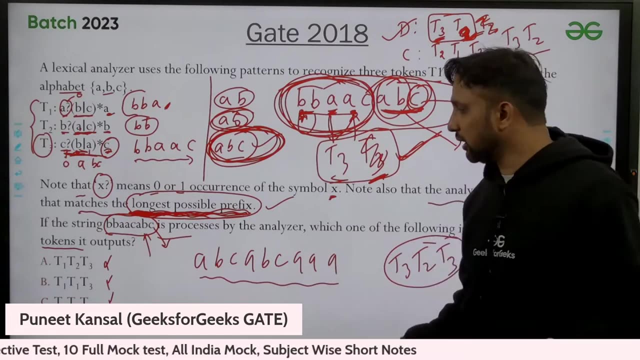 is satisfying the answer. No option is satisfying. If I can say no option is satisfying the answer, Okay, If T3, T3 is not given, then I, I, I can say only one thing: No option is satisfying here. 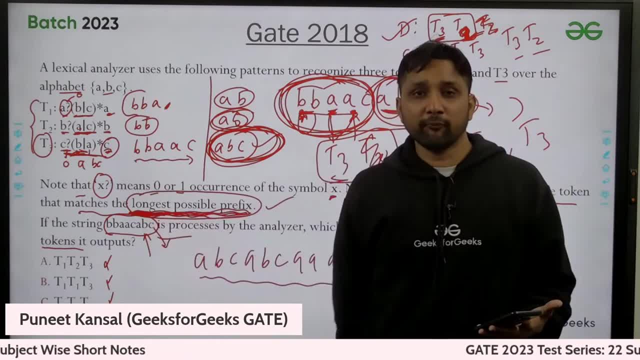 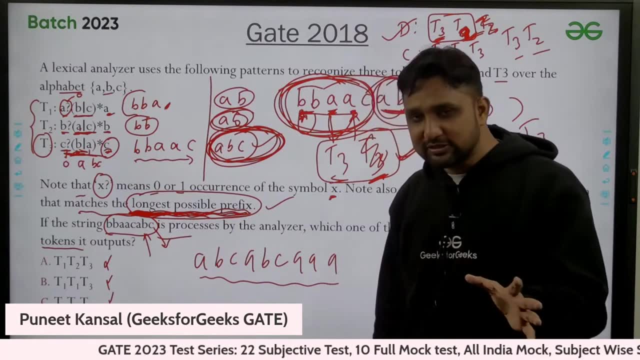 as answer. Otherwise they need to give one more option. none of the above, Otherwise the option is wrong, And this is this also happens sometimes in GATE exam. None of the options is actually is right And they give marks whoever attempt the question, whoever. 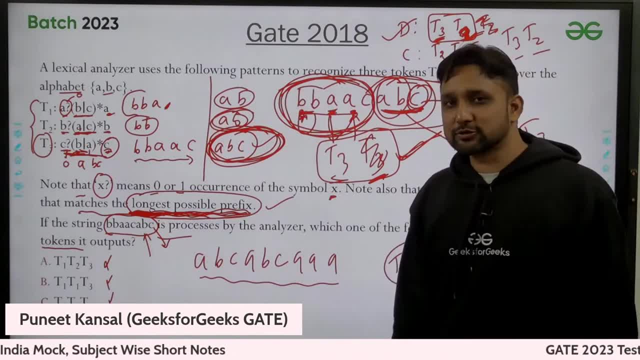 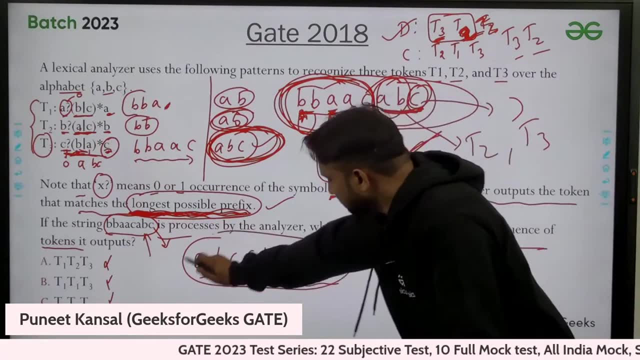 write the any of the option, everyone get the marks for that question. This also happens in exam, Sometimes like this, Sometimes like: but For this you are trying, So we already get the answer. T3, T3, T1. 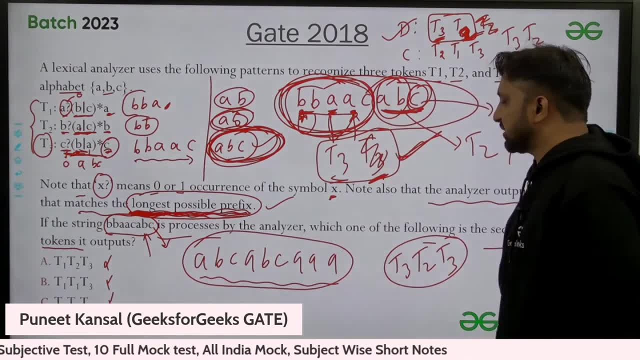 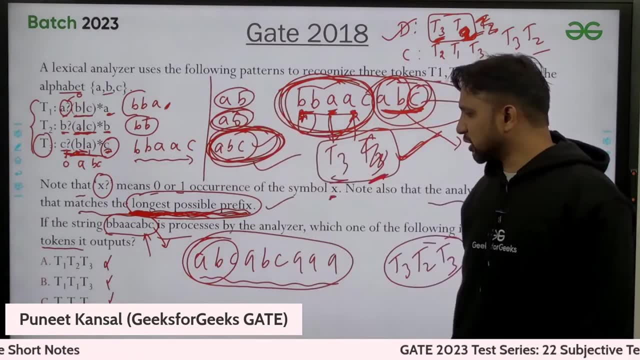 from Divyanshu. I think Divyanshu is right. Yes, Divyanshu are right. So this is the longest string I can generate, which is can be generated from T3 itself. You can check out here Again: T3.. This can be generated triple A directly from here, Because this: 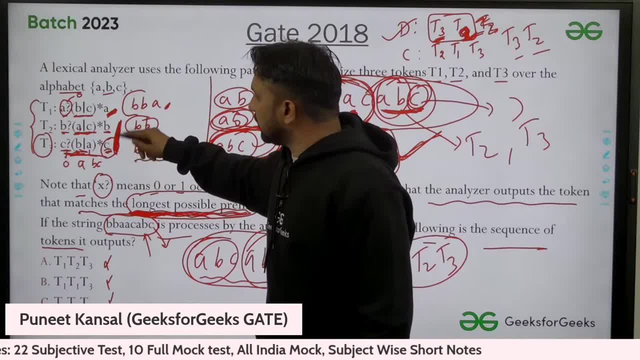 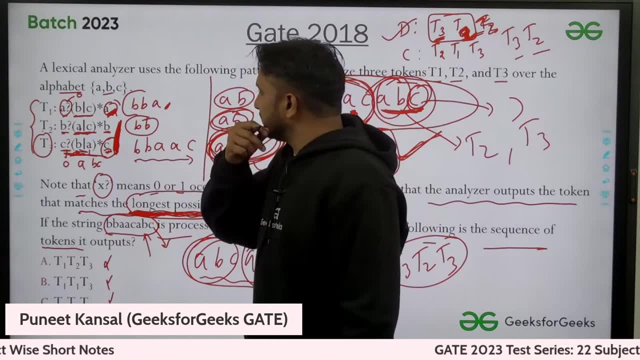 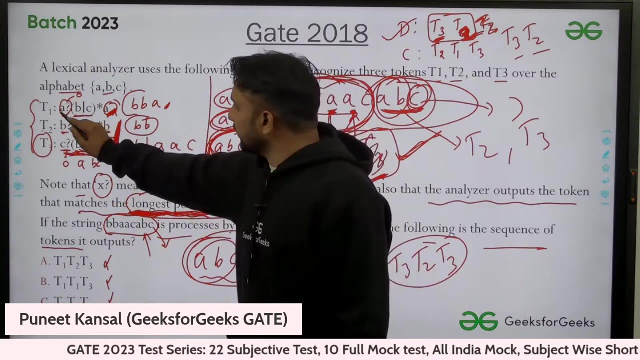 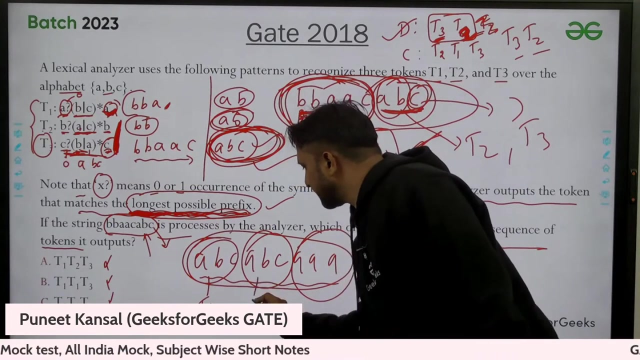 is ending with A, No other, no other token. T3 is actually ending with A. We need to consider this only. But but wait, We have triple A, So we can generate 2 A from here. But we need to take even this is T3.. This is. 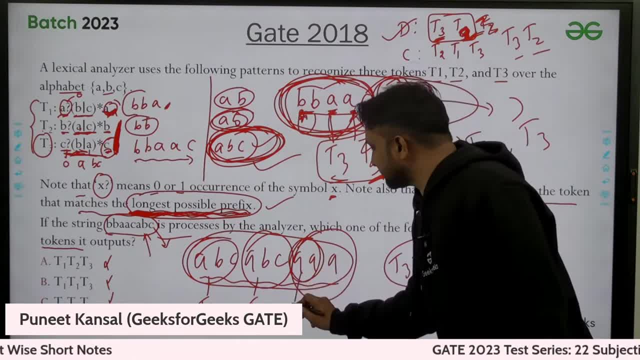 T3.. This is, I think, this is T1.. Again, this is T1.. So this will be the answer. You cannot say you cannot generate 3 A from here. This is T1.. This is T2.. This is T3.. This is T3. 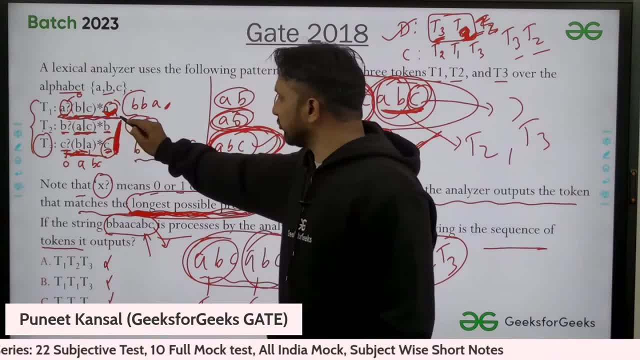 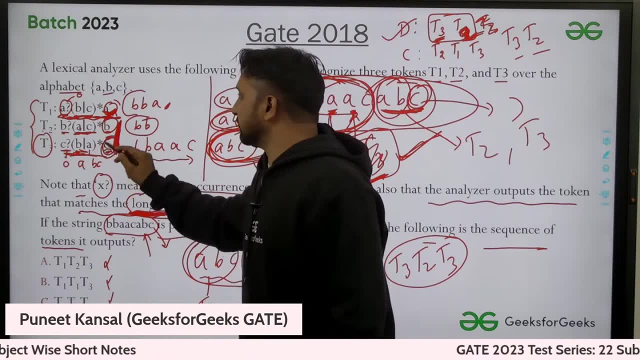 Can you generate 3 A's from here? Can you generate 3 A's? No, We cannot generate 3 A from here. We can and no other we can use actually, Because all are having ending with B and C. We need to use T1 only, But in T1, you cannot generate 3 A's We can generate. 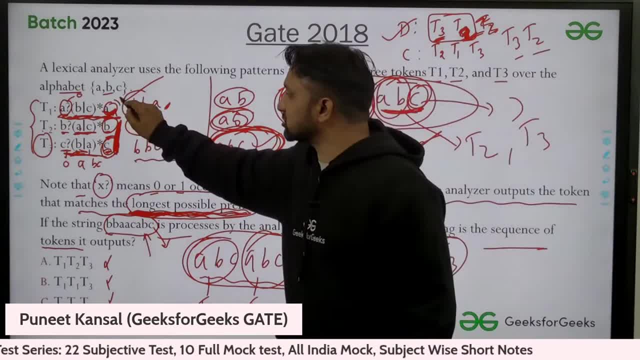 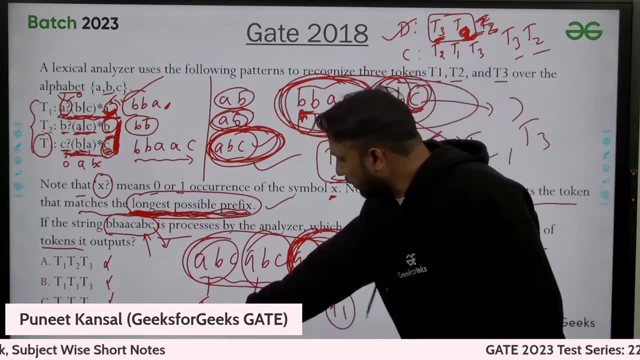 at a time 2 A's only Because A is not having star closer anywhere. I can consider 1 A and 2 A, And last A is also generated by T1.. So the answer should be T3,, T3, T1, T1.. 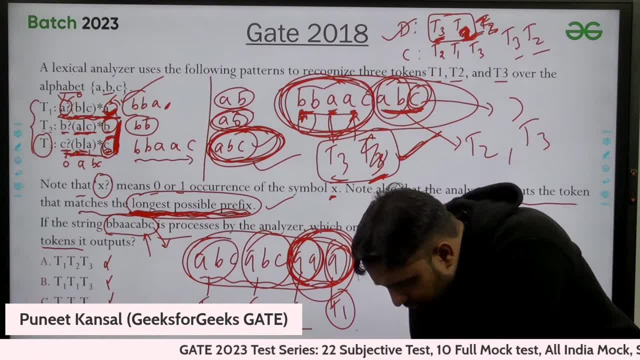 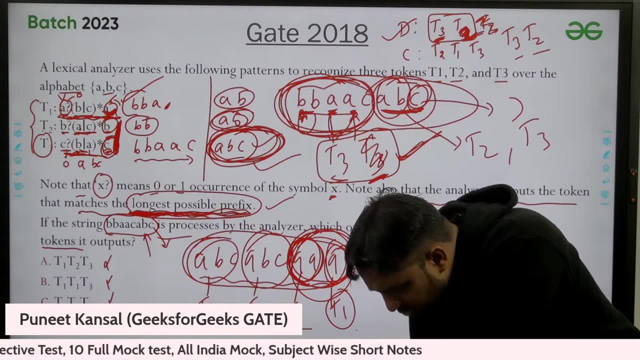 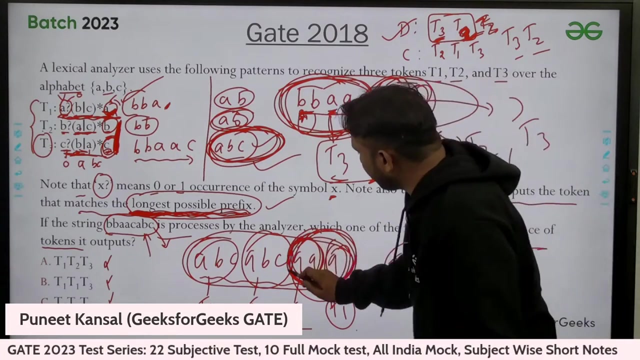 Yes, Vir, you are right. And sir, should not it be 3 times T1?? No, not 3 times We are. we can generate 2 A's actually from T1.. 1 A, we can consider this, 1 A, we can. 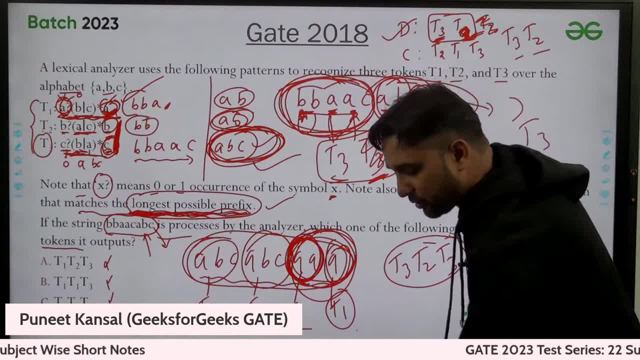 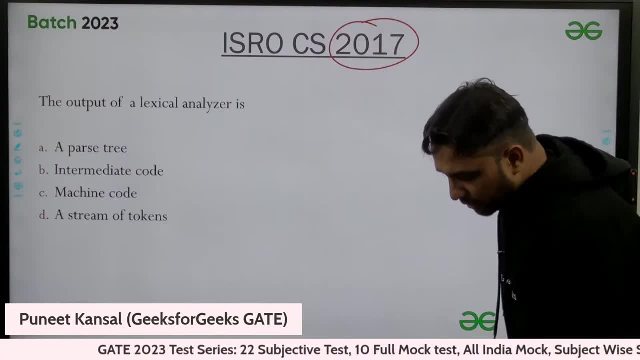 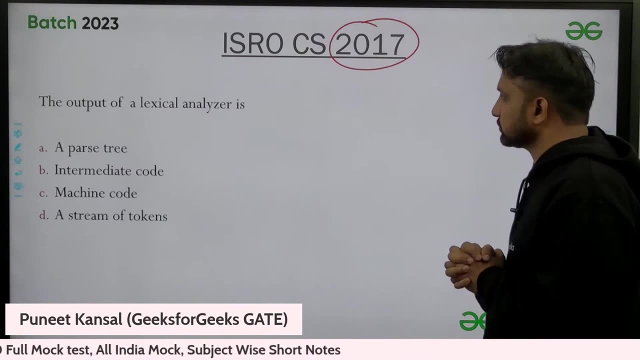 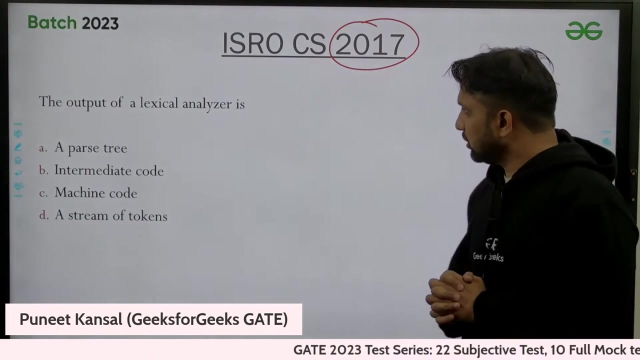 Okay, Okay, That's it for this question now. We have spent so much time over here. Please try this one. It's for 2017 one. Let's try to cover maximum questions. Please give answer fast now, Everyone. please give the answer fast. So what is the output of lexical analyzer? 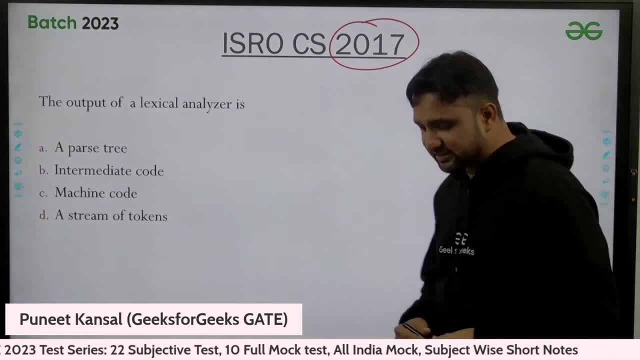 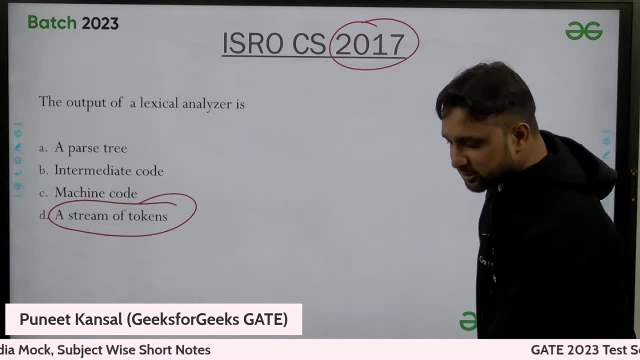 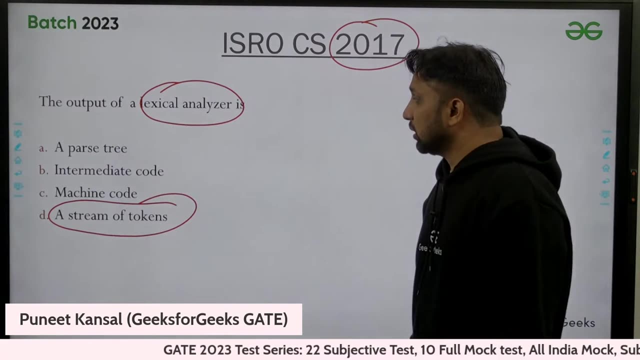 What is the output of lexical analyzer? We already We already discussed this thing And you are giving right answer already: A stream of token Token stream. A stream of token Token stream. That is the output of lexical analyzer, which is the first phase of the compiler. We are not talking about the we. 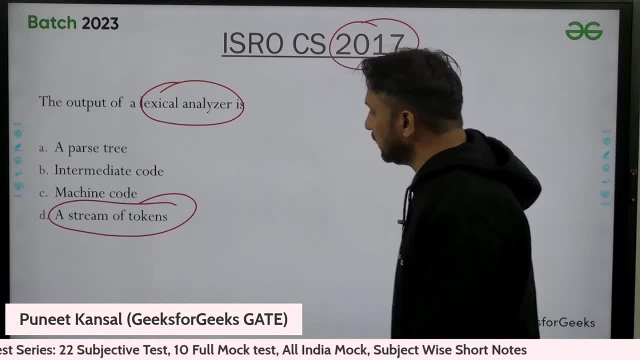 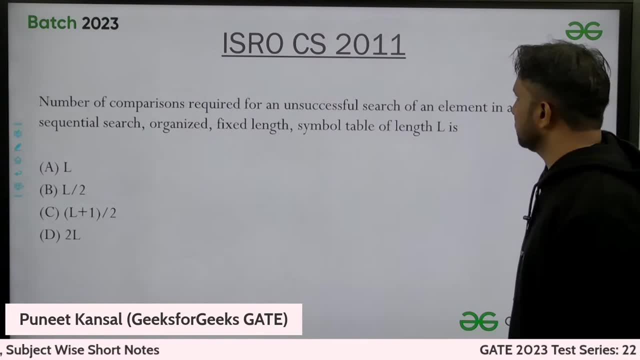 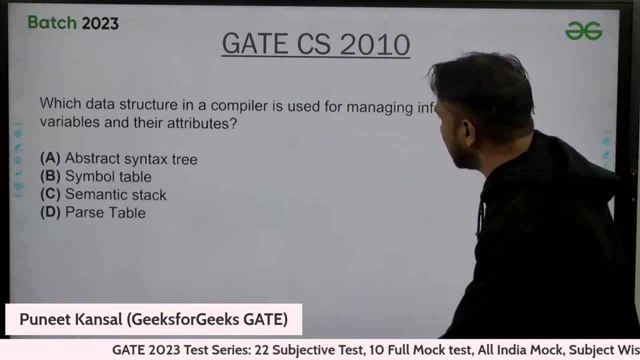 are not talking about the compiler output. We are talking about the one phase of the compiler output. Okay, So these are the right answer. Check out this one: ISRO 2011 one. Okay, Okay, So let me check out if there is other question also. So this one is also easy one Which? 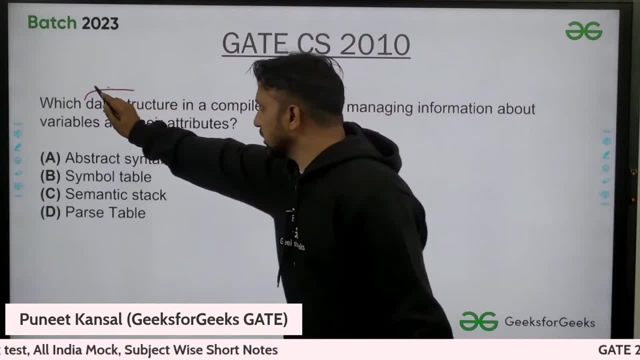 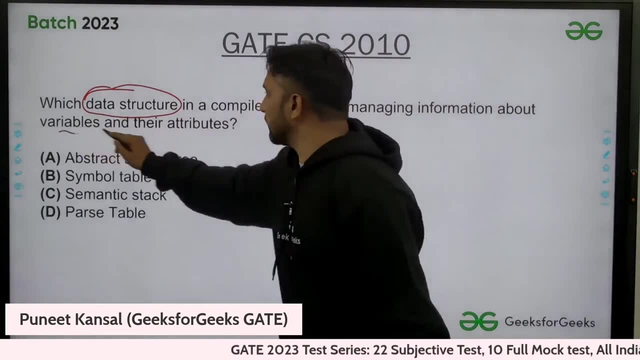 of the data structure. I will come back to previous question. So let's cover the easy one: Which data structure in a compiler is used for managing the information variable and attributes? Which data structure is usually in the compiler To manage the variables identifiers? 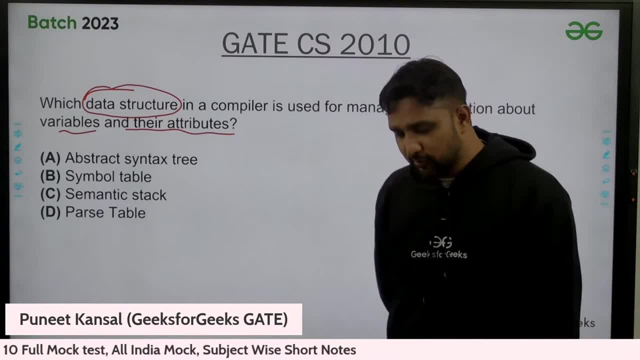 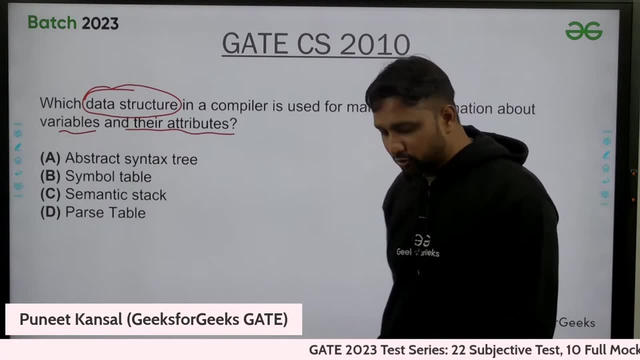 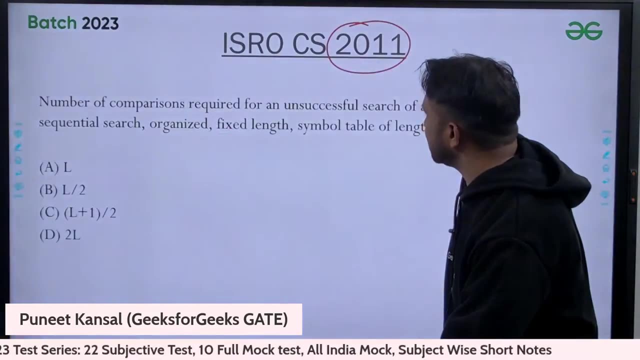 You people know. You people already know. Okay, Okay, So we get the answer also from you. you are giving the right answer. symbol table: yes, That's it actually. one more question was left, this one, you can take snapshot of this. 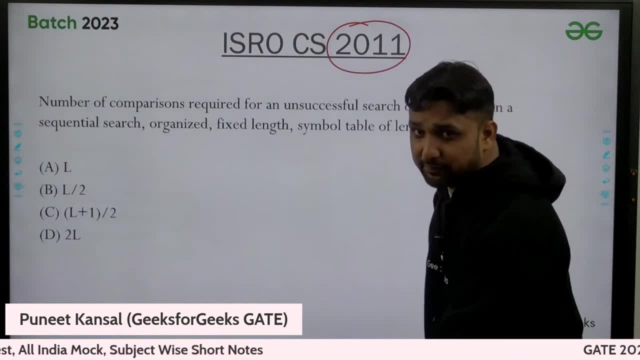 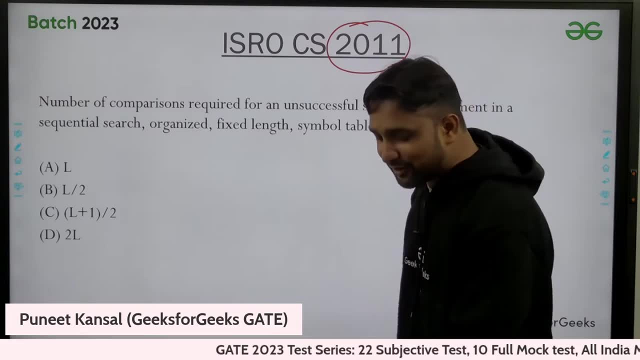 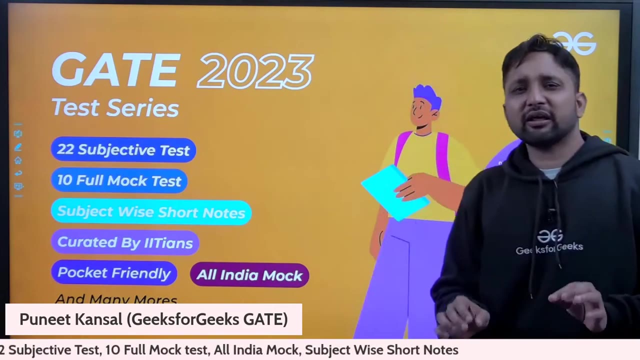 question and you can write the answer in the comment section. please write the answer for this question in the comment section, not in the chat box, so that I can also get benefited. Okay, that's it for this session, and we have covered each and everything about lexical. 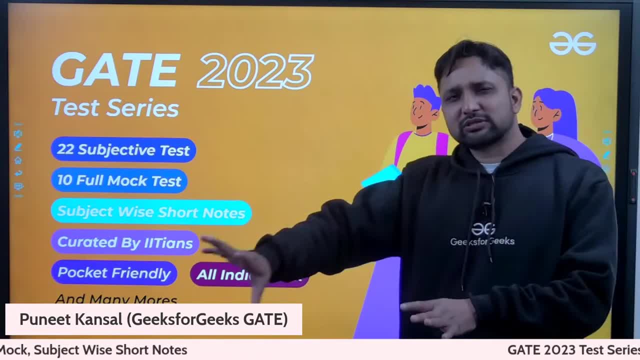 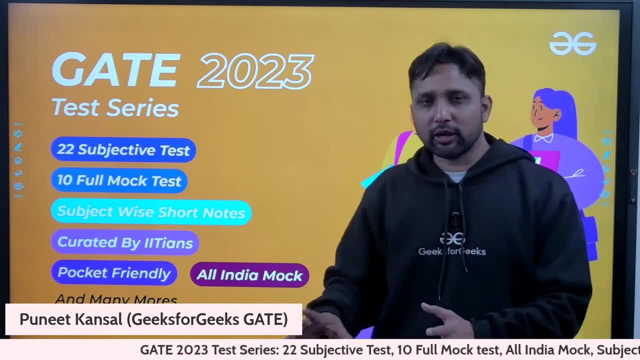 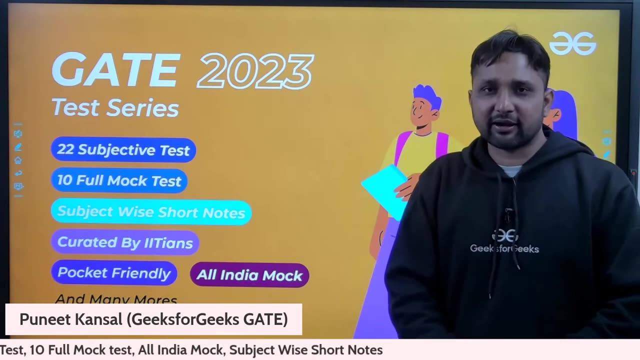 analyzer through, maybe by using the concept, by discussing the concept, or maybe by discussing various examples, or maybe by discussing the gate questions also. but we have covered each and everything. Now you do not need to know, you do not need to go anywhere else for lexical analyzer. 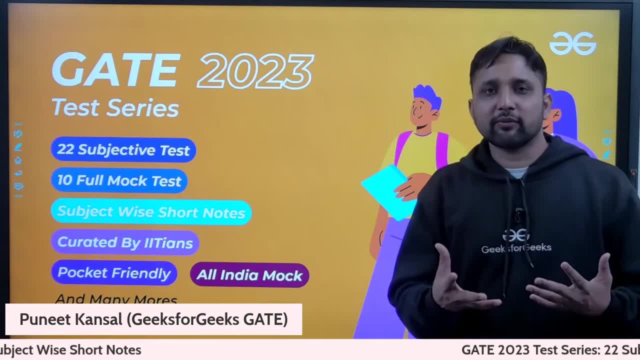 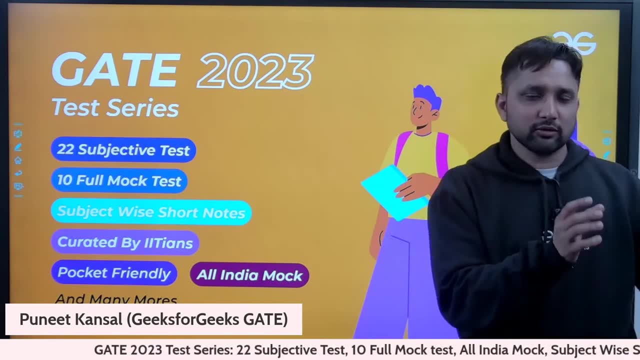 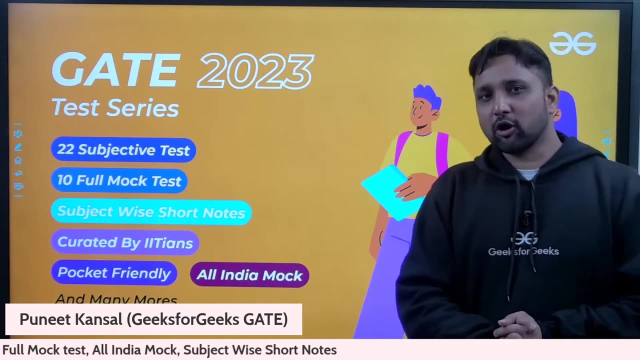 it's better now you just take the questions. You can try to find out the question from lexical analyzer. this lecture was sufficient for answering every question actually. now they will make little bit tricks everywhere and I hope you will be able to solve each and every question now from lexical analyzer. 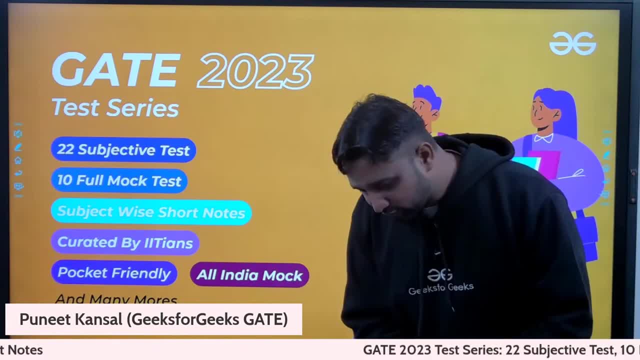 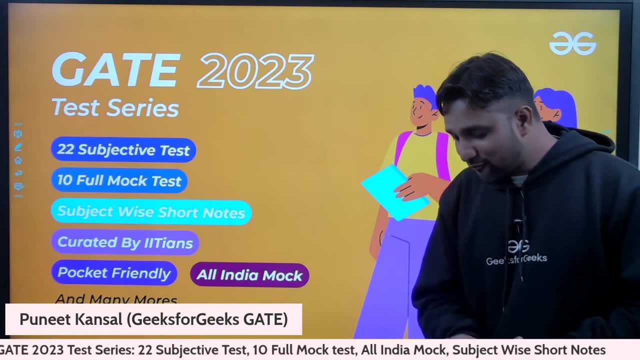 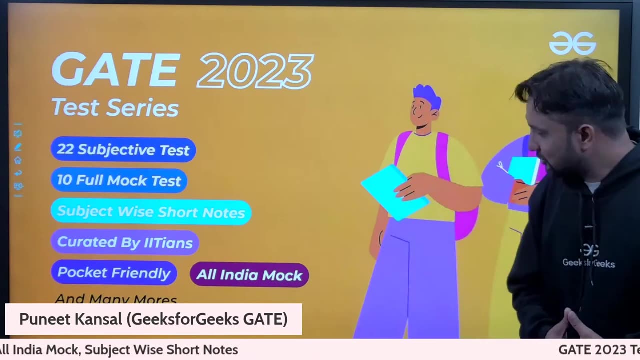 So, thank you, thank you everyone, for keep joining me for such a long time. for two hours you are continuously with me. you do not go for lunch also, so now we can eat the lunch and we can sleep. Anything else to ask? 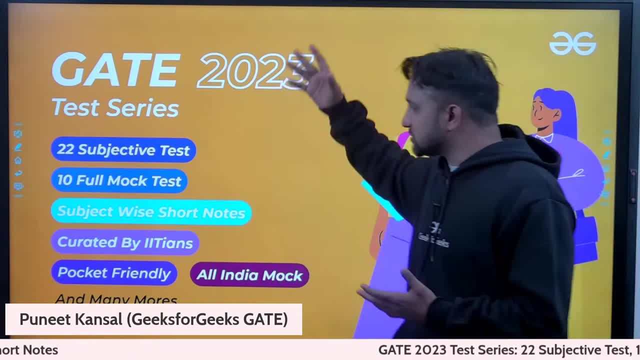 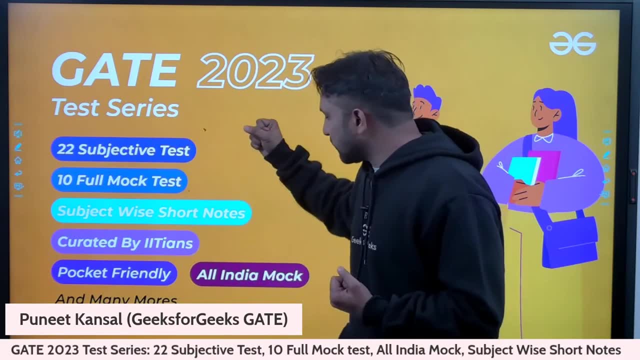 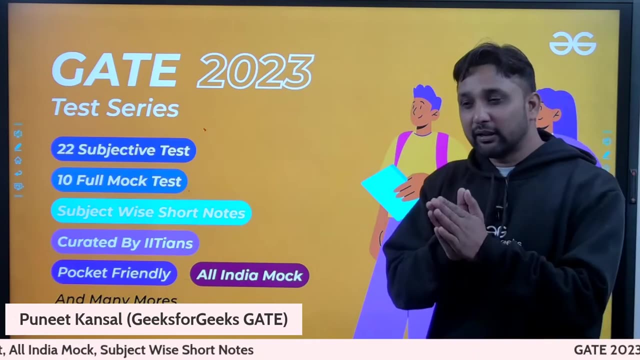 So this is the gate test series from GeeksforGeeks site. so much subjective test are there? ten full mock test are there? so many things are there, and that is also pocket friendly, so you can go for this test series also, which will bring, which will raise your level actually. 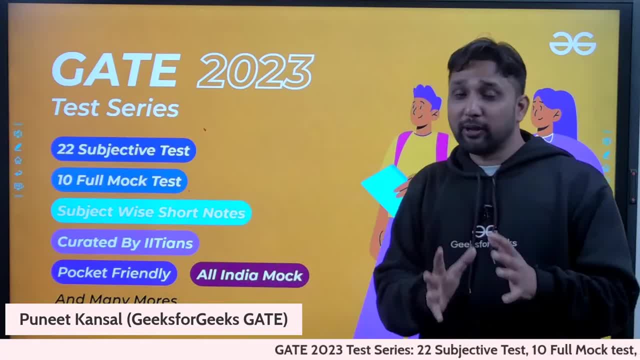 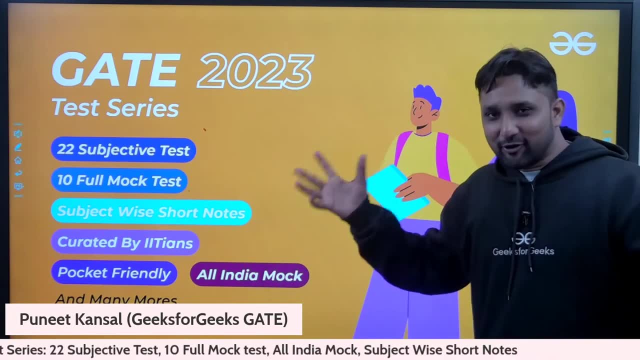 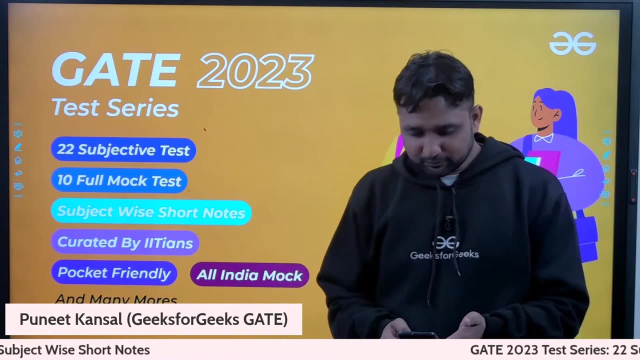 and if you are able to score good in this, believe me, you are going to get below 300 rank in gate also. Otherwise, what we can do is at least we can go for this free course, complete this free course. best of luck everyone. keep working hard. thank you. 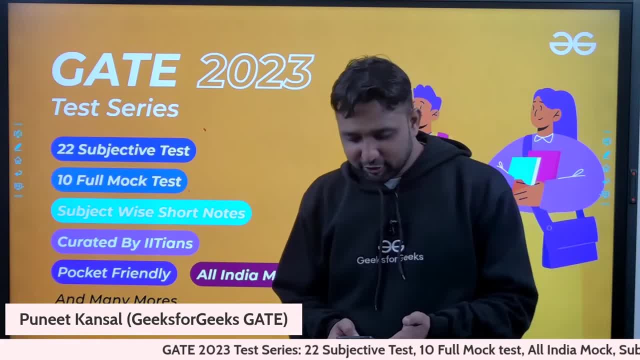 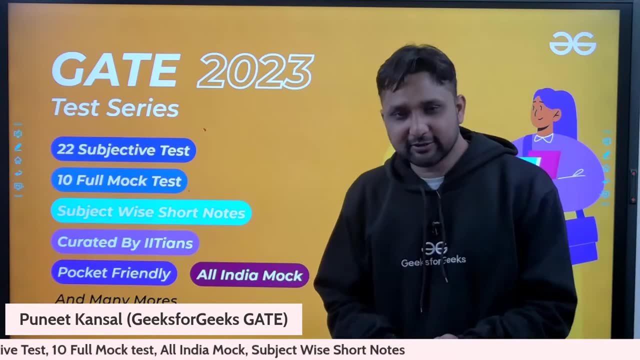 Thank you, Harsh, for this comment. thank you, Harsh, thank you everyone. thank you. thank you Jerry, thank you Veer. thank you everyone. So I am now ending the session. thanks, we will meet in the next lecture, okay. 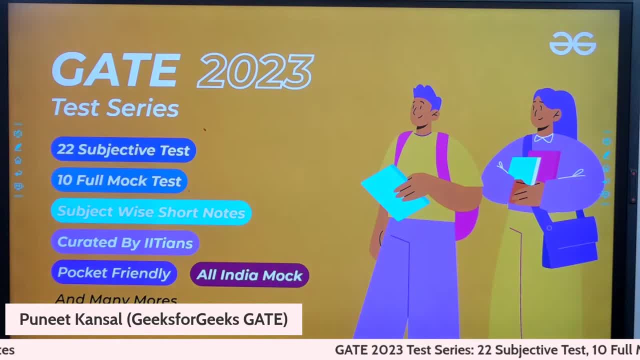 Okay. Subtitles by the Amaraorg community.